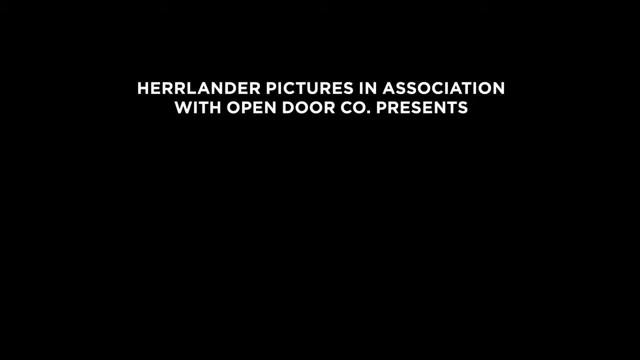 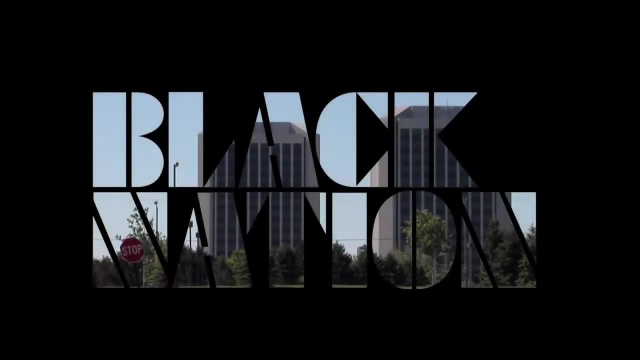 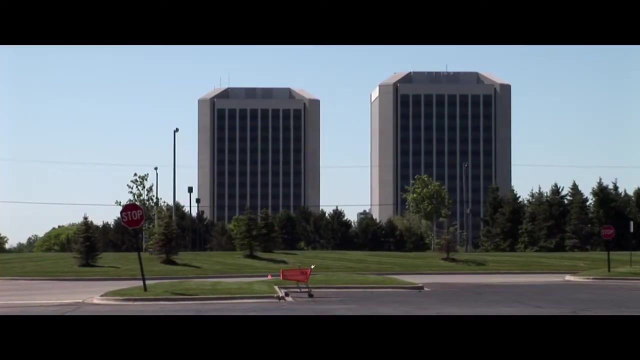 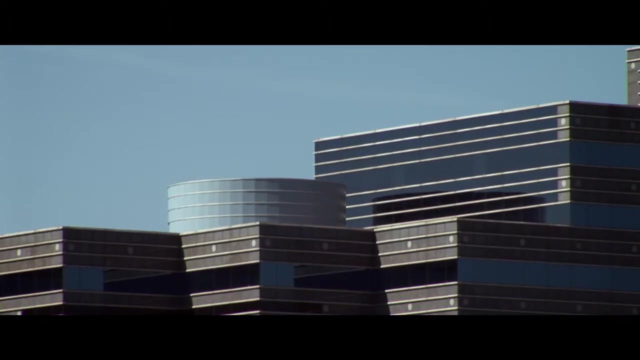 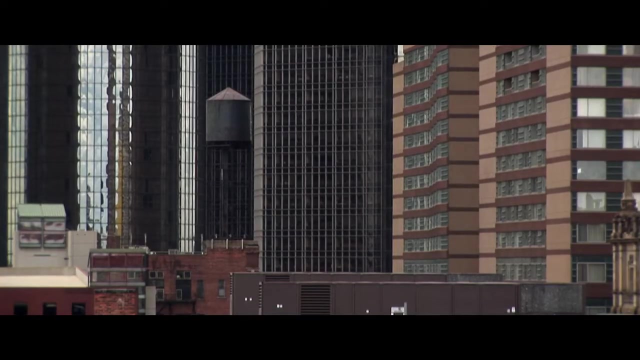 Thank you. We live in an enemy system. We live in a network of institutions that were created by and serve the interests of our oppressors, And you can only be a part of that institution if you're going to serve its interests. The old saying: people get the leadership they deserve. 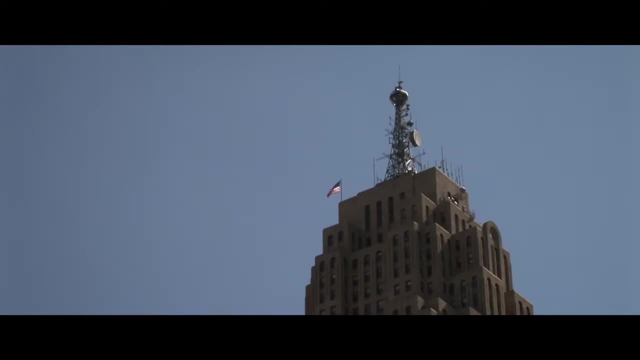 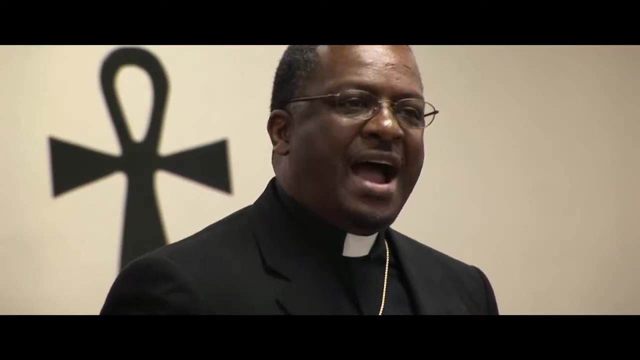 Well, America has the leadership it deserves. It wants that kind of leader Who is going to secure my life, My power And everybody else be damned. I don't care about y'all dying down there in the city. I don't care about homeless people. 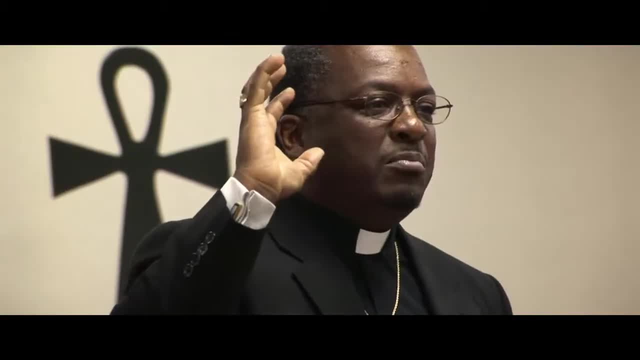 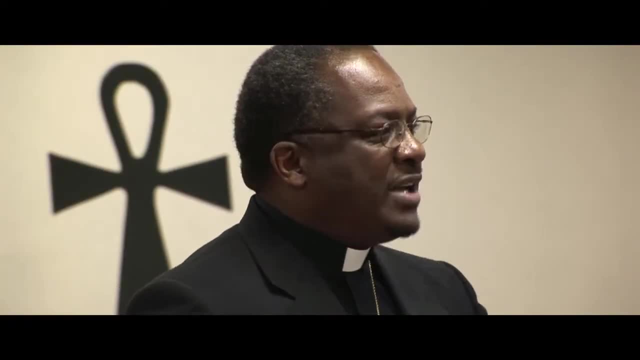 I don't care about no permanent underclass. I don't care about black people being warehoused in prison. I don't care about none of that. What I care about is I can stay out here with my 2.5 children. 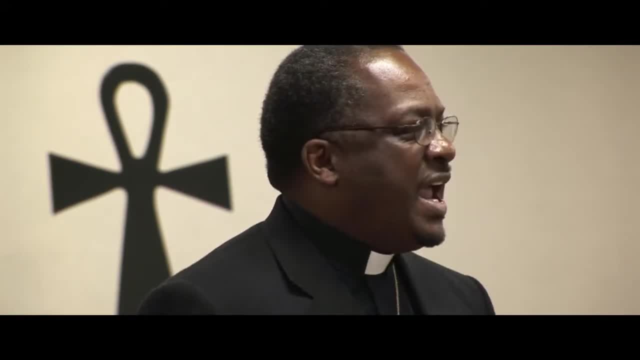 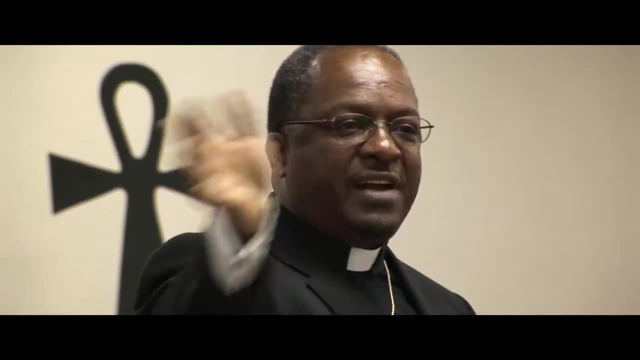 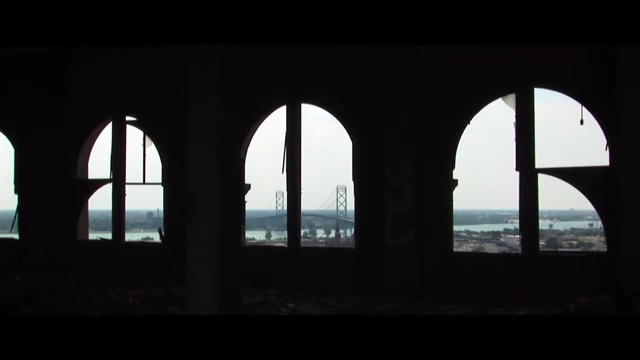 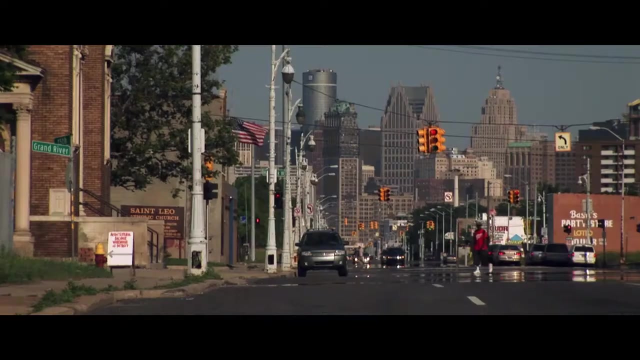 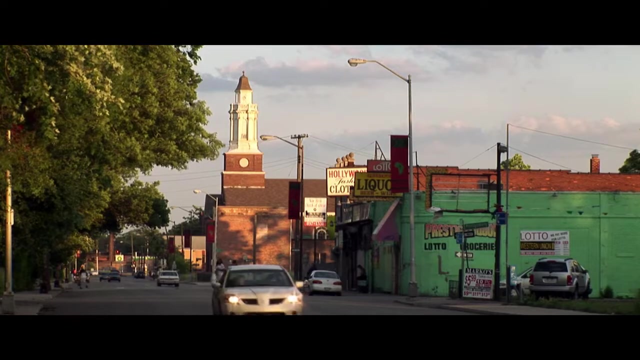 They can go to fine colleges, get decent jobs and I can live my sunset years on my boat, next to my lake, in my cabin, With my flag flying overhead. That's what I'm concerned about. Good morning brothers and sisters. Good morning brothers and sisters. 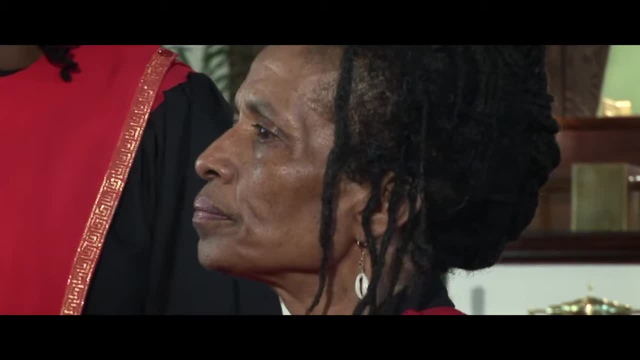 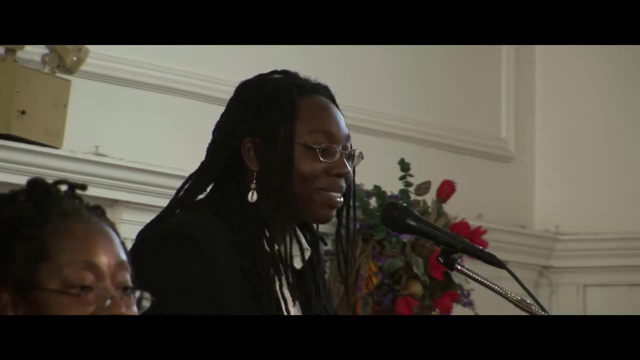 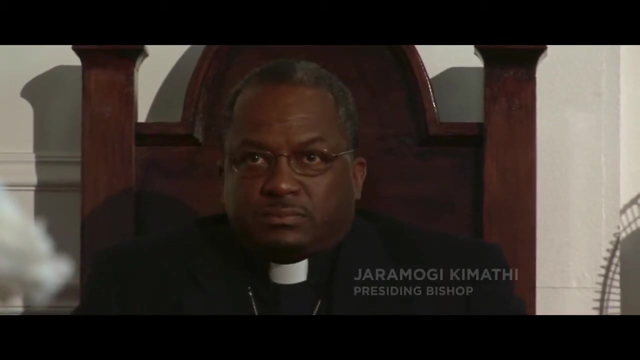 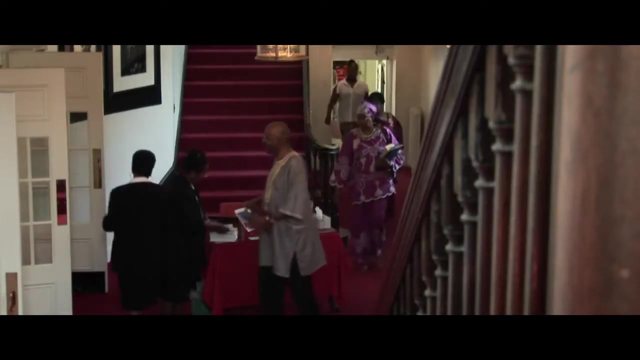 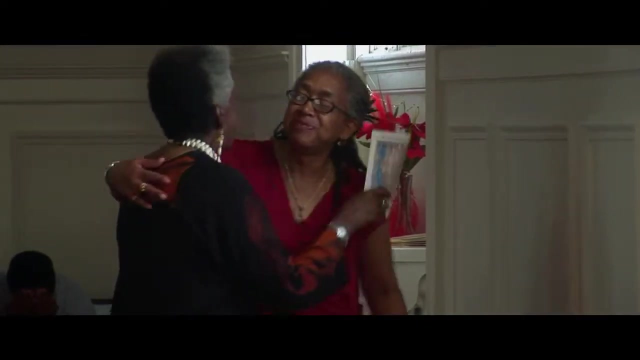 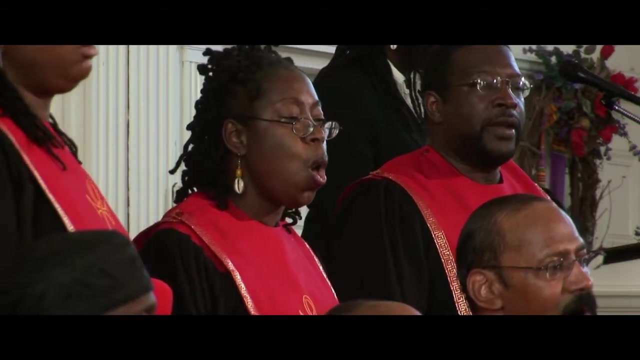 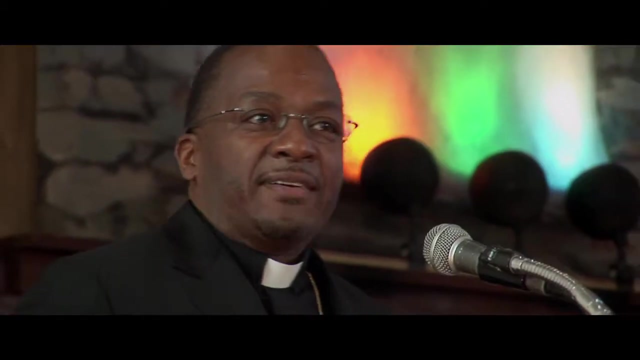 This is a glorious day. Not only is it the day that God has chosen to honor the brothers, Because today is Father's Day. Today is Father's Day, Hallelujah, Amen. Let the congregation say Amen, Amen. Can I get a Father's Day? Amen? 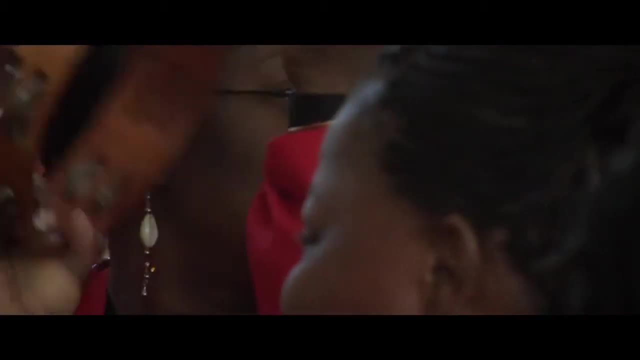 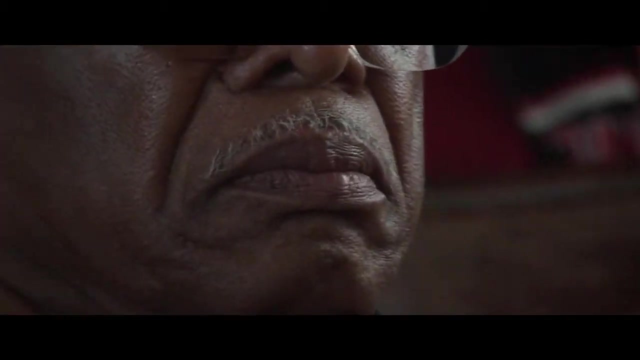 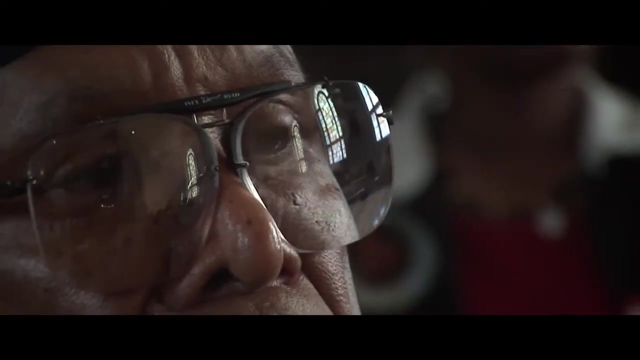 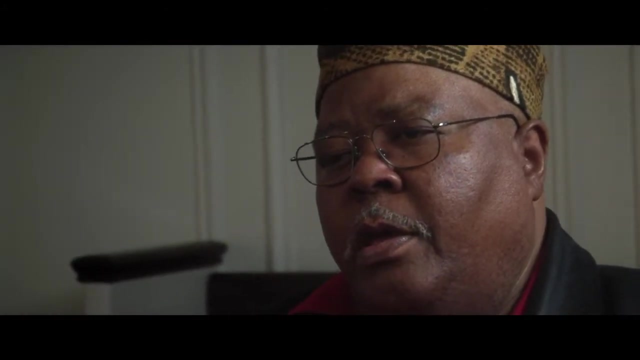 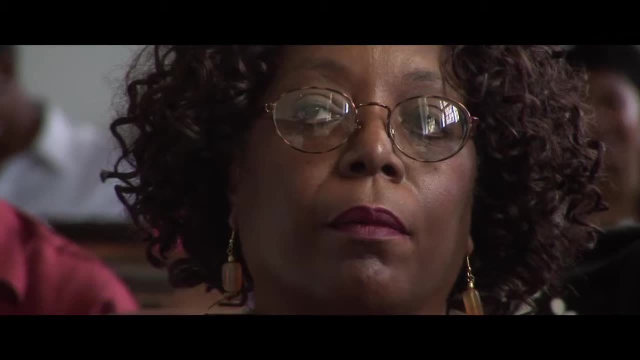 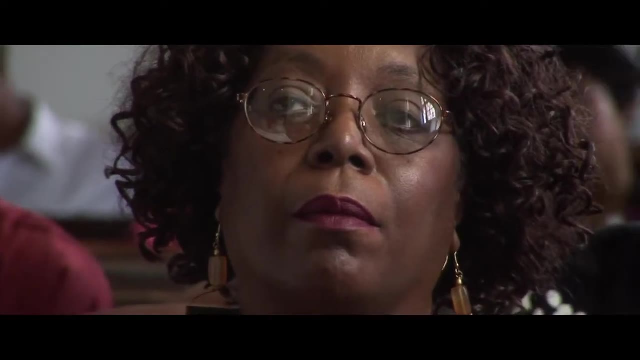 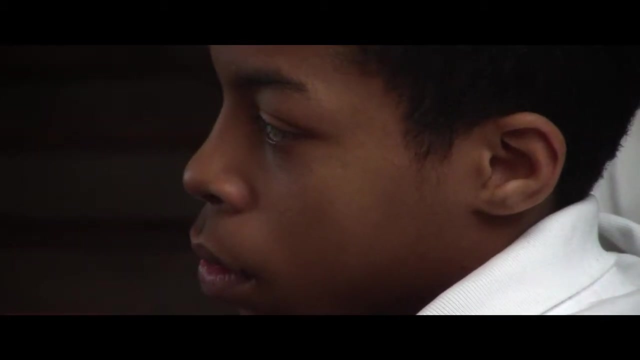 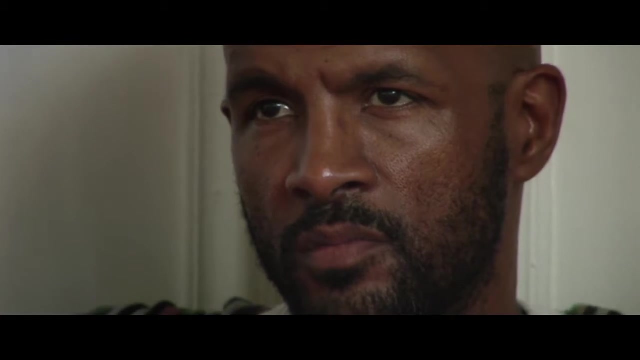 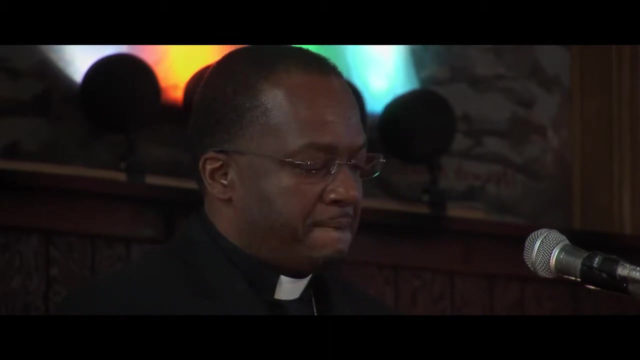 this is not just a problem for black men. it's a problem for the whole black community. see, manhood is not about male machismo or male ego. manhood is a quality. it's a quality. manhood is characterized by strength, bravery, self-reliance, responsibility. manhood dreams big dreams. manhood makes a way. 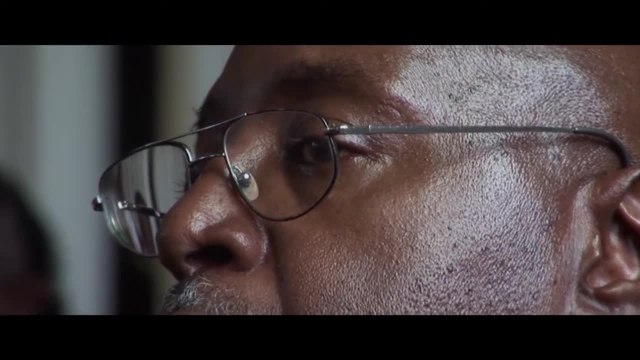 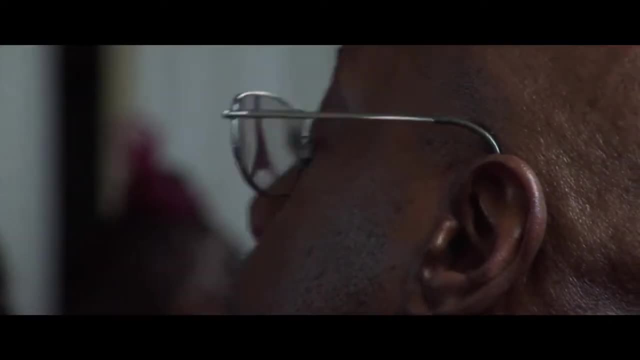 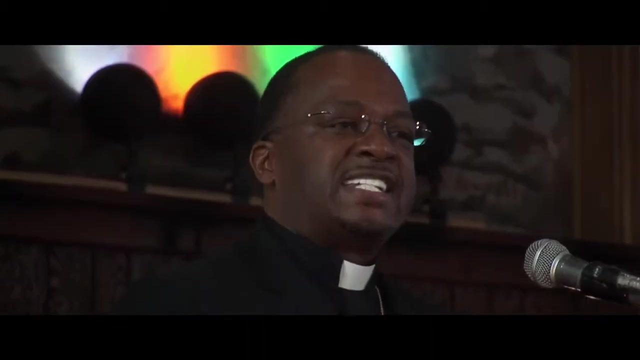 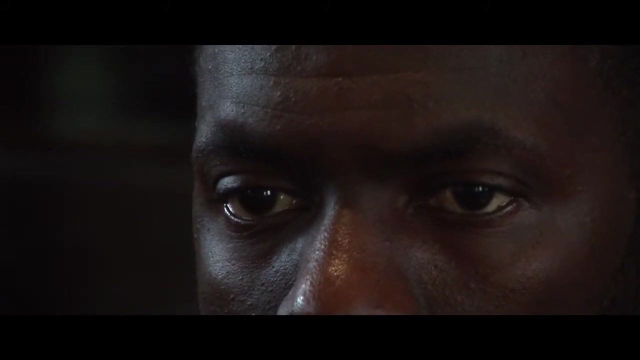 out of no way. manhood is essentially about dignity, the value that God built into every human being. it means you have value. when you believe you have value, you do not let people treat you as if you don't have value. so when people have a difficulty celebrating manhood, we are saying something about ourselves. we have 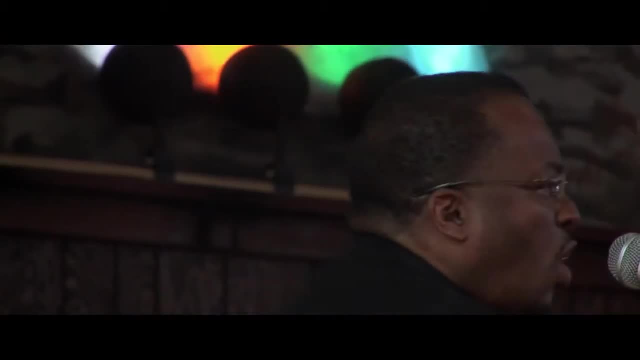 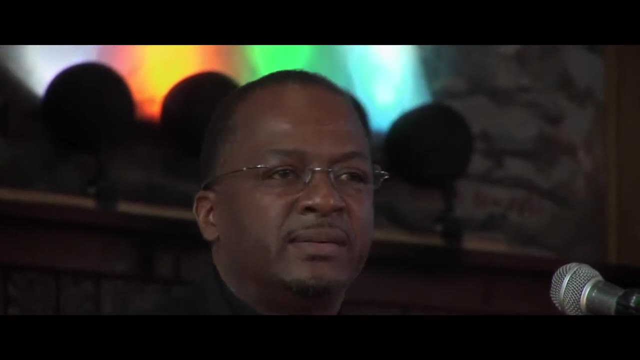 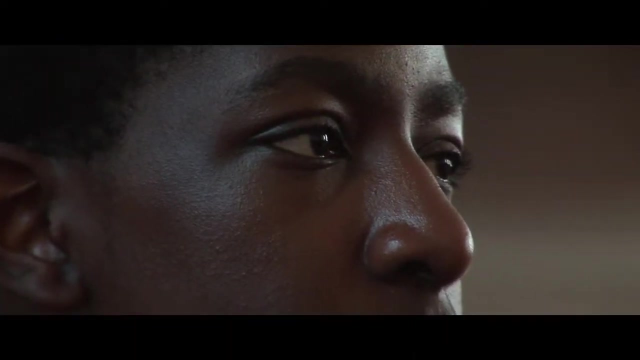 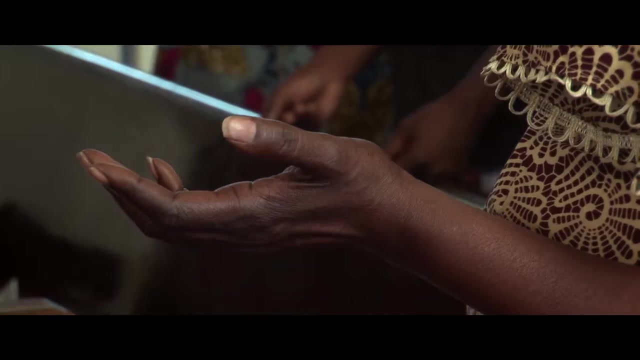 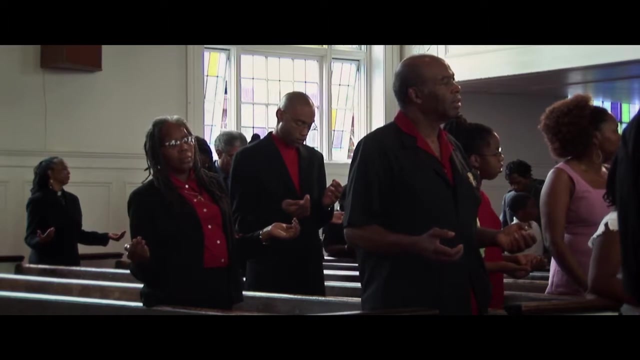 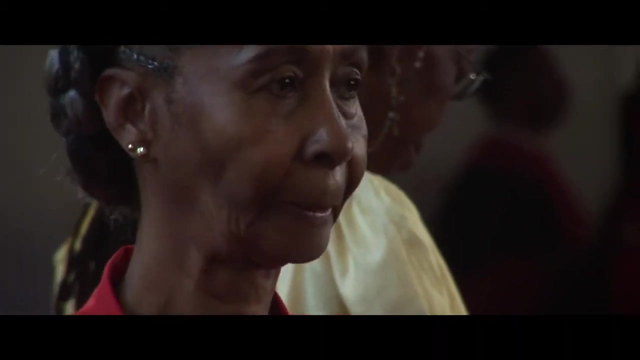 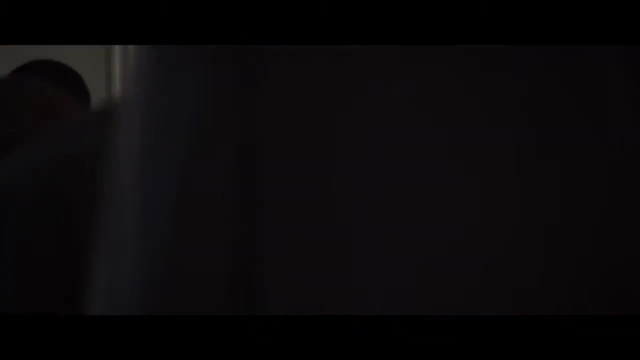 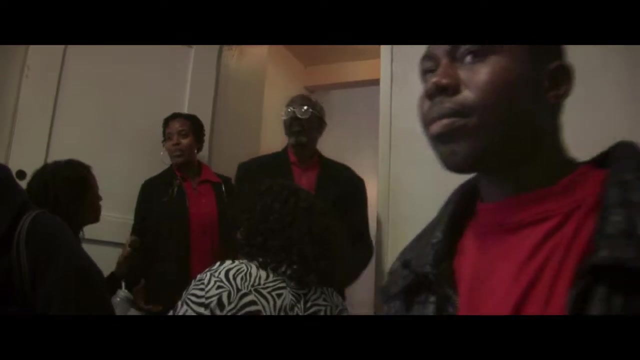 difficulty celebrating courage is because we're losing courage. If we have difficulty celebrating honesty, it's because we're losing honesty. And if we have difficulty celebrating manhood, it's because we're losing manhood. You a gangster man, Huh. 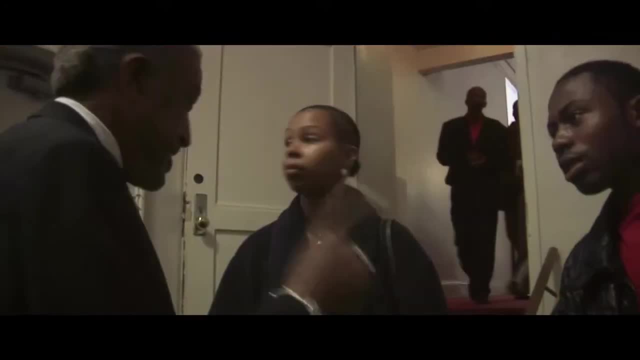 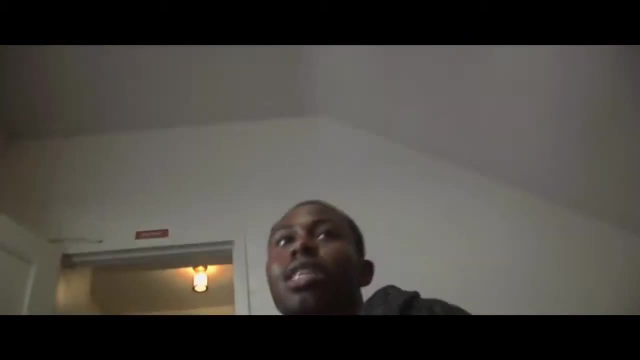 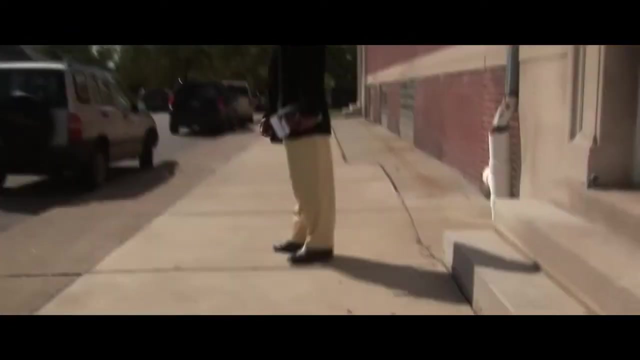 You a gangster. I don't know why he says that. I don't know why he says that in church, Where you at now About to go home. You need a ride, So let's go. So, Orlando, how you been. 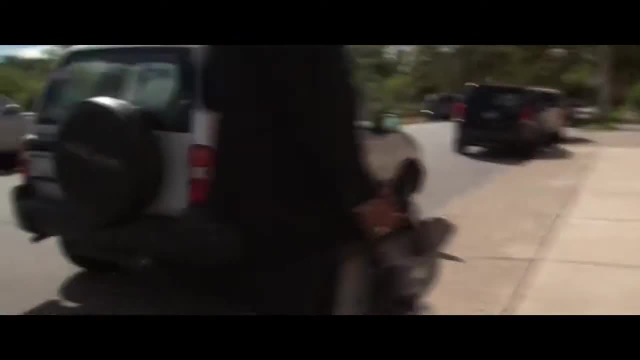 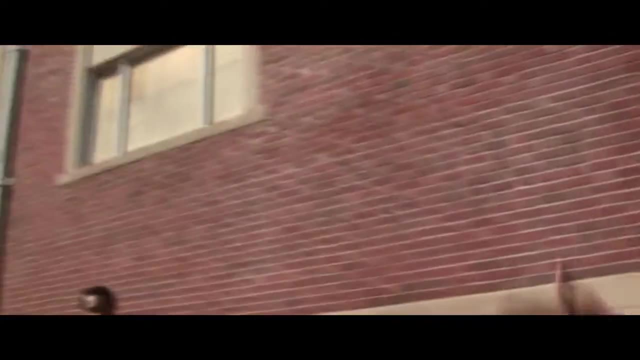 You know me: stay in the projects, do my thing. the main thing, Orlando, why don't you stop that? That is what I'm up to. That's where you grew up. You are not in a project. You live in a subsidized housing in a high rise. 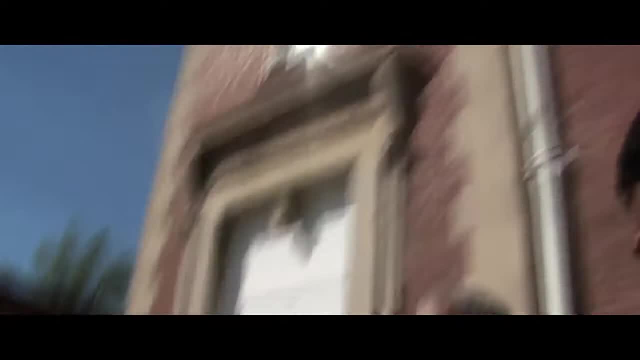 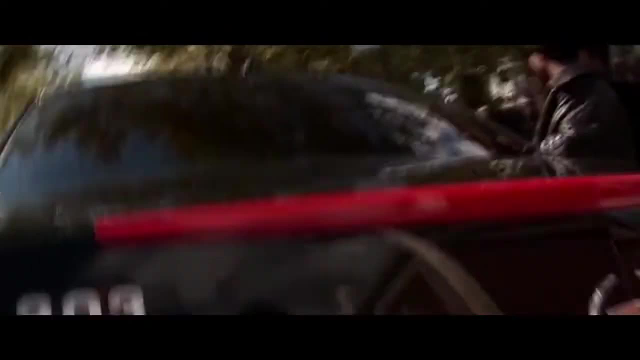 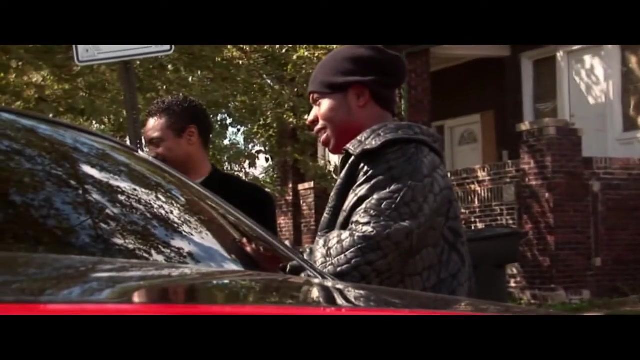 You were raised, You were born in the projects. You need to get out of that mindset. Start by telling the truth, Orlando, So that's not the truth. It's not the truth. You're not independent. singing and whining and singing that song. 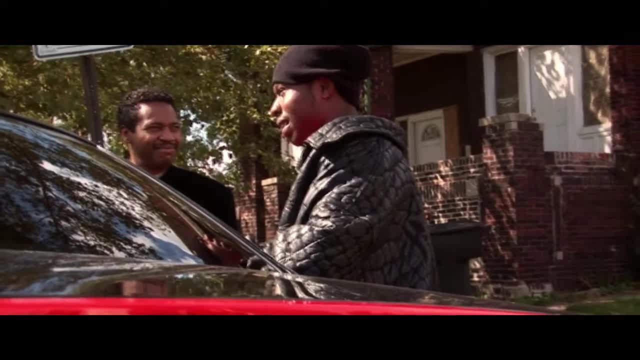 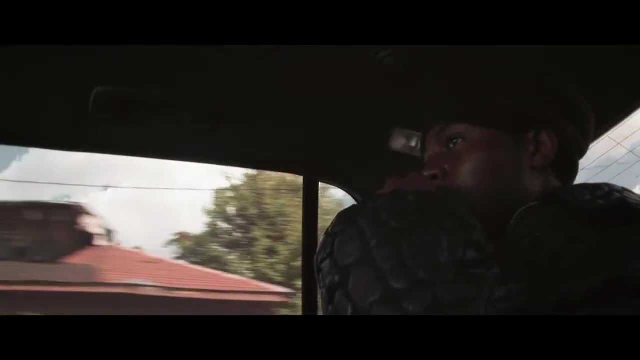 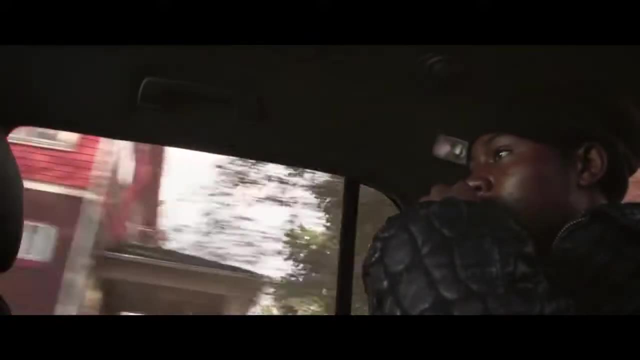 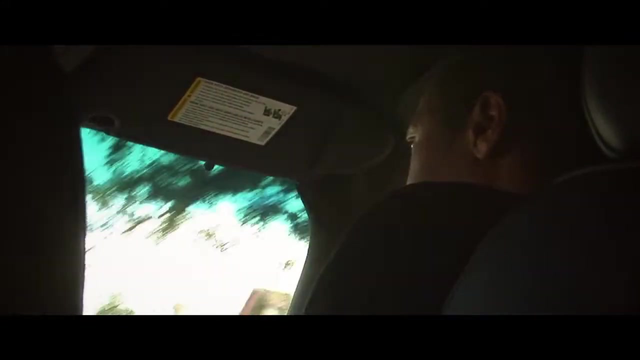 You have every opportunity. Listen to the cardinal. You have every opportunity for success if you let yourself have it. Yeah Shoot. I grew up all around Couple of places on the east side: Glenfield Street, Greensboro Street, seven mile out of drive area. 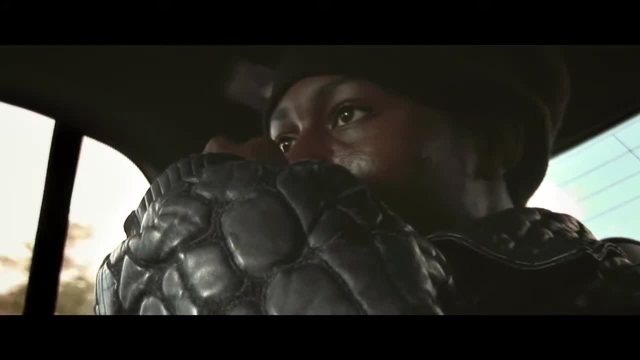 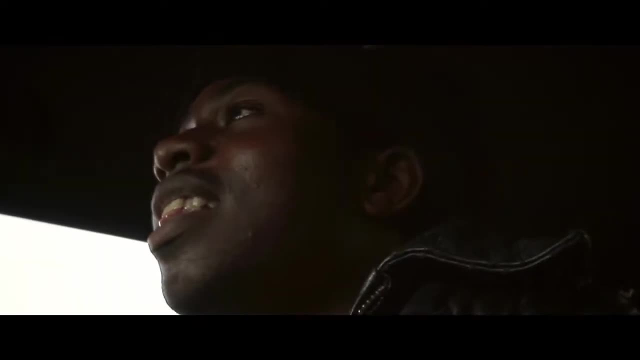 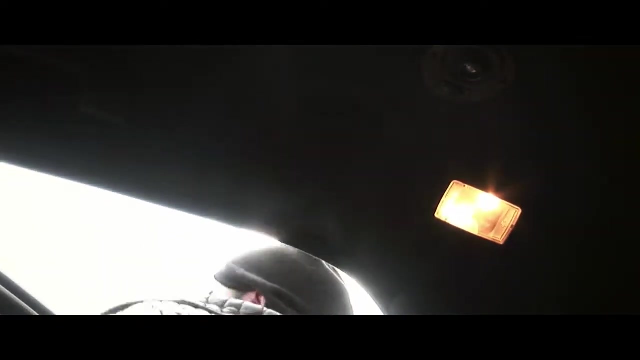 Right now I got my father staying with me until he get on his feet. I'll see you later, Orlando, Give me a call. Thanks, Mark, I appreciate the ride. See you everybody. OK, See you All right. 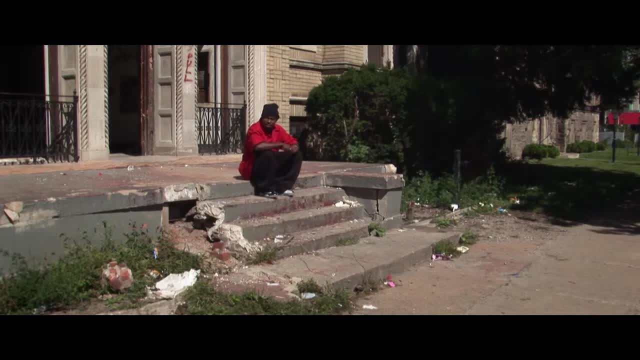 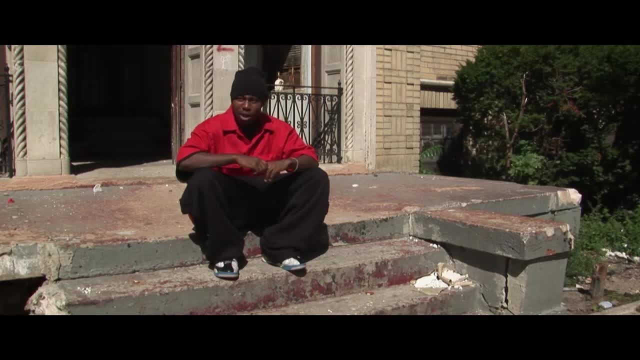 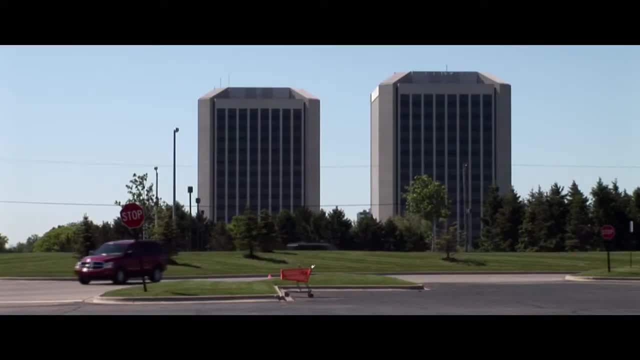 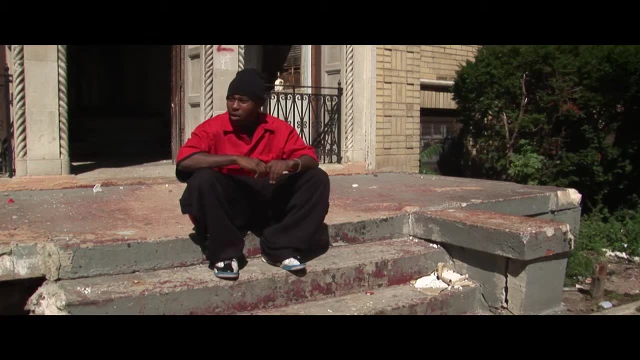 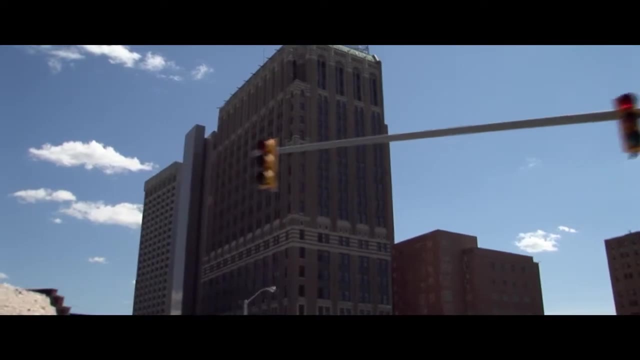 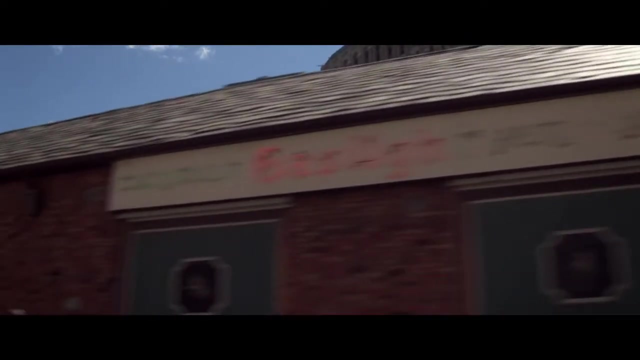 on second and Blane. Right now I don't work no more. I got into it with somebody at my job. I was working in a new center area just picking up papers, Keeping the area clean, basically. He told me to come back at a certain time. I wasn't looking at the clock and I was doing my job and 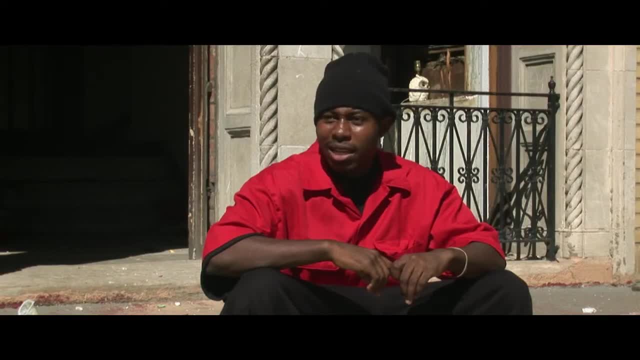 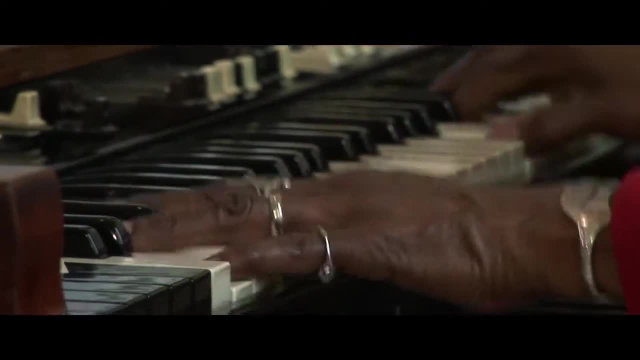 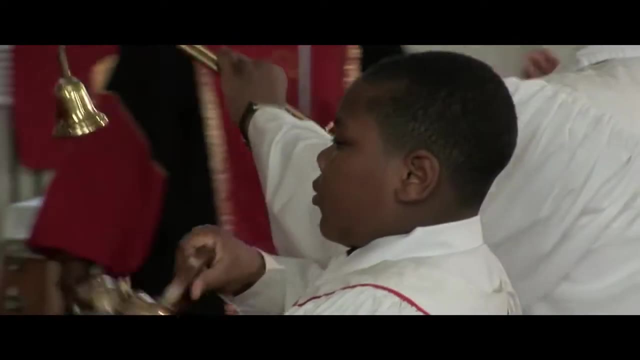 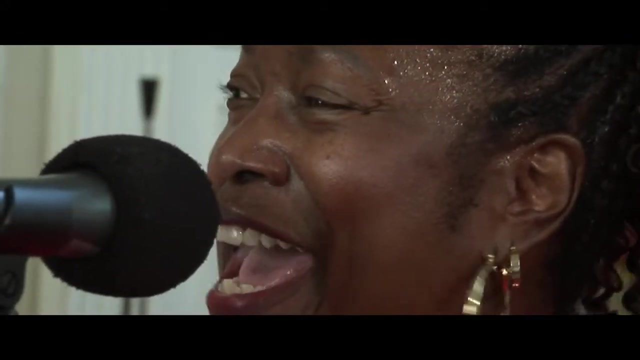 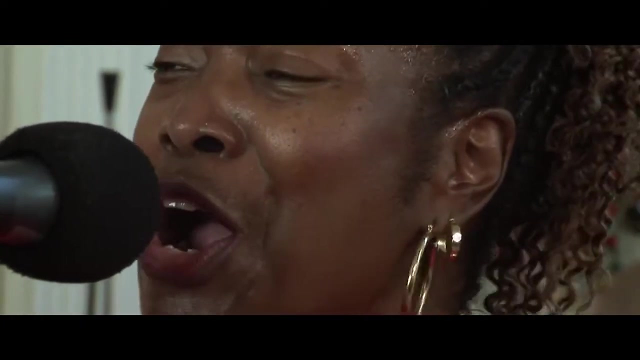 He started just talking crazy man, so I just left, man, and I ain't never go back. We walk in the light, Beautiful. Oh, Come on, come on, Come on way. Oh, Don't do drop Mercy that. shine so bright, then shine all around us. 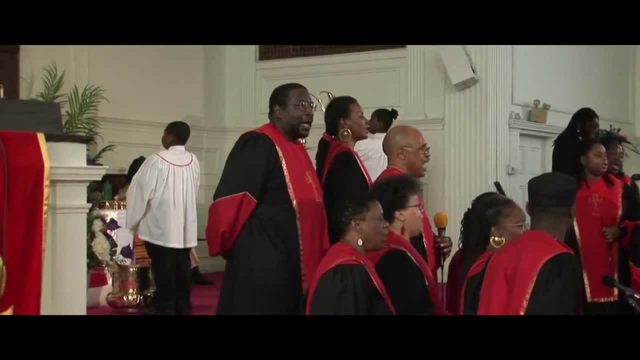 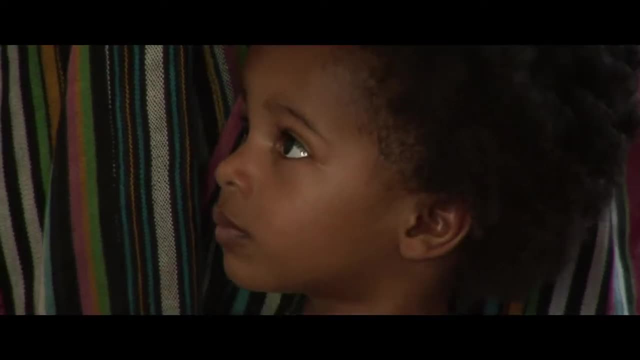 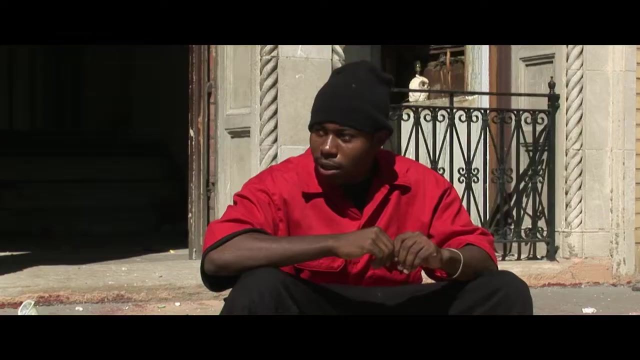 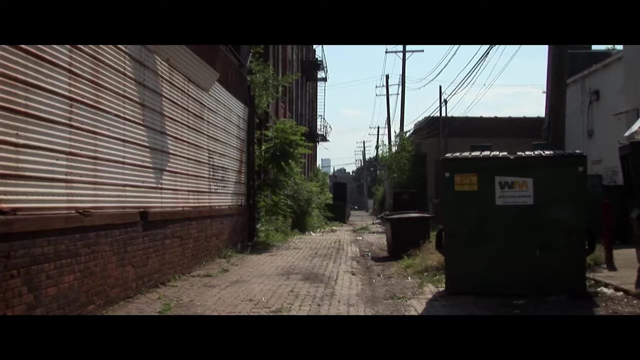 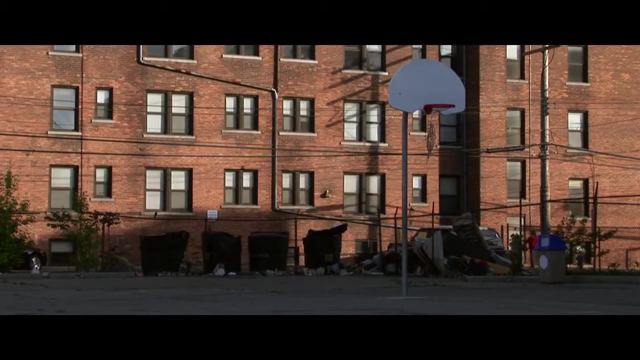 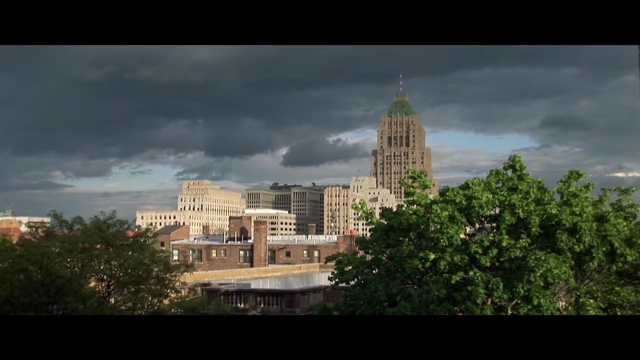 Begging you Lord by day, And now Cause Jesus. Oh, He's a lie, He's the light of the world. We In the night, Yeah, Beautiful light, Come on, come on, Come on way. Oh the dewdrop, Oh, The crisis of the black male is the single most devastating problem facing black people today, and 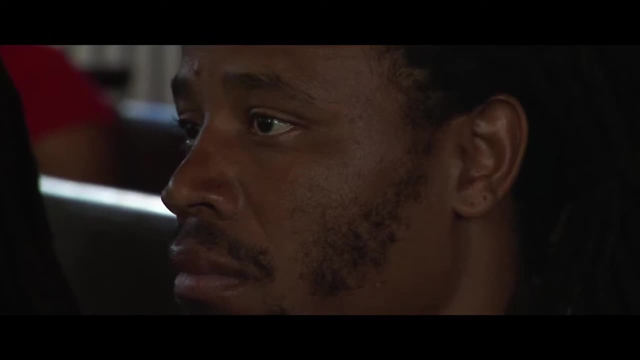 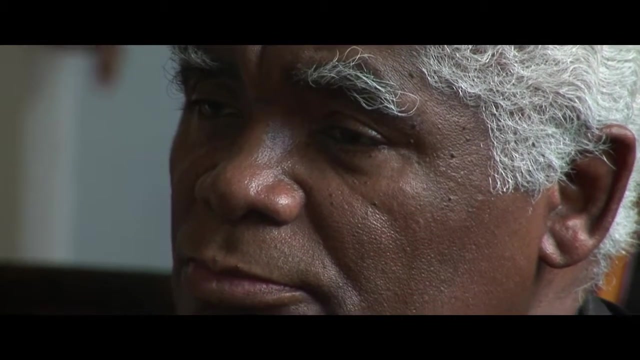 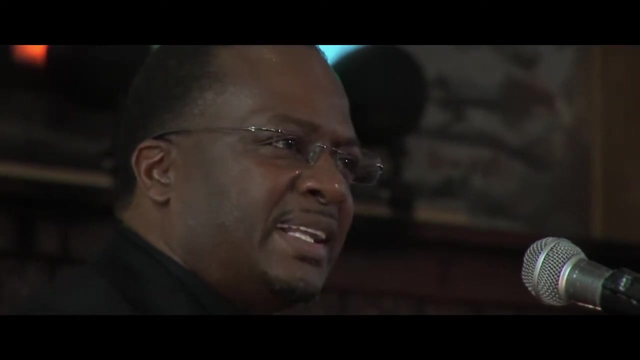 We are, according to the New York Times, sleeping through the Holocaust. There hasn't been a genocidal violence. this devastated the black people since the slave trade. You have noticed? You haven't noticed that Black men are being systematically destroyed? the Everybody's having a hard time? I'm not kind of trying to compare suffering, but black men are being. 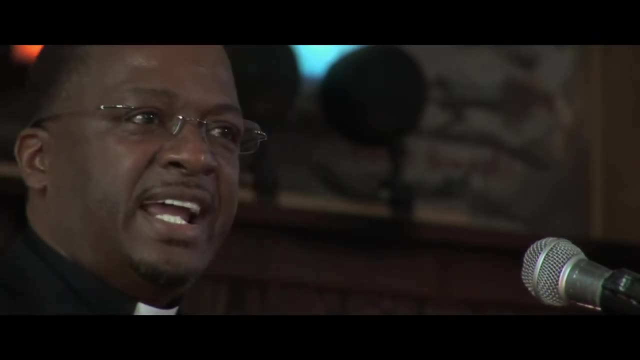 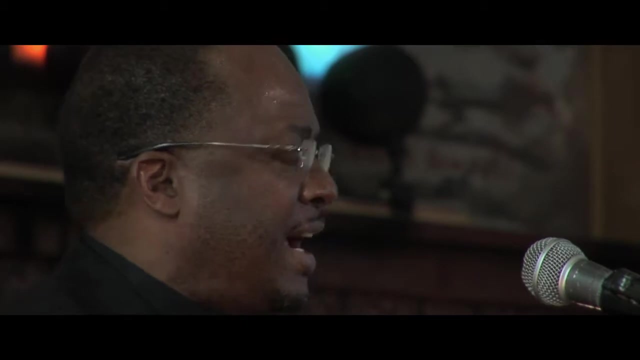 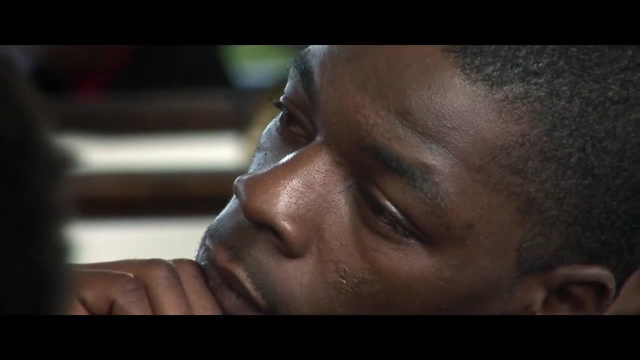 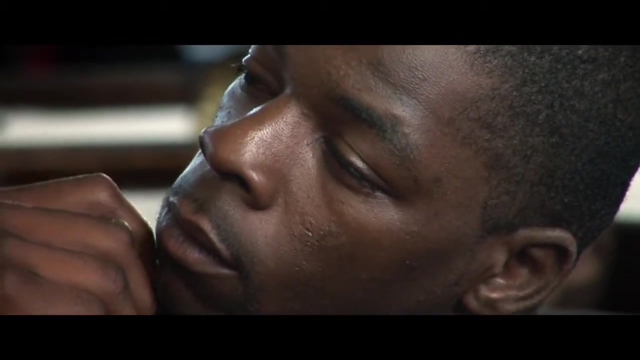 systematically wiped off the earth, not intentionally. There's nobody's playing. It's a convergence of negative problem. at the same time, and the makers aware of this. the National Urban League's report for 2007 is dedicated Solo to the crisis in childhood, to the crisis of black men and black manhood, and this report reports that one. 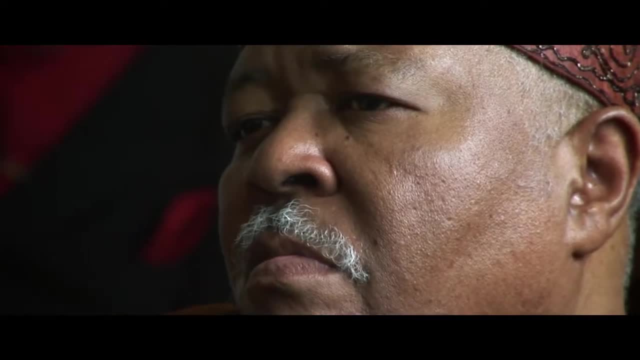 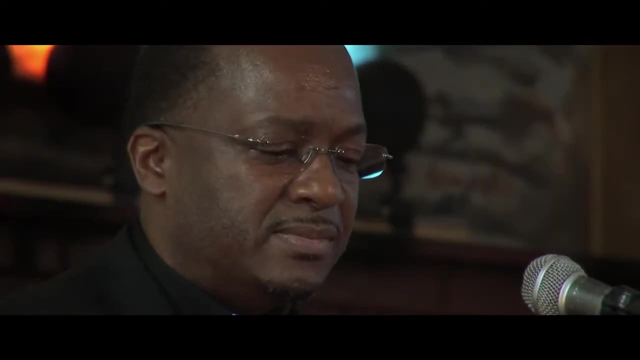 in every three black men is tied up with the penal system and it's projected by 2020, two of every three, two of every three, will be tied up with the penal system. it reports to 20% of black men have been eliminated for voting came. 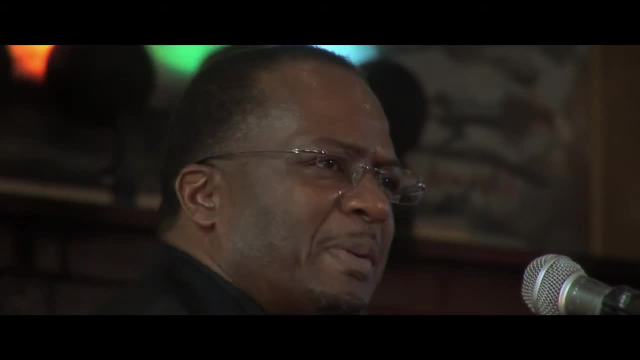 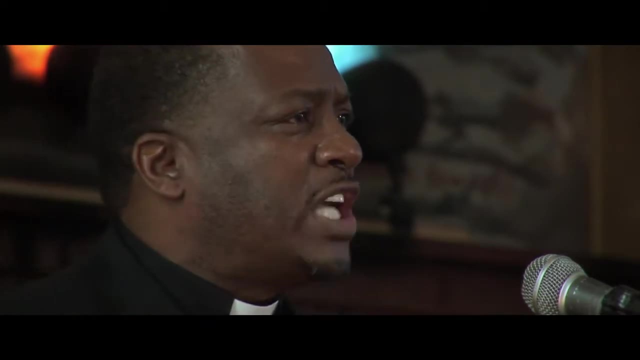 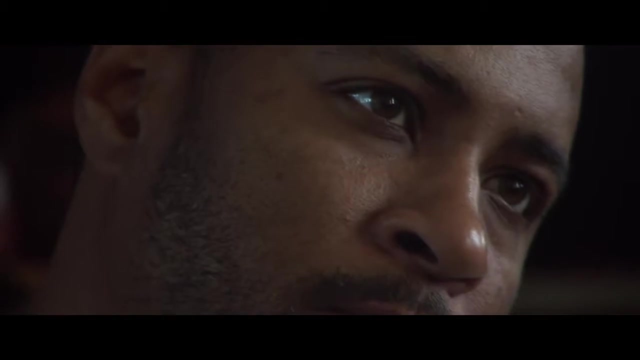 both came, both 20%. 20% of change. a whole lot of elections 20% would have had. would not. if we've gotten that, didn't do it. eight years of George Bush. if 20% of black men could vote fully, 20% can't vote because they got felonies on their. 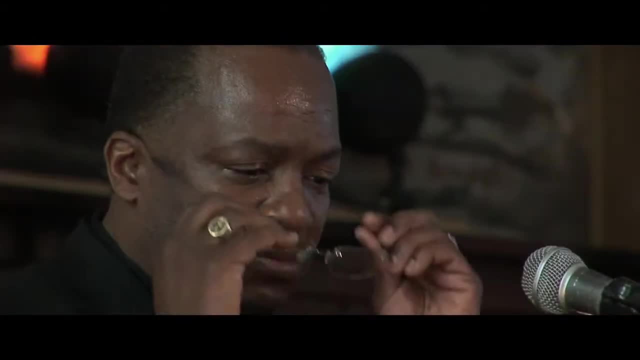 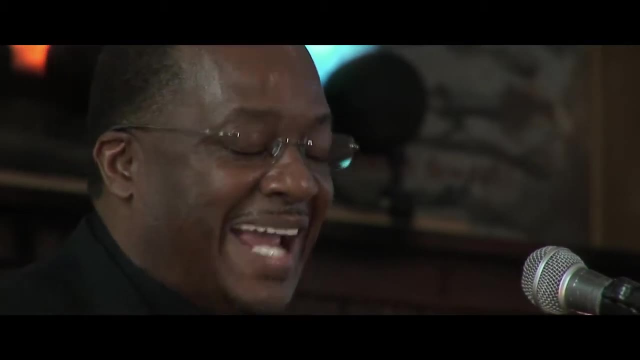 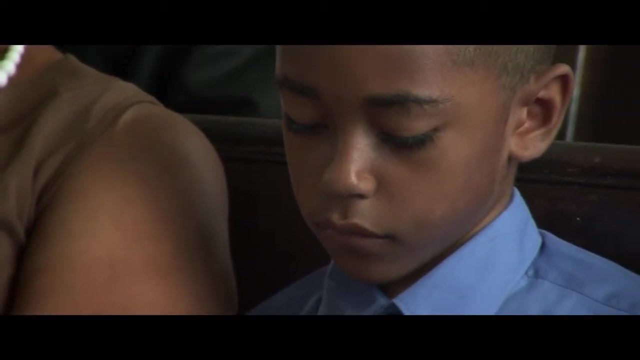 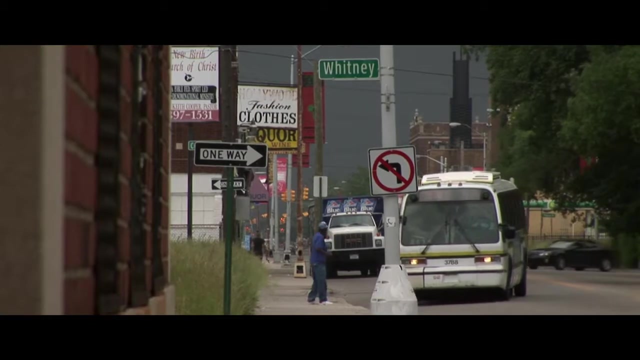 records and they've been disenfranchised, can't vote. the report goes on to say that the dropout rates in city among black mail is as high as 80%- 80%. how do you grow up in a knowledge world with no knowledge? the report goes on to say that 50% of black males are unemployed. that's. 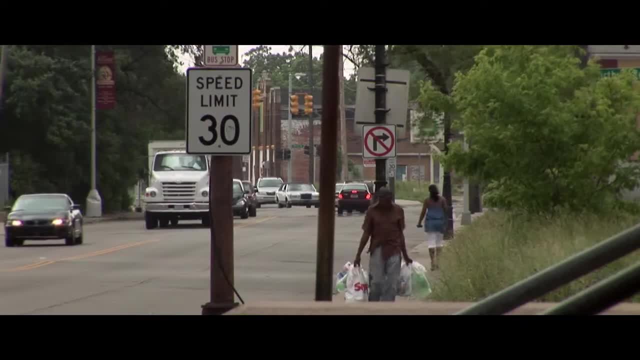 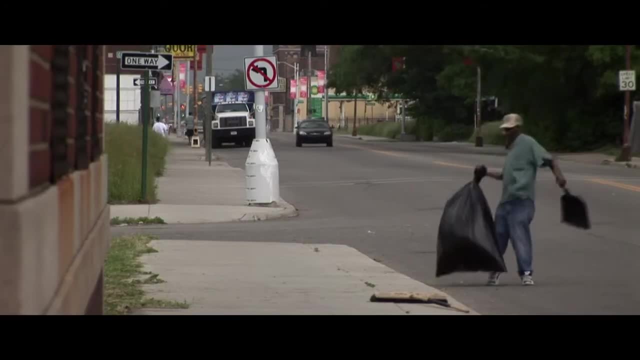 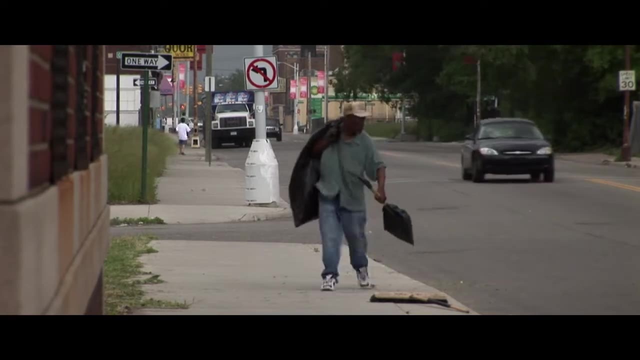 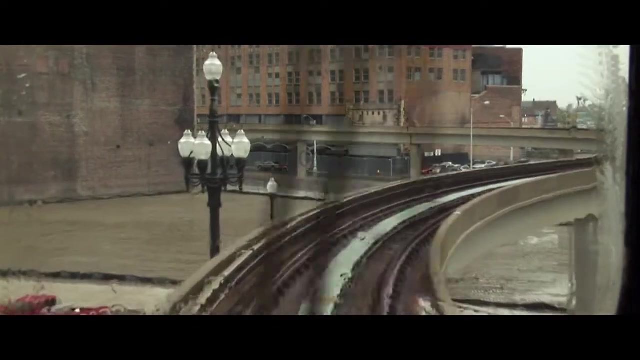 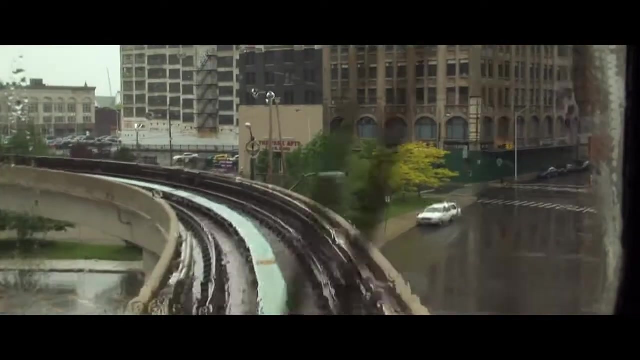 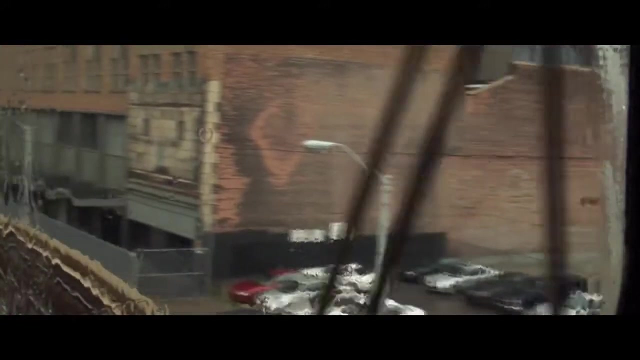 half of the men in the country ain't got a place to go to work a job. can't bring the check home. spices 24-7. you Detroit, a unique city in America during the beginning of the 20th century, right after the depression, the auto. 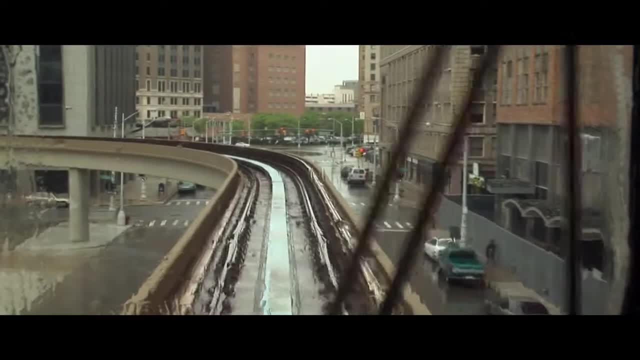 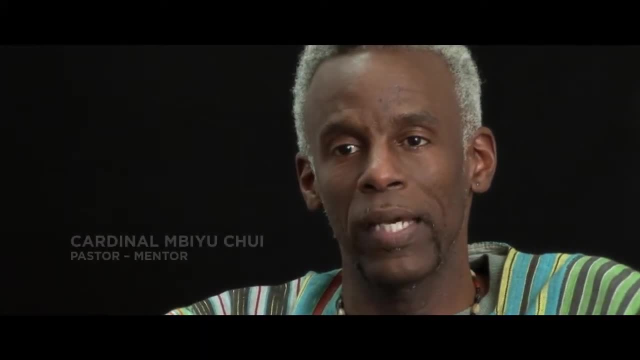 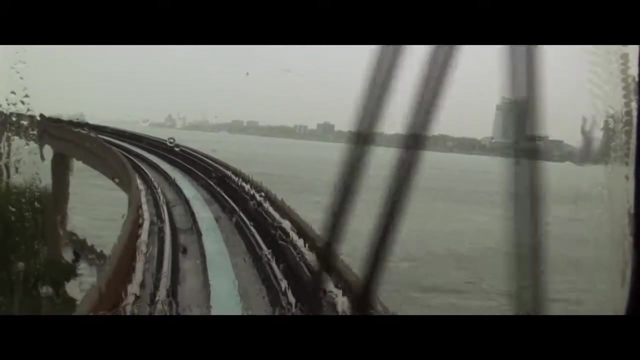 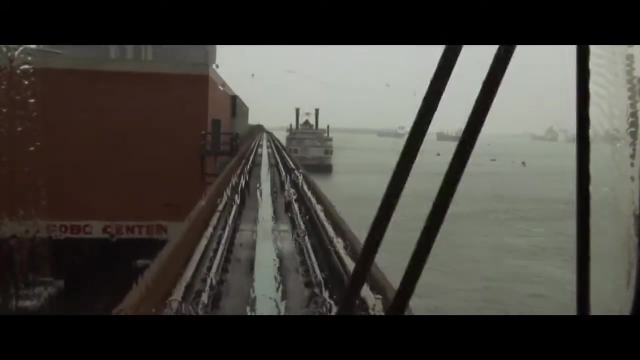 industry began to grow, and so you could come to Detroit and get a job at one of the auto industry plants and find a decent living, and that's what happened. so a lot of black folks from Alabama, from Georgia, from South Carolina began to move their families slowly from the south to the north. 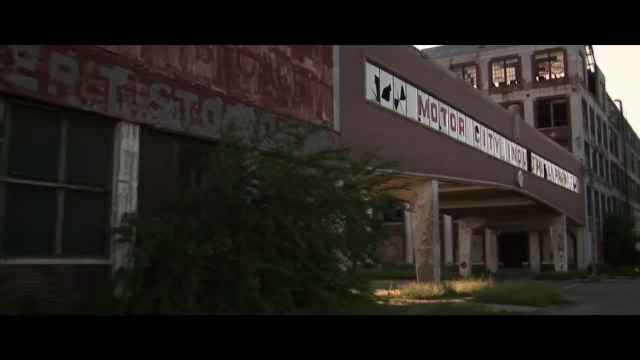 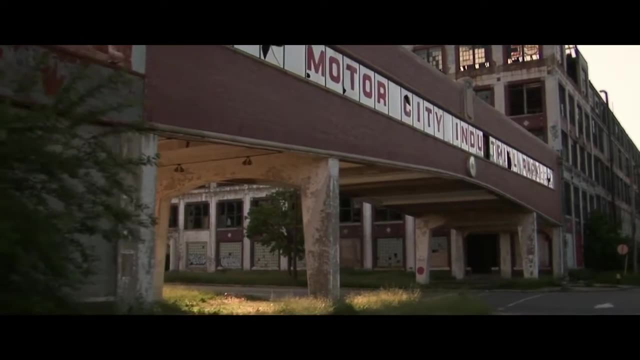 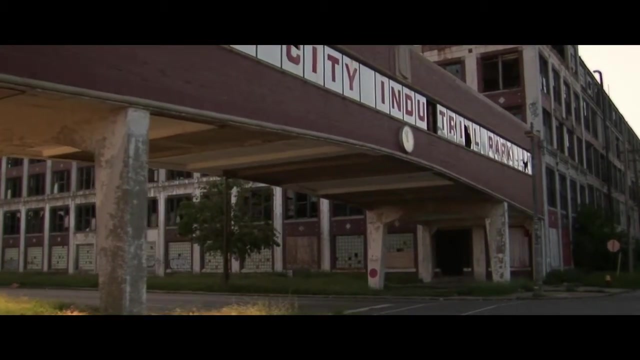 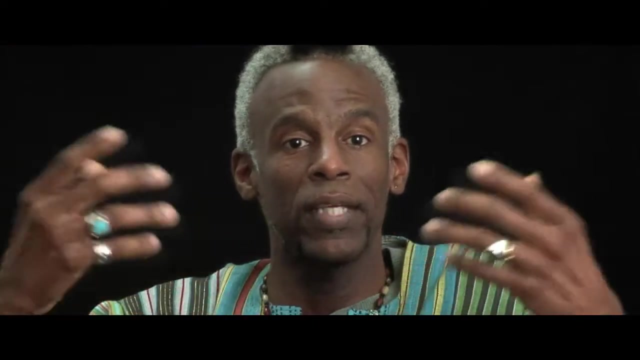 you. but after the economic boom of the 70s and 80s and we started moving from industrialization to post-industrialization, with robots and machines and computers doing everything, the unskilled labor of black people began to become obsolete, so the jobs began to disappear. 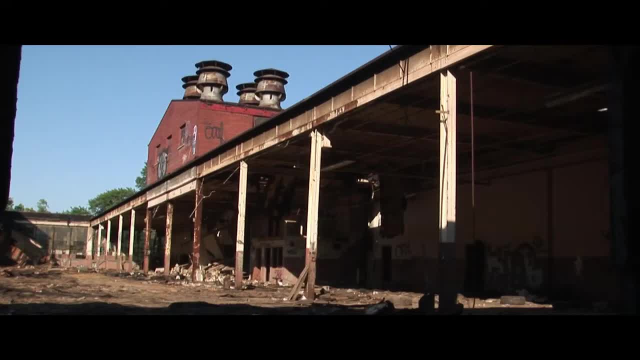 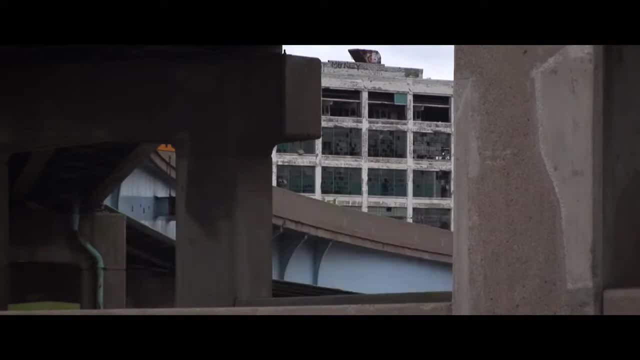 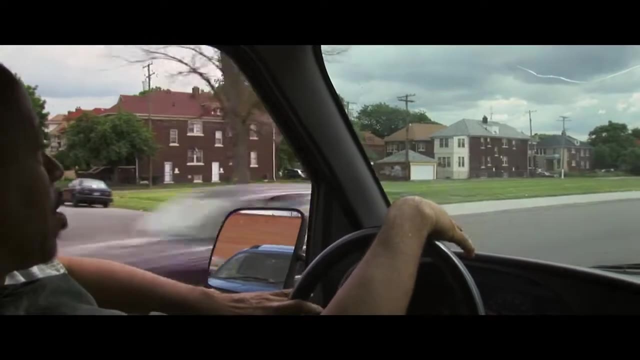 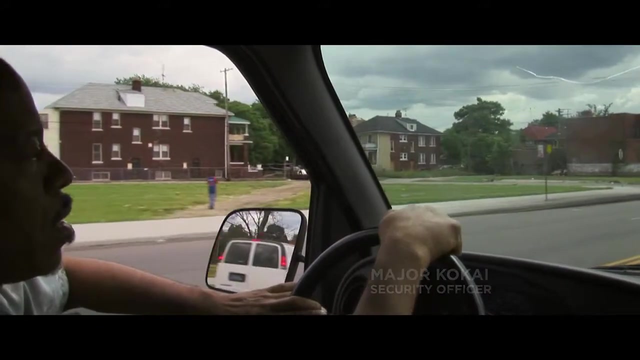 they treated Detroit like you know how you have an embargo on a foreign country. I feel like they did that with Detroit because they had a saying here like the last one out of Detroit: turn off the lights. you know businesses were leaving a lot of the plants. the automobile plants actually closed and automobile plant might have 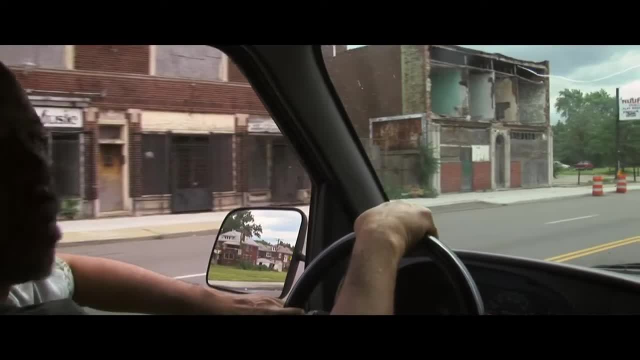 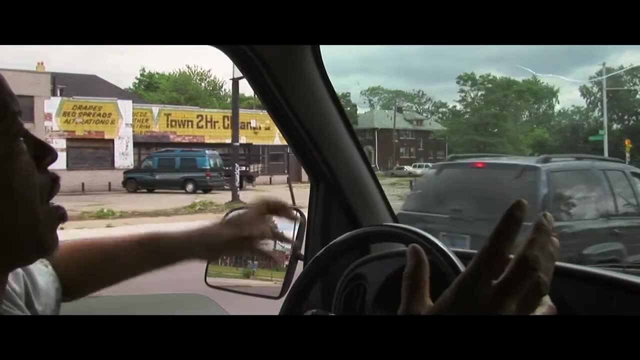 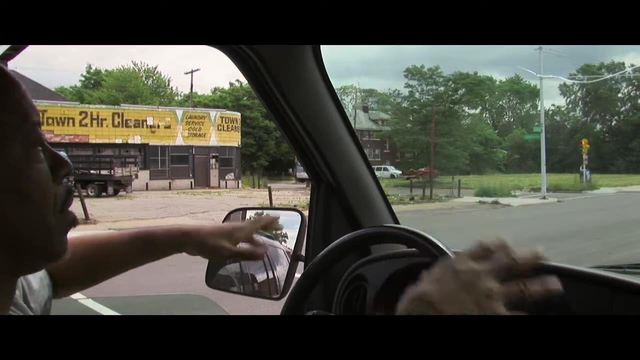 like 10,000 workers for that plant, you know, because they were working three shifts. and then you add in all the little businesses that made parts for that plant, or the restaurants, or you know whatever supplied that plant, you know. 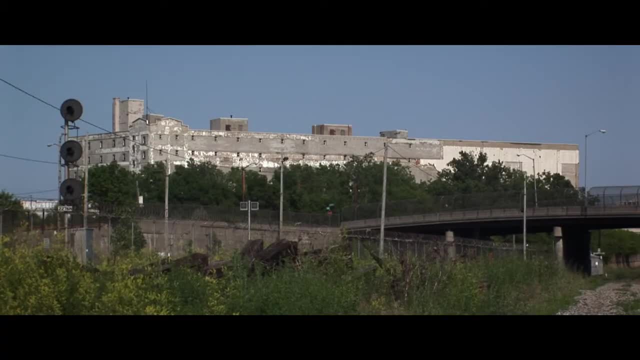 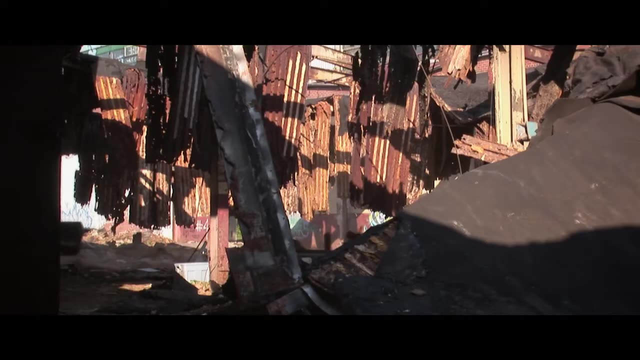 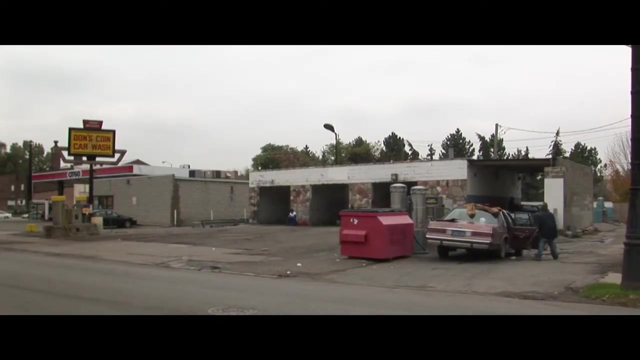 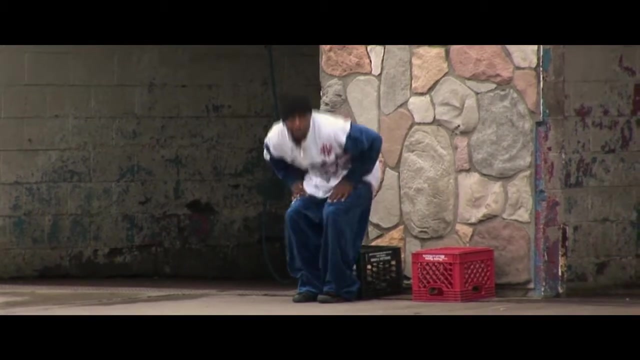 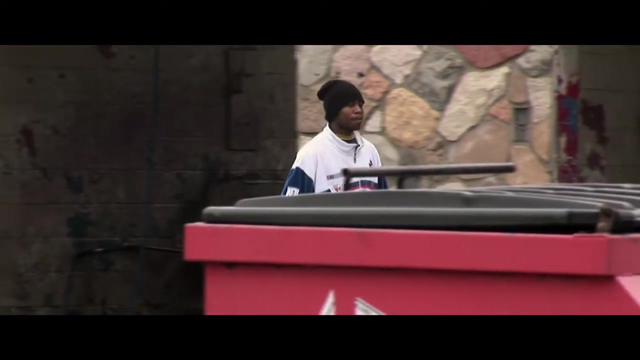 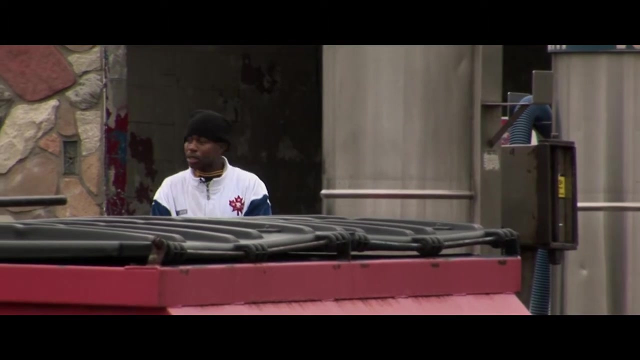 and so one plant could be 20,000 jobs gone. True man, I sell everything, man. I call myself the greatest hustler man because I sell CDs, DVDs, incense, clothes, Trying to chase some money. That's about it. 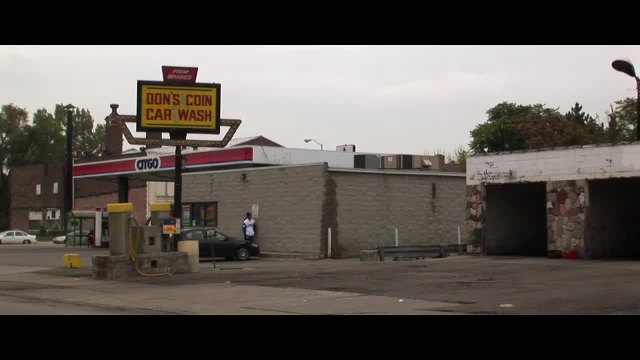 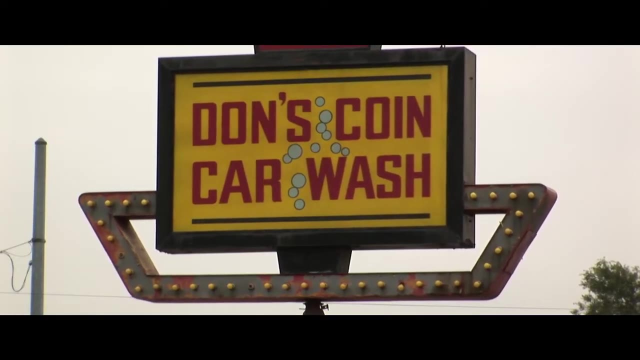 I'm trying to get a fee. I need the whole dollars. Oh, come on man. All right, stay right here. I'm about to get changed. All right, You can let me get in on that. Oh, you want to get in on it? 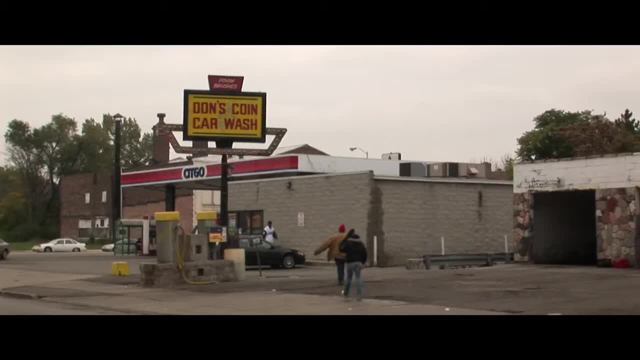 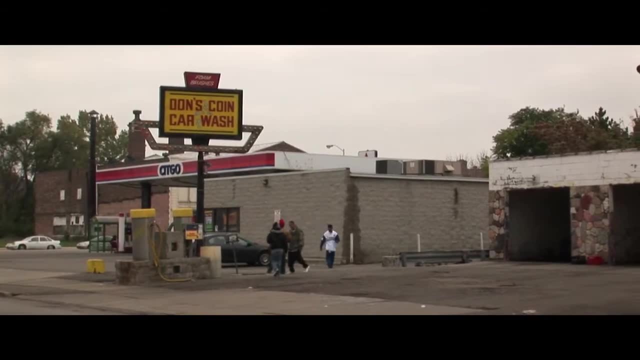 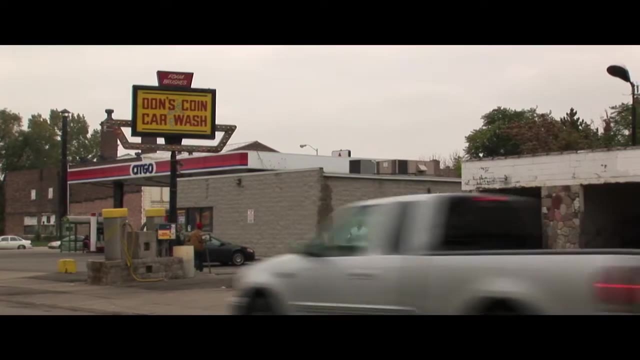 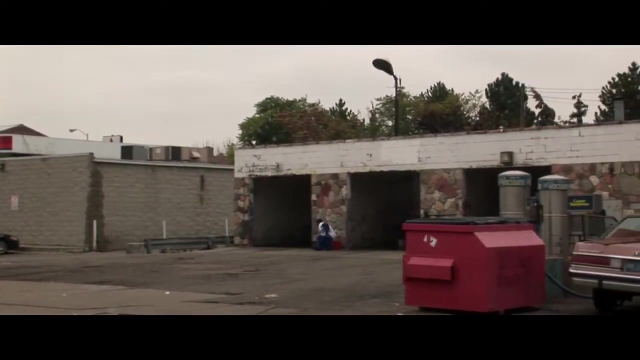 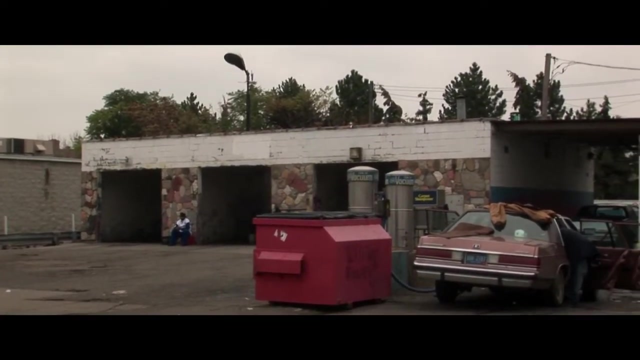 All right, All right. My family been poor generation to generation to generation man, My grandfather, my father, my mother, her mother, My parents did the best they could, but it's like, since they grew up, like me, like they ain't really high much. 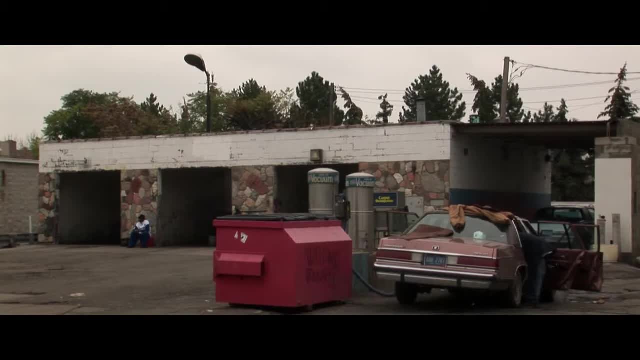 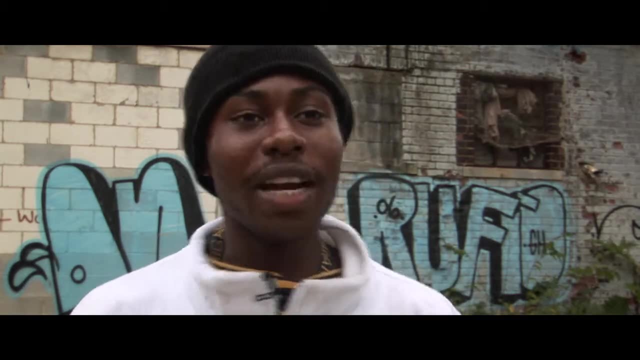 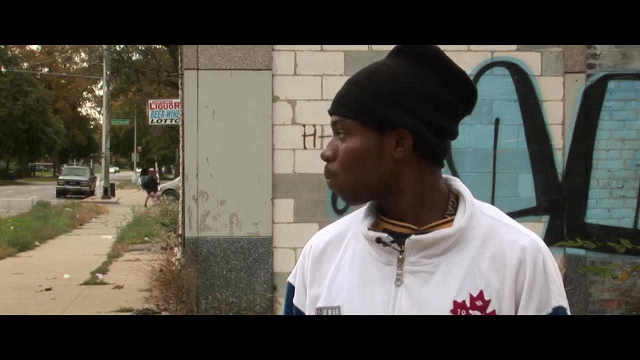 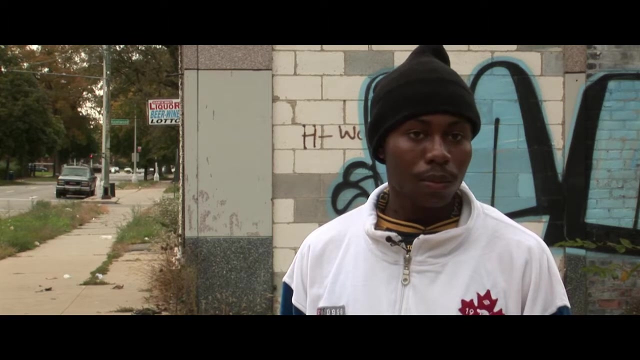 They ain't really. I can't really explain it, but it's like it could have been better if they had a better childhood. That's what I'm going to say. I chose as a topic today the pathway of the heart. 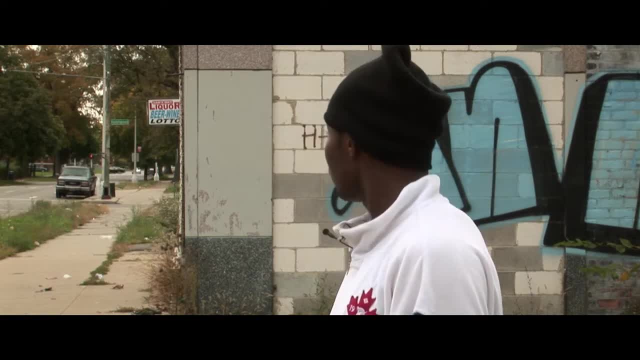 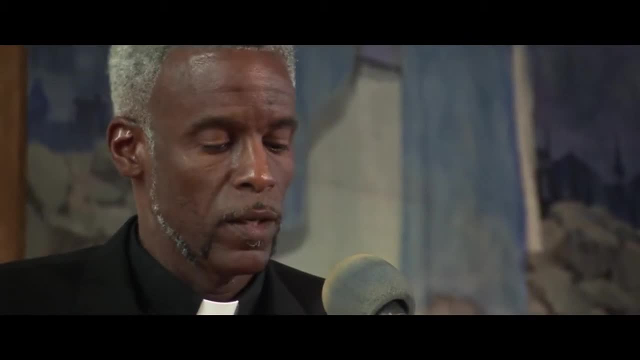 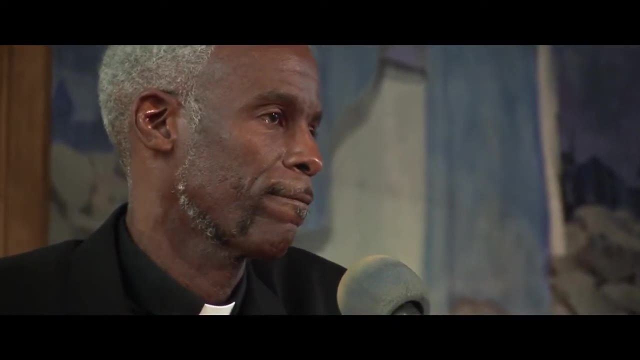 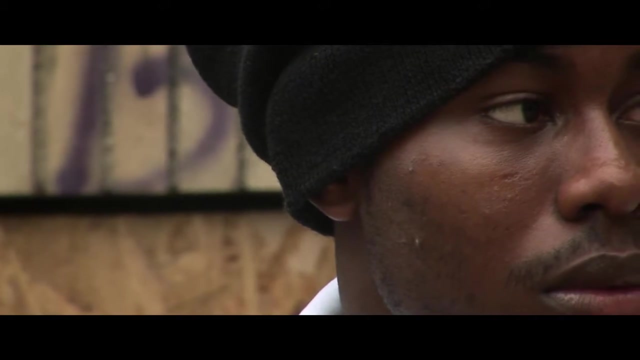 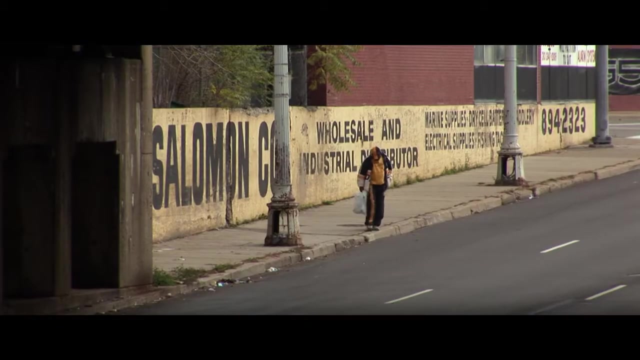 The pathway of the heart. According to the experts, there are many paths in life, but according to the Bible, the most purposeful one is the pathway of the heart. Fundamentally, the Bible deals with how people must live together In the story of Joseph, who had 12 brothers. 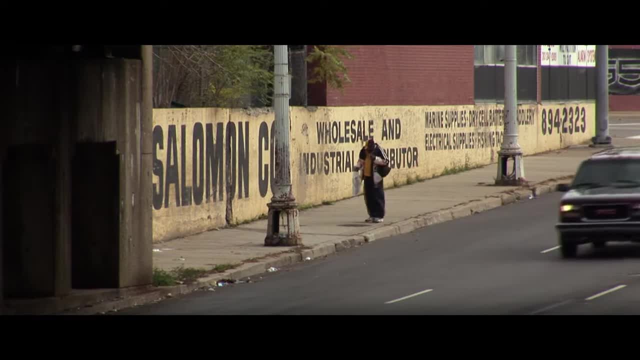 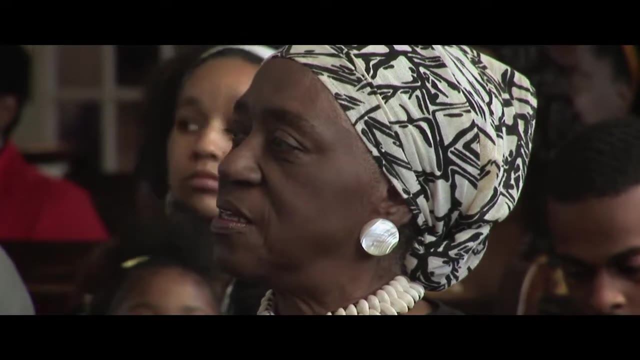 he was a foolish dreamer. He really believed in his dreams, and so he shared his dreams with his brothers, and his brothers became jealous and they sold him into slavery. But that story is about how people must live together. Living communally is the pathway of the heart. 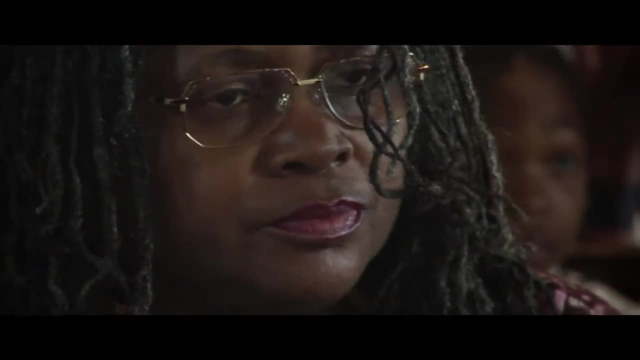 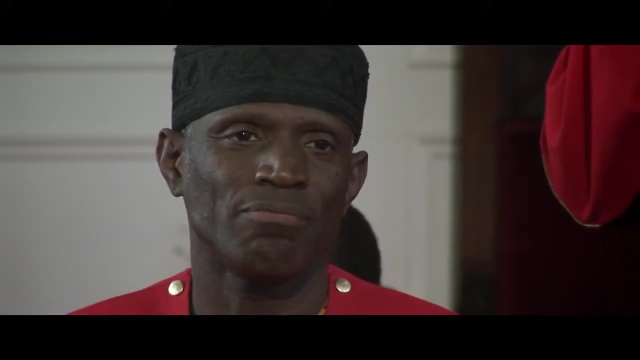 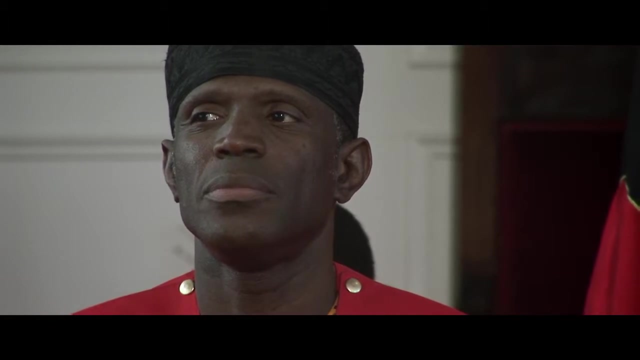 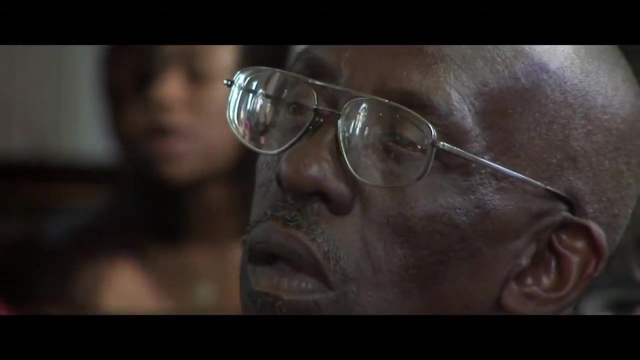 The basis of communalism is acceptance and understanding. Acceptance and understanding doesn't mean that you necessarily approve of someone else's behavior. Acceptance and understanding doesn't mean that you just means that you are willing to hold the space for somebody, For them to be who they are and where they are. 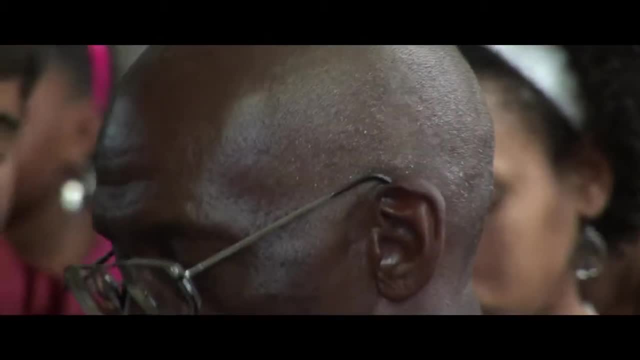 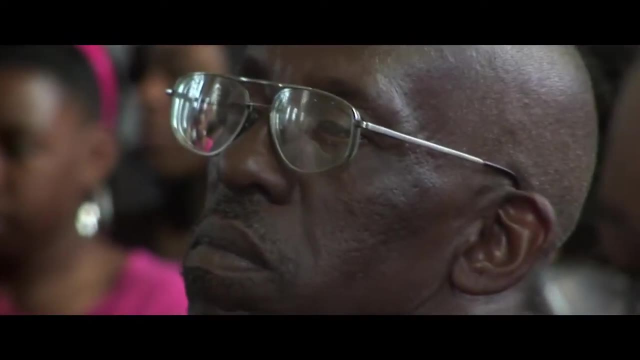 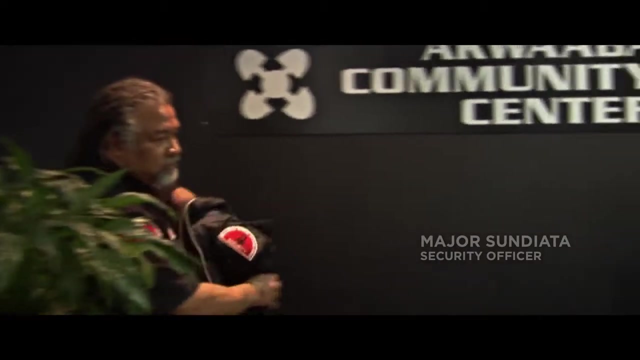 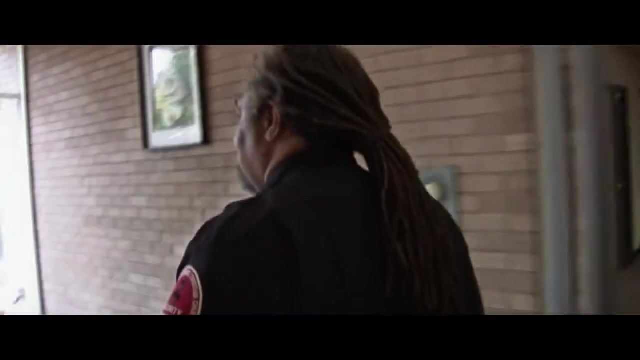 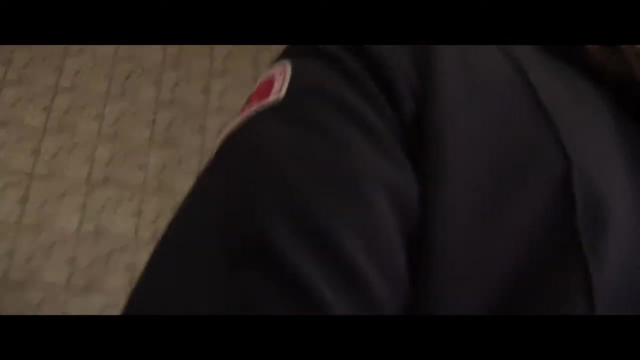 until they're able to grow and become what they ought to be, You're going to hold the space for them. That's what acceptance means. Yes, all right, Okay, Okay, Is this an official gathering? No, this is just an orientation gathering. 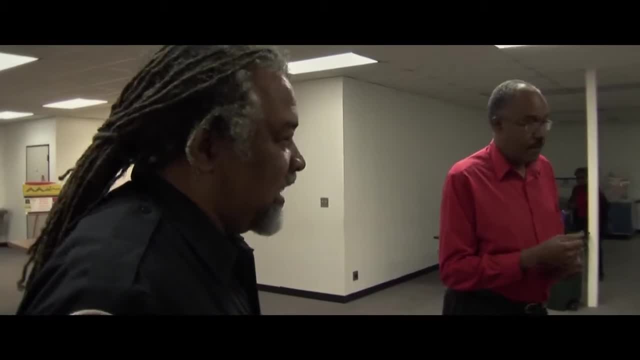 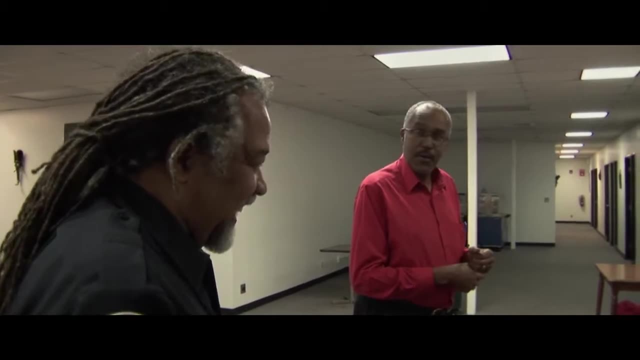 You know you haven't had enough brothers singing solos, They put me on the choir. Thank you First, Captain. I was told that. Put my daddy out there. You were told that. Yeah, I was told that. I was told that. 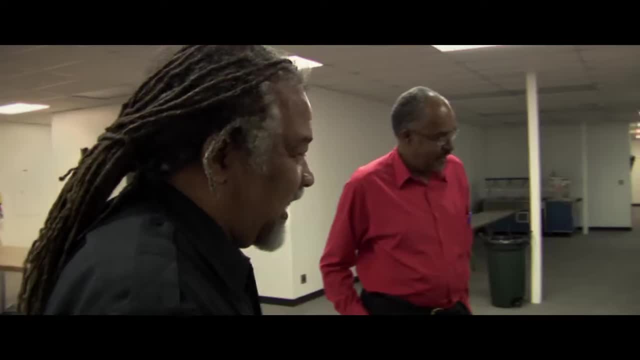 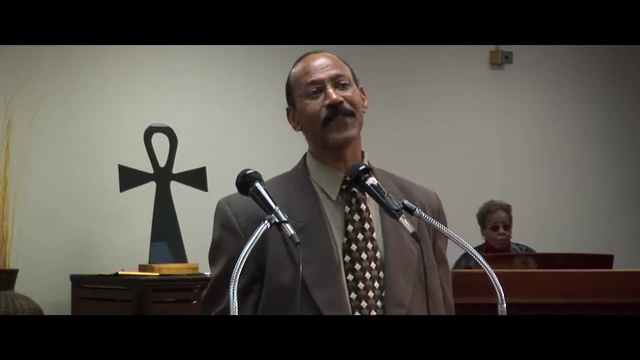 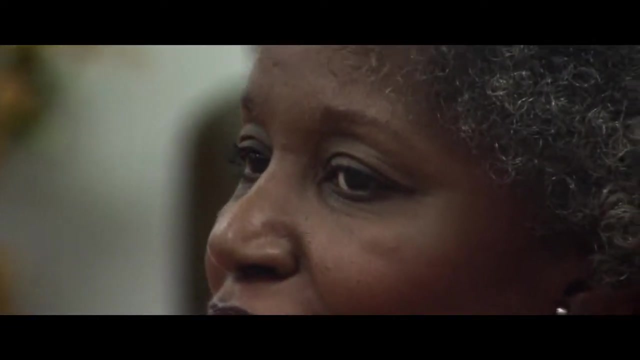 I got something from my heart. You got me too. brother, Come on, Give me that old time religion. Give me that old time religion. Give me that old time religion. It's good enough for me. now I say: I'm so glad that Jesus listened to me. 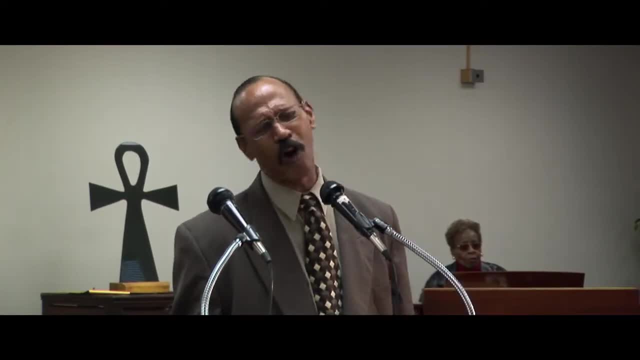 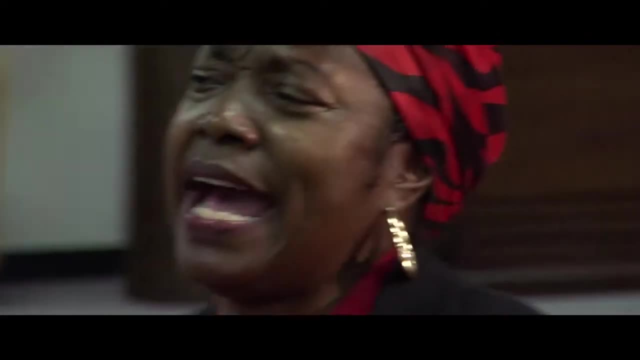 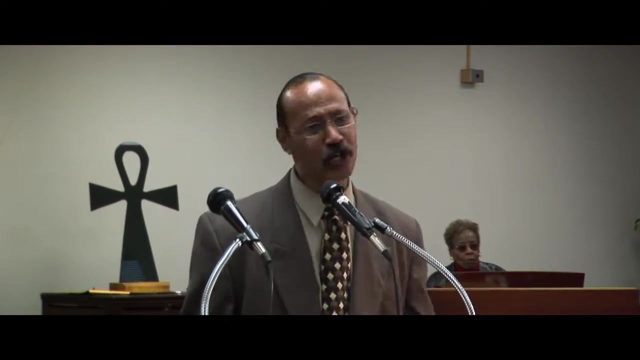 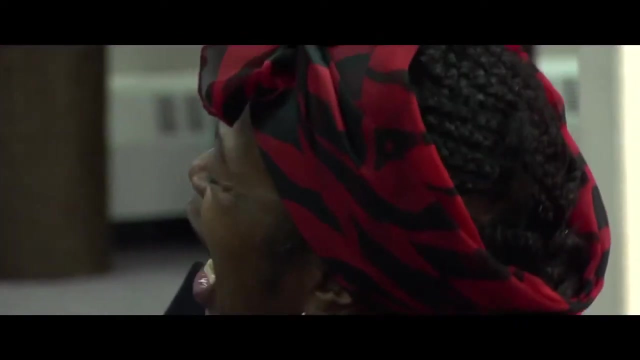 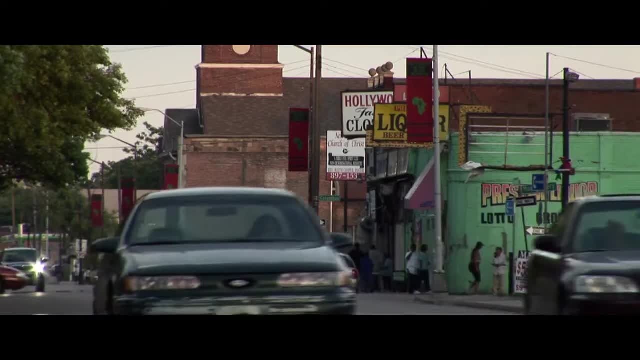 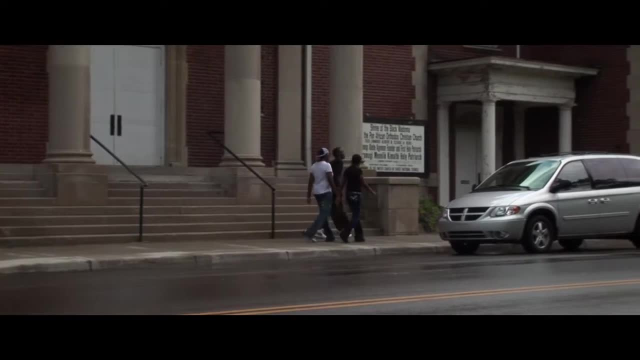 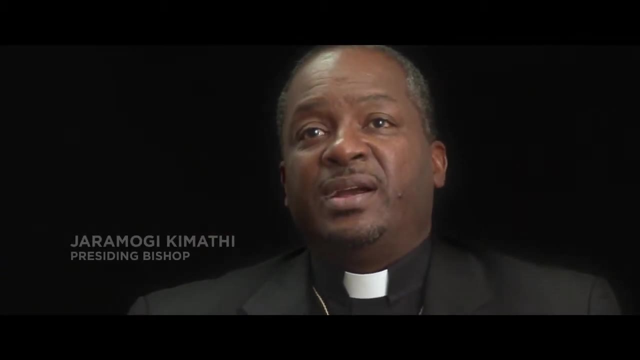 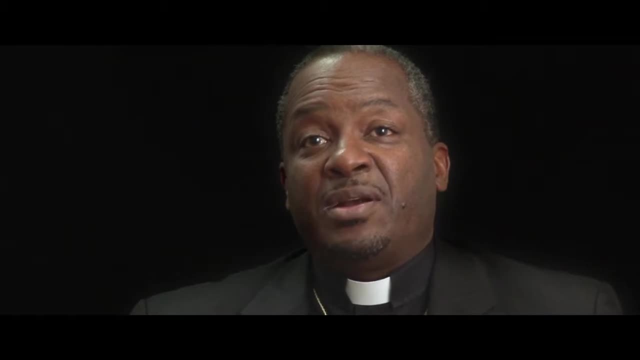 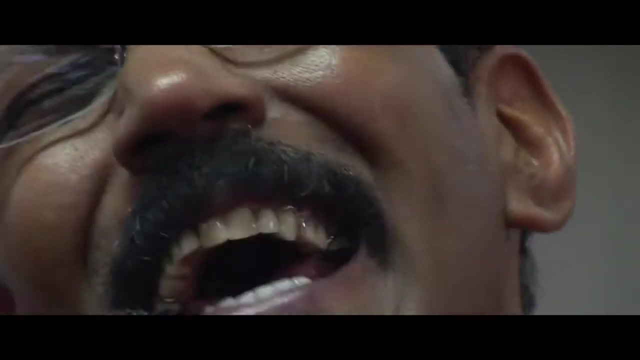 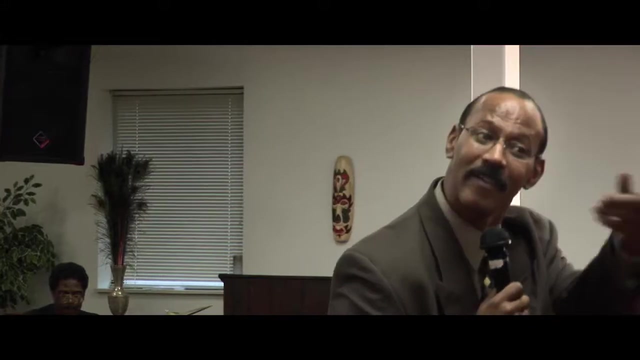 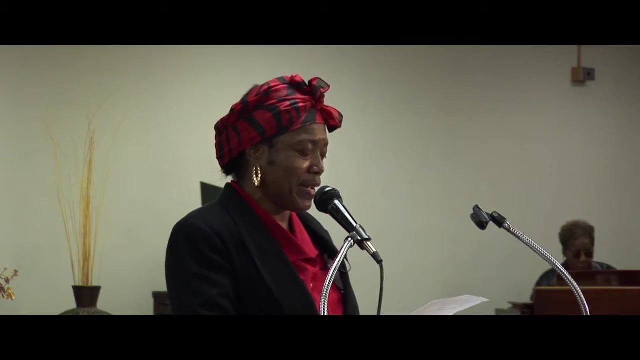 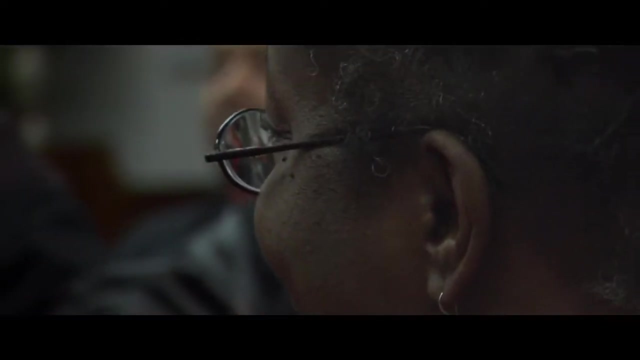 Was about liberation. It's about building a nation. It's about a Oppressed people trying to get free Or trying to stay free, Amen. Let's go on to the story of Ananias and Sapphira. so somebody tell us the story in a nutshell. 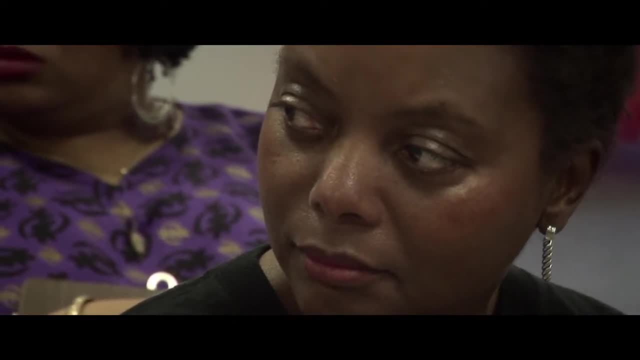 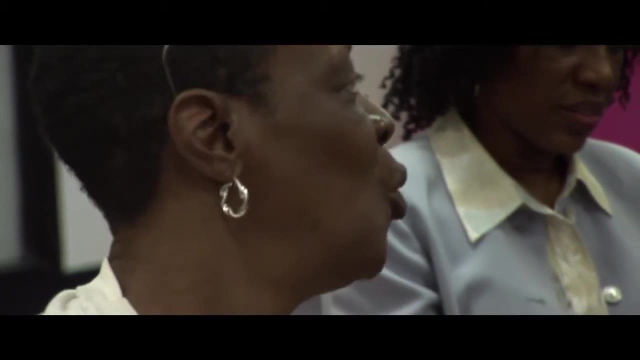 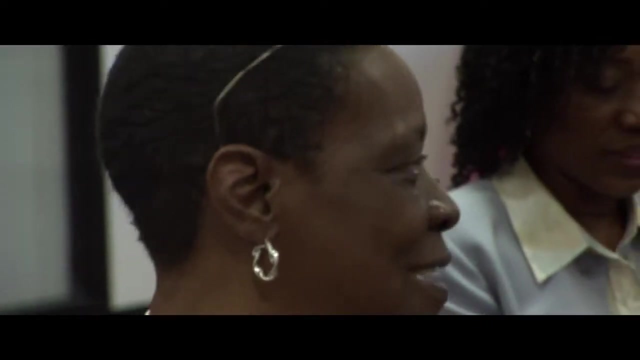 They sold their property And they didn't turn in All the proceeds. Okay, they turned in most of them and held back a little bit. So so when? So first they came to Anna Ananias and gave him the opportunity to be honest and tell the truth, and he didn't, and he 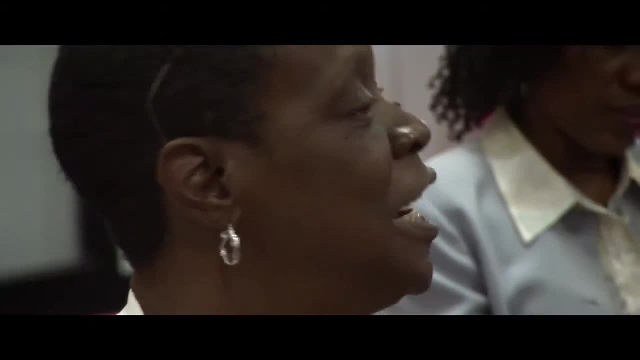 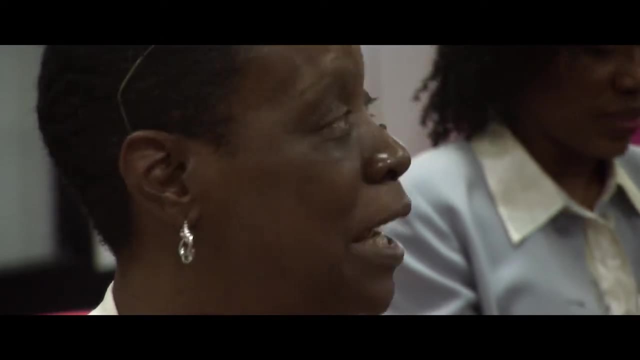 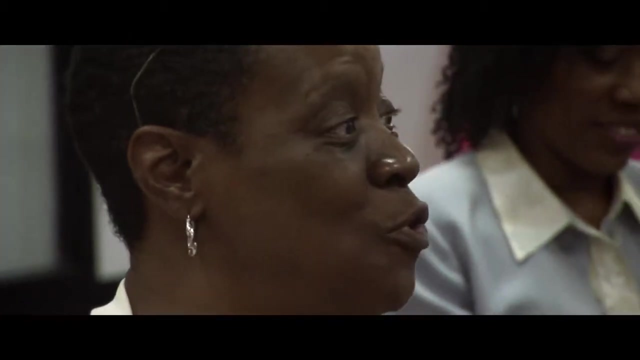 Dropped it. and then they came to his wife and she had the opportunity to tell the truth And she lied to, She dropped it, And that's the moral of the story. Then they told him the story. You lied to God. They said you, you know, you didn't lie to ma'am. 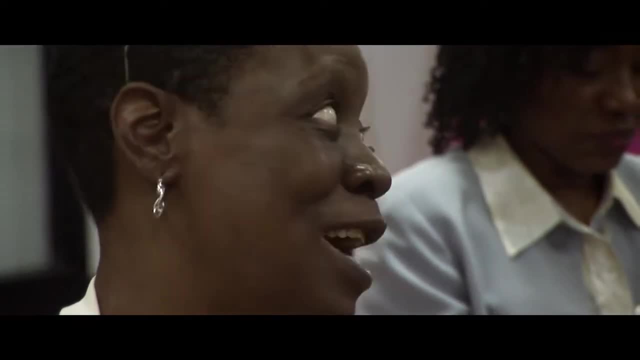 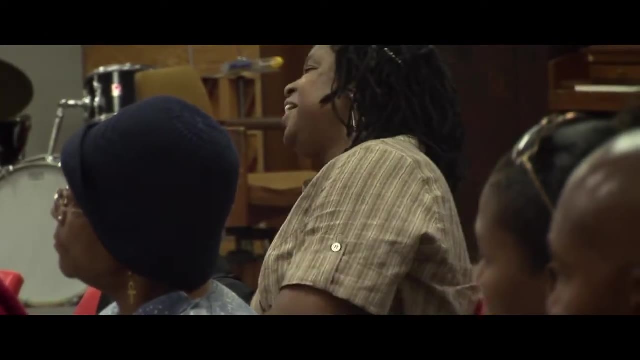 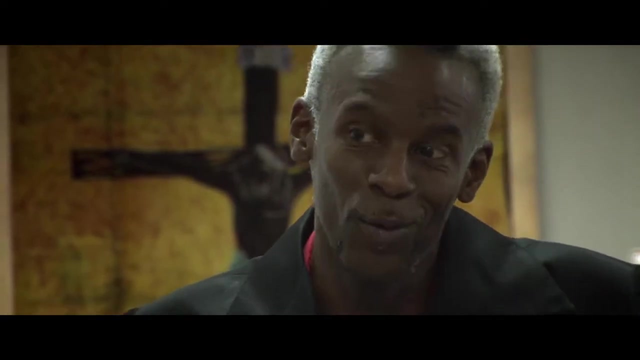 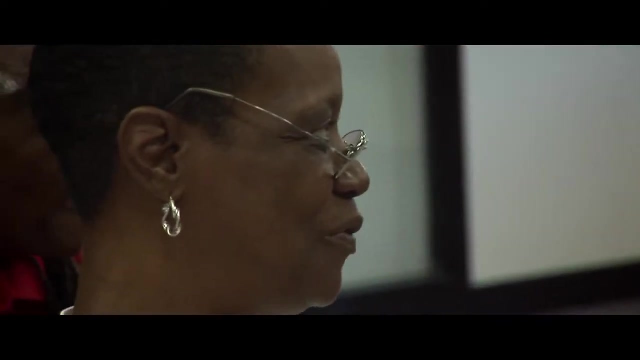 You lied to God, and when you lied to God, you got some terrible consequences. Now I know why we have issue with that story: because you think about all the times when you Didn't tell the whole truth, And Ananias Goliath's deception is all of our deception. 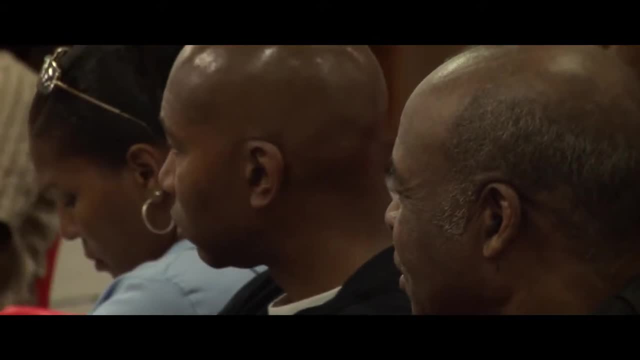 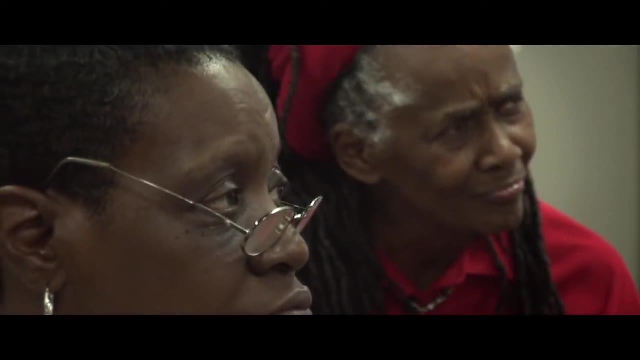 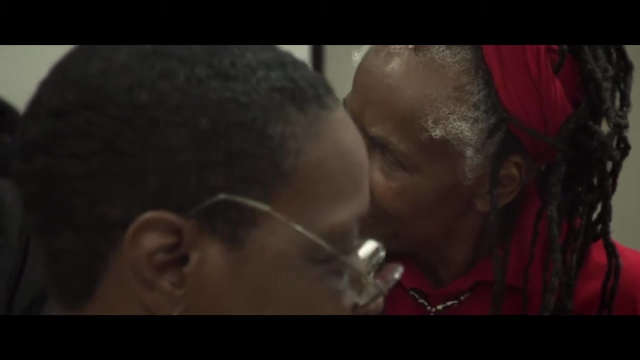 How many of you know that it is easier to lie to yourself than it is to lie to somebody else? It's much easier to lie to yourself than it is to lie to somebody else. That's the kind of deceit that resides on the subconscious level. 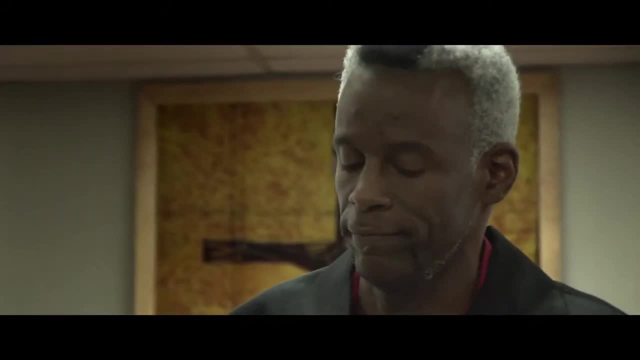 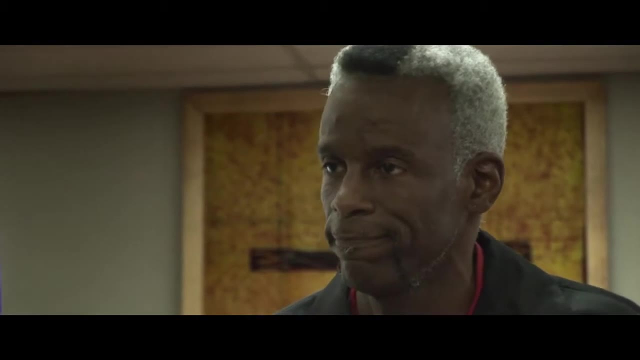 You repress it, you deny it, you pretend like it's not really there. That's a person who has lied so long that they believe themselves. When I was in the seminary- a lot of the young aspiring preachers there- they would pull me to the side and say: 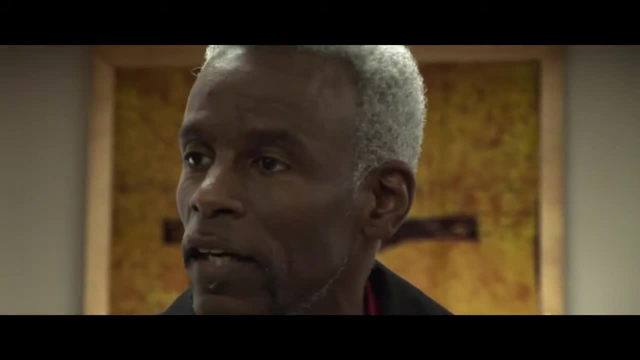 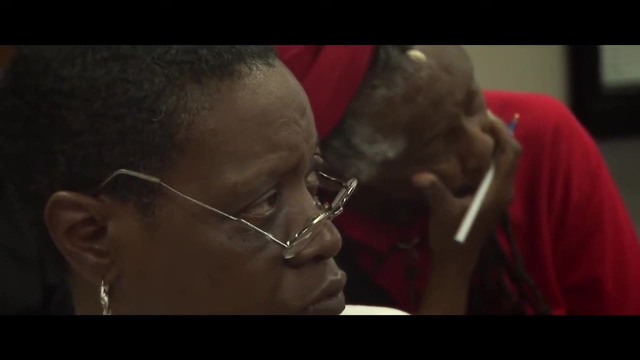 you know I want to learn a little bit more about the shrine and about Reverend Clay. you know They wouldn't say it in class, But what happened was when they went back to their church and tried to introduce black Christian nationalism. 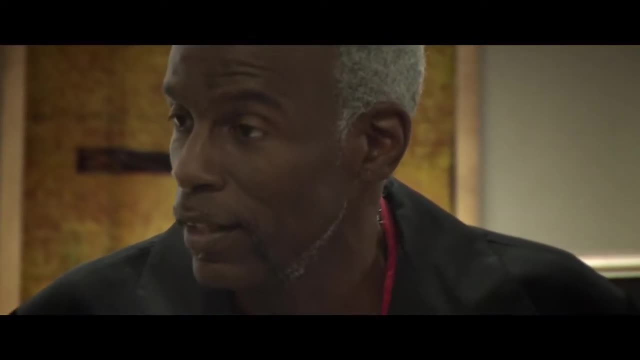 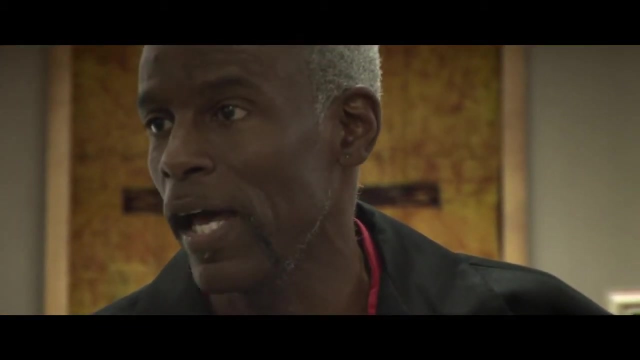 people said: you know, people did not want to hear it And they didn't understand. I said: well, when you've been lying to people for 450 years, they don't want to hear nothing but the same old lie. And when you come in talking about Jesus was black, 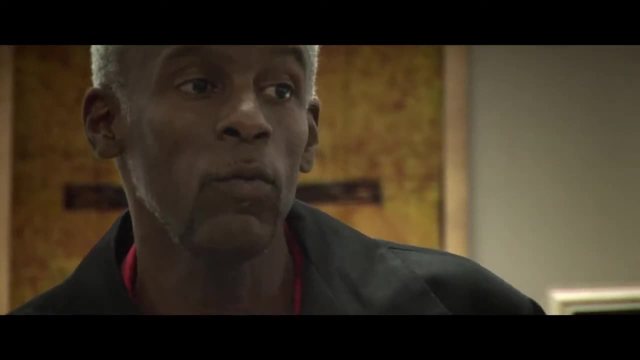 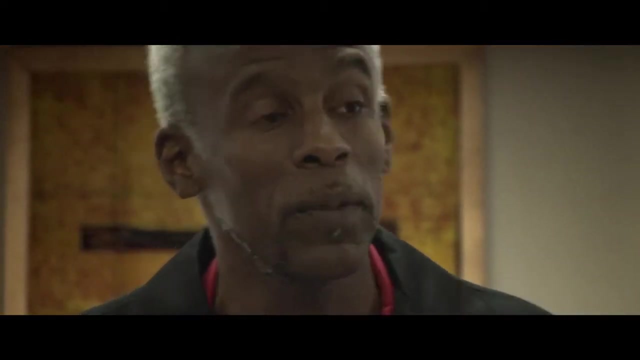 they're going to run you out, And that was you know. basically, they were just talking about the historical blackness of Jesus. They wanted to be able to say that in their pulpit but they couldn't Because on the wall they had a picture of a blonde-haired, blue-eyed European. 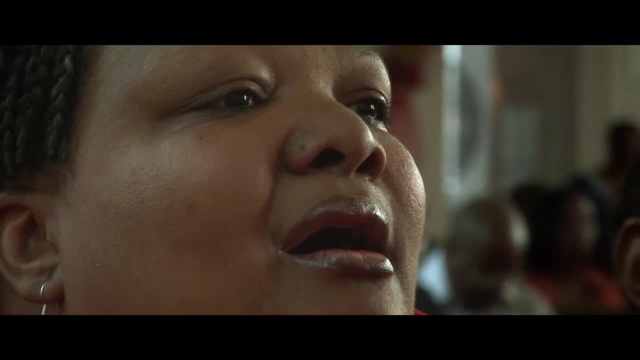 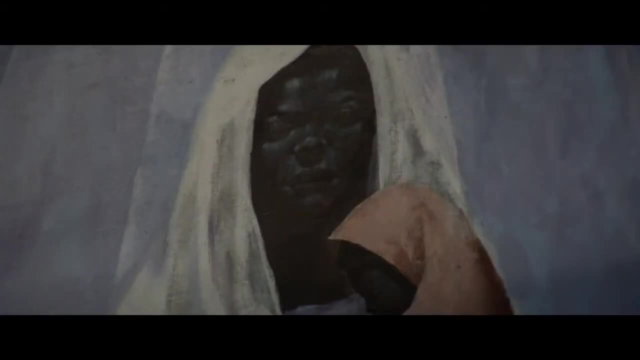 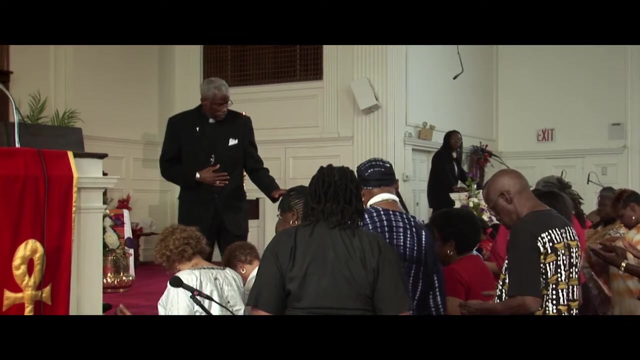 Right, I don't feel no way to die. There was no black iconography in America that presented the people in the Bible as people of African descent. Certainly nothing that dealt with Jesus that way. As a matter of fact, this was the most controversial aspect. 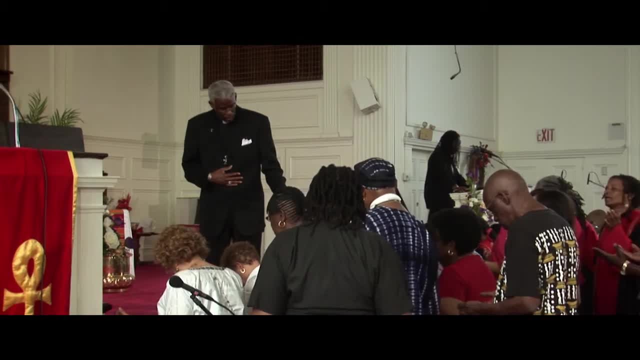 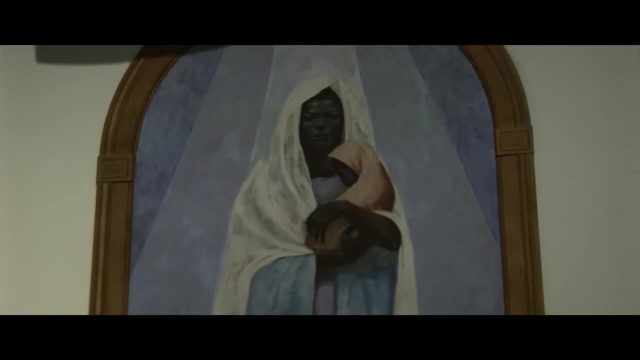 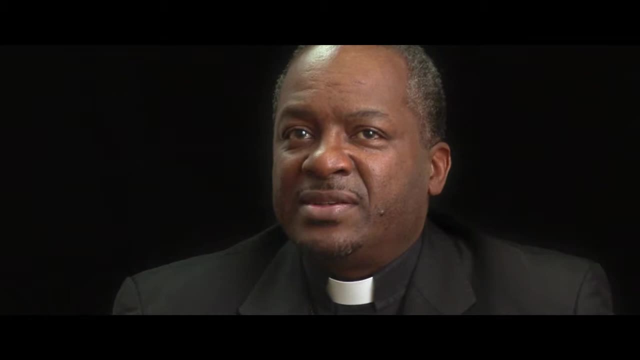 of our organization in the beginning, the fact that we could be so audacious as to think that Jesus might be black. It doesn't seem so profound today, but it was profound in 1967 when the Madonna was unveiled. It was a really big thing. 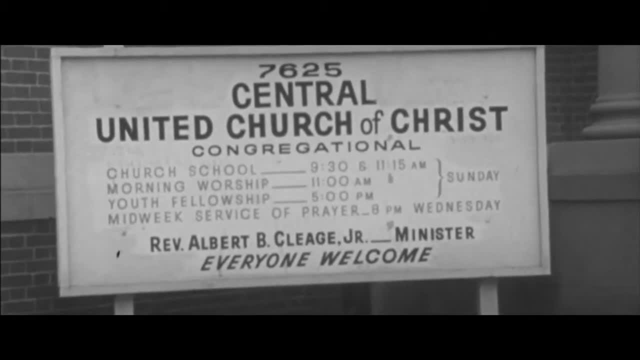 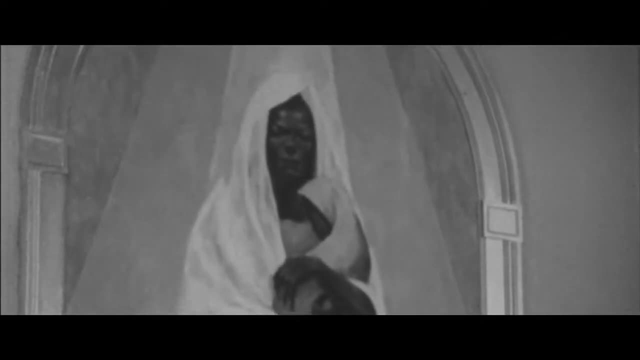 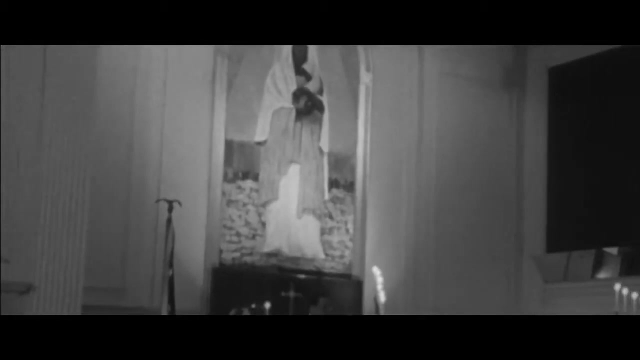 1967, we're Central United Church of Christ. We unveil it. The women of the Black Madonna, Jesus, he was a part of the black nation And he taught people to be a part of that black nation. We immediately caused such a controversy internationally. 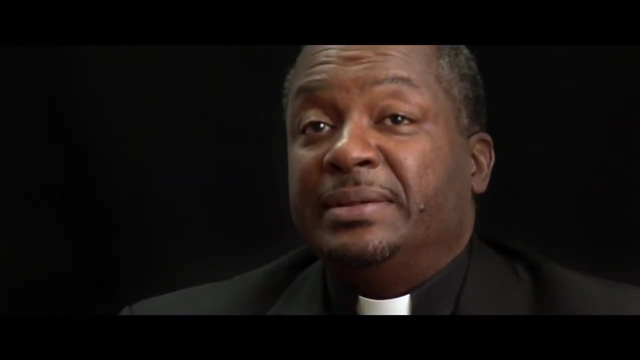 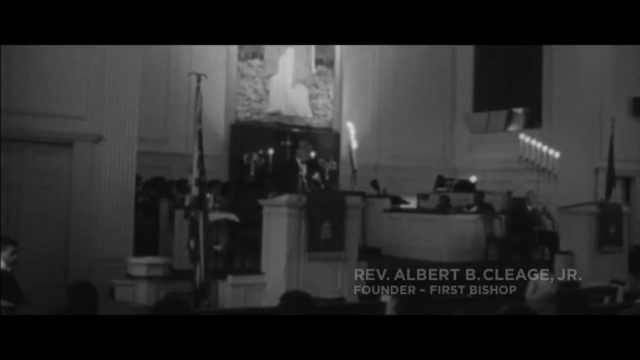 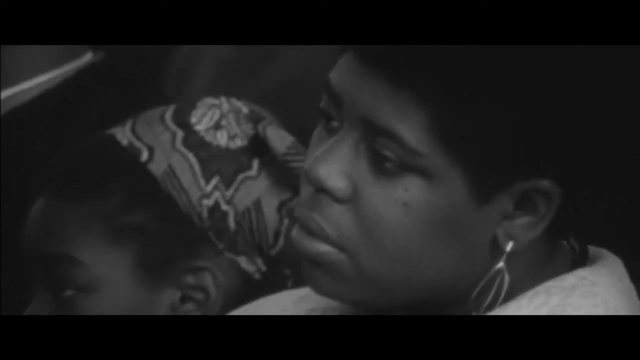 with a black depiction of Jesus and Mary. Immediately, the name is changed that same Sunday of the church to the Shrine of the Black Madonna. He never said: be free up there someplace. Jesus was concerned about freedom, about the unity of a black people. 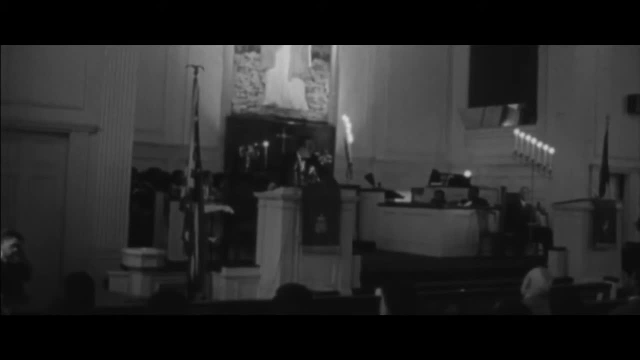 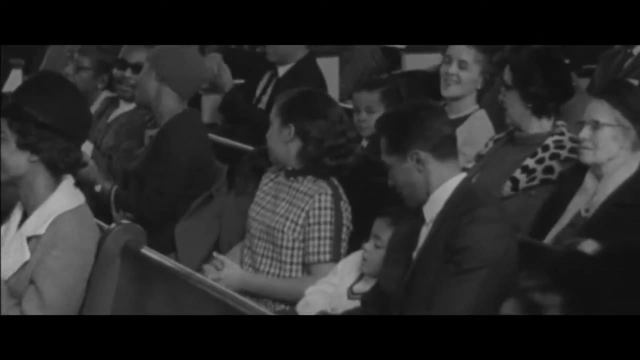 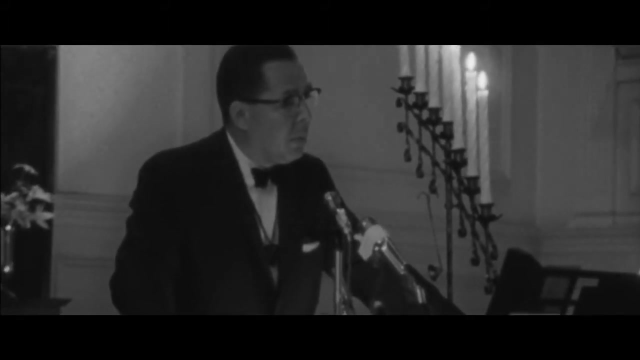 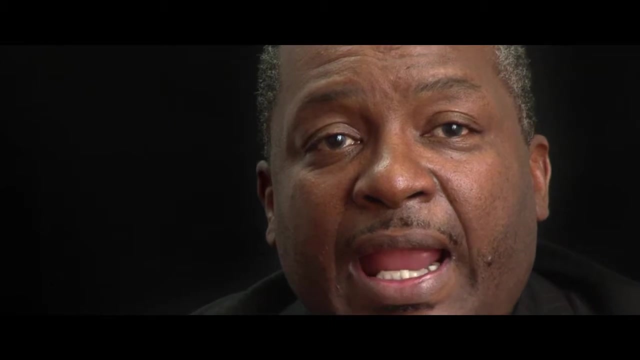 fighting against the oppression of a white, gentile nation role. Unlike most people in the church, our founder was not. he did not come from a working class background. He was a black person of significant privilege. He was a very sophisticated and cosmopolitan man. I think that that has helped our organization in the sense that 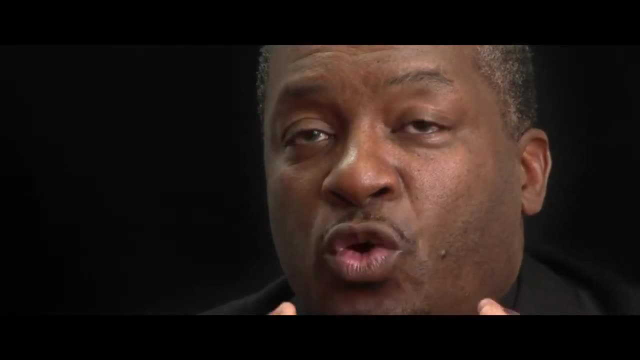 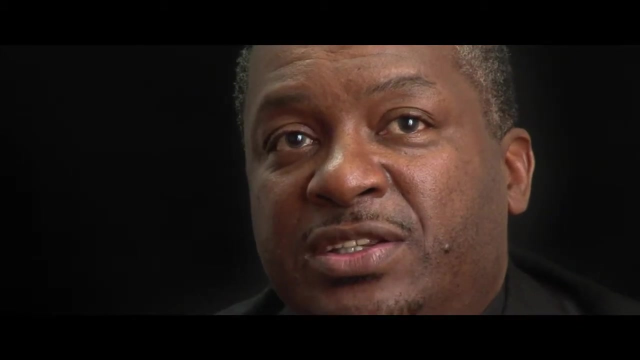 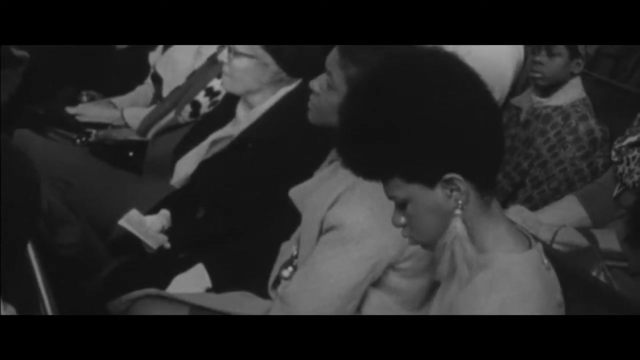 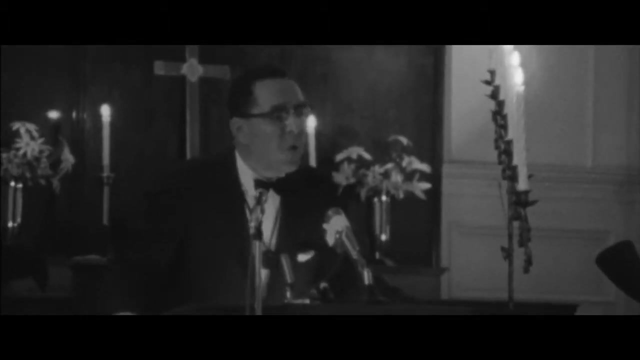 it has. he has taken basically working class people and stretched them, broadened them so that they could think of things and behave in ways in which I don't think would have been possible without his influence. And yet look at us, powerless, everywhere we are in these United States, Oppressed, browbeaten. 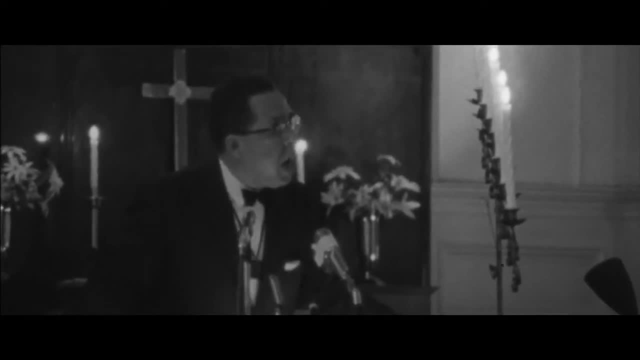 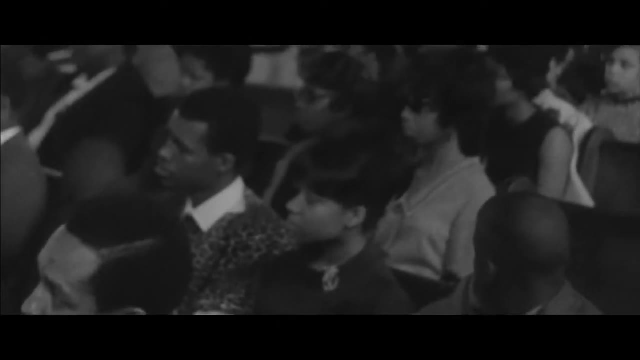 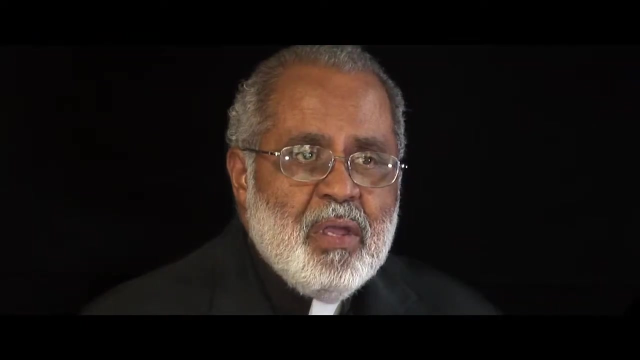 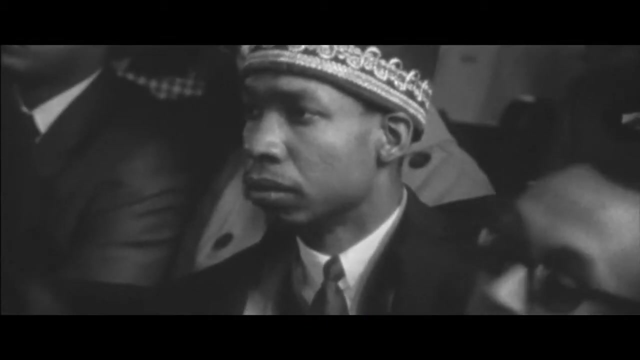 beaten by the police anytime they feel like it. unemployed, kicked out of jobs for no reason. Most black people of that time were feeling the sharp edge of racism and discrimination in this country. I was real angry, you know, wanted to take hold of things, You know I was ready to line up and get the arms. 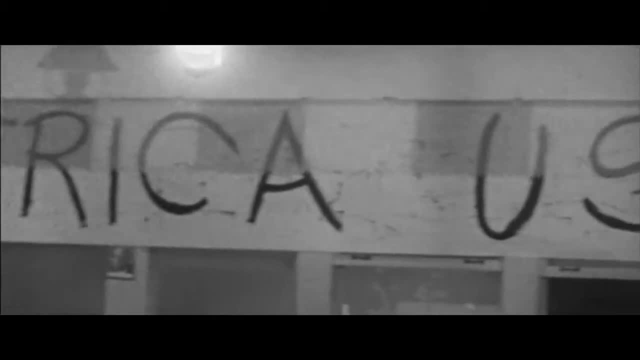 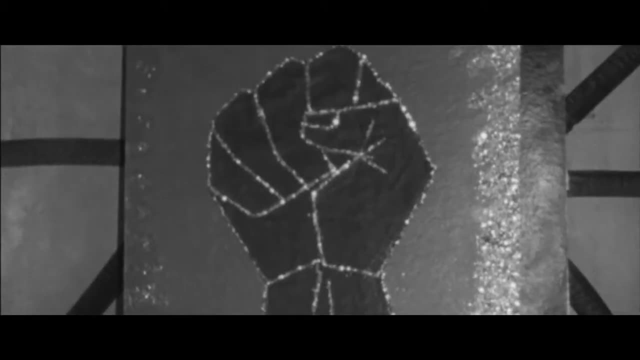 the guns right then. I mean, that's where I was coming from And this seemed like a place I might be able to get it. We aren't playing games. We're building a nation. we're trying to get free and we're fighting to do it. 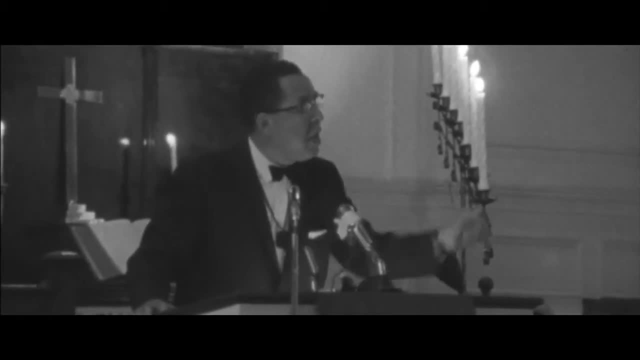 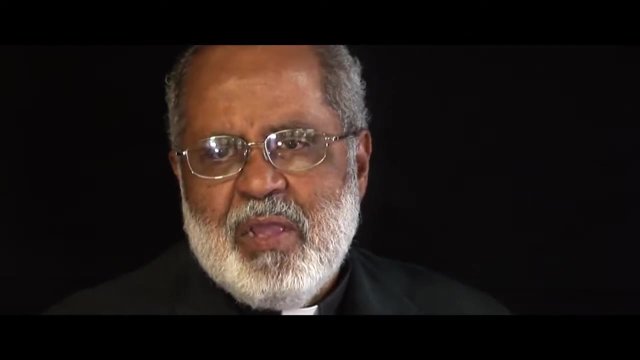 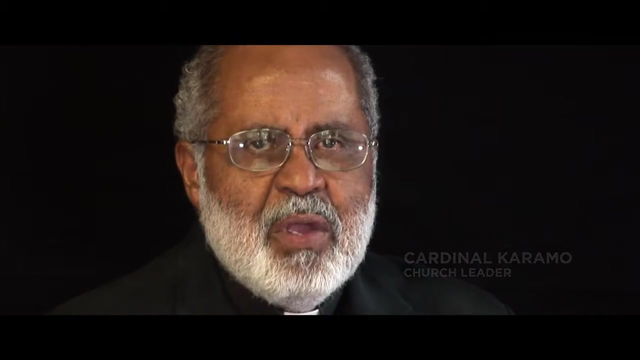 Jaramuji Abebe came to explain to me. you know about the need for organization to be organized, to be focused, and you know, going back to even the time when we were closing these, boycotting these stores and and this kind of thing, jeromoji would tell us- and when we get a lot of times when we 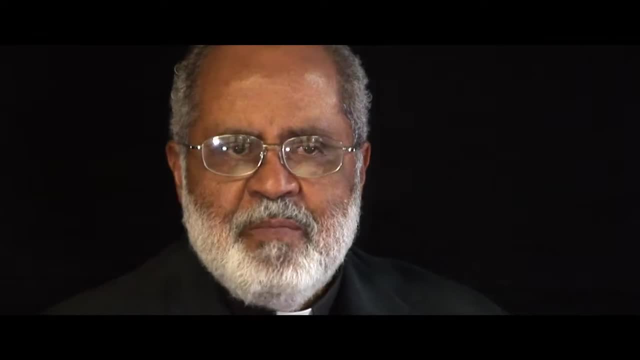 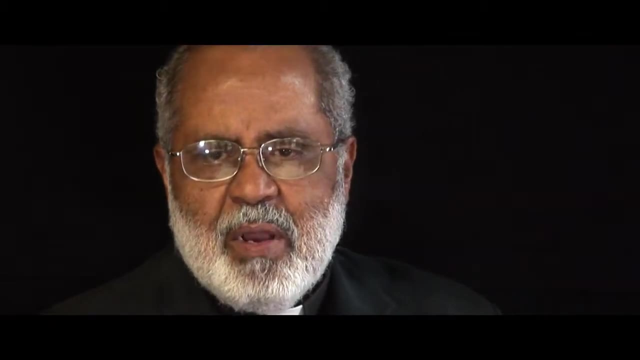 we get them to a place where they were willing to negotiate and he would send some of us off down to sit down and negotiate with him. he would say, now don't go down there being flamboyantly black. well, you can come back there and talk about all these people you put to the sword, but you 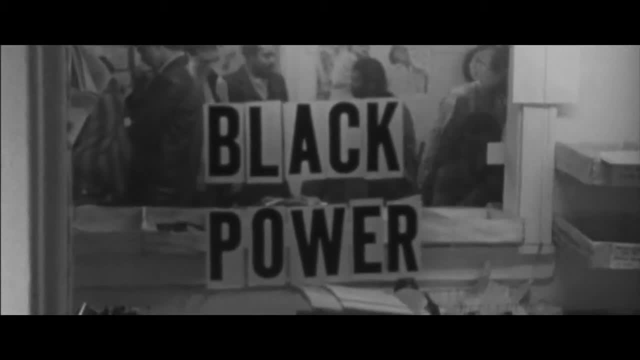 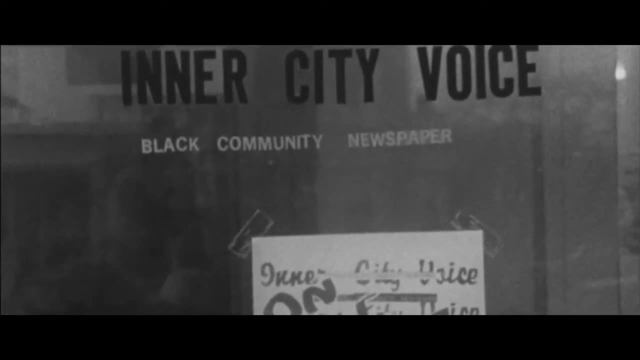 didn't bring anything back. you know you haven't negotiated one job, you haven't negotiated one service that needs to come into the black community, but you feel good because you jumped on a bunch of people and and gave them a good whipping. when you grow up, you're going. 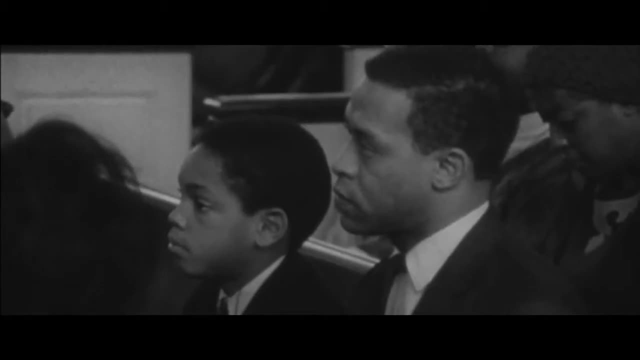 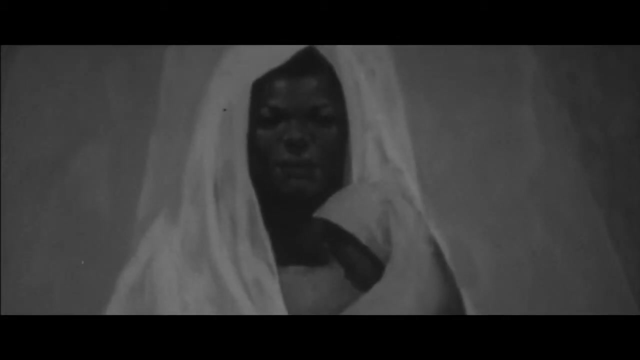 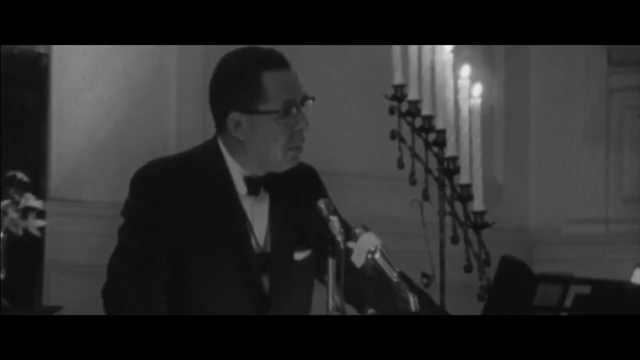 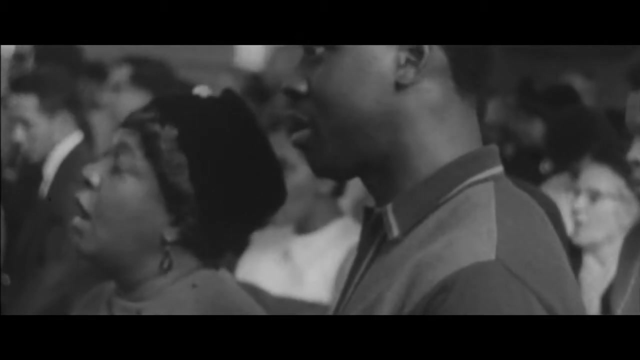 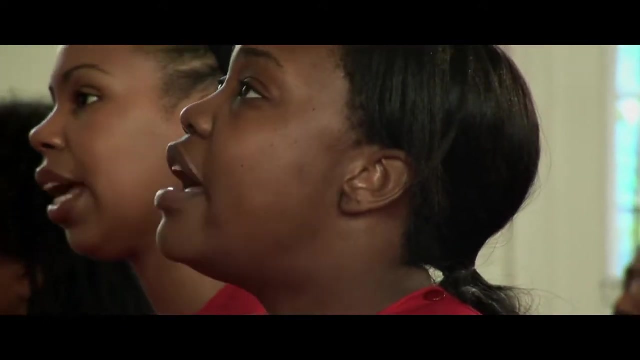 to have obligations, because we're not going to be free by that time. there's still going to be something for you to do in the name of jesus, our revolutionary black example. glory be to the father. we are his chosen few. may we strive for freedom till our paths. 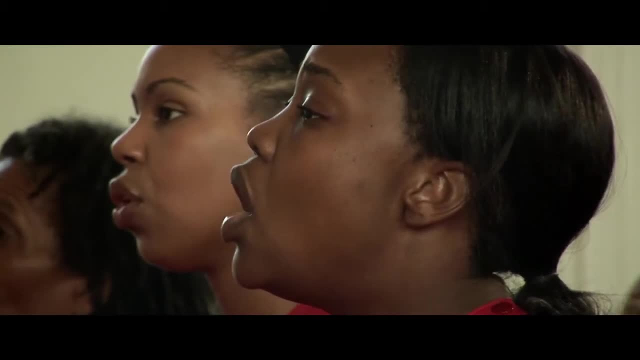 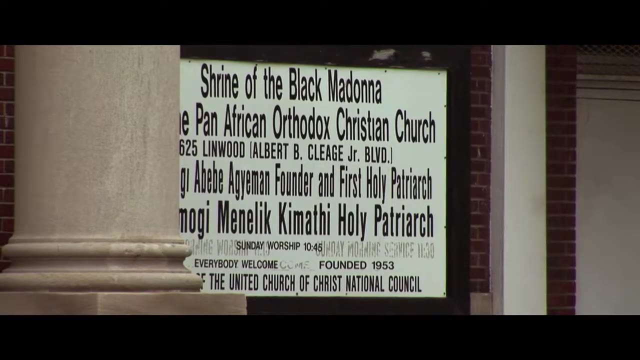 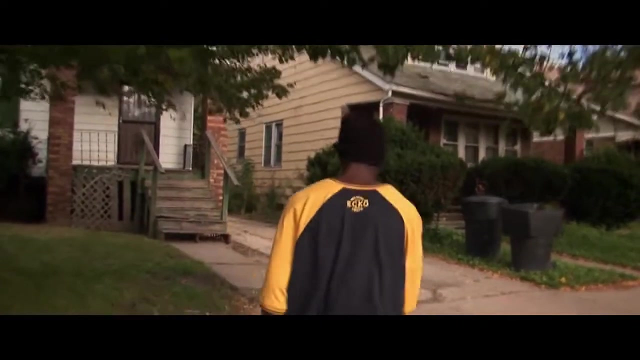 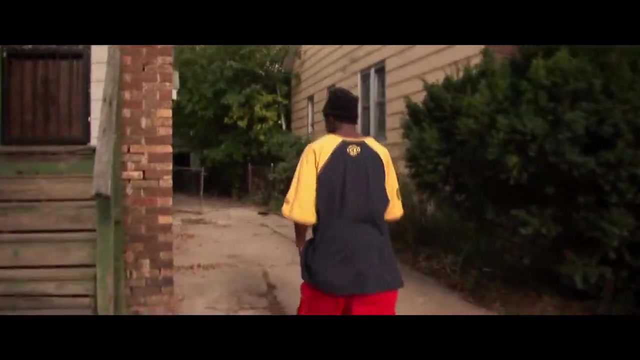 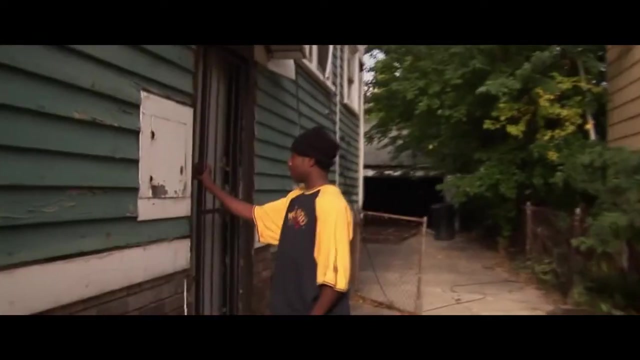 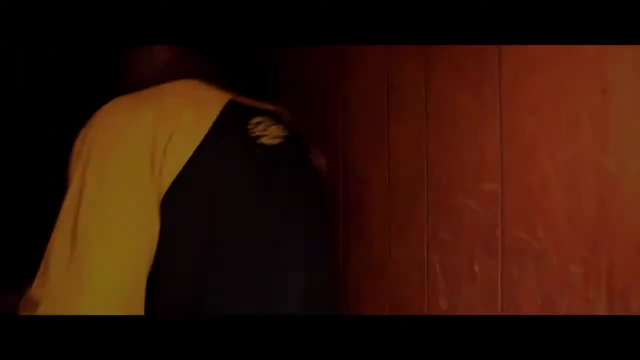 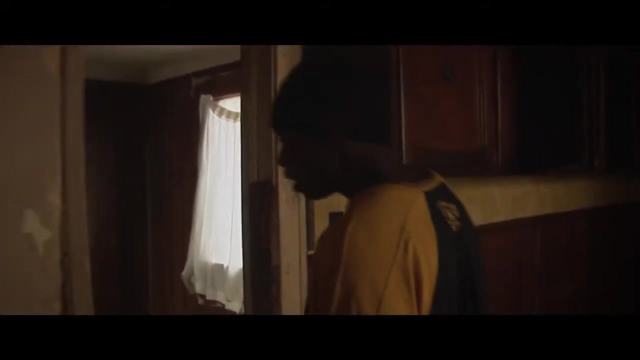 get through manifest and God, glory and love of you. I used to stay here about three, four years ago with a couple of my cousins and they'd make us move around and go wherever they were gonna go. and, you know, once we've made a place for us to meet, 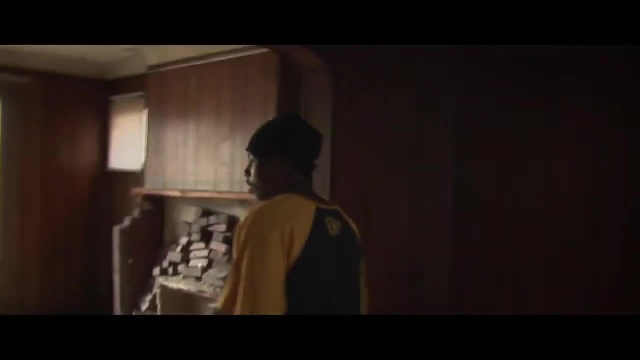 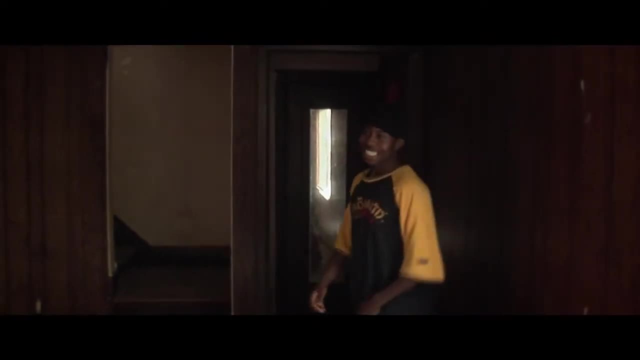 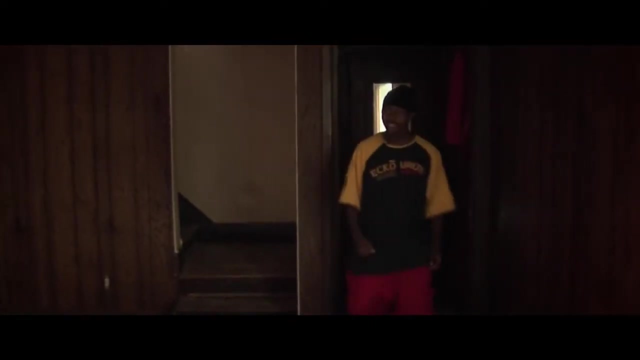 and to sort of make a place for ourselves and to talk about this. we feel so comfortable in a room that is independent and peaceful. I'll tell you one thing that I want to say to you, who I think he's not going to be with, but he's going to be with us. 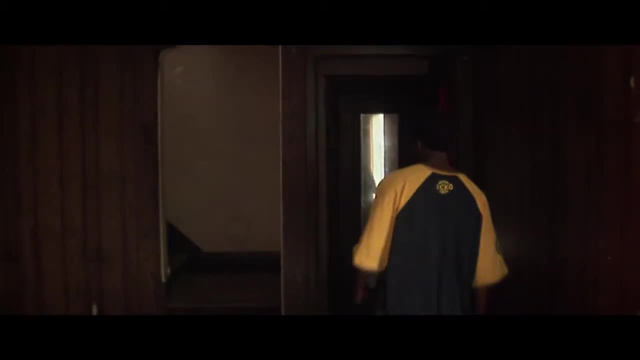 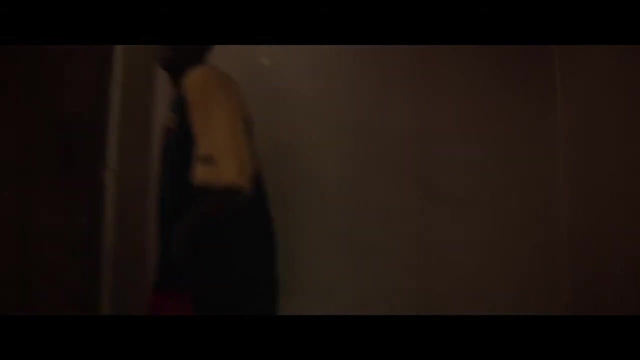 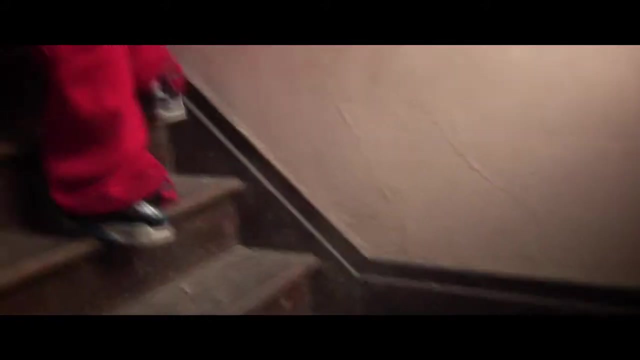 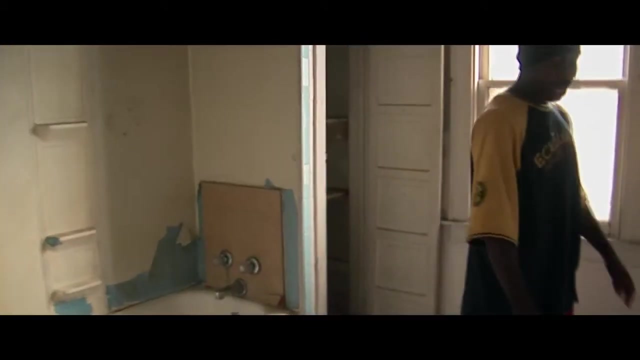 and this thing. you know we're going to have to treat him like a human being, man. So sometimes I used to sleep upstairs and everything It's the bathroom man We ain't had no toilet. man. We ain't had no running water man We used. 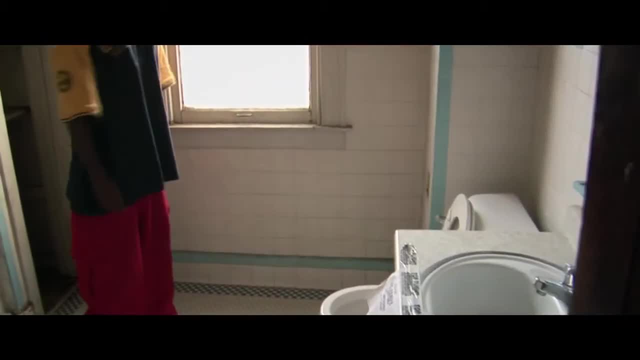 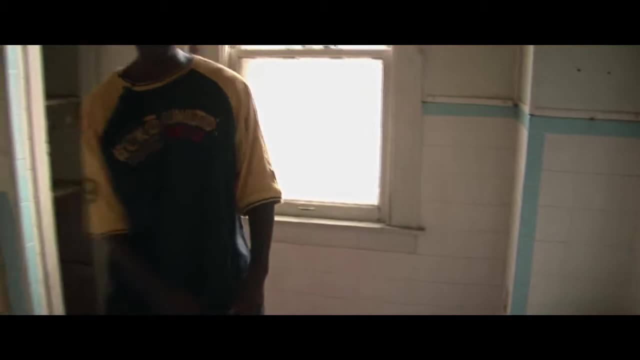 to take bags. yo, You know what I'm saying. You might want to get that. yo, We used to take bags and we used to do what we had to do in the bags, and then we take the bags and just go dump it. 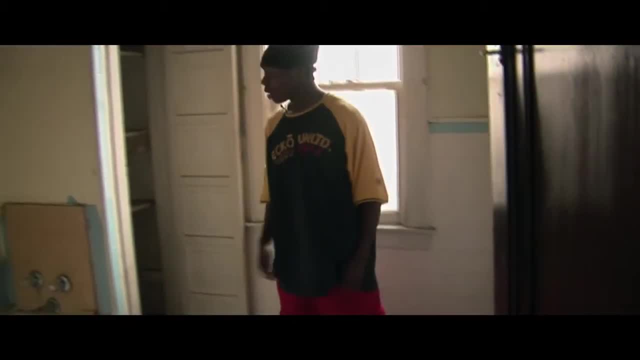 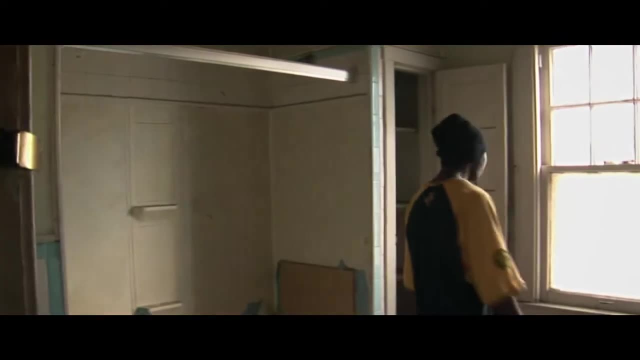 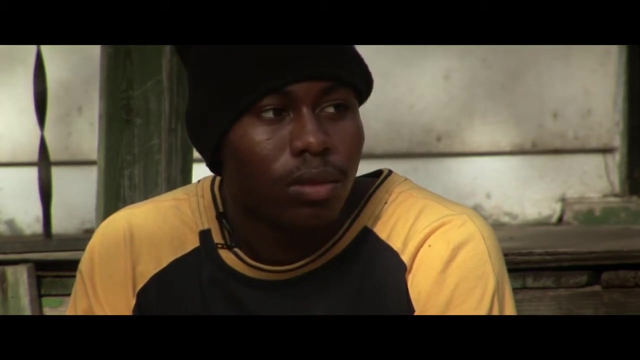 man. Simple as that. yo You know what I'm saying. We ain't had no bathtub, no, nothing. man, Shoot man, And that's what it is. If there's a human problem, then you can have a ministry to it, And our ministry is to the. 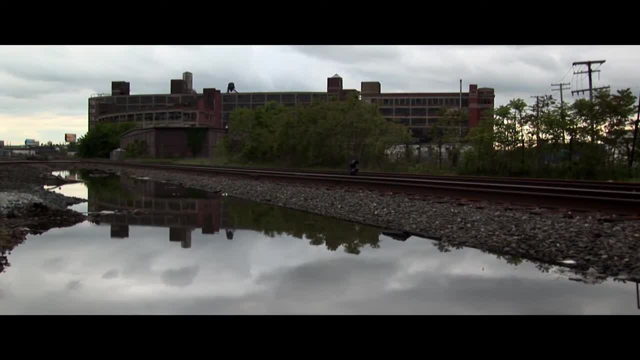 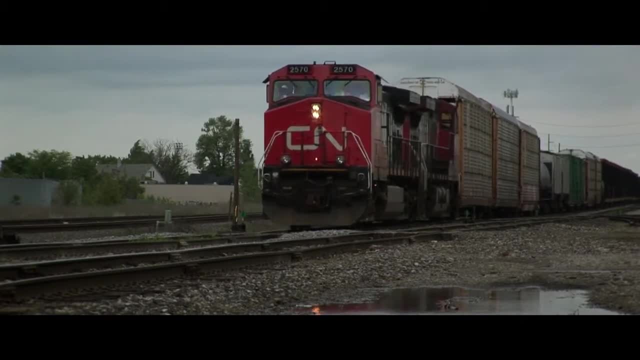 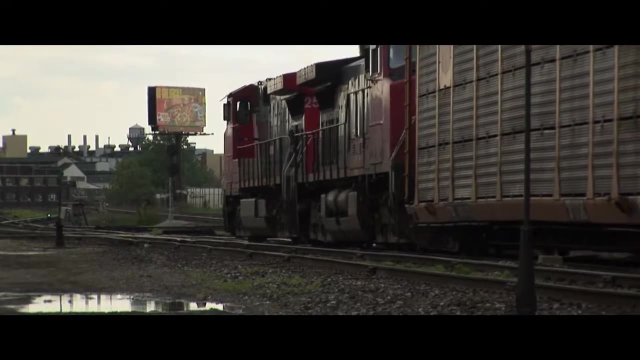 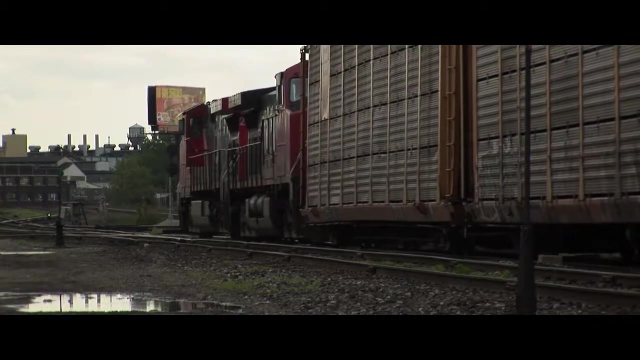 survivors, Survival victims of an African holocaust. A lot of people think they're doing their children favors by not telling them stories from the South. Then you're making them think that all this way that they live is just a natural order of things. 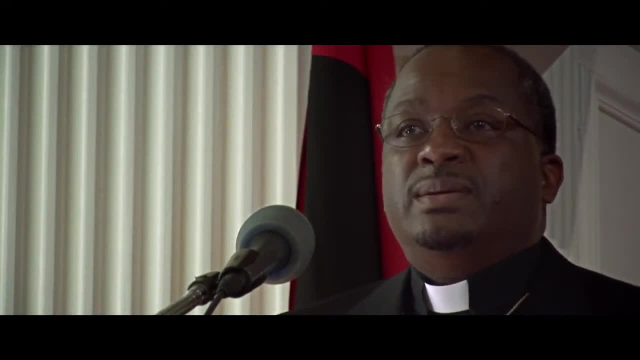 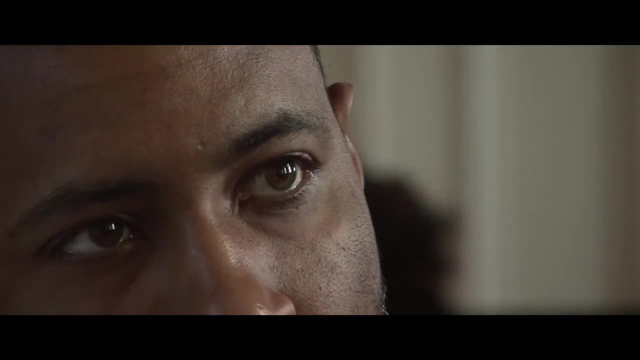 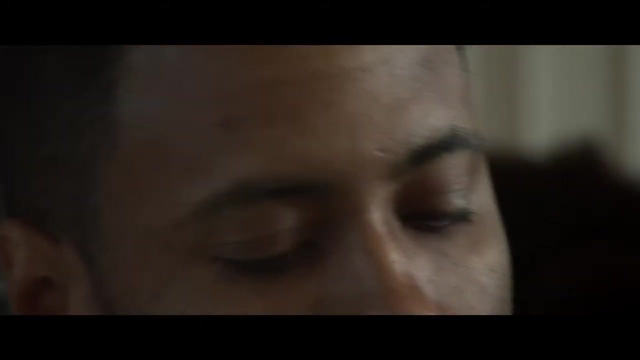 You're tearing them down from their dignity too. They need to know somebody did something to me. They need to know. Most people don't know that during slavery they wasn't trying to capture men, They killed men. They killed men because men had dignity and they were going to transfer their manhood. 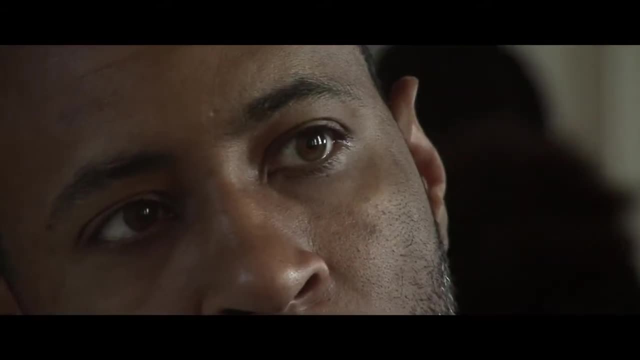 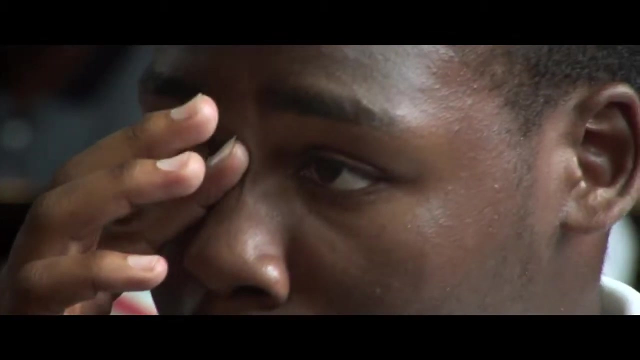 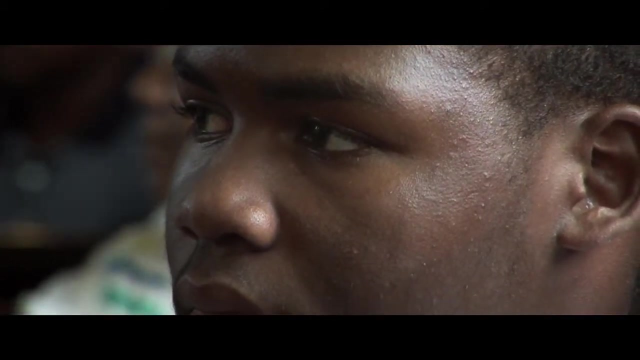 to the rest of the community. Next, thing, they knew everybody was going to be fighting, And removal of the men gave them the right to fight. They gave them time to turn the boys and the adolescents into domesticated animals that would work their whole life in order to make their oppressor rich and powerful. 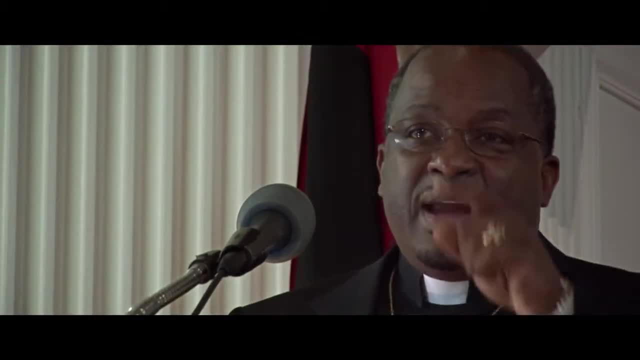 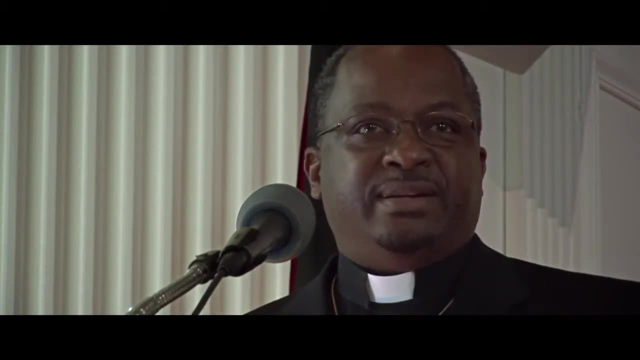 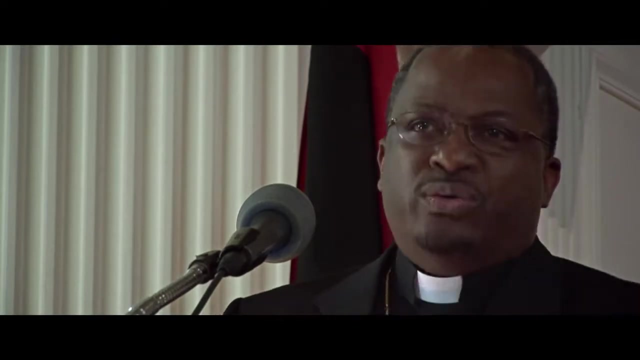 It wasn't enough to declare the whole group to be inferior. I have to make you feel inferior. I have to do things against you that rob you of your dignity. and it's not enough that I can enslave the group or declare the group inferior. I've got to make you individual. 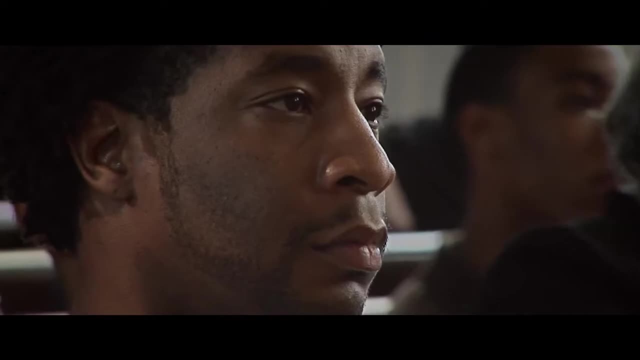 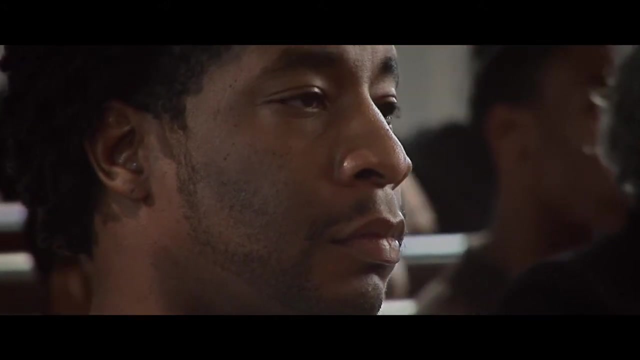 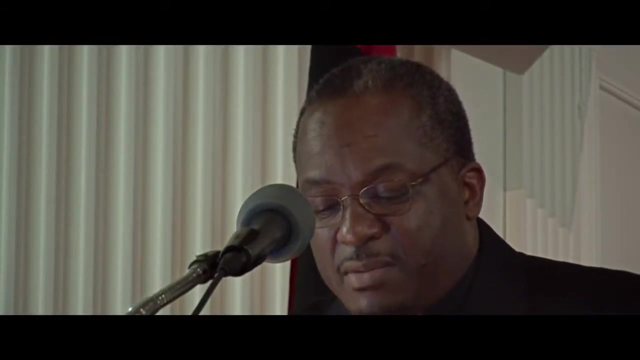 I've got to make you feel inferior By being cold in a house where the wind is coming through, where you can see the stars through the roof and the dirt on the floor. I want you to think about it just for a moment. I want you to consider something. How do you? 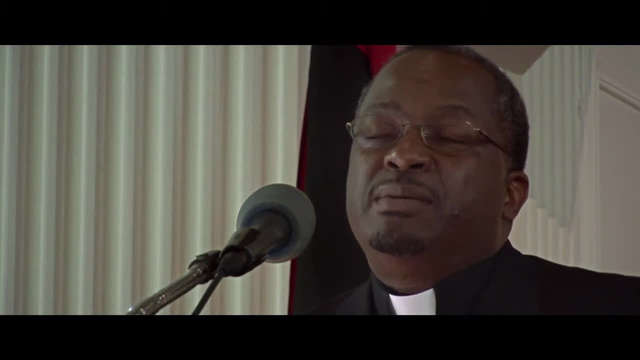 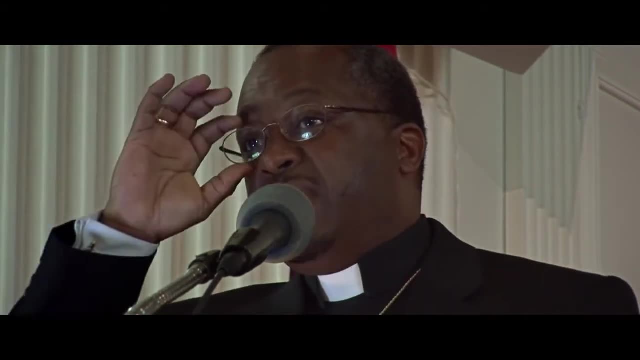 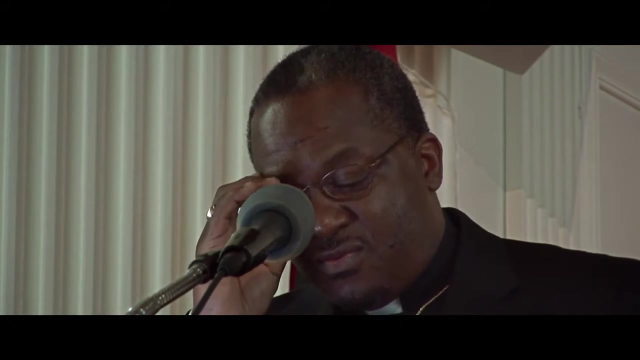 think all of this made the black man feel Really. Come on, I'm not talking about what you understand from your reading history books. I'm not talking about the facts of the matter. I'm talking about how do you think it made him feel. 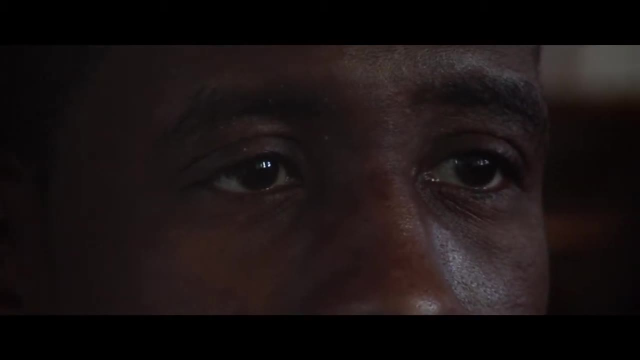 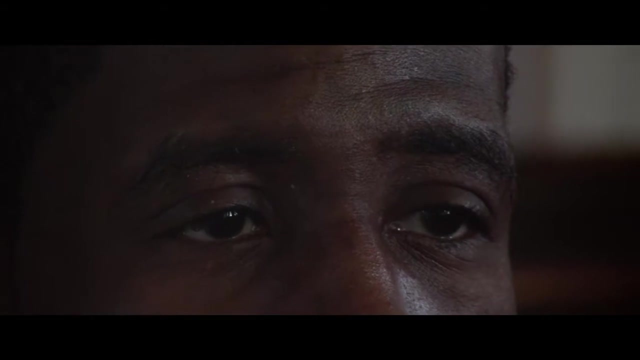 How did it feel to have no control over your world? Come on, How did it feel to being able to protect your wife and children? How did it feel? How did it feel to have your wife impregnated by the same man who's robbed you of everything? 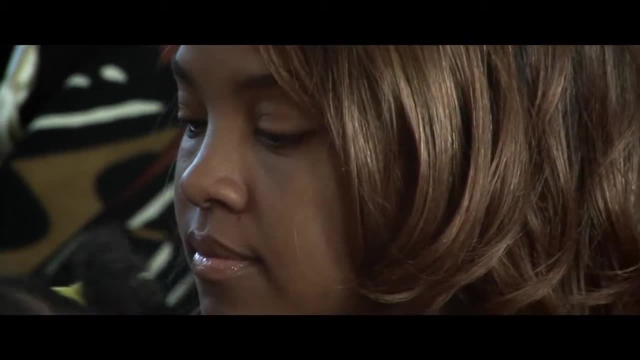 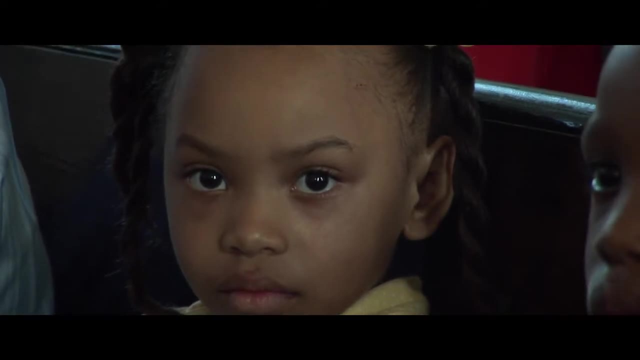 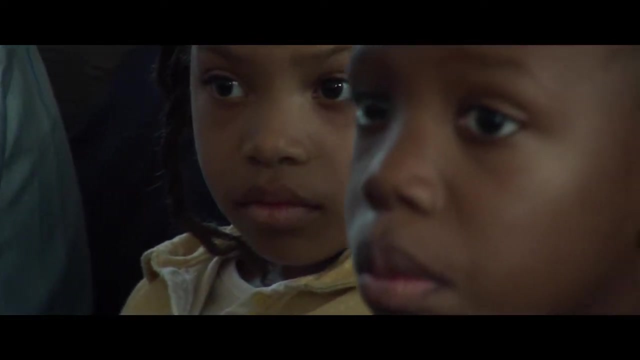 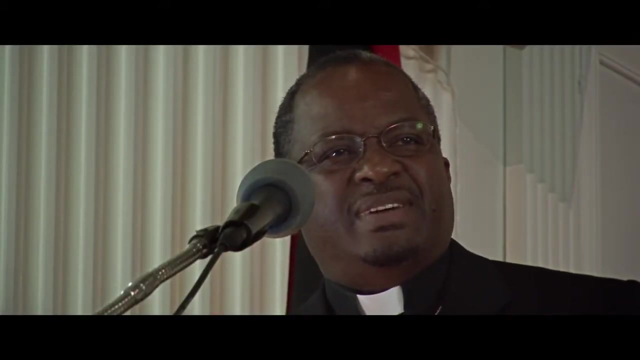 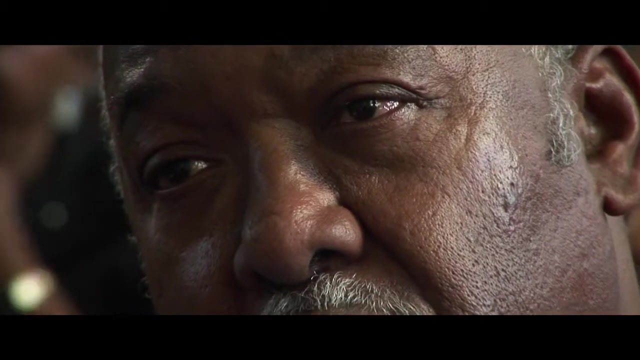 and has gotten rich off your label. How does it feel? How does it feel to be able to protect your pretty little girl from lustful advances? How did it make him feel when he was beat like an animal for acting like a man and rewarded with food thrown on the ground for acting like an animal? 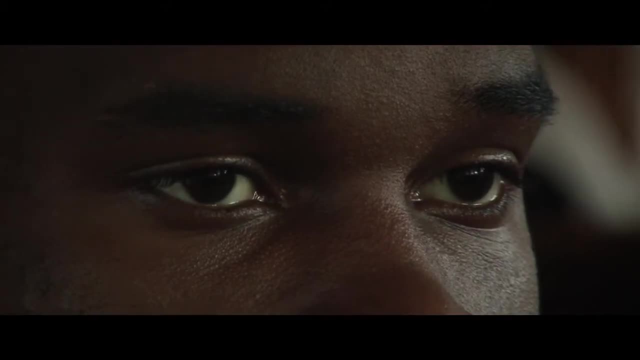 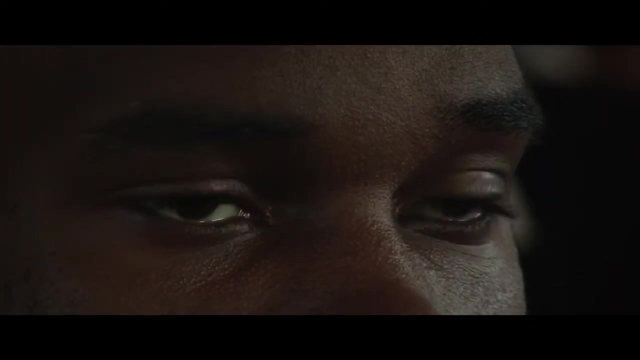 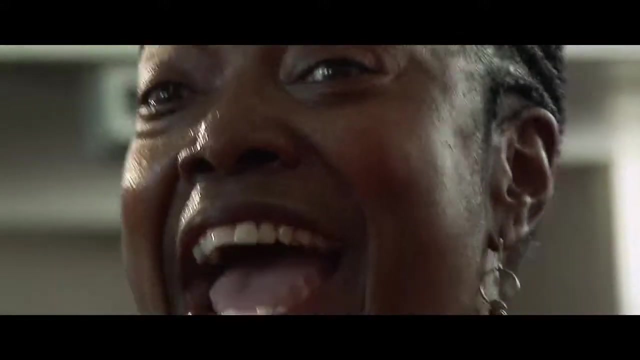 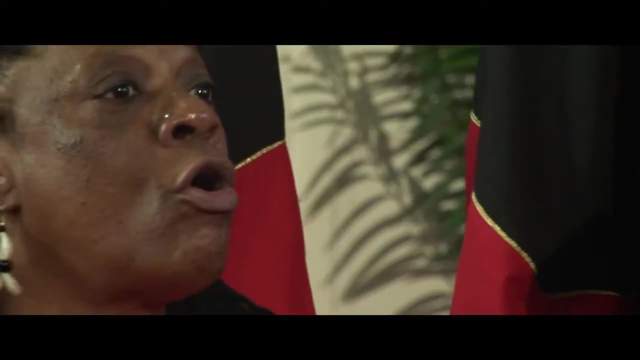 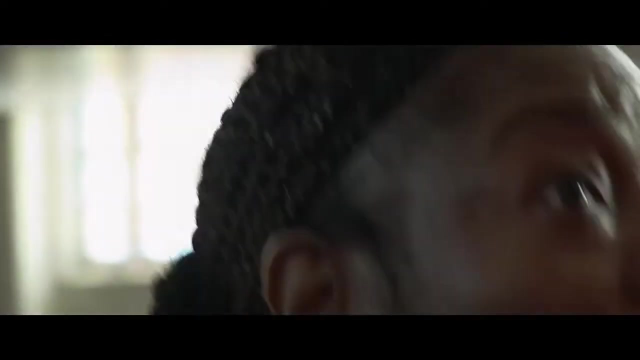 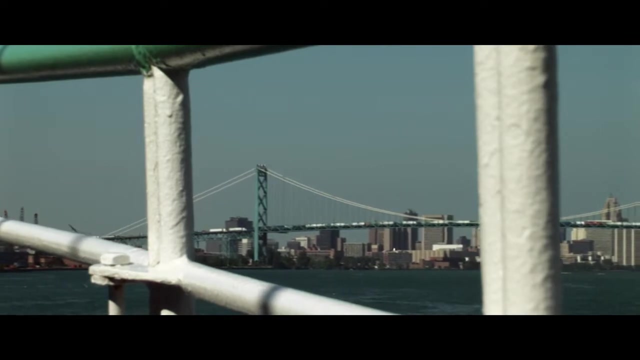 How did it feel to be called boy until he was old and then called uncle for the rest of his life, but never called a man? How did it feel to be called boy until he was old and then called uncle for the rest of his life? 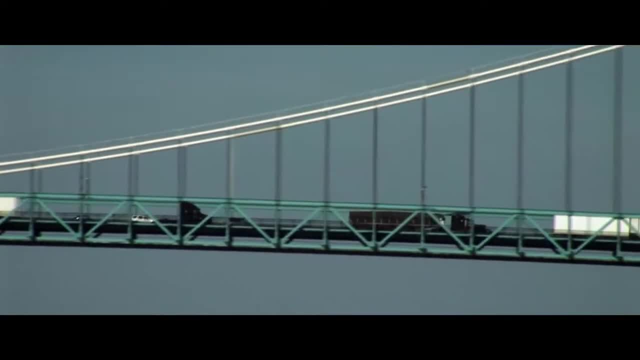 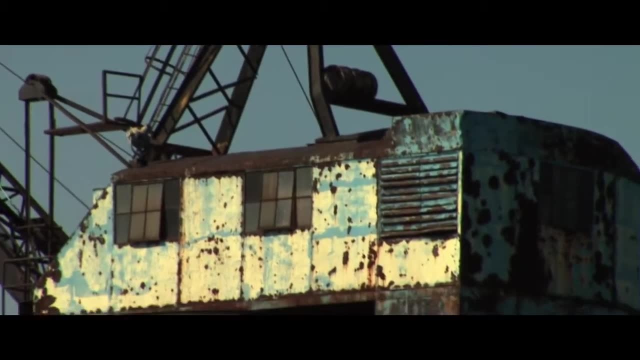 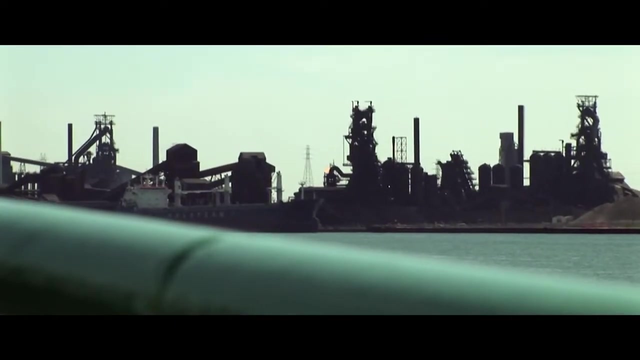 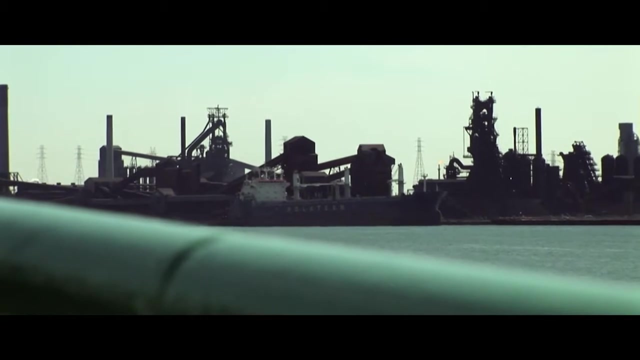 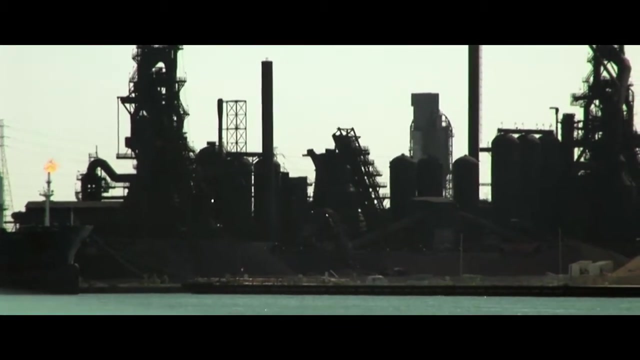 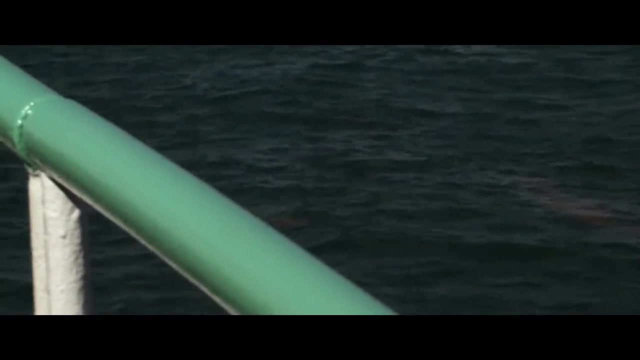 How did it feel to be called boy until he was old and then called uncle for the rest of his life? How did it feel to be called boy until he was old and then called uncle for the rest of his life? It was a brutal system of slavery that was unknown in human history. 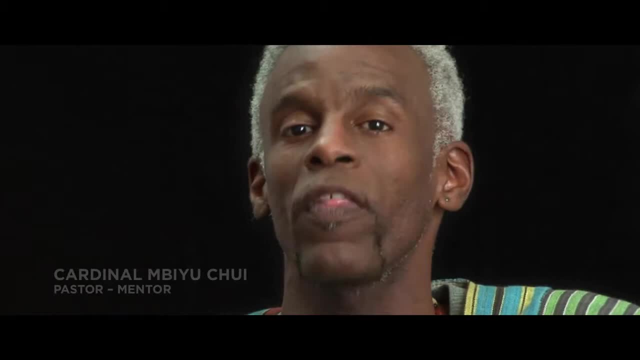 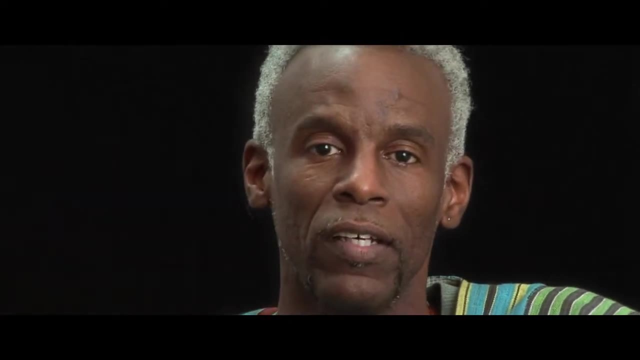 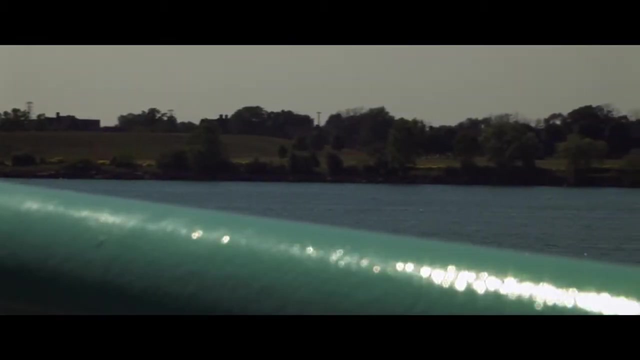 See, slavery wasn't new in Africa or any other place in the world. There were always servants throughout human history. But the African had no concept of the kind of slavery that the transatlantic slave trade was going to bring to them. The middle class was going to bring them slavery. 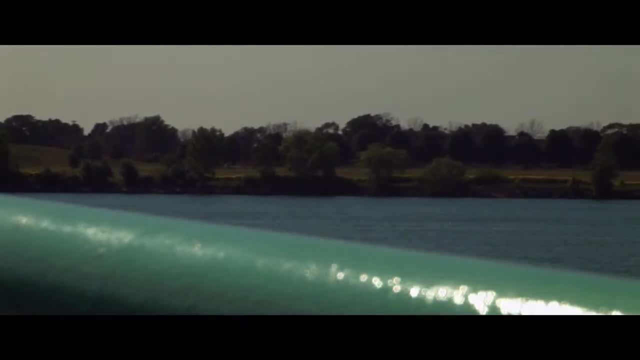 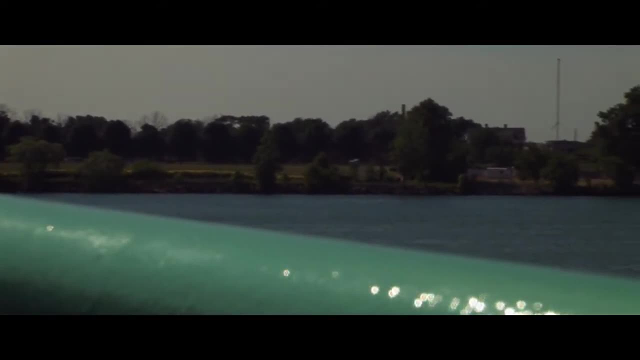 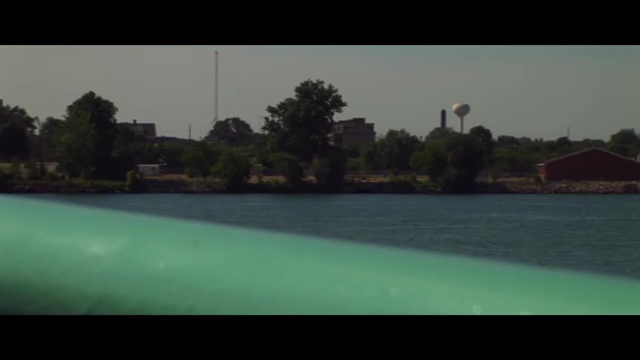 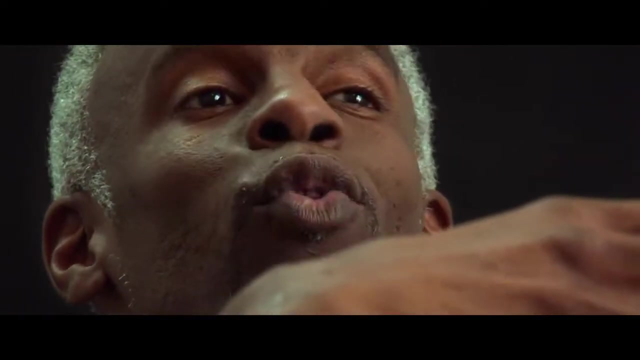 The passage when Africans were taken, just by virtue of the nature of the voyage, determined a whole different kind of system of institutionalized slavery, Because, in order to make the 90-day voyage from the western coast of Africa to the New World required that Africans endure the most implorable conditions. 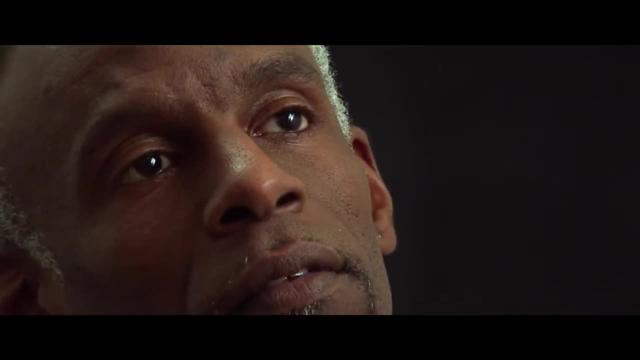 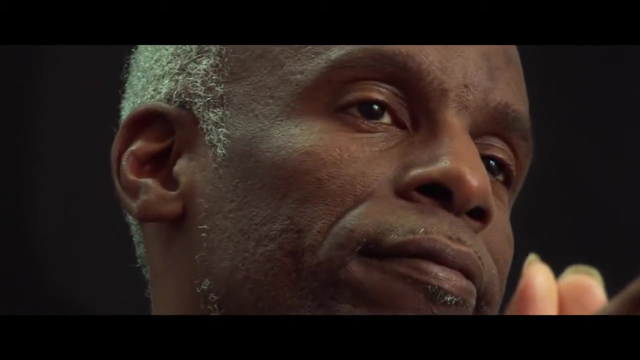 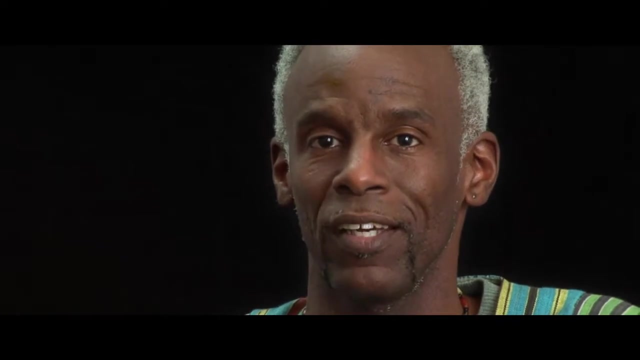 We were packed, Faced the back, side by side, in the hold of the ship. 90 days of wondering why is this happening to me, Where am I going? What is my fate once I get there? Many Africans never made the journey. 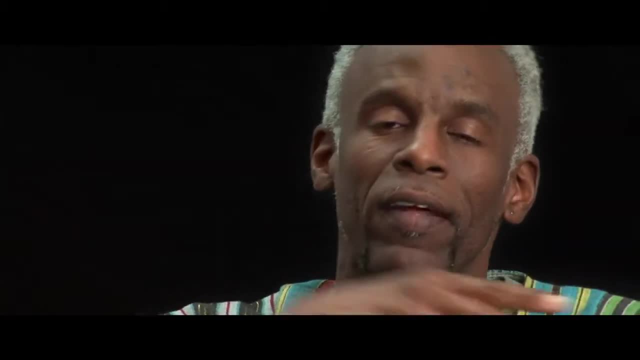 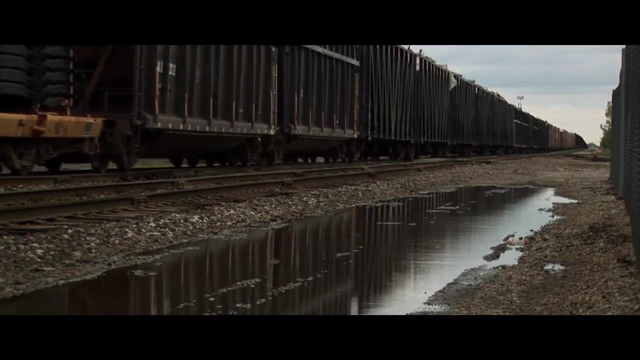 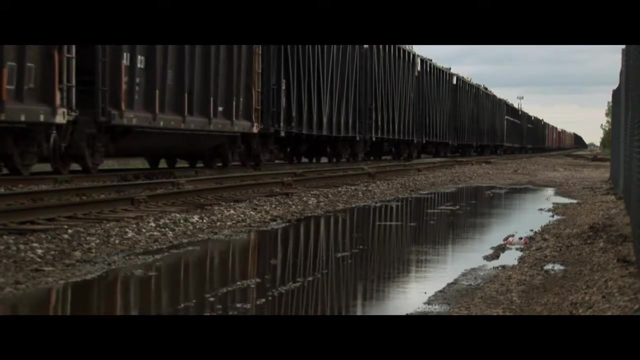 More died along the journey along the path than made it to the shores where they were being taken. It wasn't just the implorable conditions of the Middle Passage, but it was the seasoning process, Where we were put on auction blocks and sold like cattle. 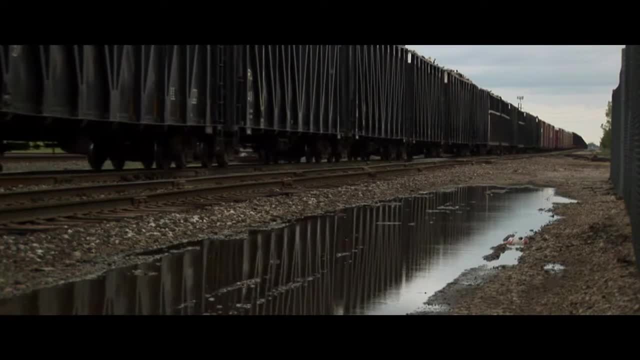 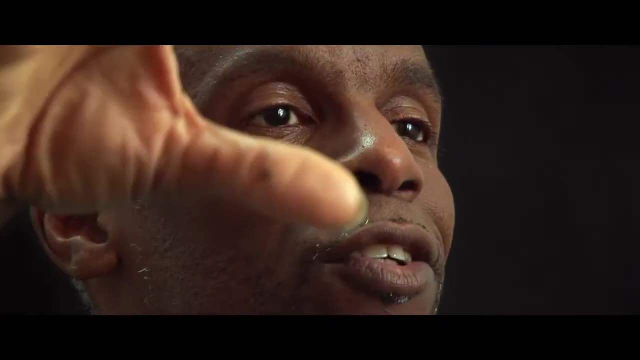 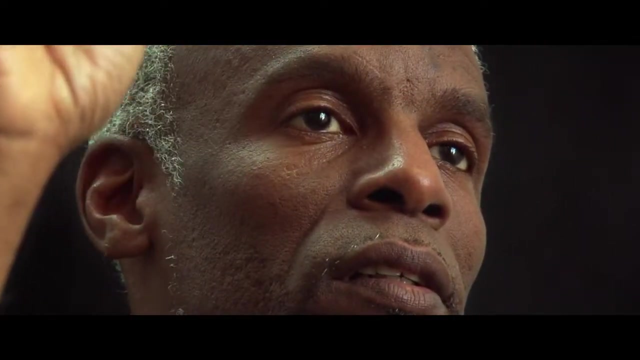 Branded like cattle, Separated mother from father, children from parents. We were given strict laws and governed under these guidelines of: how do you treat someone who is considered 3-5ths of a person? How do you treat chattel? 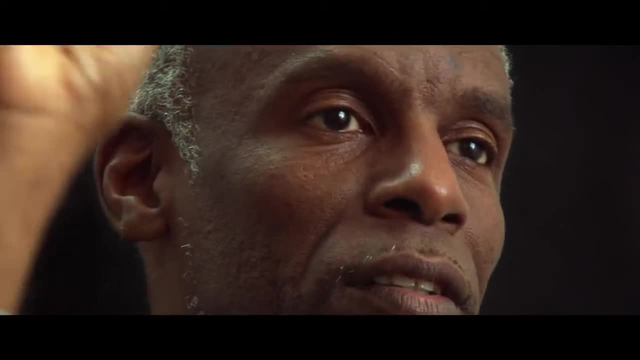 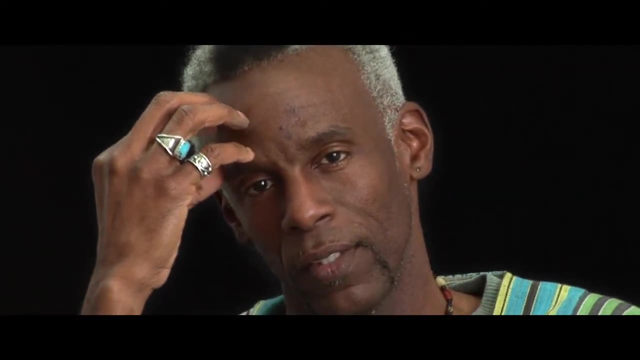 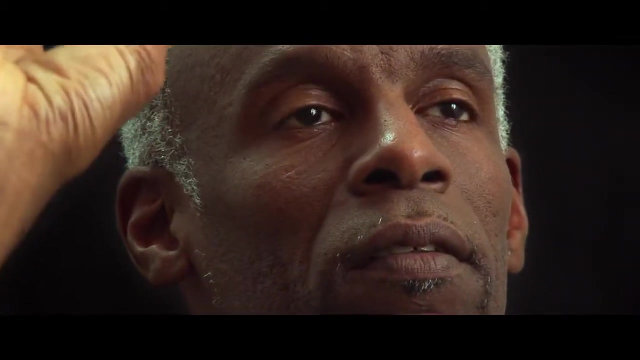 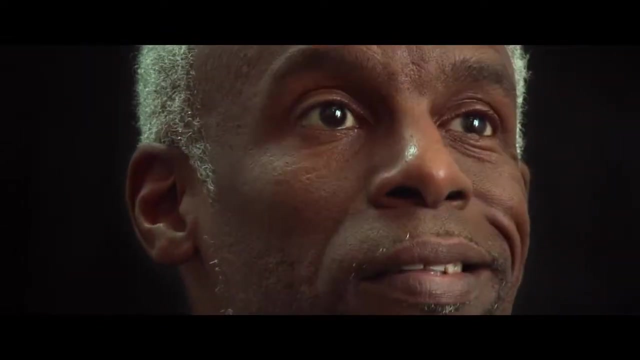 And so all of these experiences created some deep wounds in the African psyche, Created what we call a negro, A nigga. That's a human being who has been conditioned to hate him or herself. That's exactly what a nigger is, Even after the Emancipation. 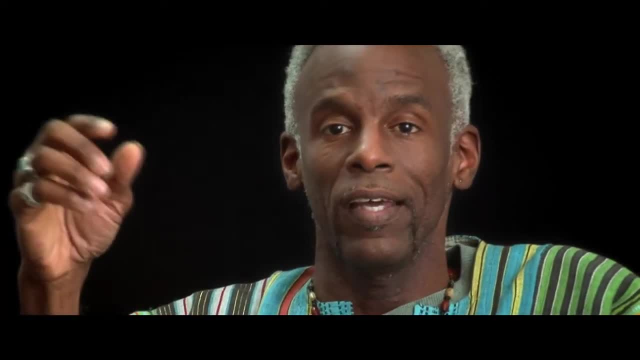 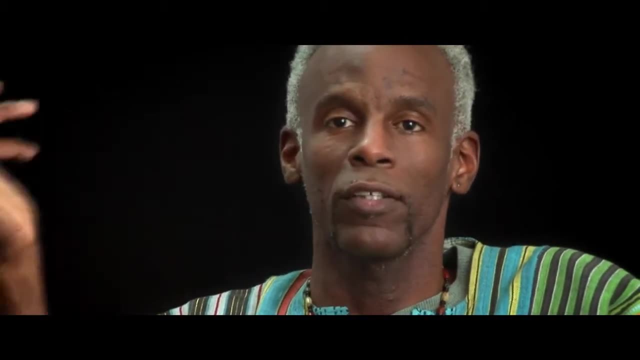 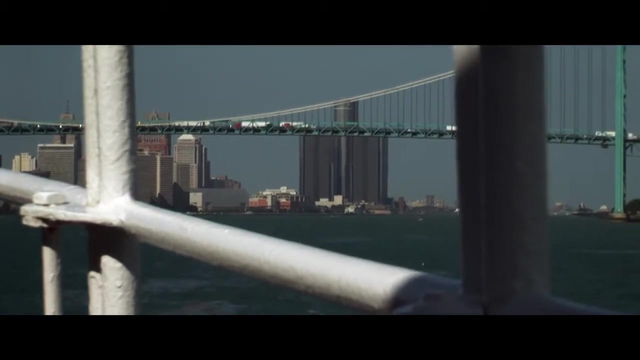 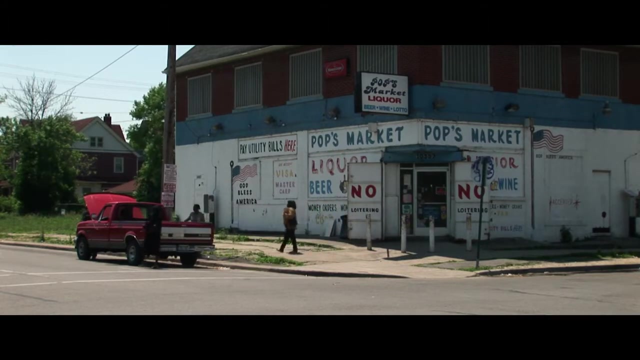 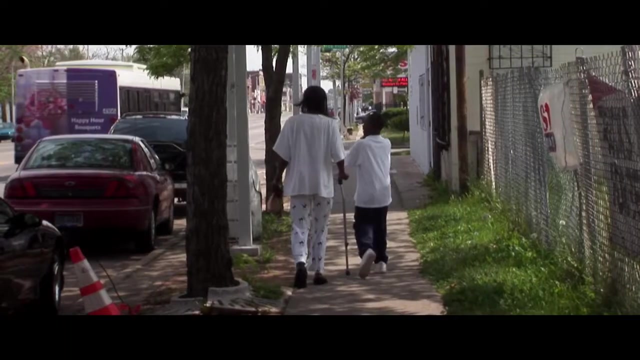 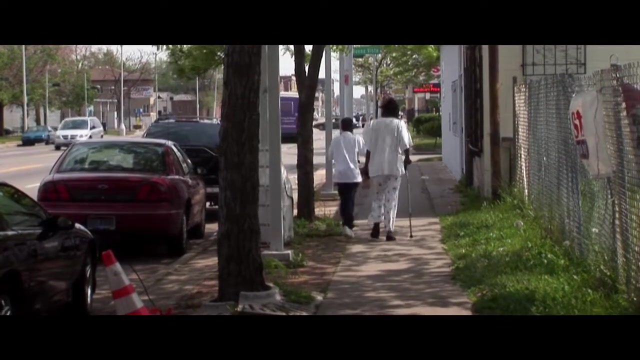 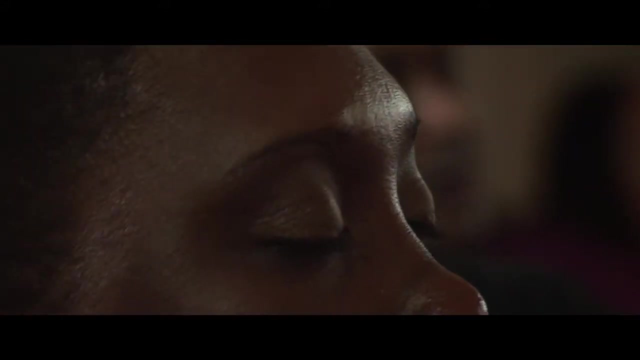 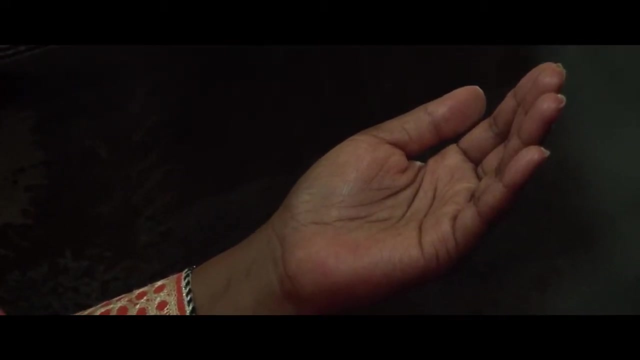 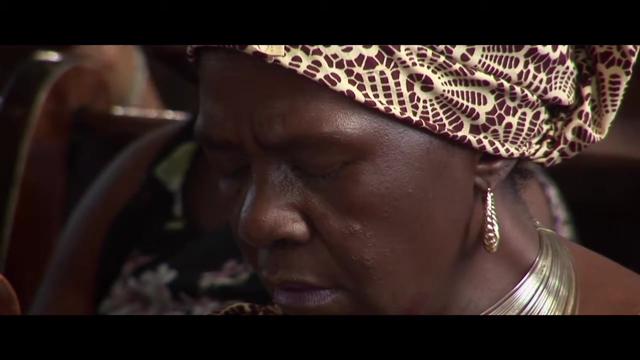 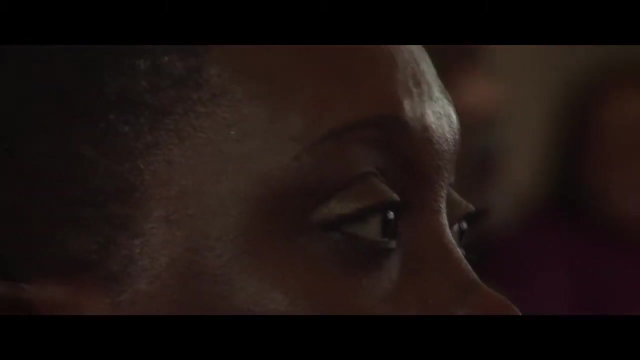 Proclamation was signed and slaves were set free. the damage that had been created, the wounds from the African Holocaust did not disappear, And so, unless those wounds are addressed, there can be no recovery, There can be no renaissance. The mothers of the Congo, of Rwanda, the mothers of the mothers who have lost their children in this, 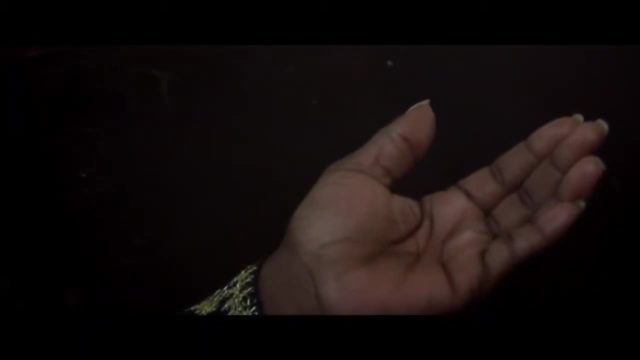 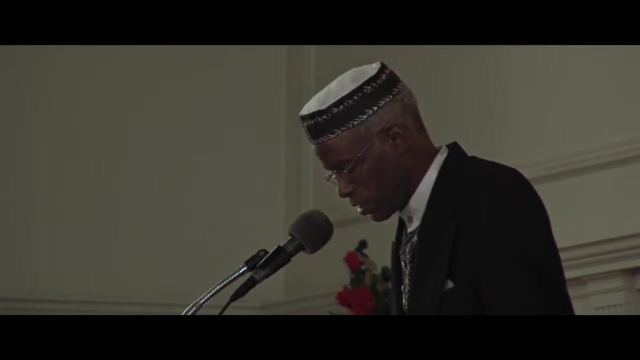 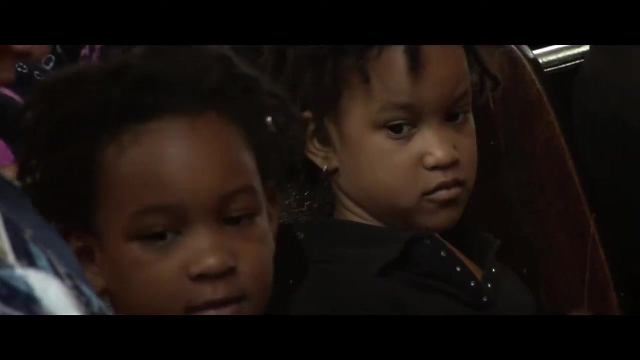 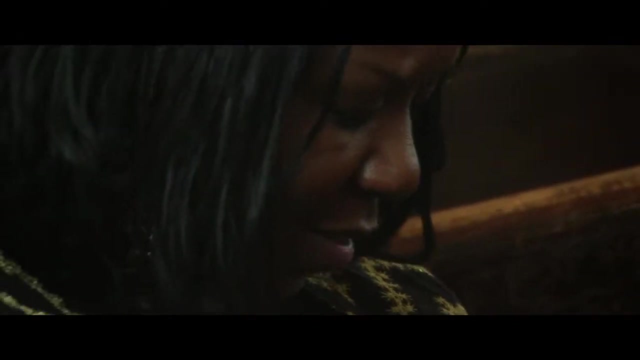 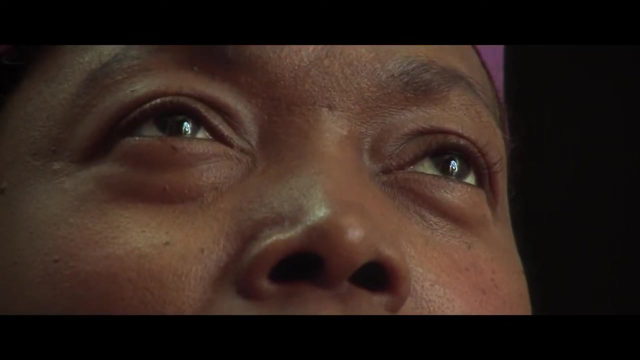 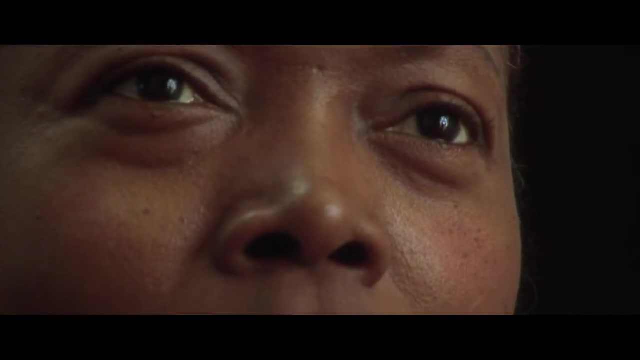 senseless war. Yes to us To hear our prayers, hear our cries, and we call upon your power, Barbara Doing-O'. Yes, Barbara Doing-O'. On April 5, 1994, I went to work that day and 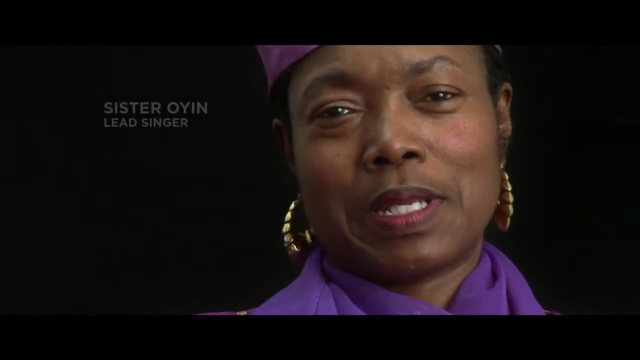 I got up- Barbara Doing- All right, Barbara Doing- And the woman on the phone was saying: I'm going to make a home that night. and my son greeted me and i asked him: had he done his homework and gotten ready? because it was near the end of the easter break? and he said: yep, ma got everything, i'm getting. 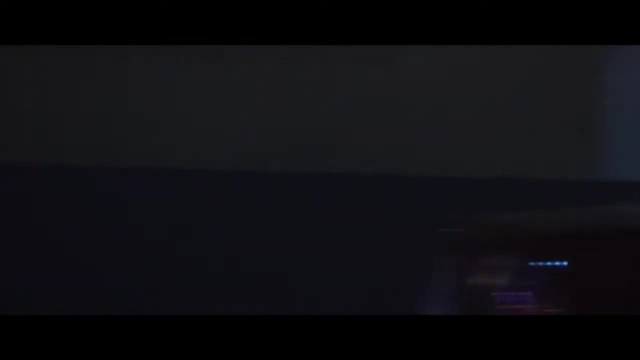 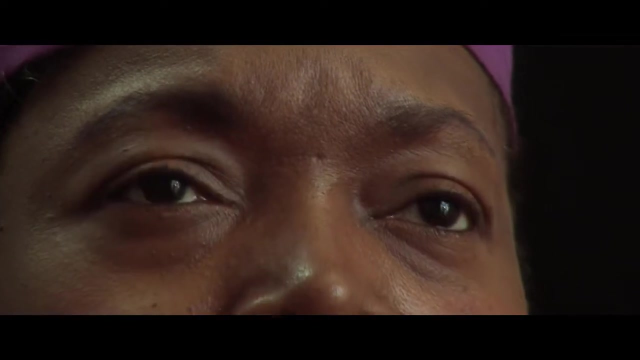 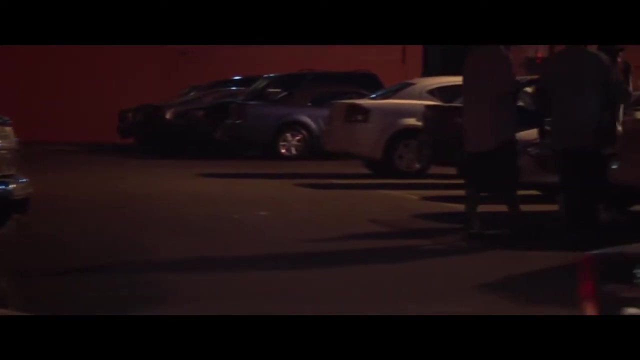 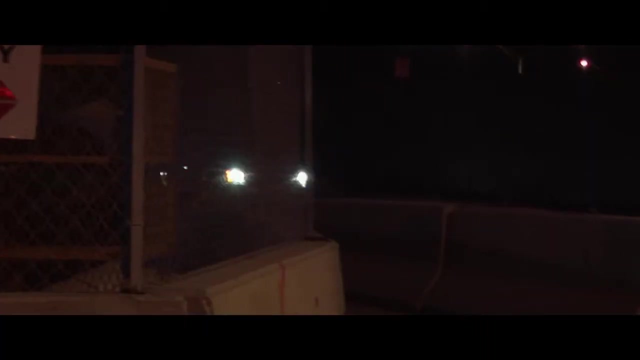 ready to go out. so he left out, and little did i know at that time that it would be the last time i would see him. my son was murdered. he was shot in the back three times. he was 17 when he was killed, so had he lived, he would be 30 this year. he was shot because he was driving the car of someone. 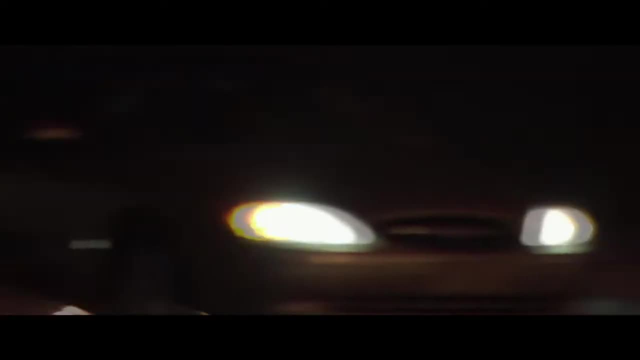 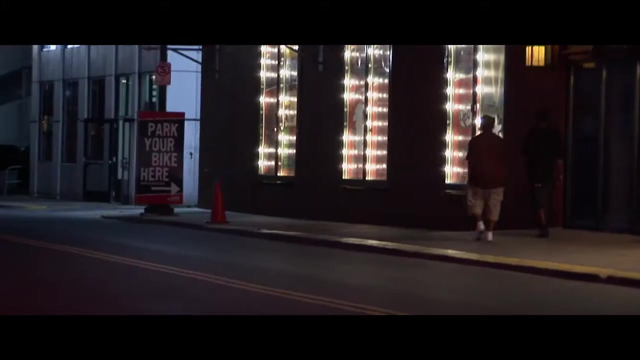 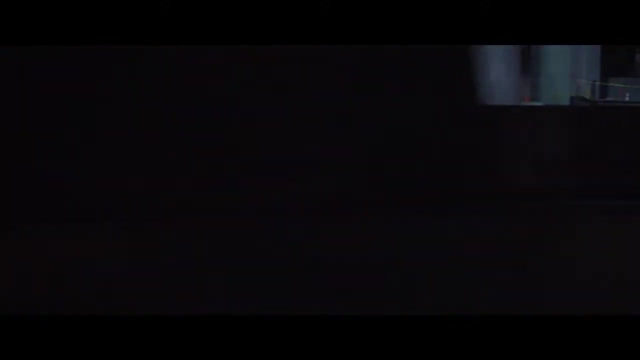 that another arrival gang in the neighborhood. they shot him because they believed that he was the person who owned the car. just every day you almost hate to turn on the news because there's just so much black on black violence that's going on and i think like 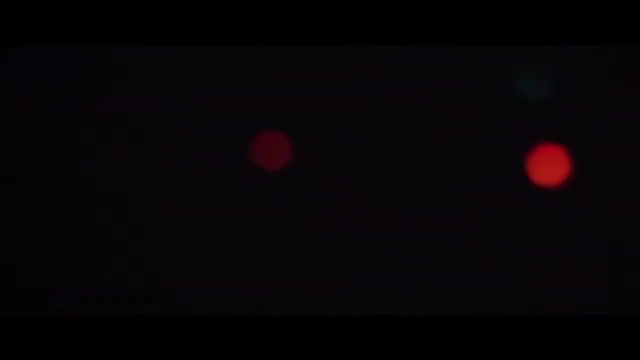 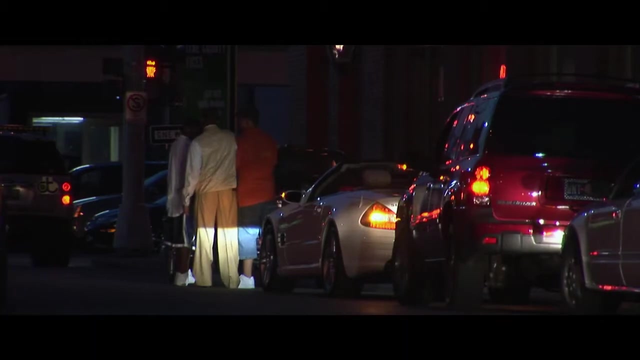 you know, you know a lot of young black men. he felt he was invisible. i think he was exposed to a great many of the things that, um, a lot of our young black men are today. um, there are a lot of temptations out there, the temptations to sell drugs, which i know. 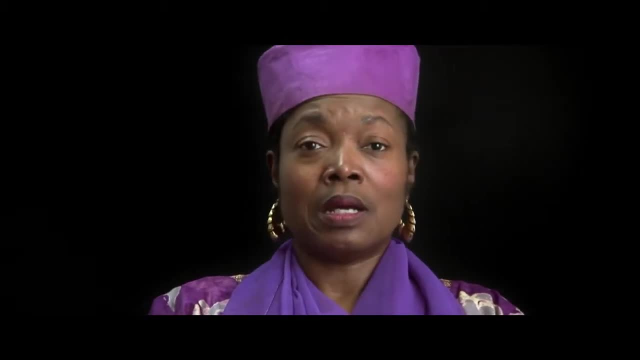 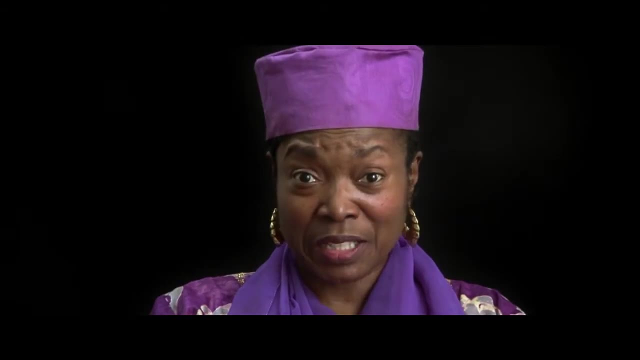 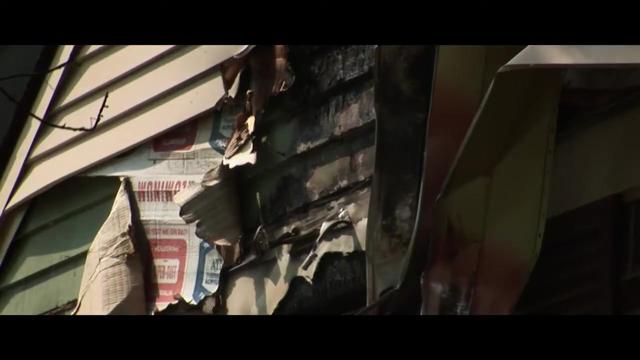 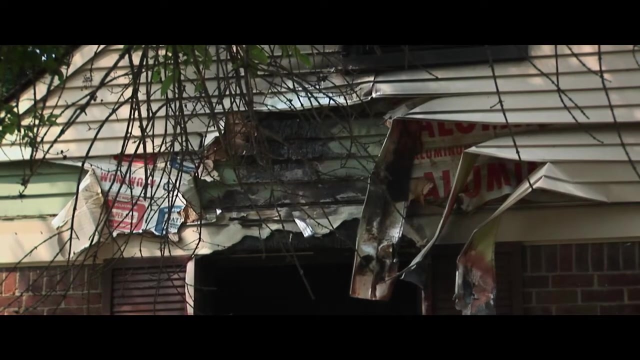 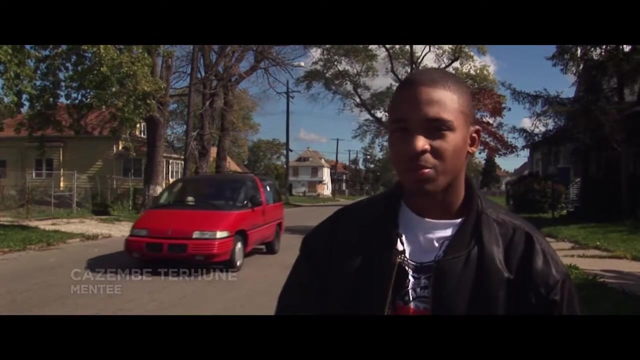 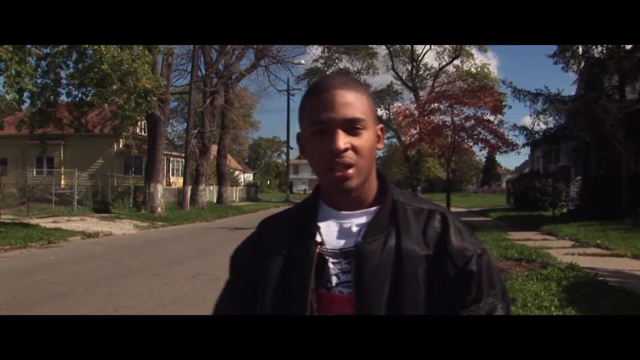 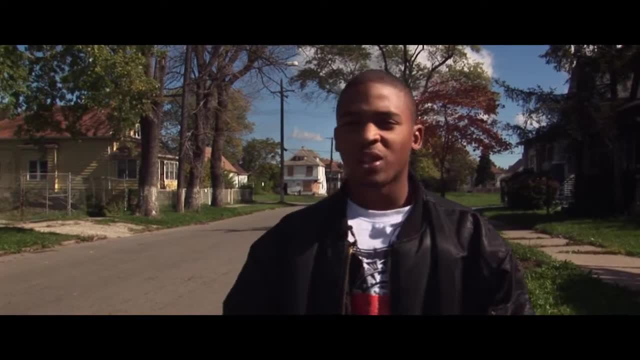 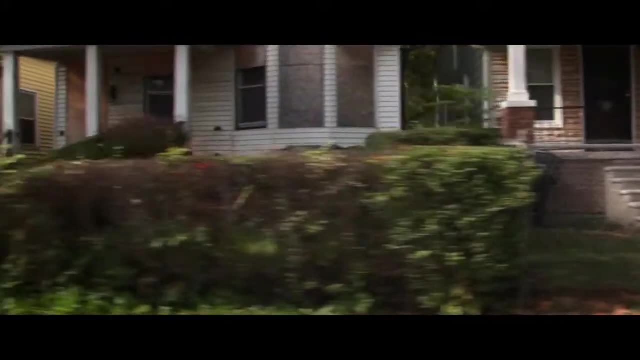 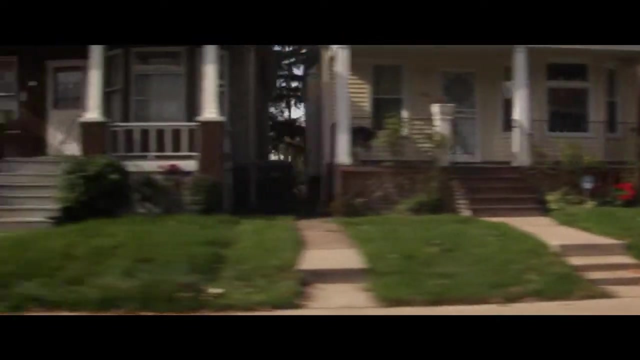 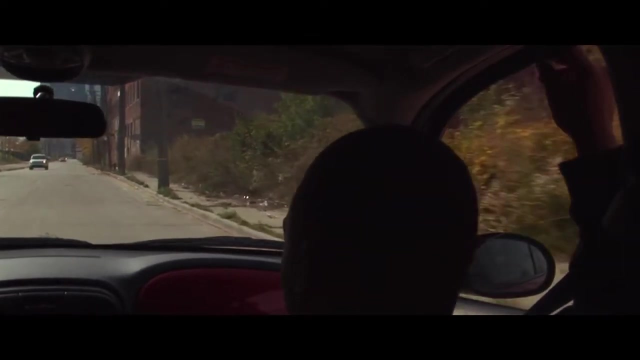 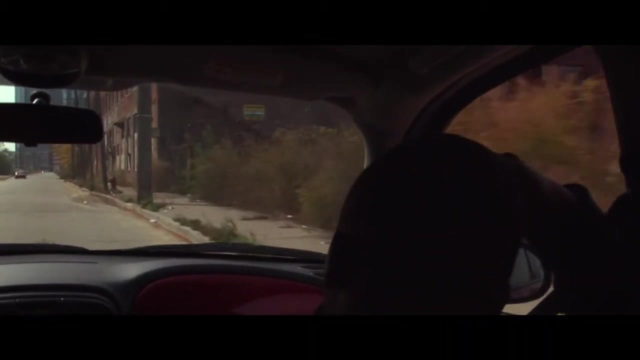 but they shot him point-blank in the head. it's the first time I see somebody get killed. numerous times I've been shot at, been in the area. I shouldn't have been in at the wrong place at the wrong time. you know it's one, two, three, four, I don't know. 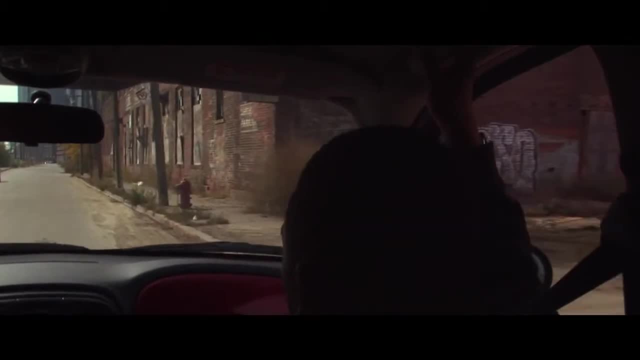 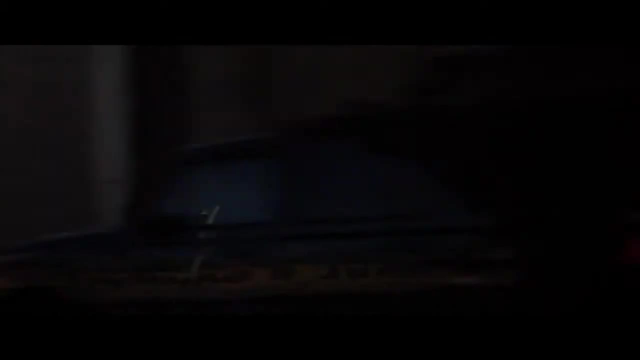 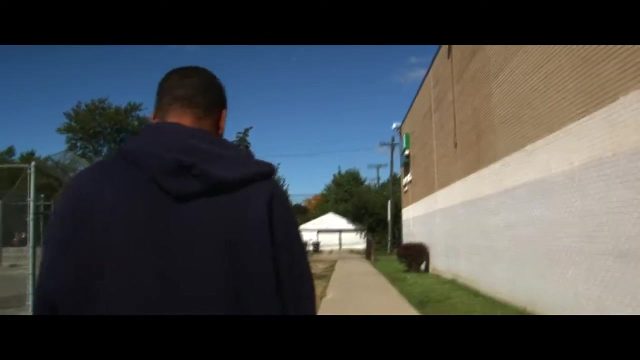 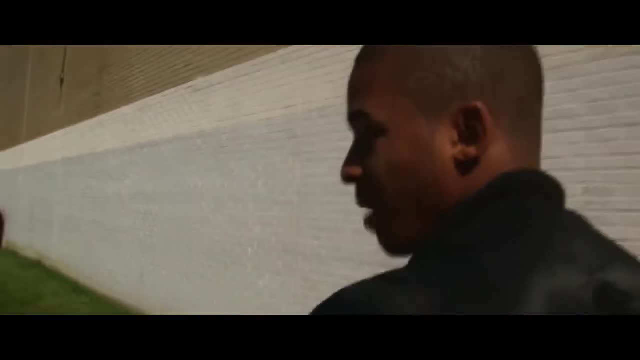 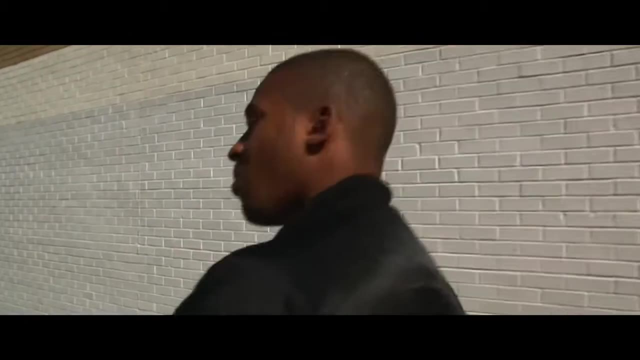 in front of the family and everything. you know it's like every time I go to that house- you know that's my, my childhood- is there time I go grab pass? I'm like I want to go in, tell my wife I want to see, with my father just standing. 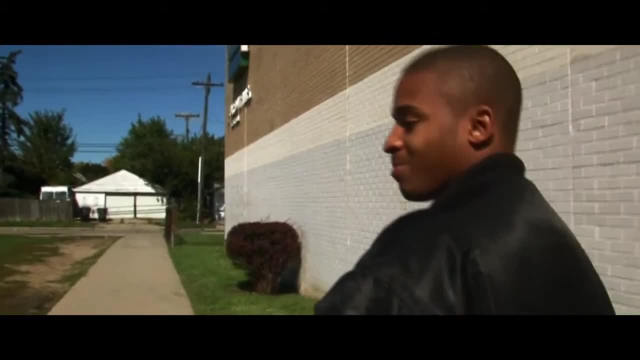 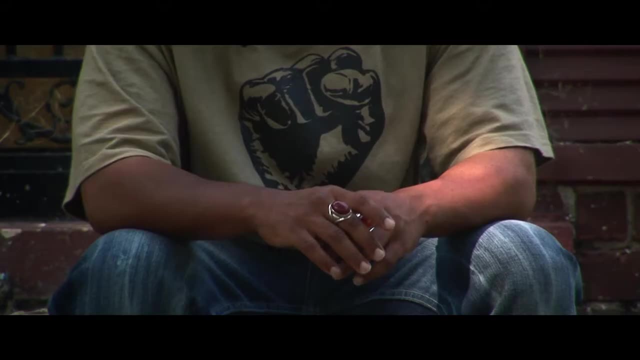 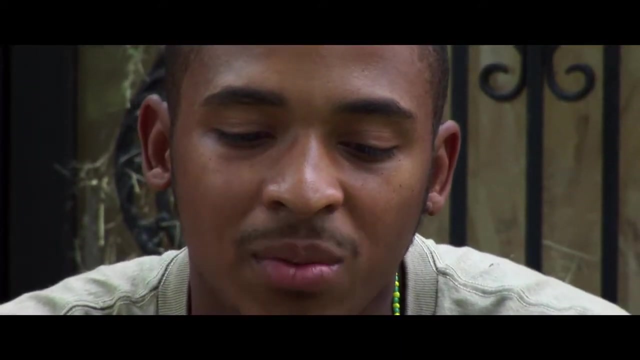 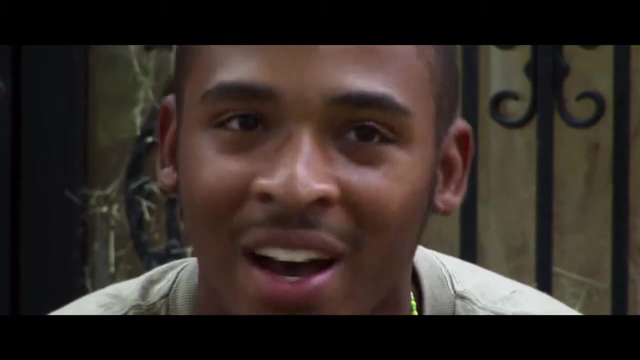 out there and the family out there welcome me in. but it's not like that. I didn't even cry until the funeral it was. it was shocking. I'm like this can't be happening. I mean, it didn't happen. my father's still alive. you know I refuse. 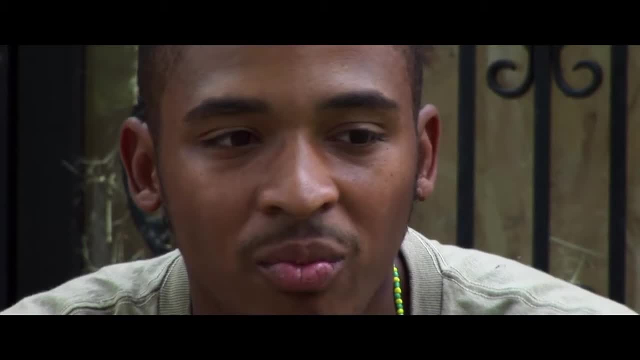 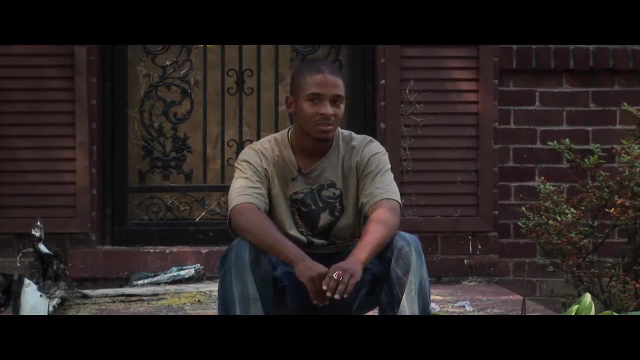 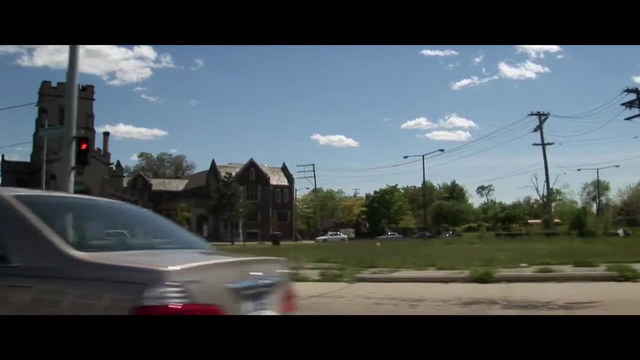 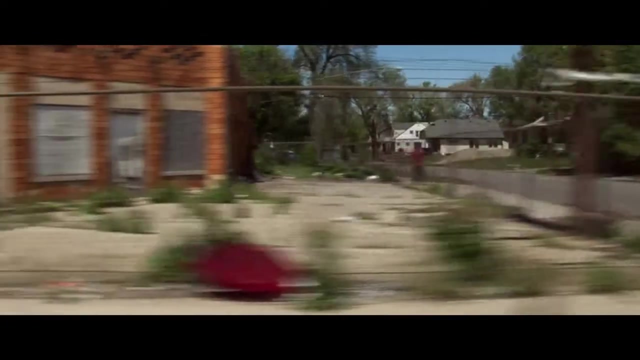 to believe that he died, but you know it was it was. it was a tragic loss. you're not. what's happening to black men in America is, in a word, genocide. it's genocide in a sense that it's the systematic destruction of a people. if you don't have men, you can't have a group, and the destruction of men, in the numbers and to the 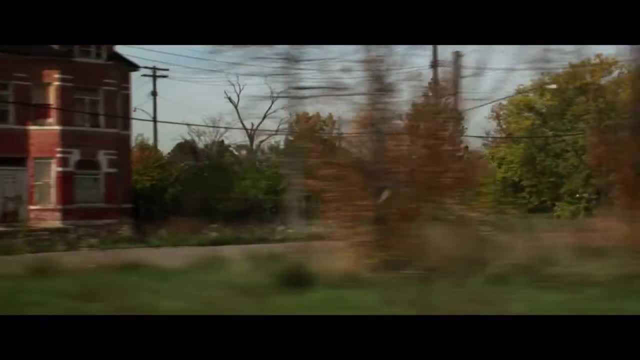 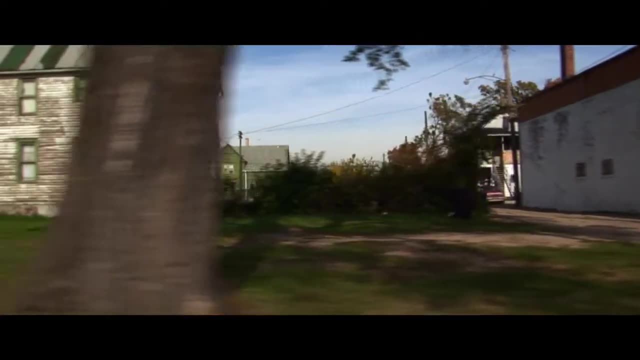 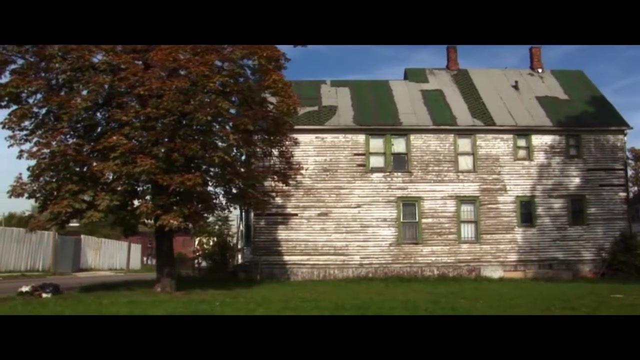 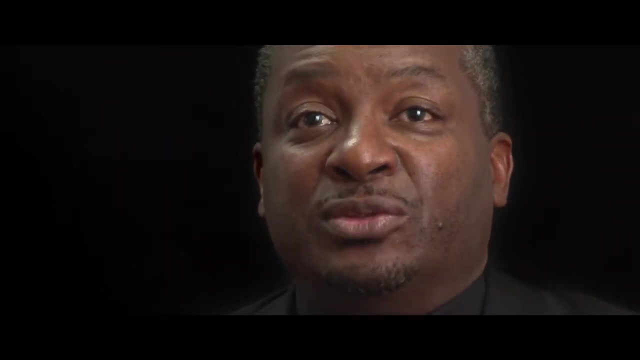 degree that it's occurring is effectively genocide, whether it was intended or not. people are falling through the cracks in a way in which, if it were anyone that had political power to bring this problem into public consciousness, there would be an outrage. but because it is basically a pariah group, that is, being that this is happening to, it's a quiet. 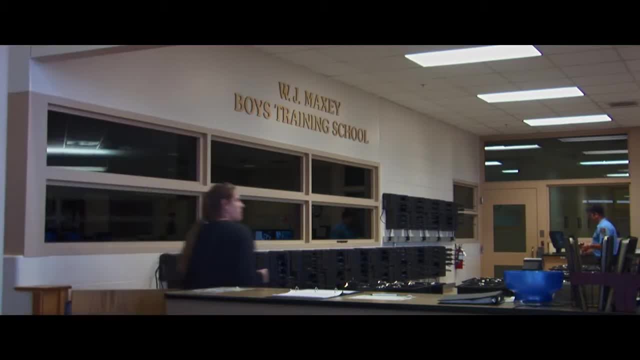 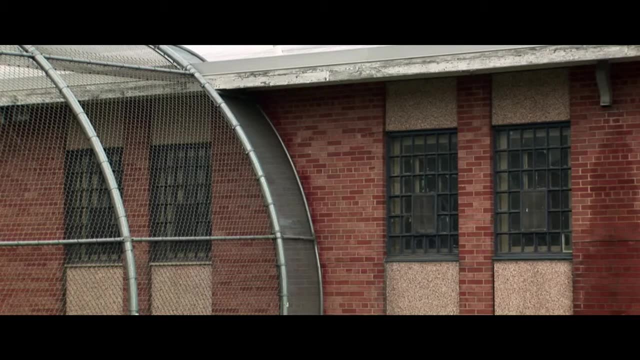 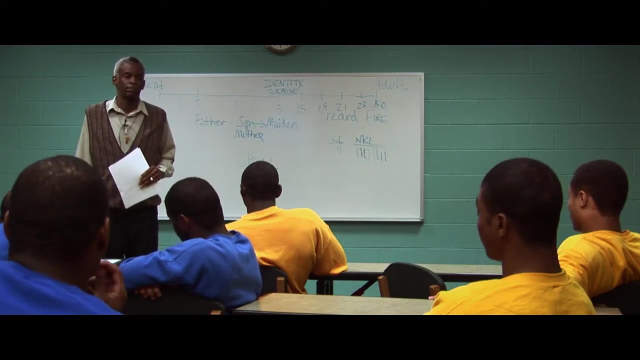 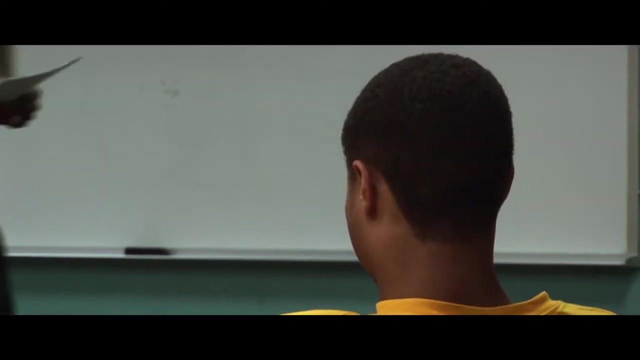 genocide. my friend, there's something special about a relationship between a mother and a son. you know what I mean by that. um, they have a special bond. a lot of times it's the spell blinds the relationship, so the mother doesn't really see the sun and what the sun is really doing. 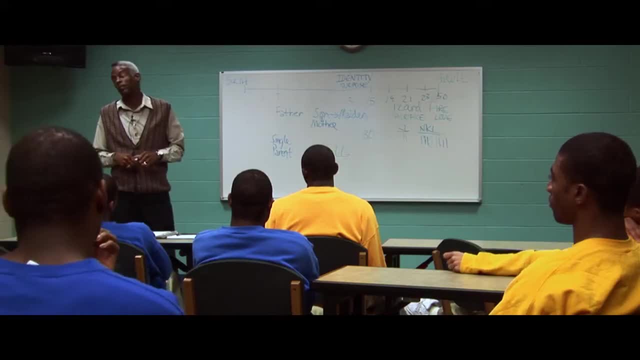 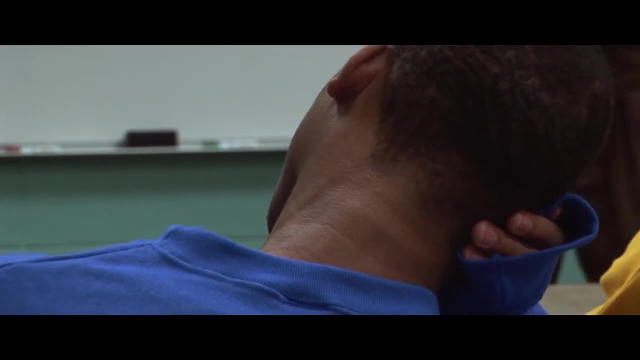 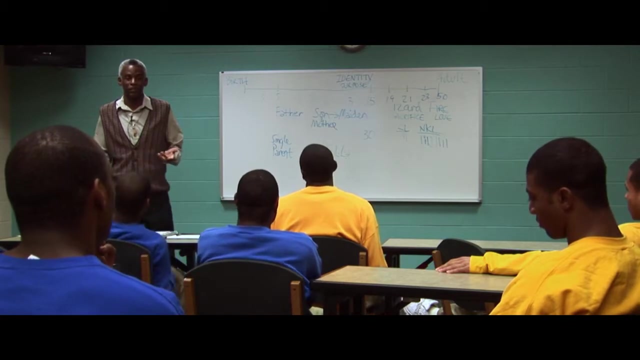 she know he's he's making wrong choices in decision, but she's looking the other way. that's my baby. that's my baby. they standing there in front of the judge. she said, no, my baby wouldn't do nothing like that. Yes, your baby would. yes, your baby would. but that that's the blindness of that relationship, and 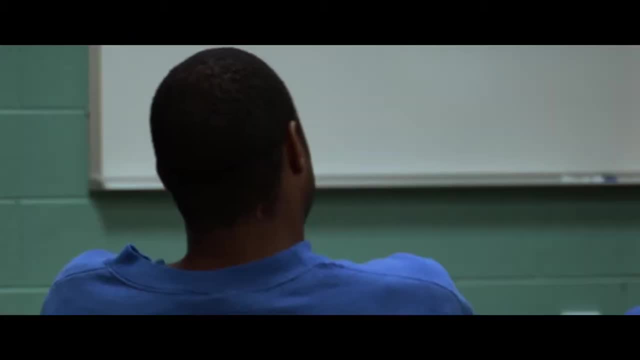 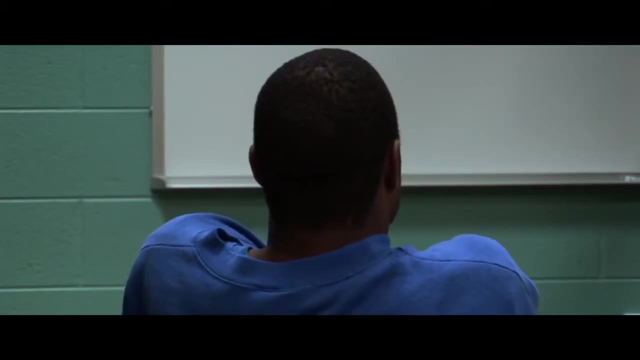 that's why the spell has to be broken. it's like they still got the umbilical cord attachment and At some point you got to cut the cord. You have to cut the cord. Your mama can't cut it. Either you're going to be a boy or you're going to be a man. 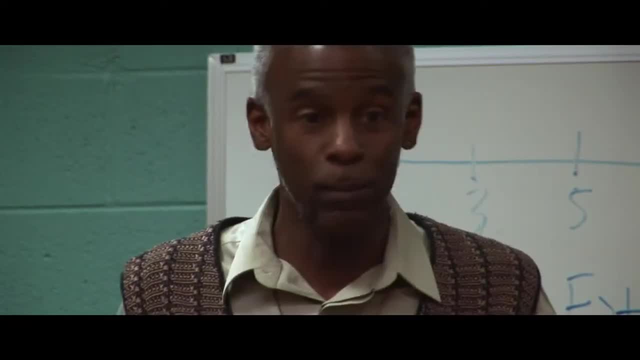 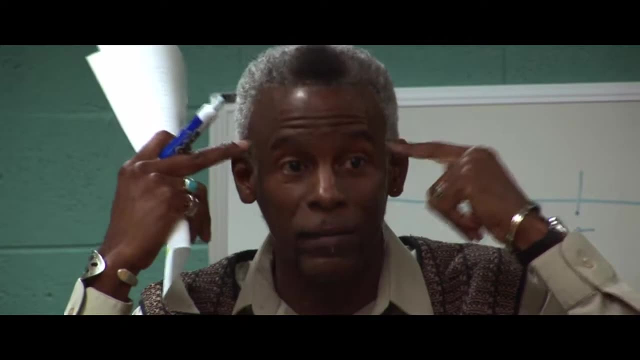 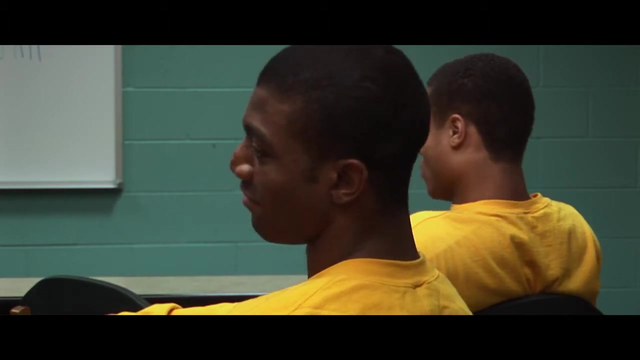 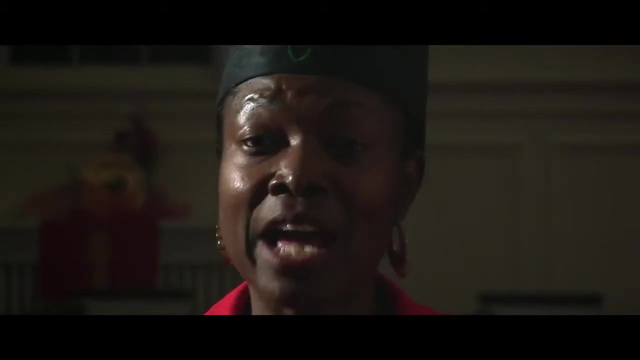 If you don't cut the cord, you'll never become a man. You're just a boy living with your mama. It don't matter where you live. you're still living with your mama. Why should I feel discouraged And why should the shadows come? 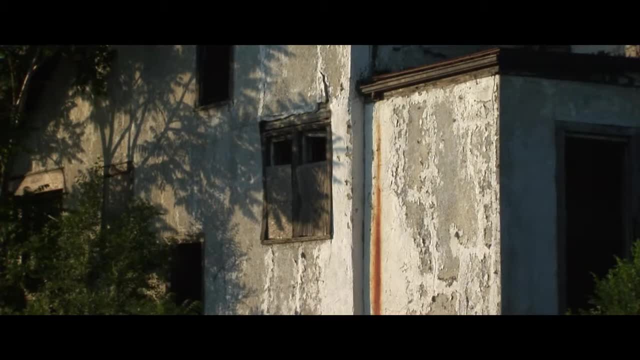 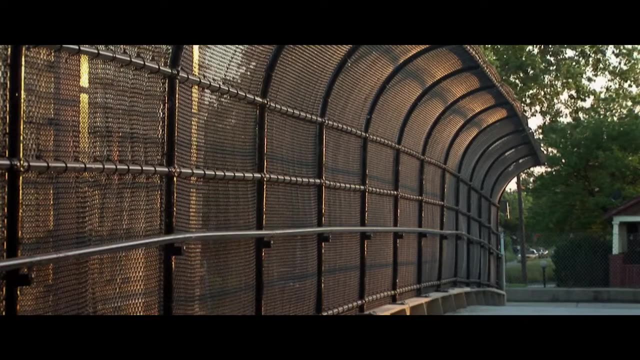 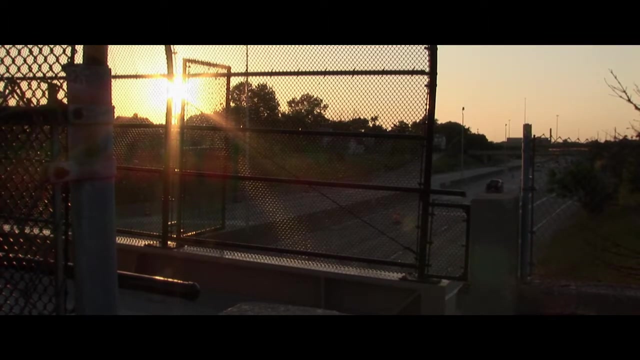 Anybody here didn't come from a single-parent family. Why should my heart be lonely? Okay, only two, three And long for heaven and home, But most of us grieve. We grew up without both parents. That's the reality in our community. 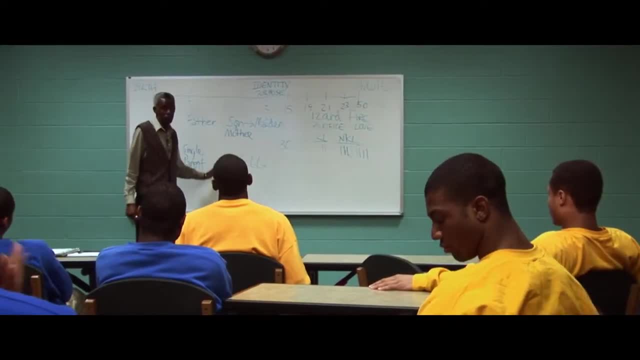 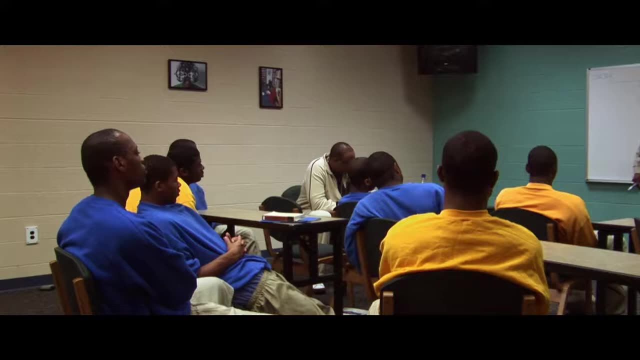 And so that makes this spell even more dynamic, Because you ain't got but one parent to lean on. You don't have your father A lot of times, even in the absence of your father in the home, Like my father was an alcoholic. And my mother and father got divorced when I was five And so I really never really knew. I have a memory of him from, you know, when I was five and younger, But that memory was all negative. You know, he was always drunk. 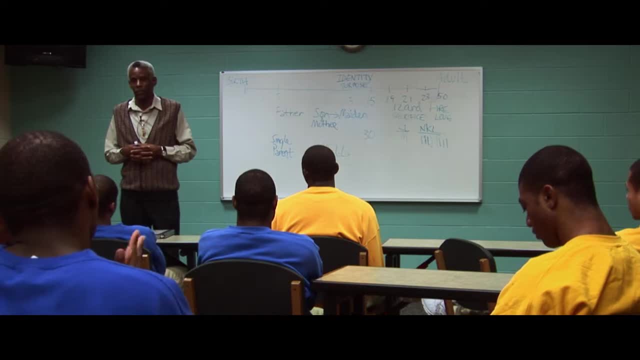 He was always beating up my mother. That's not a good memory, But as I got older, my father would call, call our house to talk. Nobody would talk to him except me. I would just listen. you know, I never knew what to say. 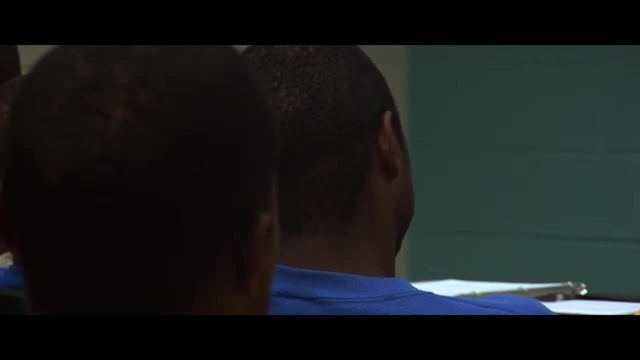 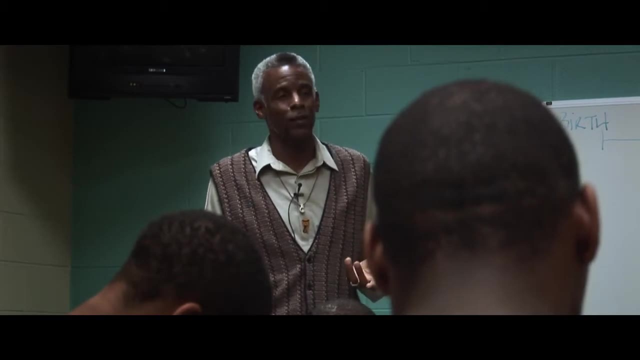 And he was always drunk, But I knew I was in his heart And that meant a lot, And all I'm saying I have to say is that that's true of all of you. There is no parent on earth that doesn't want to be with their child. Doesn't want to love their child. There are many circumstances in life that makes that impossible, Addiction being one of them. I got caught for stealing a car. I was 15 when that happened. I just turned 15, so that would be about four years I've been in the system. 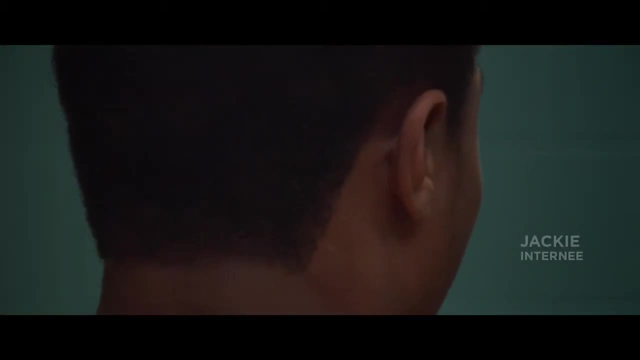 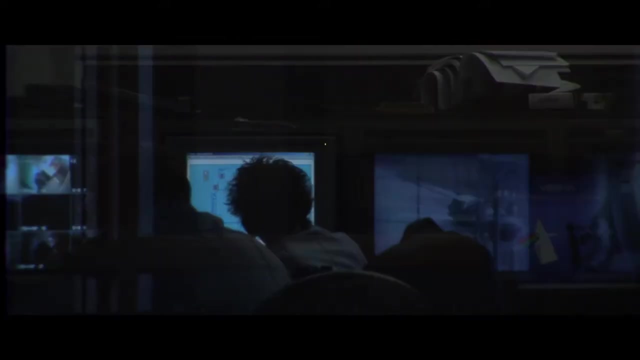 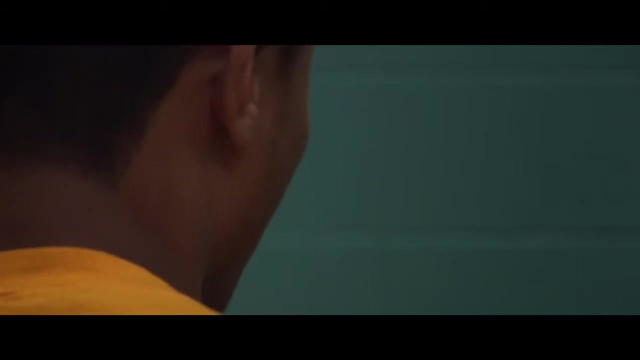 For that one little petty crime. That was about it. I stole that vehicle, Got chased, Ran from them, Caught me, Got caught up in the system. I never knew my daddy. He was a crackhead, just like my mama. My mama not, no more. 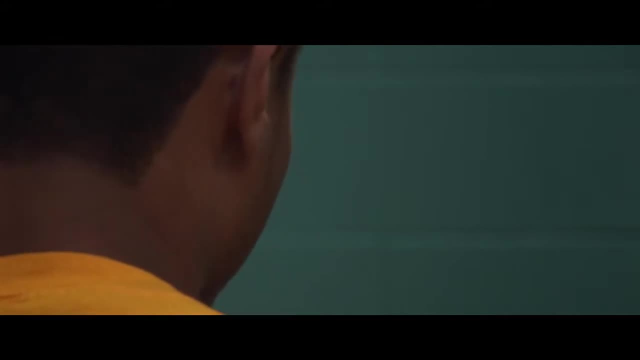 She got off of me. you know what I'm saying. She's a strong woman. My daddy: I don't know him to this day. I just seen a picture of him Never even, Didn't even have a conversation with him. 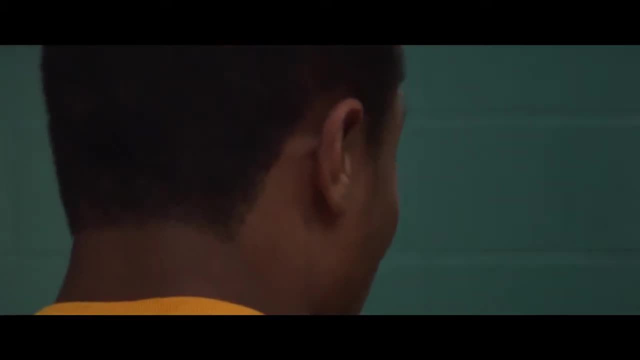 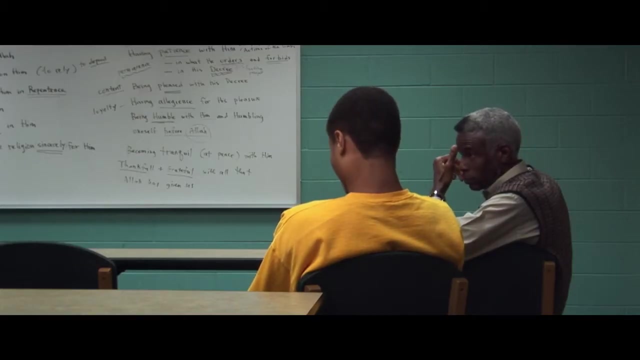 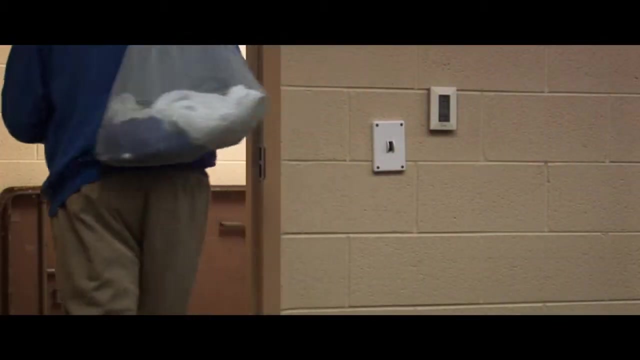 Didn't know him, My mama. she's still in my life to this day And, like you said, I ain't ready to cut that cord. I sing because I'm happy. I sing because I'm free. I sing because I'm free. 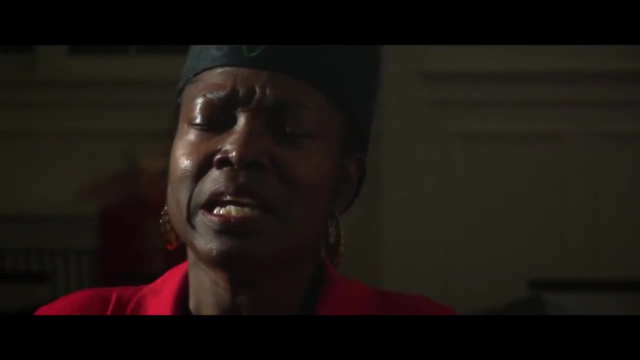 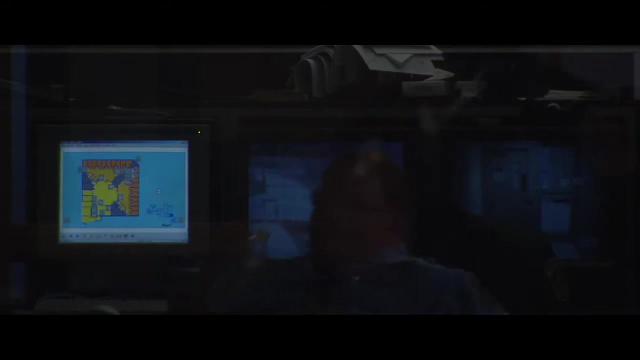 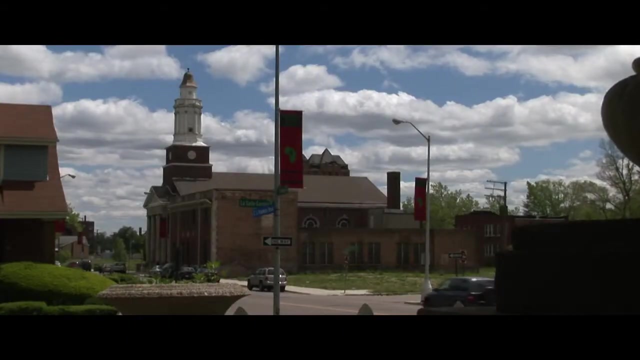 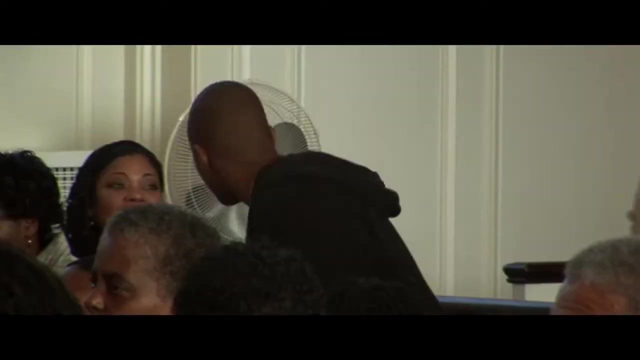 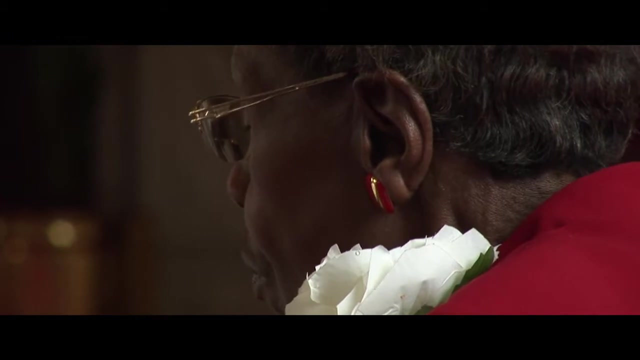 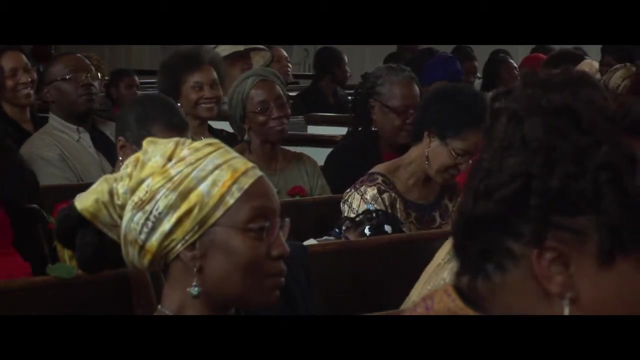 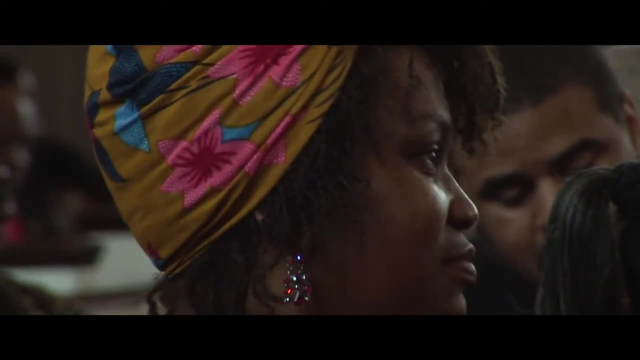 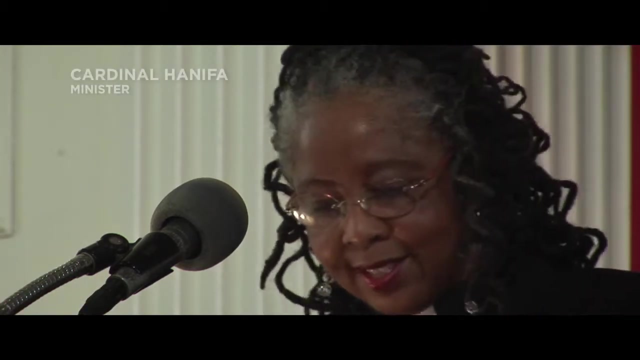 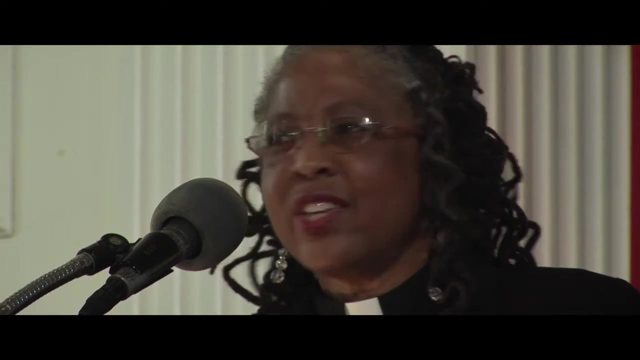 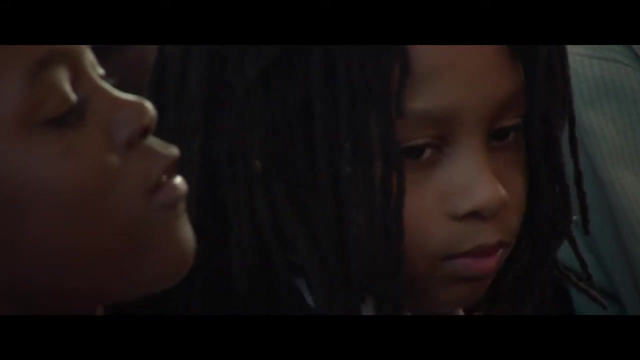 And she would say: yes, mama. And old Sockway would just give me that smile, With that charming insight of his, And he would just mysteriously change the subject, You know. And then, you know, Ta'u just completely turned the tide. He would start preaching to me. 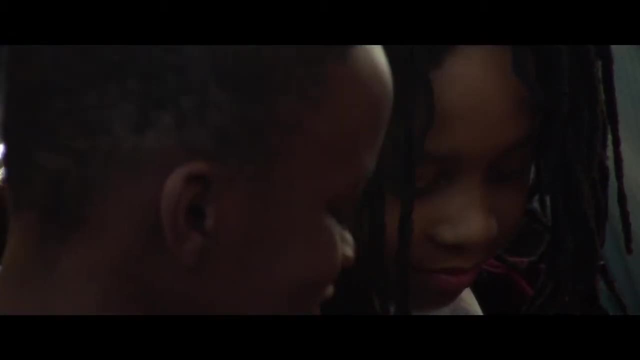 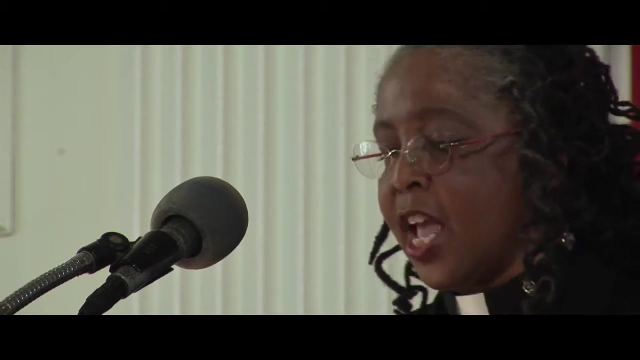 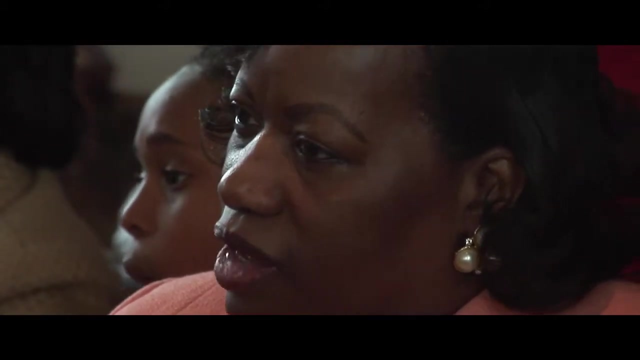 You know I told my son, old Sockway, a long time ago I could be your mother but not your father. And right here in the community of Jesus There are brothers who reached out to him. You know it takes a village. Bishop of the Willing. 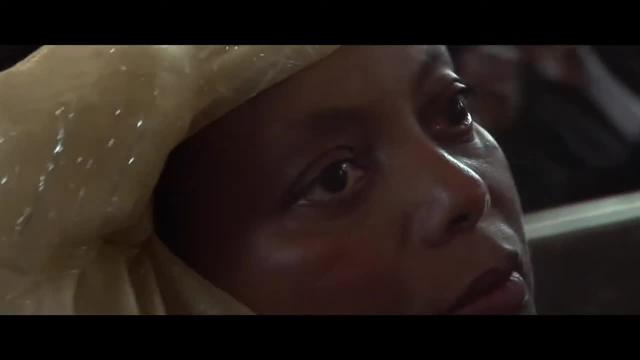 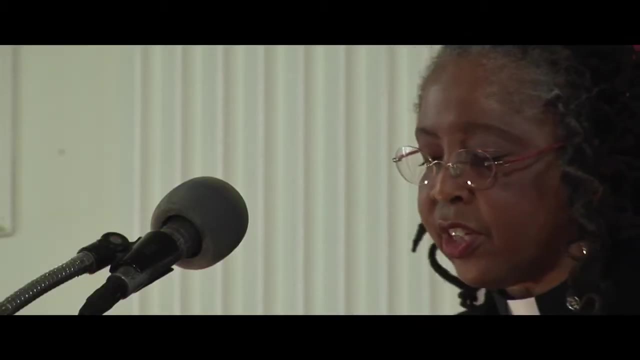 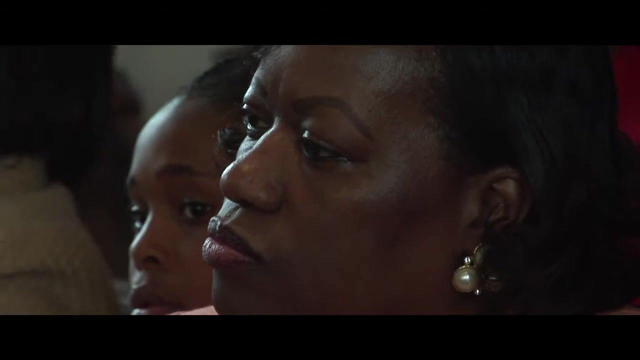 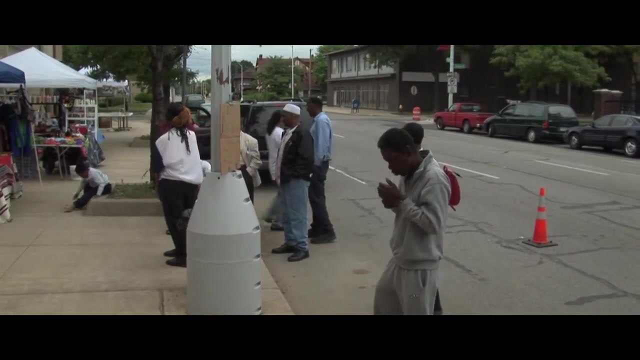 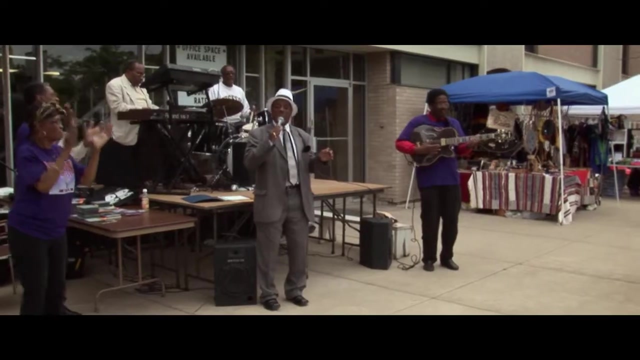 Brother of the Child. I didn't have to do it alone. Sisters, we need our brothers, Our sons, our fathers, our uncles and grandfathers. They need us and we need them. All right, Rock me, baby. Rock me all night long, Yeah. 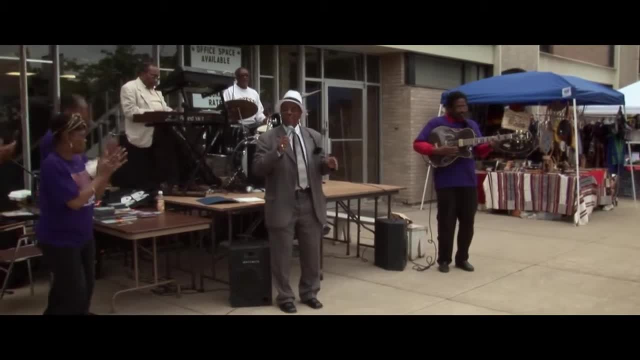 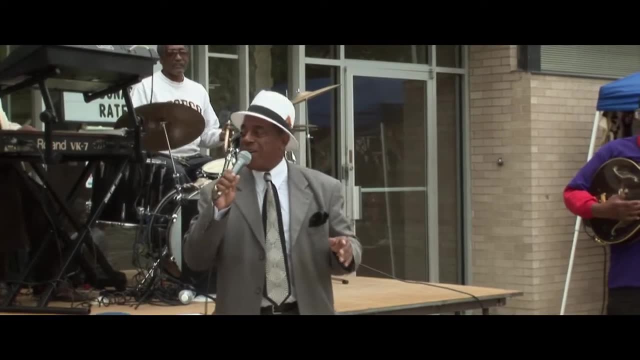 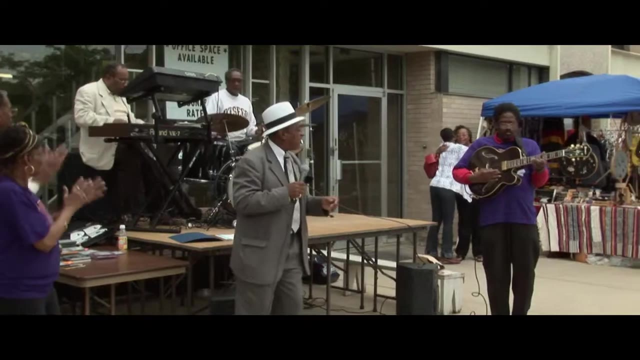 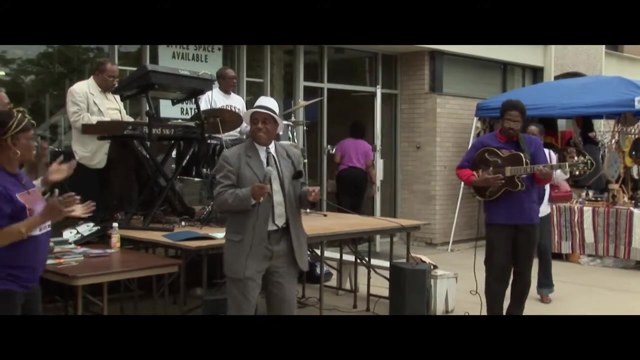 I want you to rock me, little mama, Like you think you got no balls. Yeah, yeah, Rock me baby. Rock me all night long. Yeah, I want you to rock me, little mama, Like you think you got no balls. Yeah, yeah, Okay, come on. 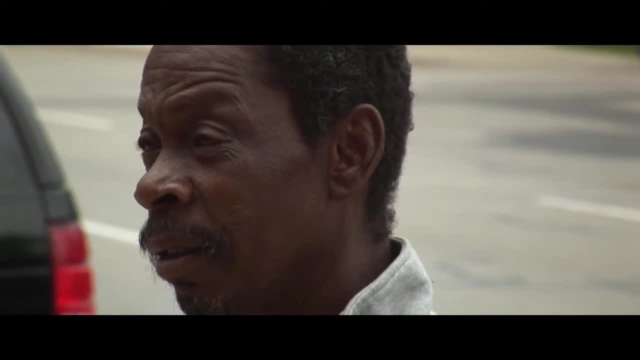 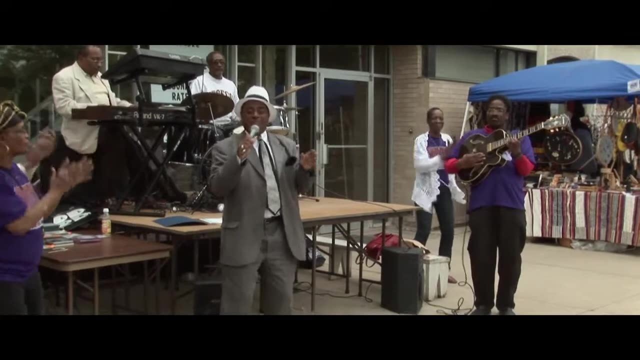 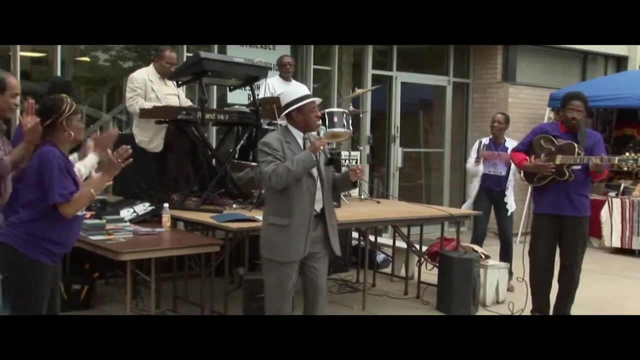 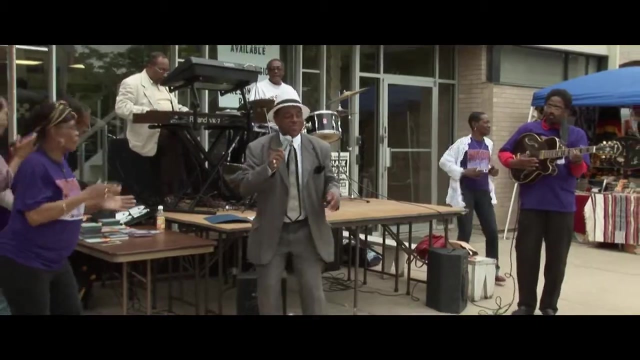 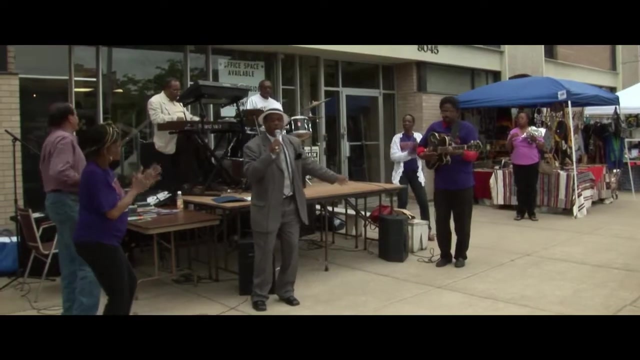 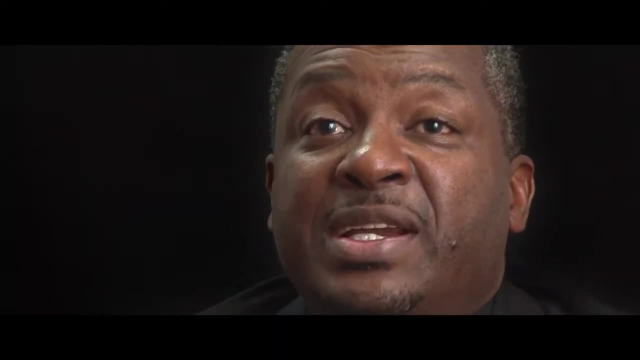 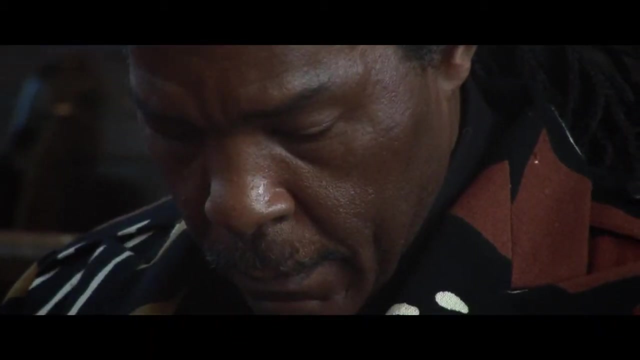 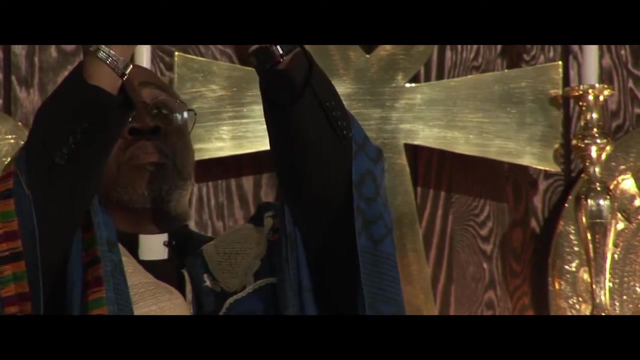 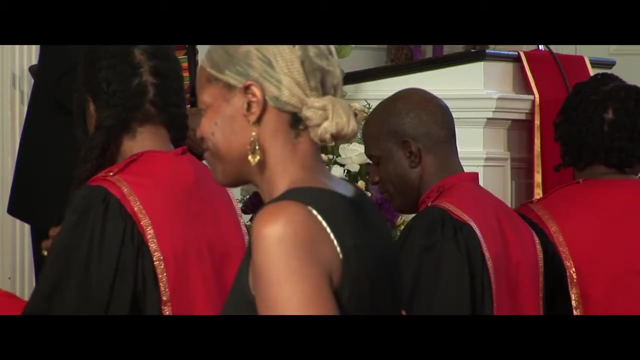 Okay, that does mean spiritual salvation, but it also means a way to live, a career, an education, a way to own a home, a way to raise a family. We believe that the church has to do all that too. Holy communion, Lord, we long to commune with you. 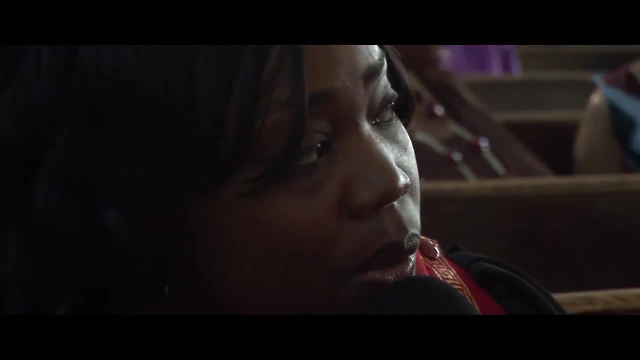 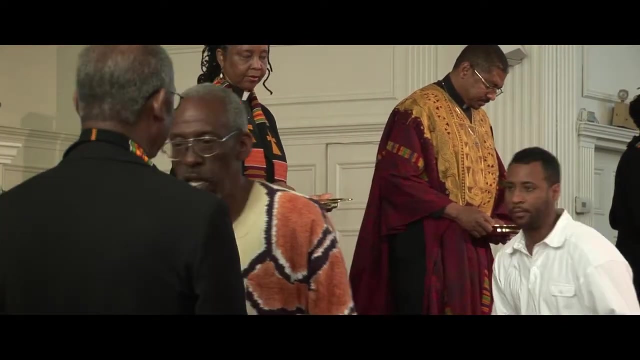 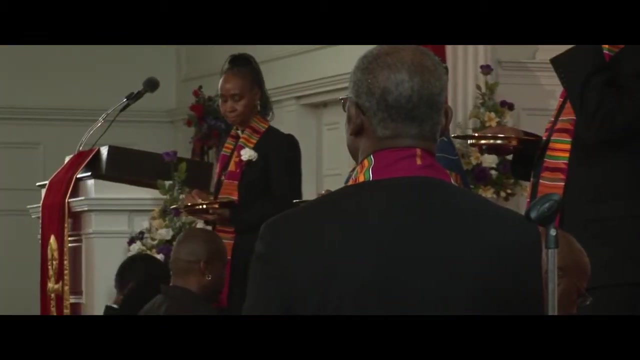 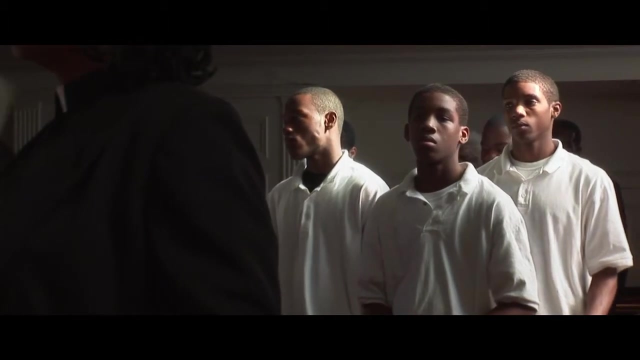 Oh, communion We're thinking of. how do we help people returning from prison who can't find a job anywhere, who have no prospects? How do we help young people get an education? We have scholarship funds that are set up to support people, to keep them in school. 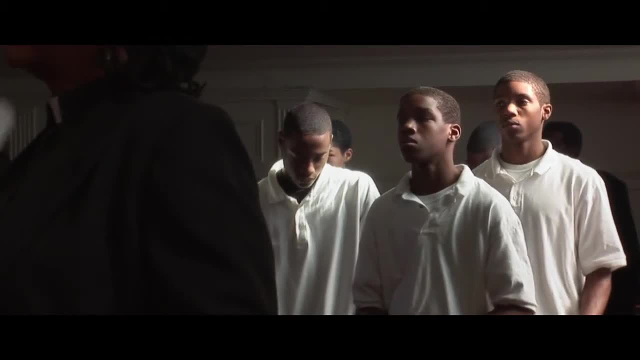 If they can't get money from any other, they can't get money from any other school. They can't get money from any other school If they can't get money from any other school. We have an obligation to make sure that that happens. 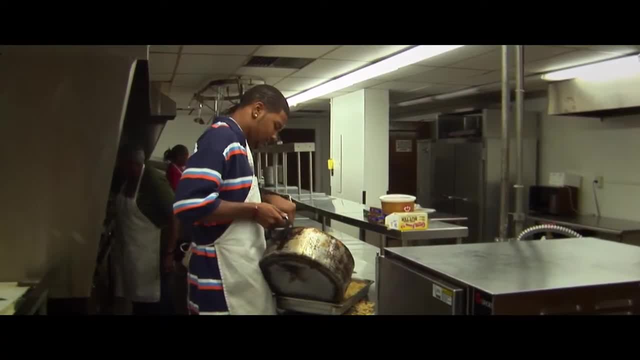 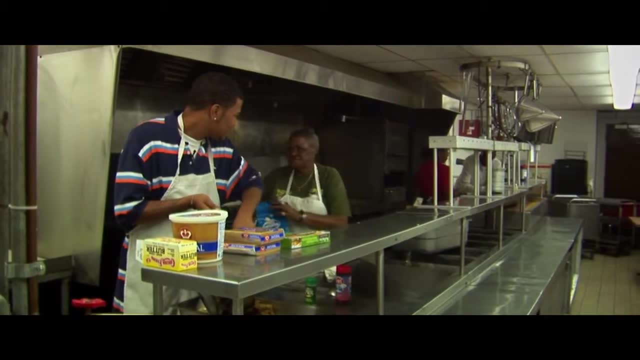 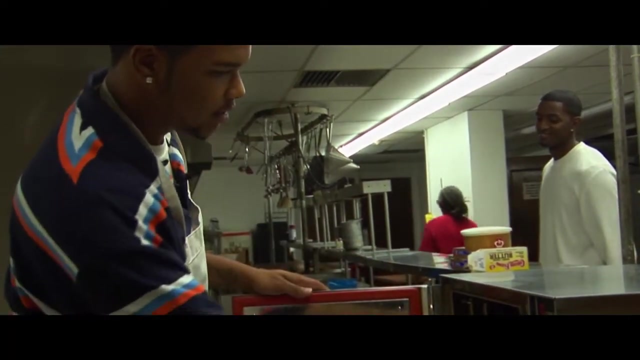 You want me to fill them up? Yes, Okay, We really have built our whole structure around the fact that what we have built is not privately held. It's communally held by the memberships. We don't pay anybody, We don't have employees. 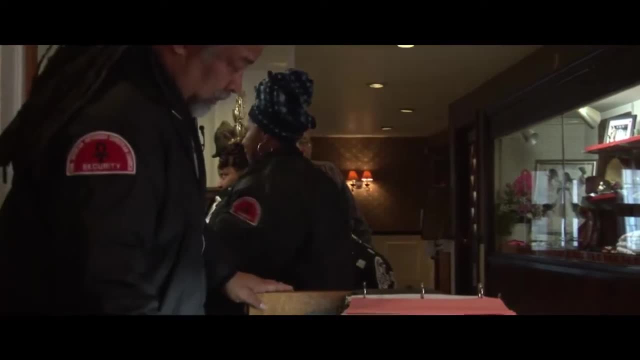 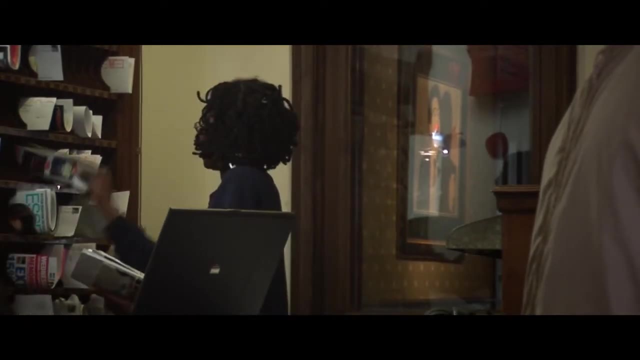 So our interest never becomes. as long as my thing works, I'm going to pay, anybody going to get paid. It all has to work for the whole situation to be viable. That was helpful, Hermione. he goes over there in a couple of hours. 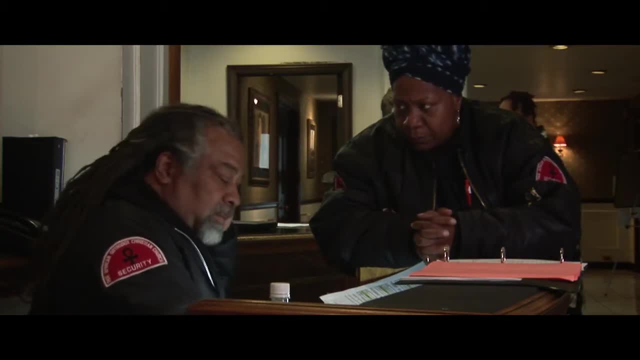 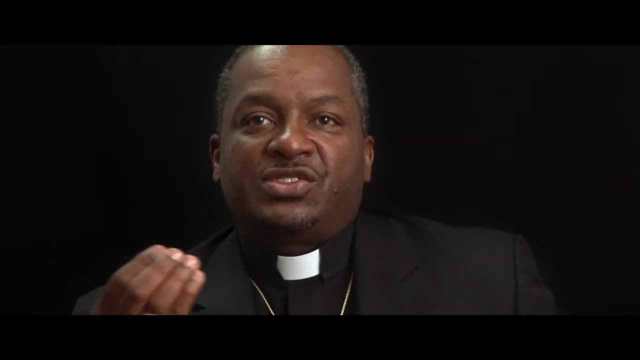 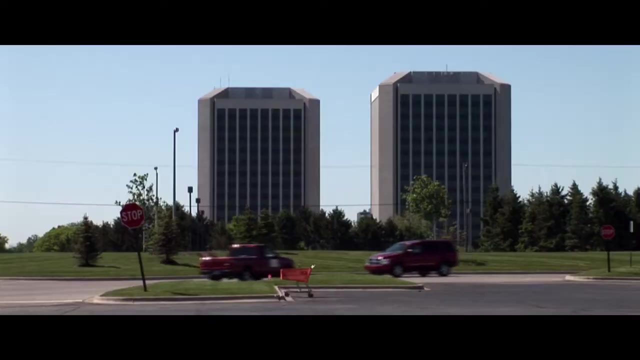 So who's got Sunday your squad? Hermione? yeah, We see institution building as the primary thing that we have to do, because you can't simply change a society. We have no control over what somebody thinks about us, And so we cannot petition people in control of institutions. 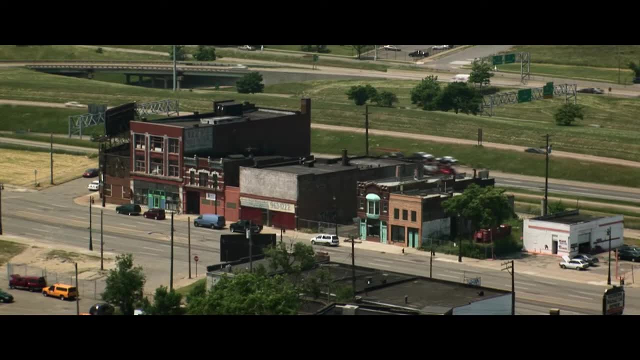 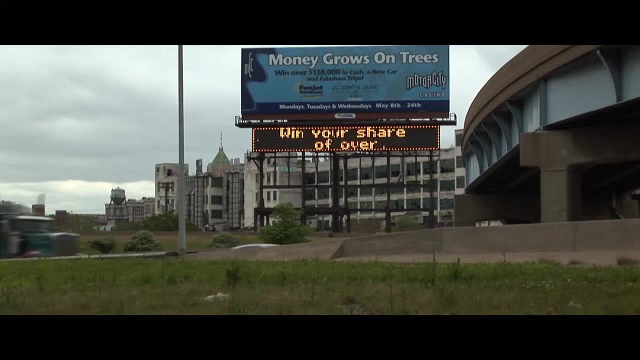 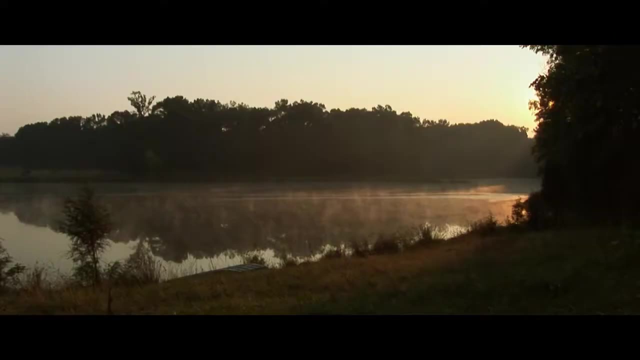 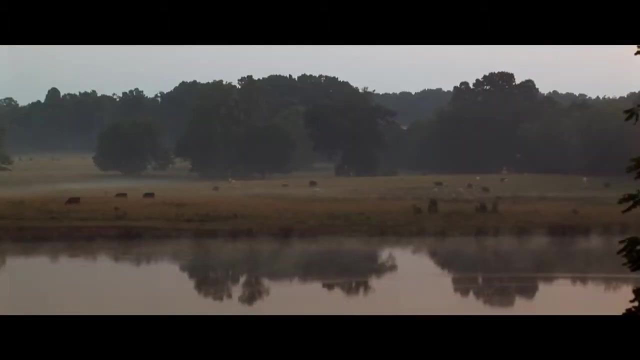 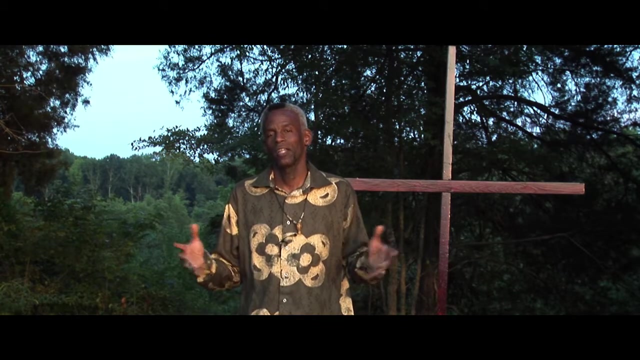 that they have built to treat us differently. Every group of people has a place that they call their home. That place is their promised land on Earth. The story of the promised land in the Bible is really the story of every people and every culture and how they became a part of the land to which they now. 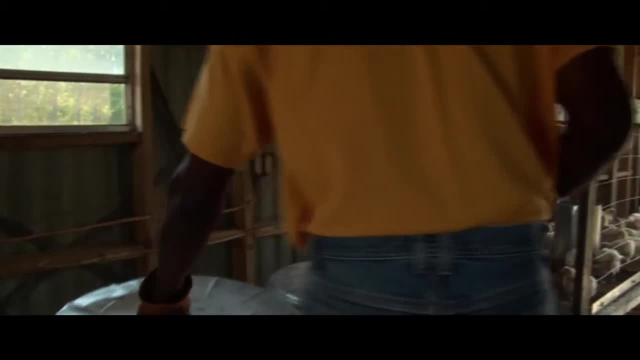 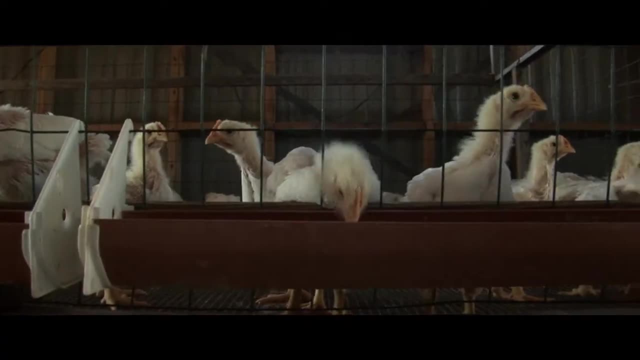 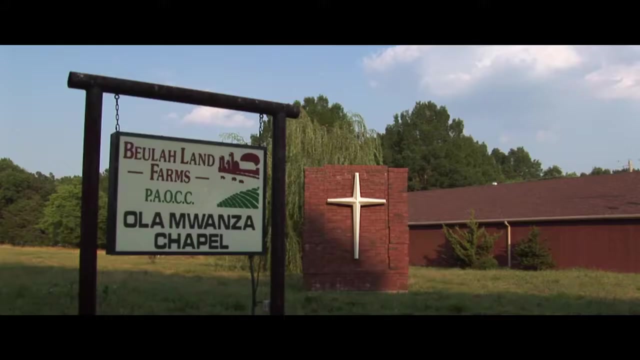 owe their roots, their history, their culture, their origins, And so our founders' vision was that we too would develop a land of our own, a Beulah land, a place where we could live, A place where we could not only provide for ourselves. 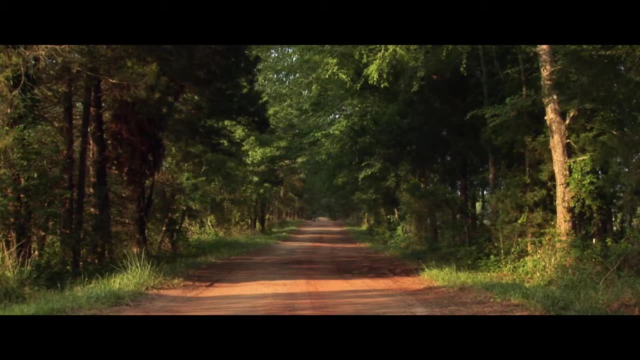 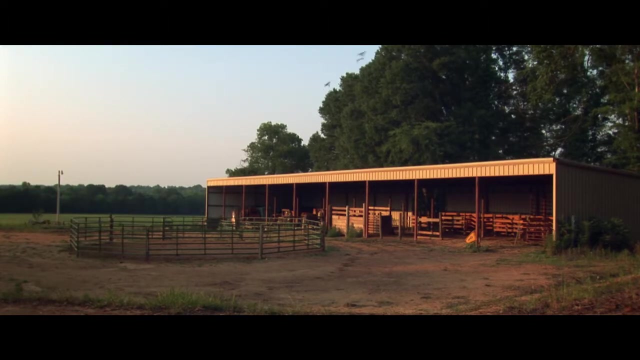 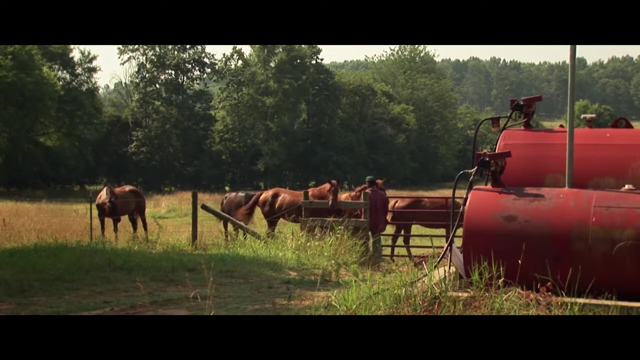 but also become a haven for those who have been disenfranchised from the corruption of city life. We collected quarters for 25 years because all real power has to be rooted in some land, somewhere. That was our founders' last big accomplishment and that is the basis of our future. 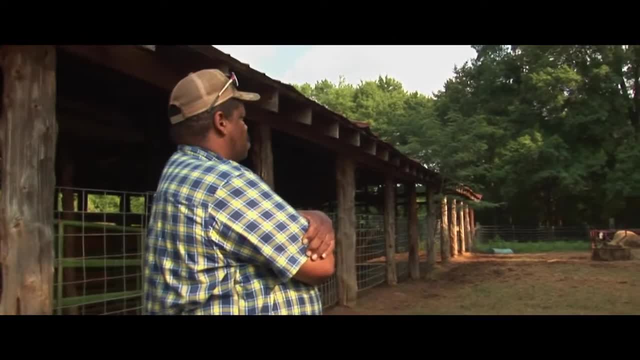 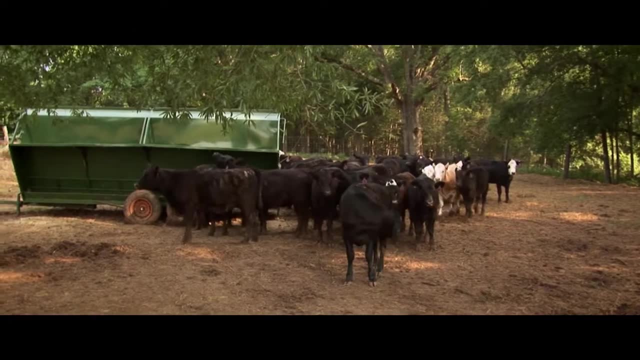 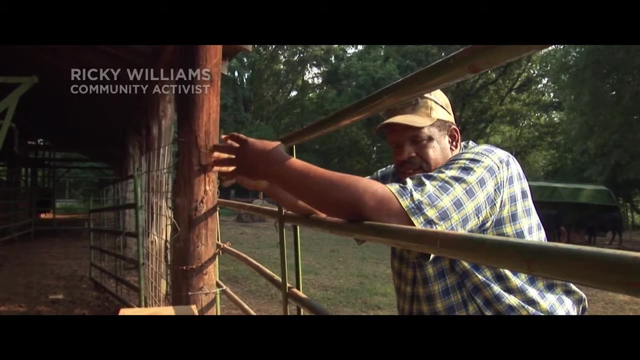 So we're good on hay. We don't think we need to put another bell out. Eventually we want to get up to maybe 1,000 to 1,500 head If we can get all of this working and put together. 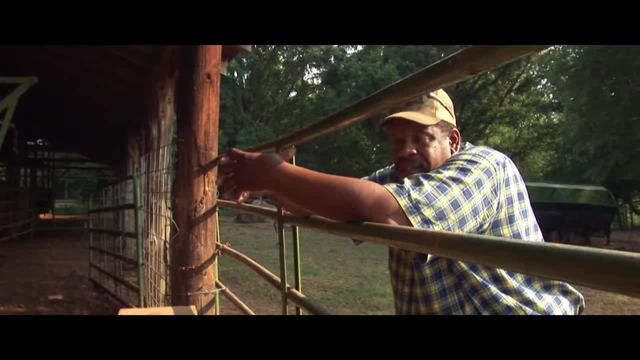 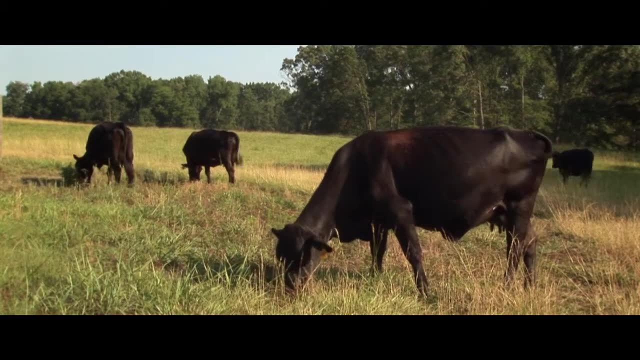 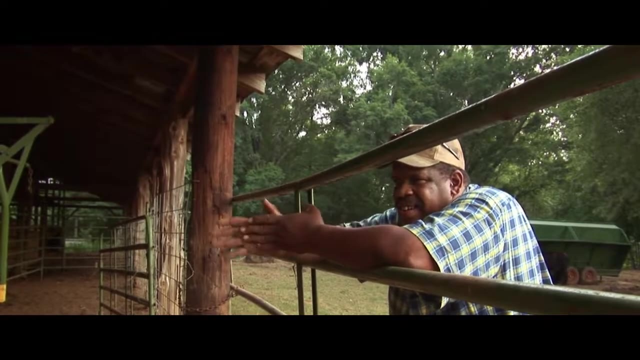 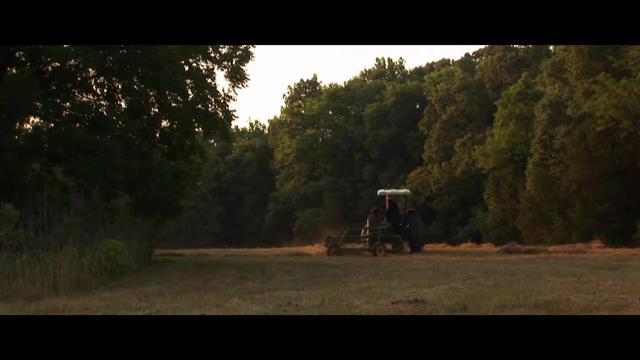 then we'll be at 1,000 head shortly And so far it's been great. I know we got a long ways to go, but it all will work out. The farm is critically important. It's about 3,000 acres of land in rural South Carolina. 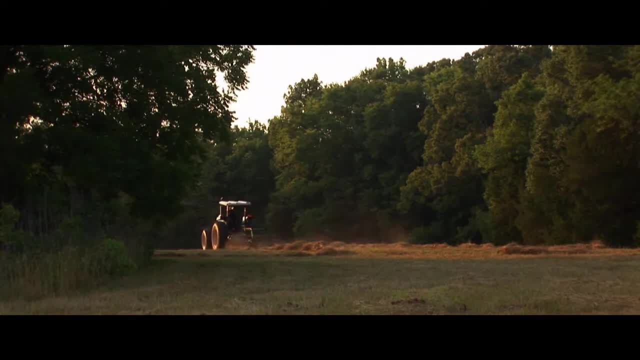 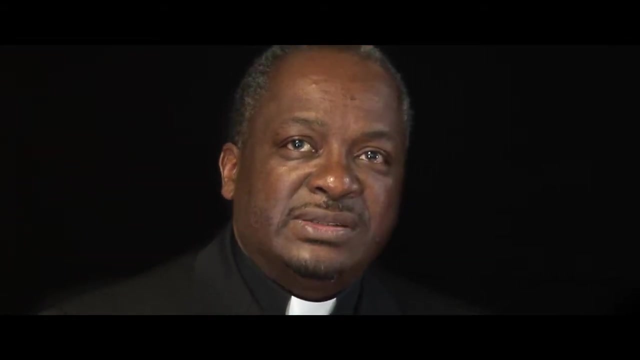 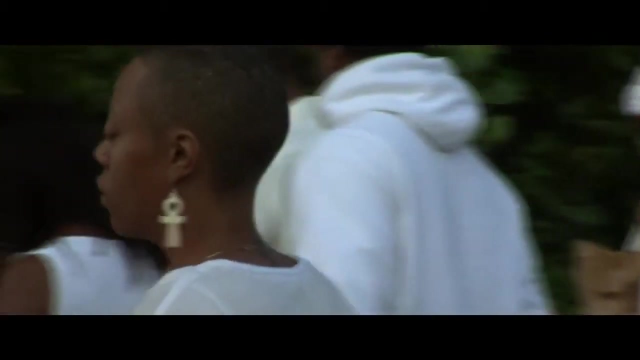 And it offers the opportunity for a number of things. Basically, though, it is an effort to try to create an economic engine that allows us to be able to do what we do without depending on the benevolence of our oppressor. This society teaches us that we're all individuals. 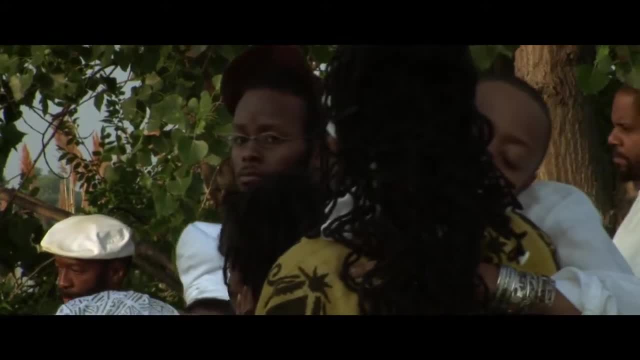 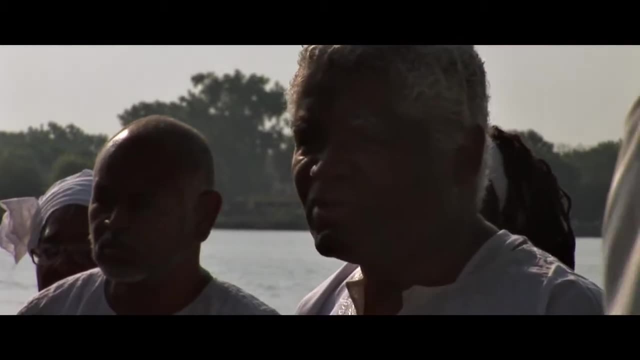 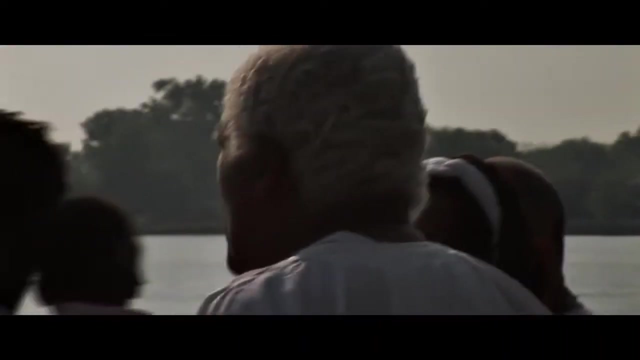 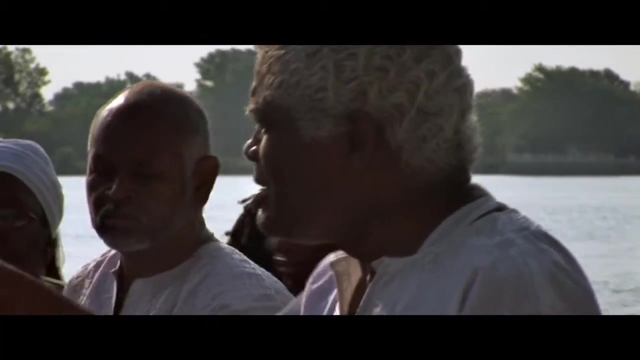 and no connection. But we were born into this world. We're the connection that goes to the beginning of time. We are our ancestors, Our ancestors are us. May the circle be unbroken. Y'all know that song. May the circle be unbroken by and by Lord, by and by. 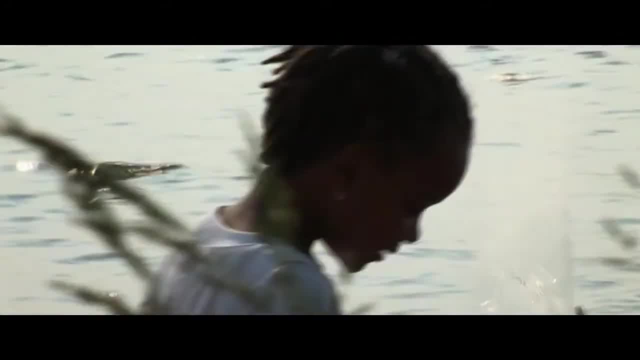 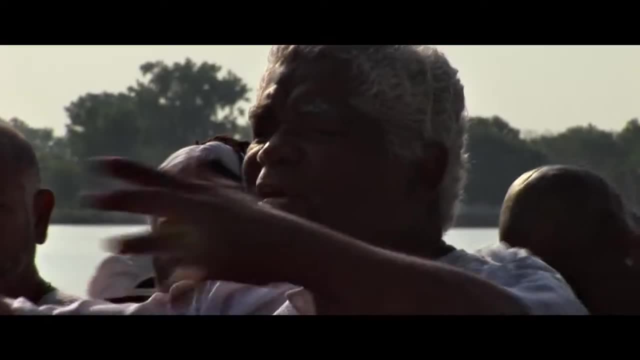 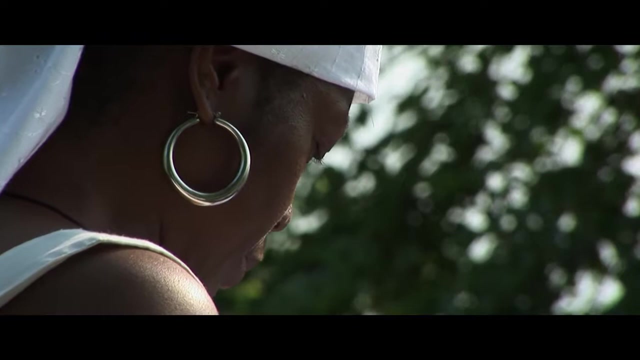 We sang that. We sang that down south And we sang that in some form of that in the motherland, Because it means that we're all a part of a process. I am because we are. Can we say that I am because we are? 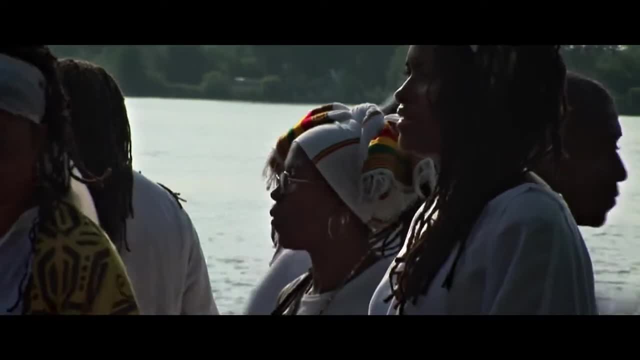 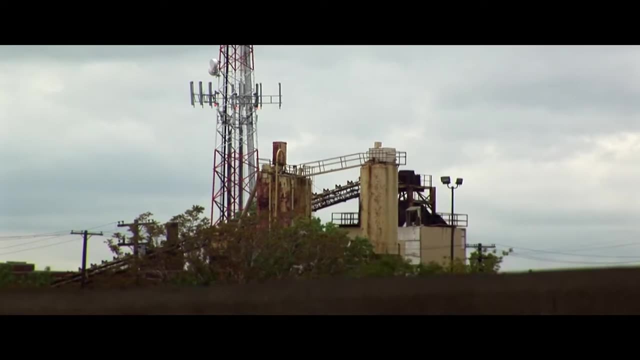 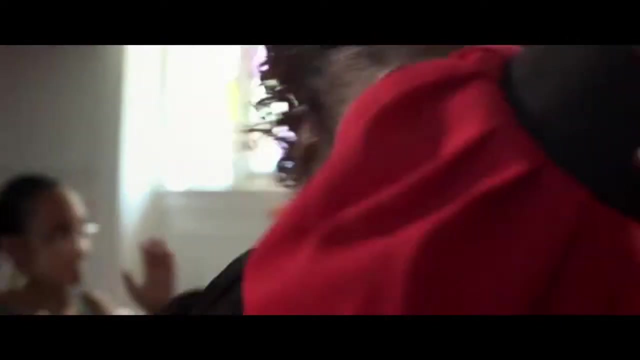 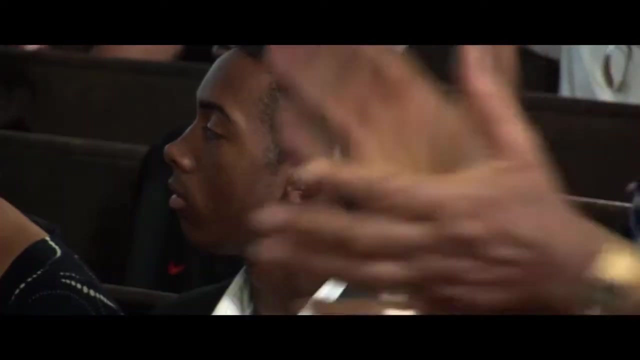 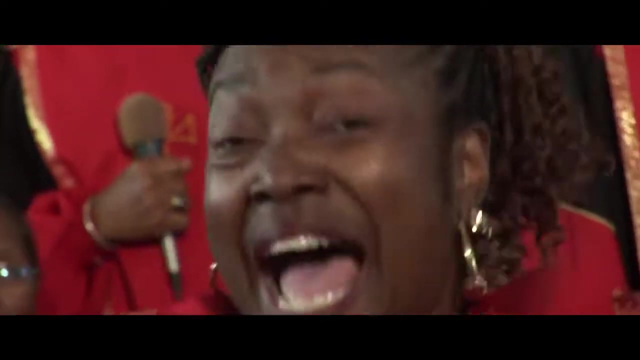 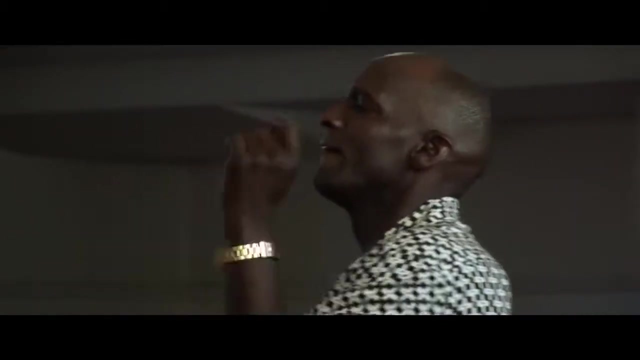 Let's say it: I am because we are. Your body does not last. Life flows on its own, Yeah, So Let's sing and laugh. Let's sing out our song to God: Yeah, Yeah, Yeah, Let's sing and laugh. 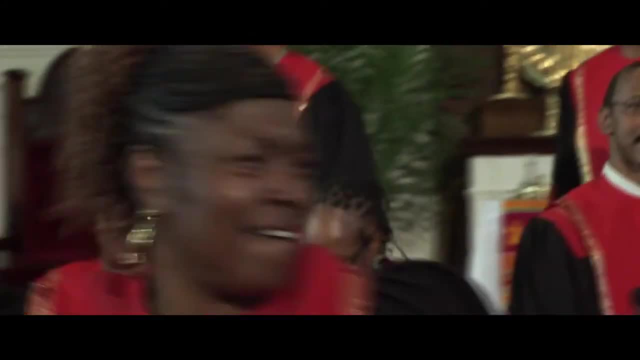 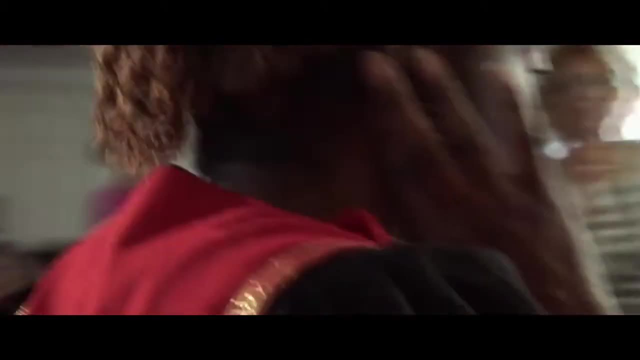 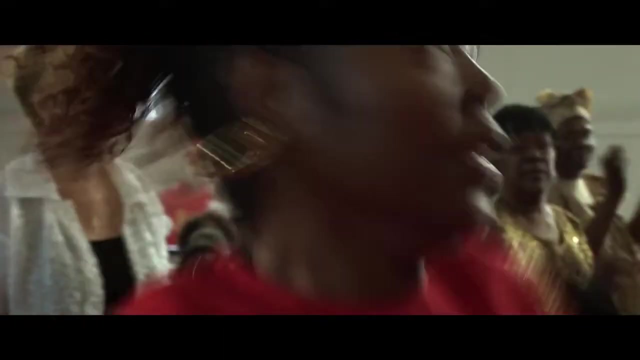 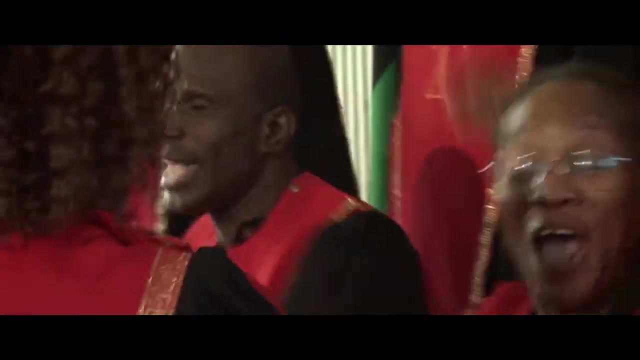 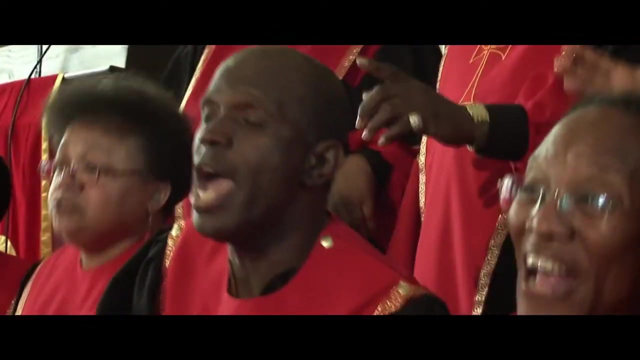 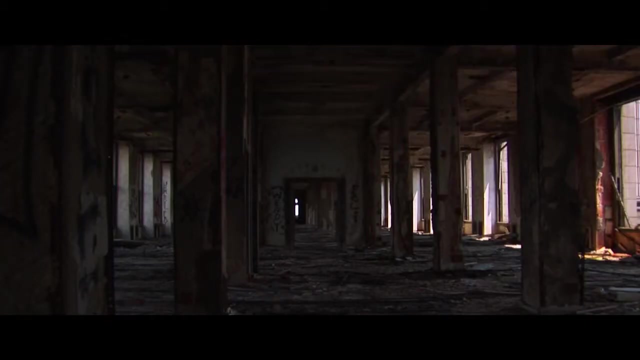 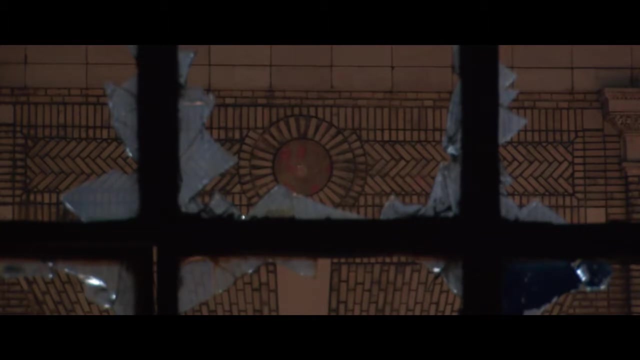 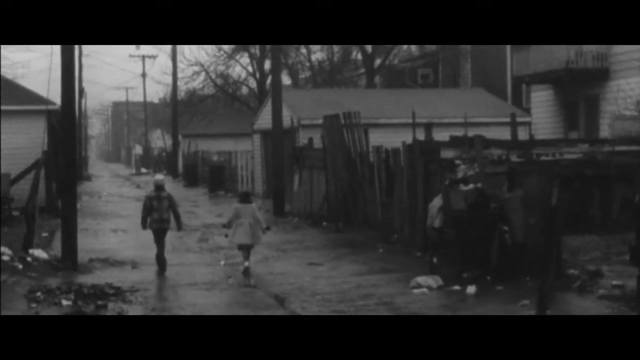 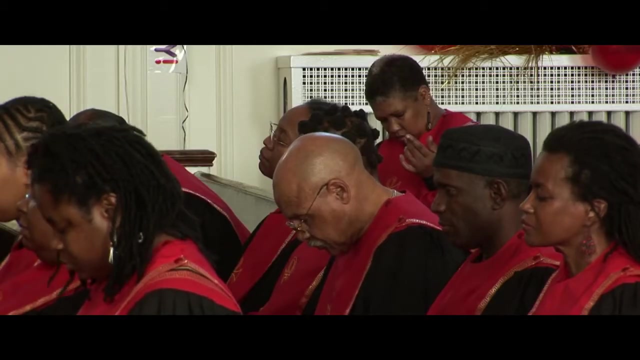 Yeah, ¶¶, ¶¶, ¶¶. We know, Lord, that our journey is not complete, because our work is not yet done. Lord, you know the pain and suffering black people have been forced to endure over the centuries. ¶¶, And time and again, you have extended your mighty hand. 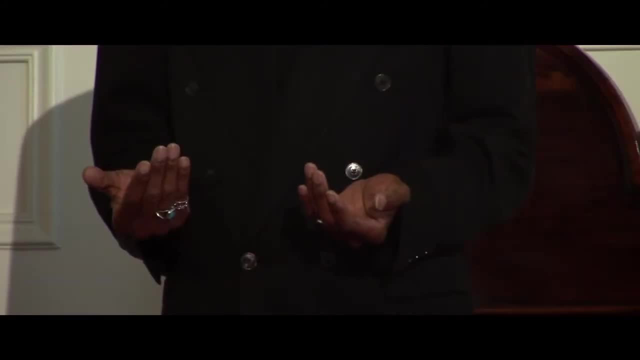 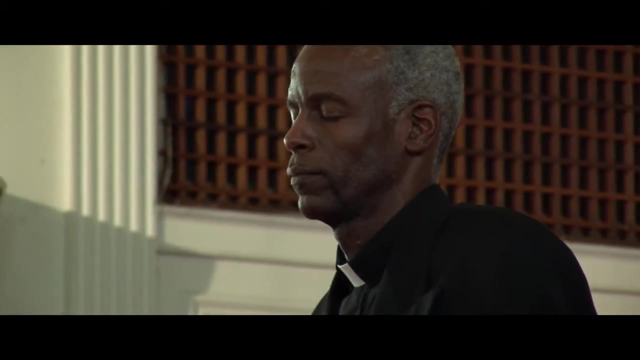 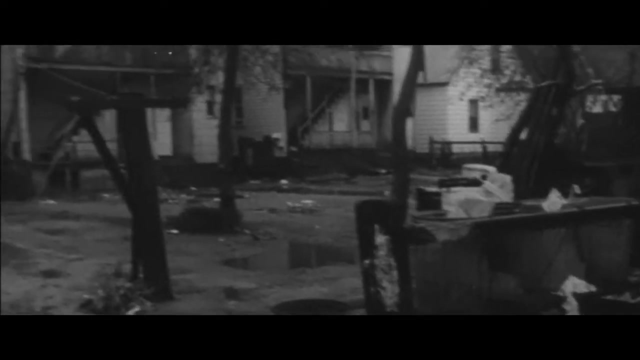 on behalf of your people. Help us, Lord, to focus on our mission, to fully dedicate ourselves to building your kingdom here on earth. Help us, O Lord, to always remember that what we do to the least of us, we have also done to you. 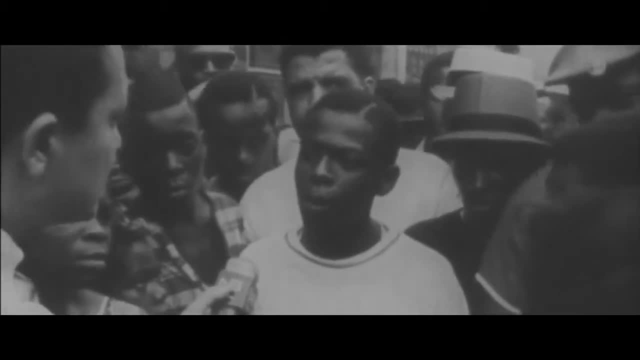 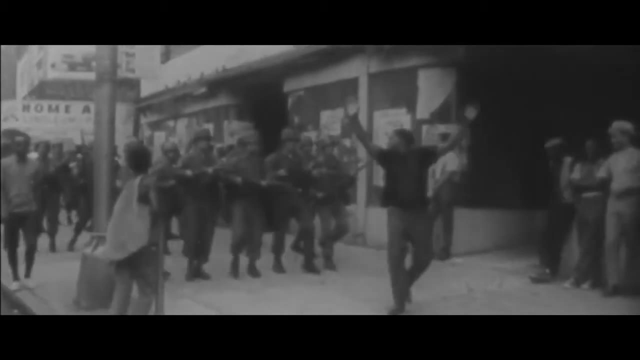 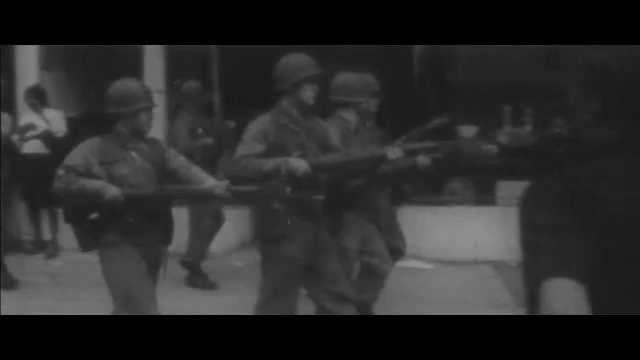 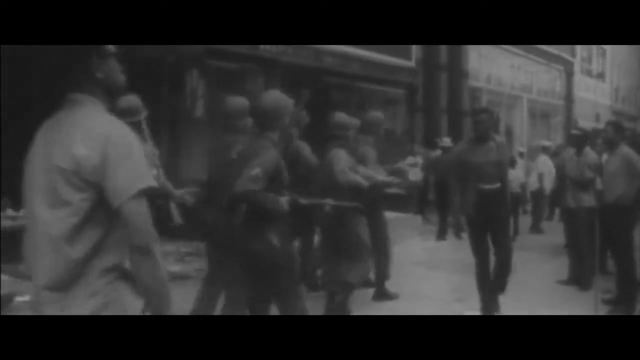 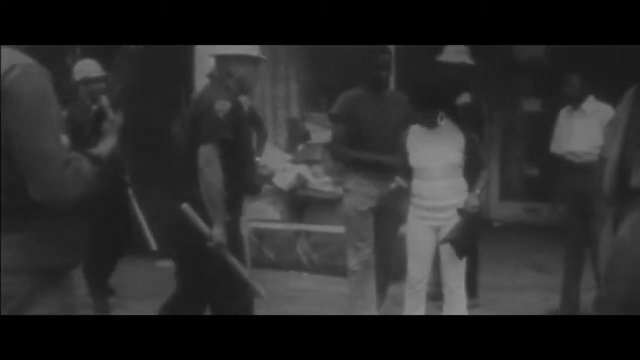 ¶¶ Tell them now: we ain't taking no more from nobody. They been taking everything we had and we ain't fading them no more. ¶¶ ¶. Hear our prayer, O Lord. ¶¶ ¶. Hear our prayer, O Lord. 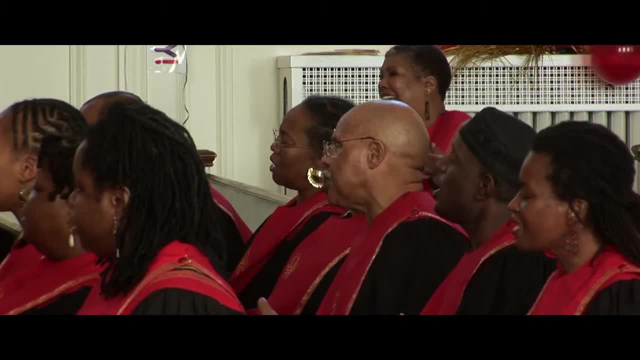 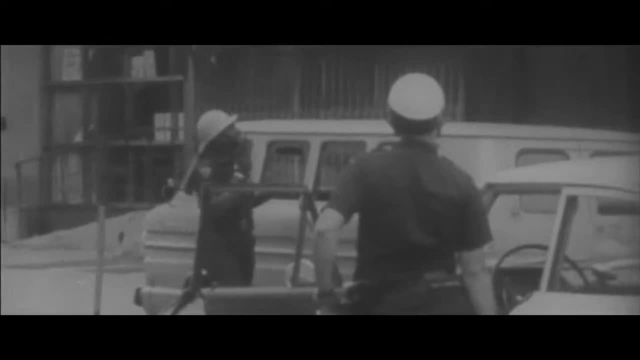 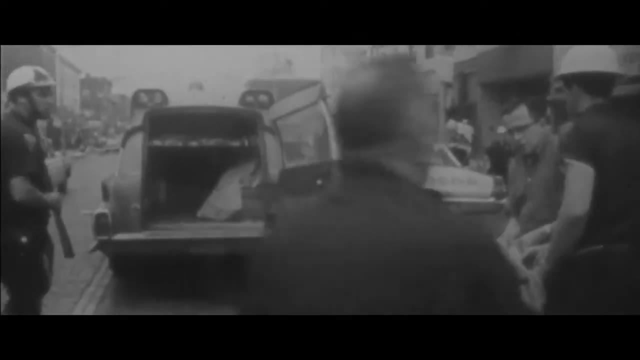 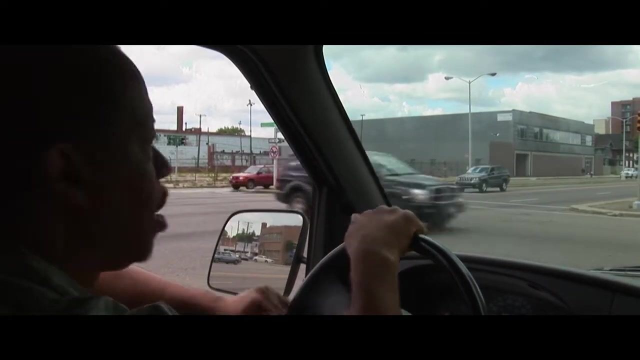 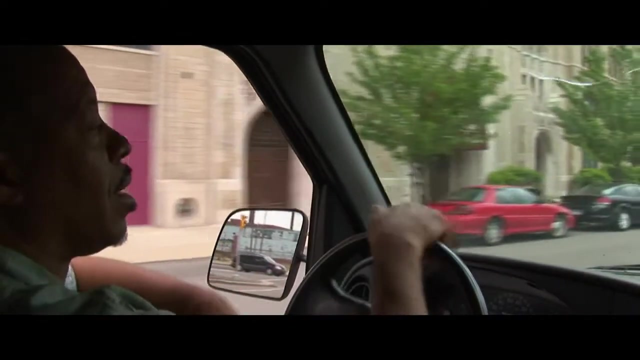 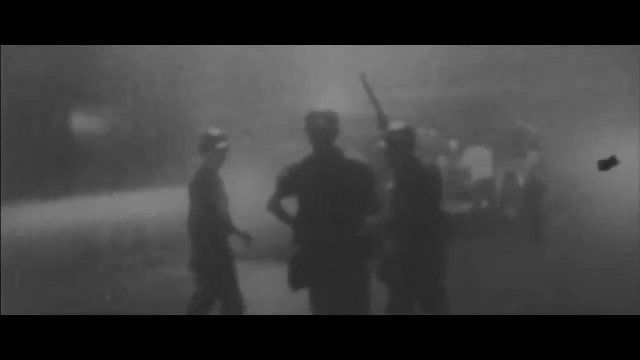 ¶¶ ¶, Invite thy ear to us ¶¶ ¶, And plant us like trees ¶¶. This is the street where the Detroit riots started. Um the 67th riot ¶¶. After every rebellion, what is it that the United States calls for? 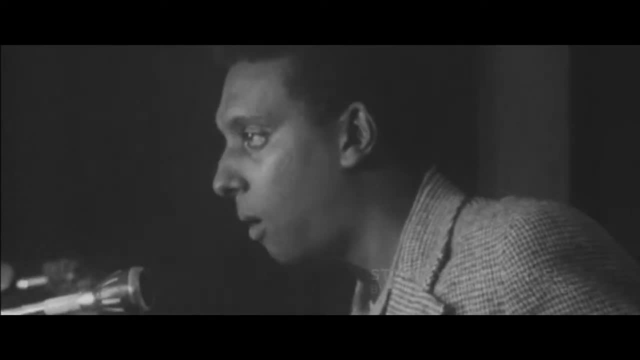 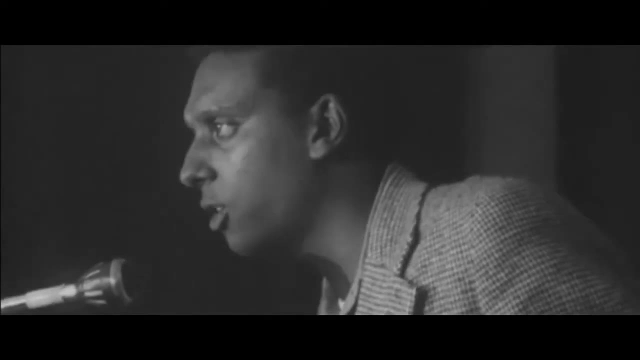 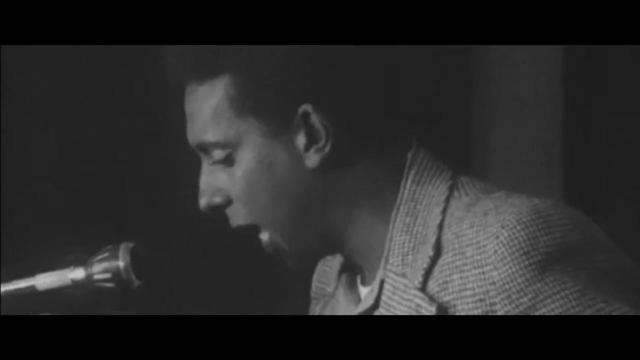 Law and order. All the time, the first thing they say: ¶¶, ¶¶, ¶¶, ¶¶, ¶¶, ¶¶, ¶¶, ¶¶, ¶¶, ¶¶, ¶¶, ¶¶, ¶¶. I am not concerned with law and order, I am concerned with justice. 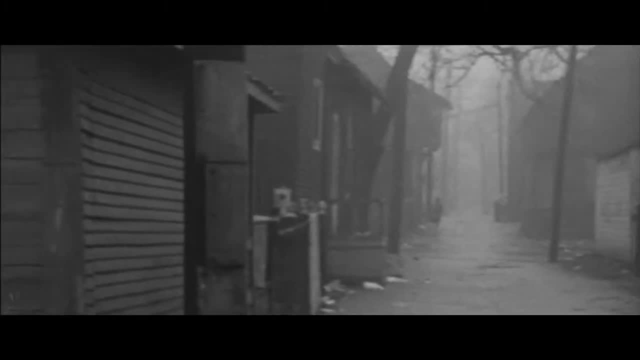 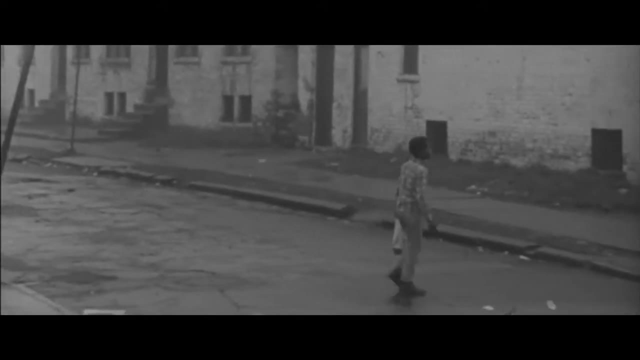 The whole process of black men in America has been the process of fighting off dehumanization. The dehumanization process didn't end with slavery. It kept right on going, Even in the 60s, when we gained a little dignity. we got loud and rebellious and confident. 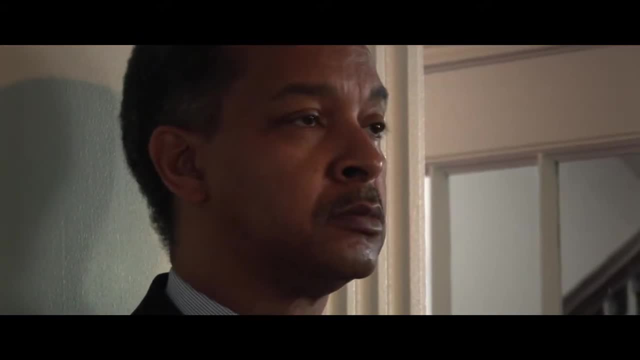 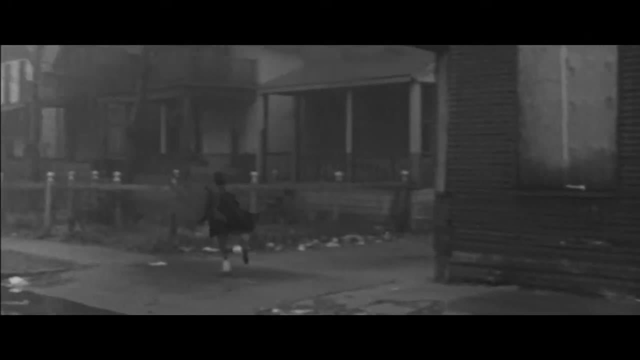 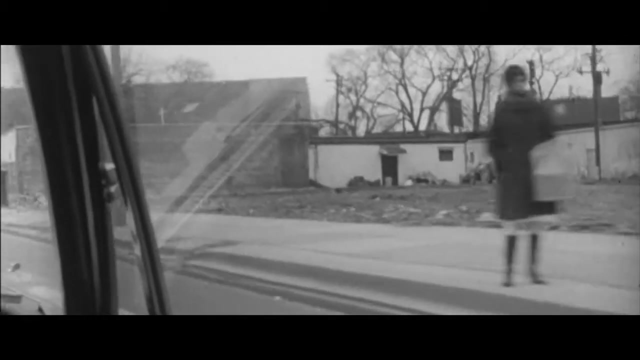 We had no idea the extent that the powers that be would go to to put us back in our place and snuff out our dignity and manhood. We had no idea A whole lot of land that you see that appears to be vacant, vacant lots. 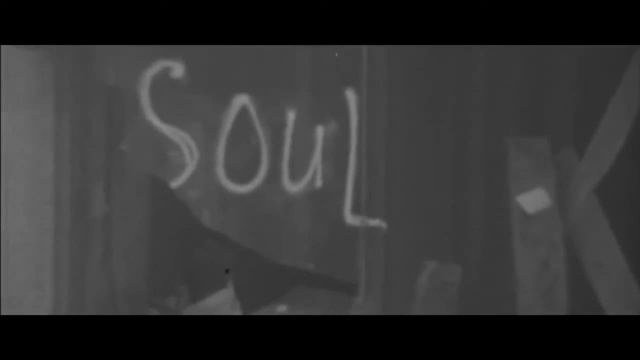 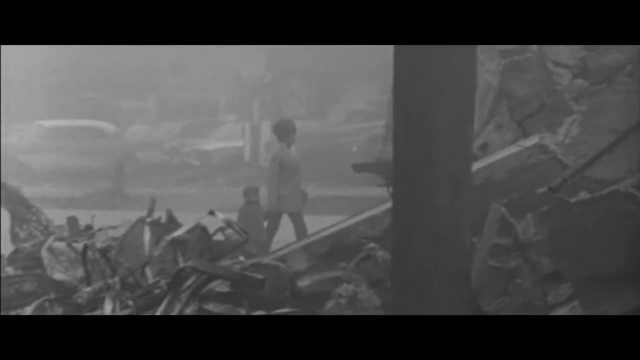 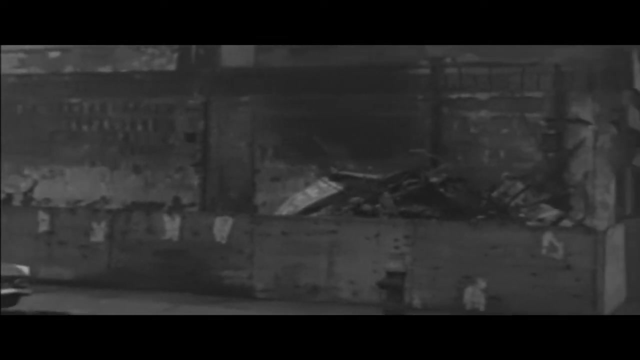 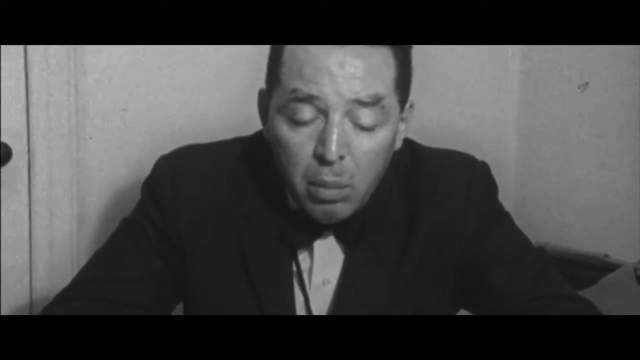 the remains, the remains of what was left, which wasn't too much. People were very happy. People felt that what they did wasn't very necessary. The rebellions, I think, were essentially the feeling of black people that the day of oppression was over. 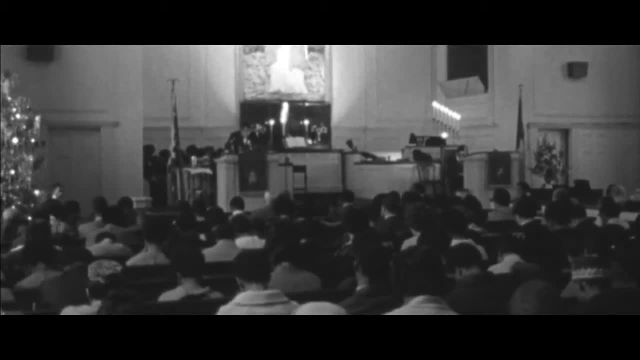 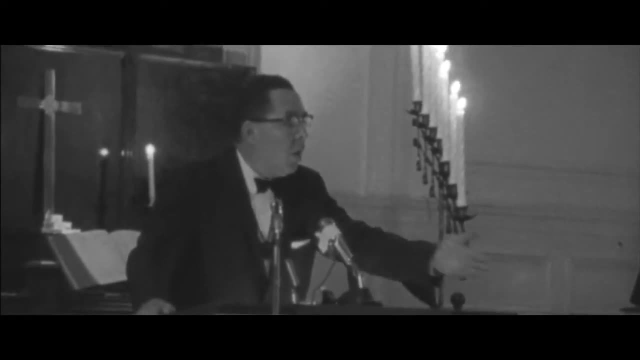 I know some of you- you know even folks in the nation here- feel a little irked sometimes because we have security measures in effect on Sunday and any time else that we ever meet. Well, why do you have to do all that? 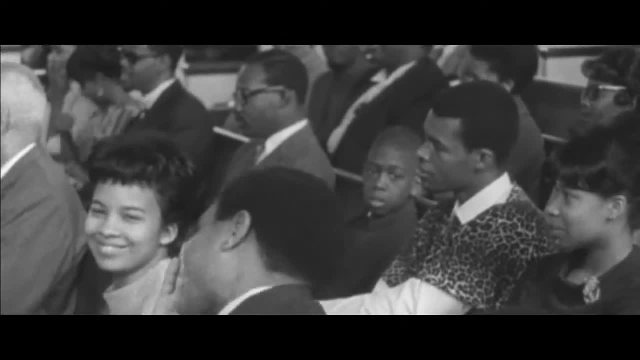 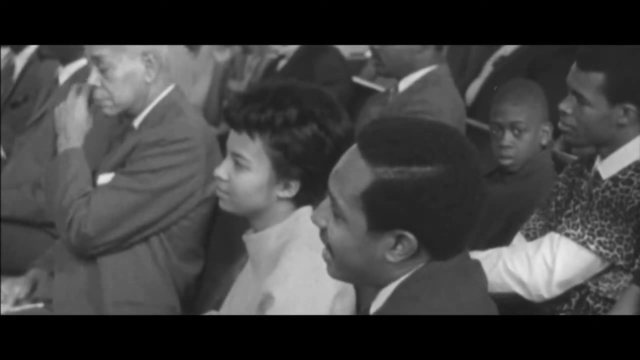 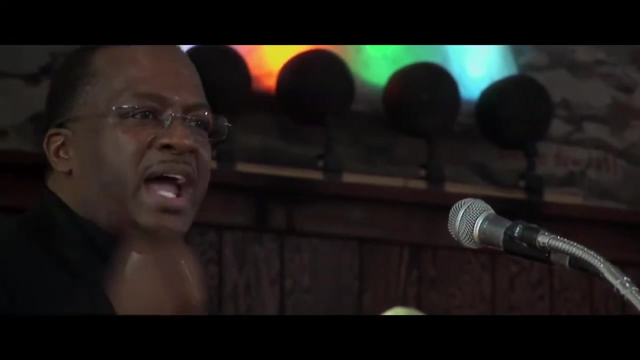 Because there are crazy white people in this world. That's why we have to do it. We had on berets and leather jackets and we were talking loud and proud and studying books and walking around talking about what we were going to do, but we had no idea that we were threatening. 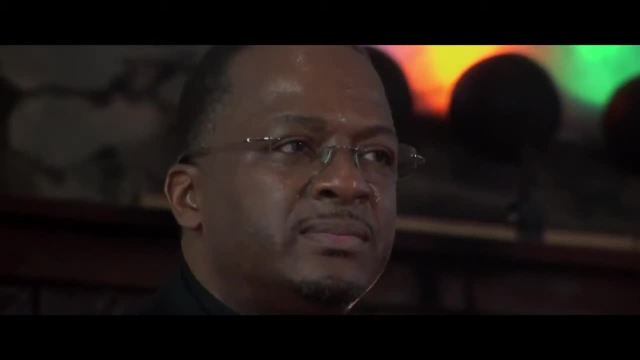 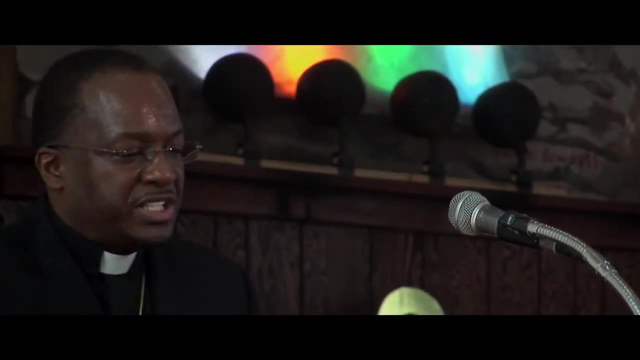 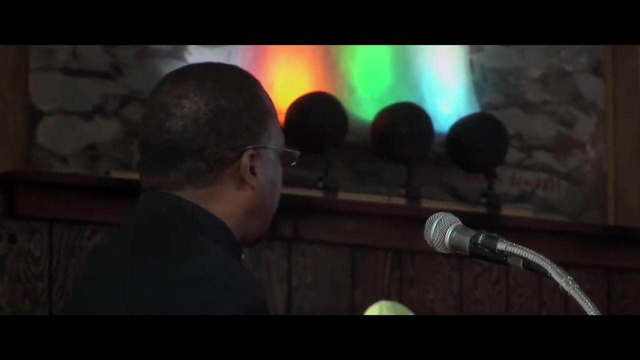 the very foundations upon which everything had been built, And so the bold, new, dangerous, revolutionary black men had to be destroyed. They had to be destroyed, had to be Used to be. our role models were Martin Luther King and Malcolm X and Marcus Garvey. 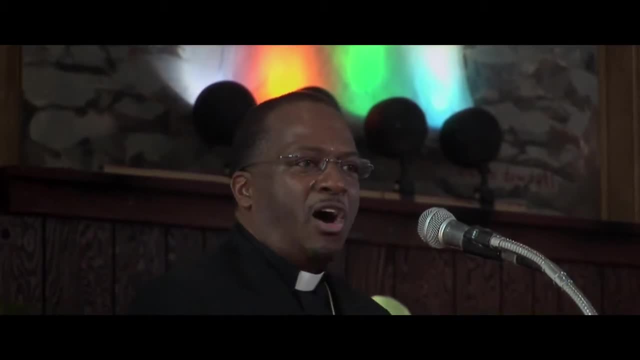 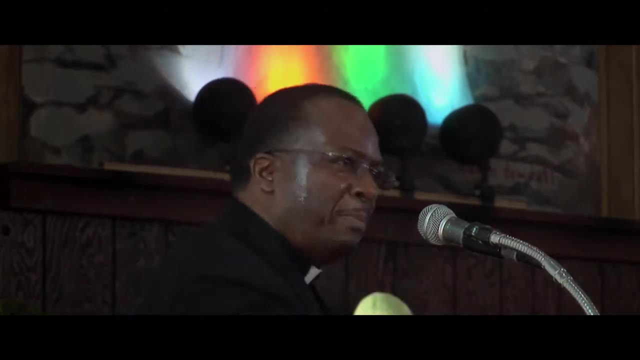 and now? our role models are pimps and hustlers and ballplayers and preachers. Our role models are gangster rappers. Our roles- the things we want to be- are not worth being. They lies, they phonies, they cliques. 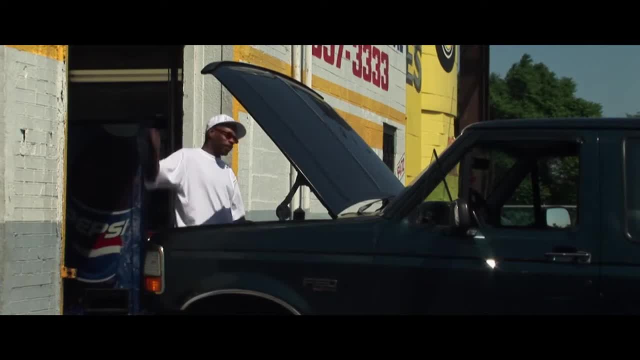 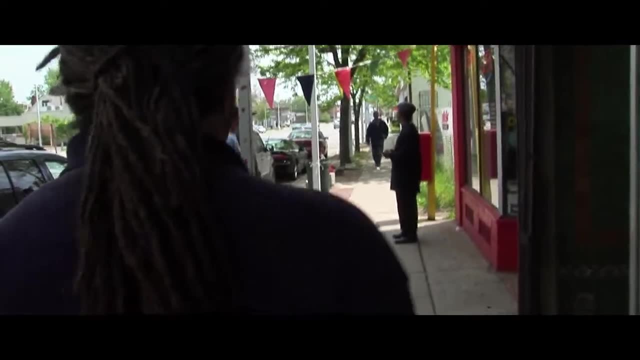 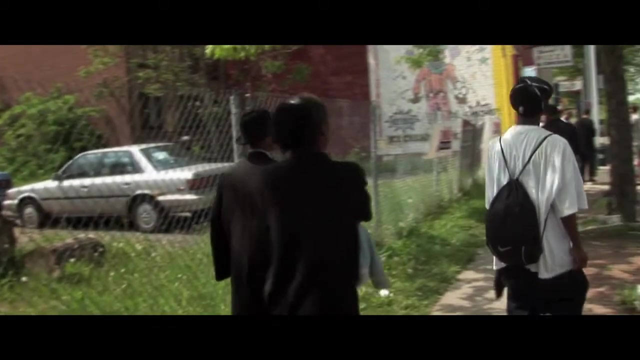 These niggas ain't never sold away And I'm the god fucking villain. They lies, they phonies, they cliques. These niggas ain't never sold away. Oh, let me get on. I call it the ghetto Negro success. 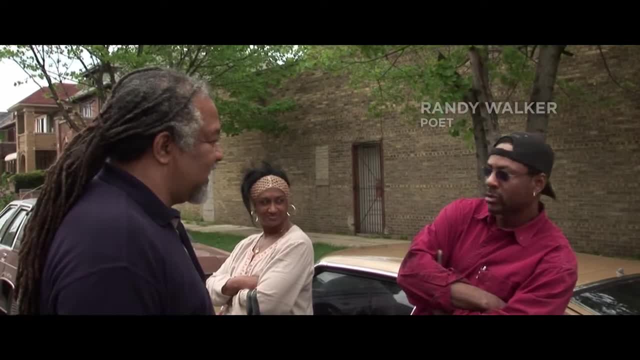 The gators. get some fur, get some jewelry. that's as far as we want to go. Get a caddy with some wheels on it, with a clown. that's it, man, We done arrived right, We sure did. 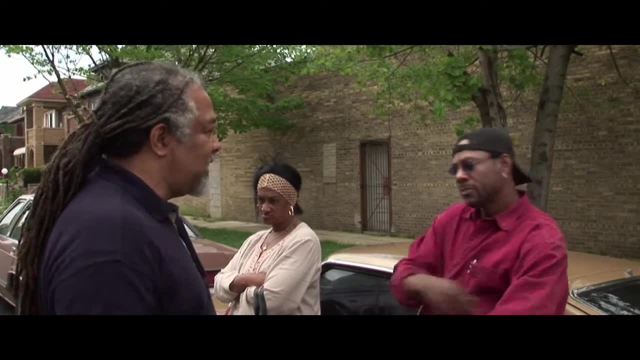 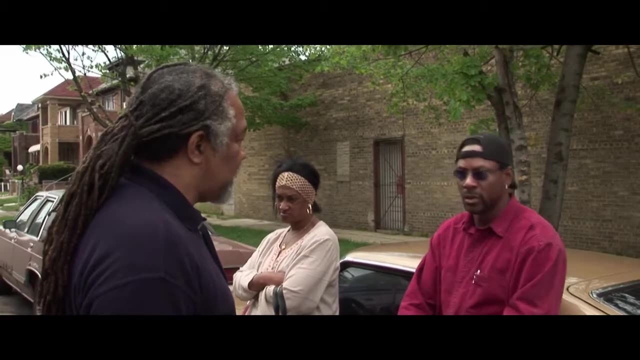 It ain't about that. you know, It's on the street. everybody made it. That police system goes back and it started forming back in the day Sixties and seventies. Superfly started propelling it. you know because before the movies came out, man. 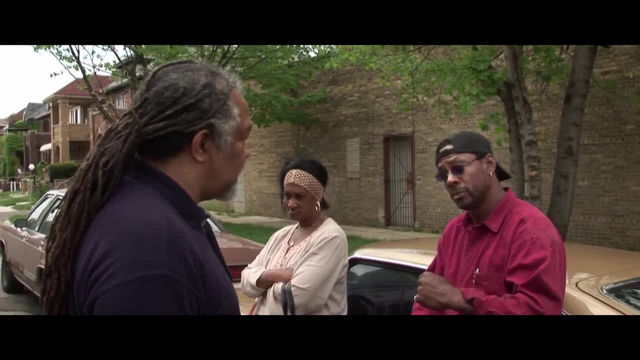 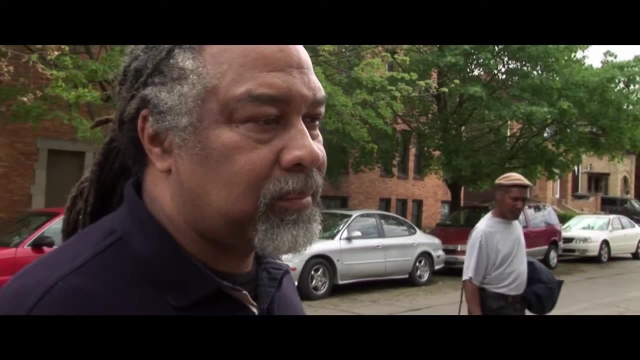 you know we was like this here. We had a purpose, We had a common bond. The Afro meant something, This meant something. It's real easy to you know redefine people if people don't know who they are. You know. 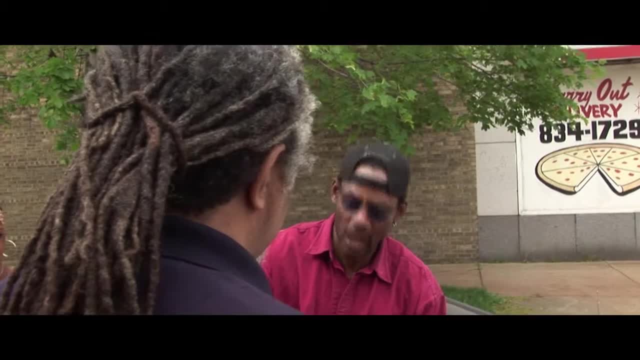 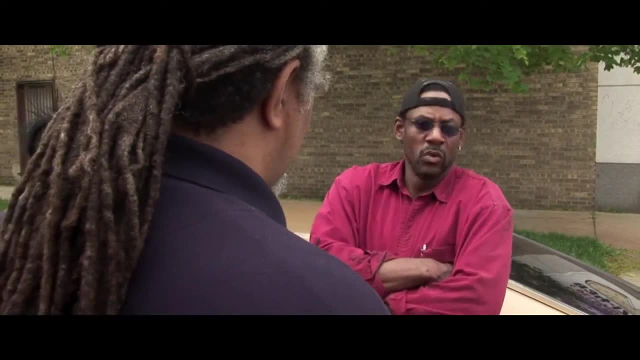 And the only collective identity that we have, you know, is slavery. Yeah, You know, And the civil rights struggle, But most people trying to deny that. Yeah, And we don't want to talk about that. Yeah, And everybody talk about the Jewish Holocaust. 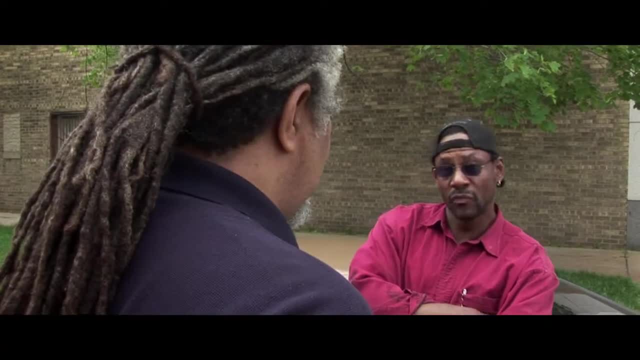 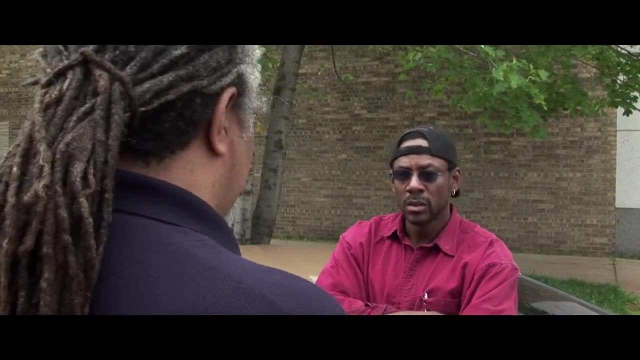 Yeah, What about this one? You know we lost five times as many people. Yeah, At the end of that thing, they knew who they were. They went through counseling. Yeah, They got reimbursed for the money they lost. They still knew they were Jews. 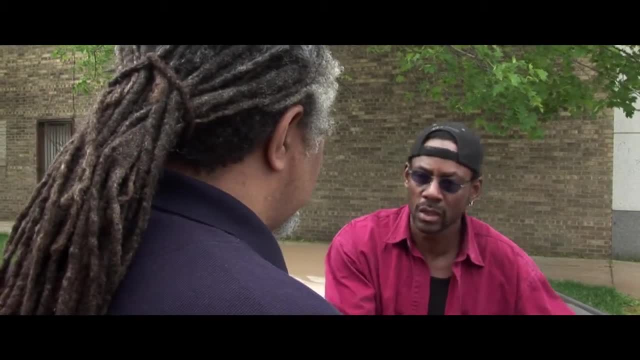 Yeah, They still knew their history. Yeah, They still got their language. We didn't have nothing but what the white folks gave us. Yeah, And I don't care how much people argue this, We ain't all the same Okay. 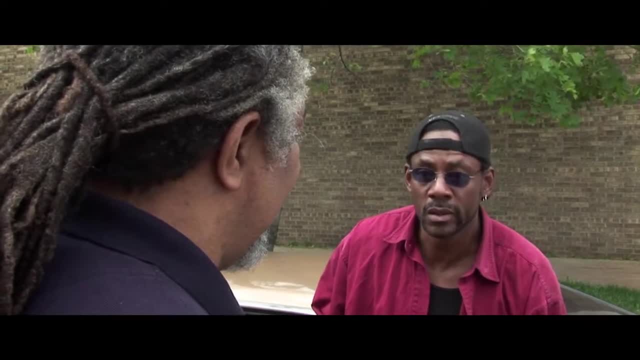 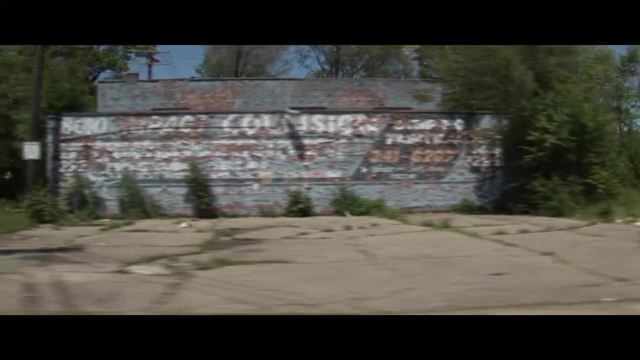 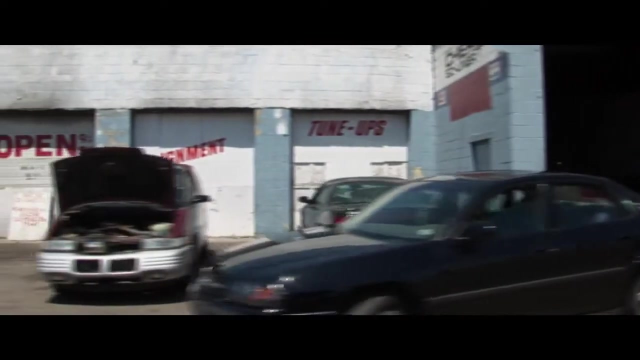 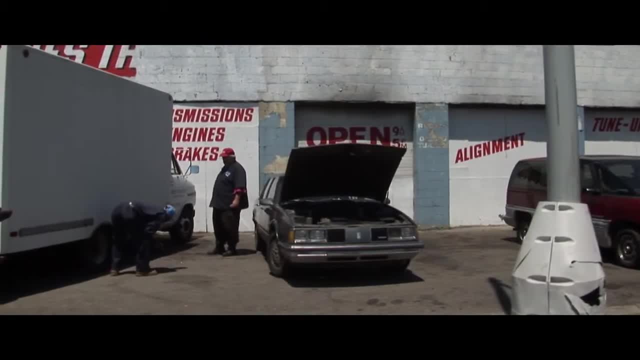 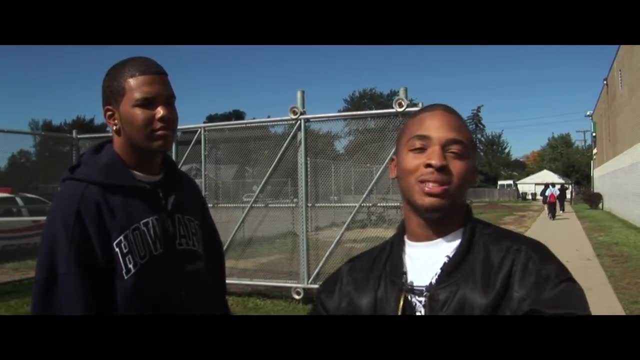 Yeah, Yeah, I know, Yeah, Yeah, Yeah. First book: I peeled When I was about 16, picked up my first book. it was a book on pimps out of Pym Women. I mean, that's all. 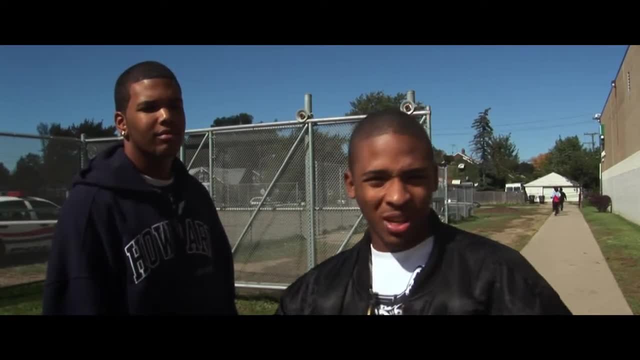 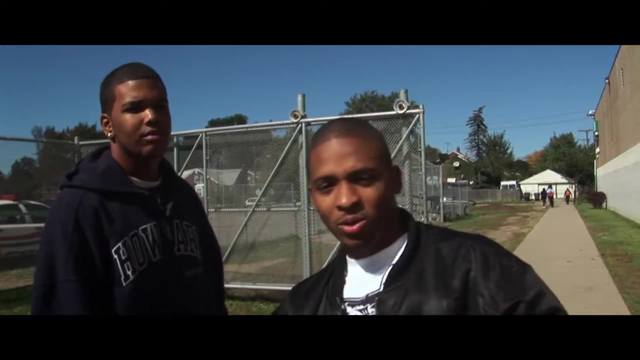 that's what I was trying to be Like. I said that's what I was trying to emulate. That's the only idol I've seen, because he was the one in the neighborhood that was popular with the gold chain and all the women and stuff. 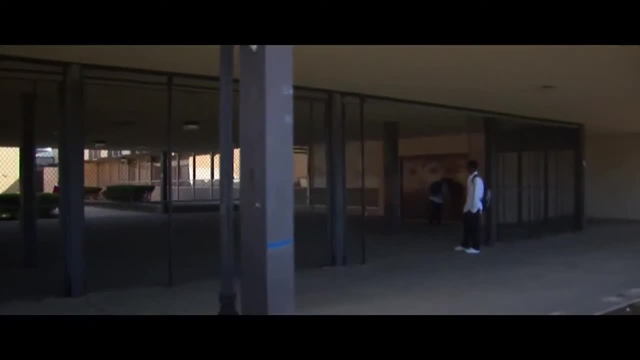 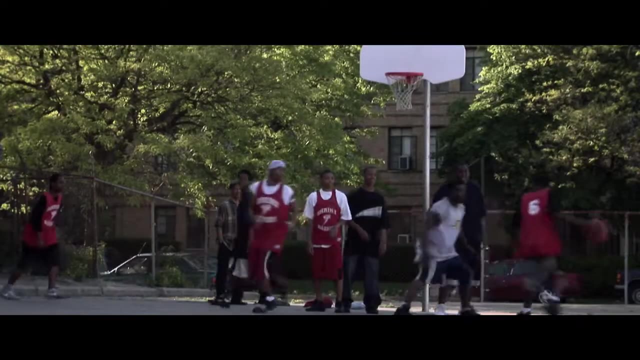 And then my cousin. he see me read and he finally put me s to the side and he said: hey, I've got a book on Africa. You wanna check out my little bank? Sure out, and just read this. And I read it. I mean, tears nearly came to my eyes. I want to learn. 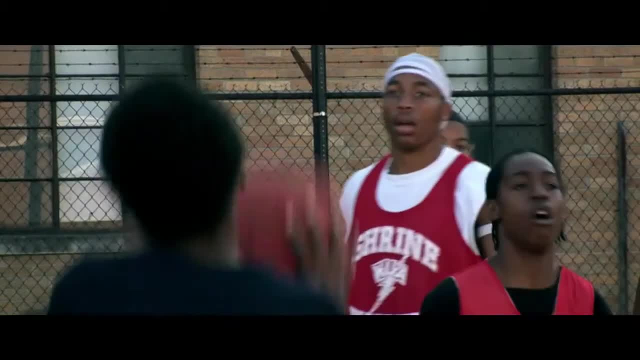 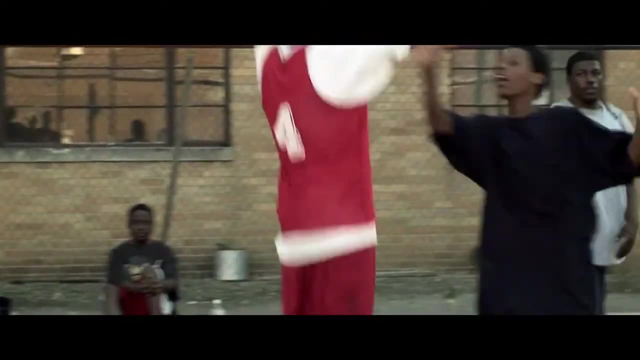 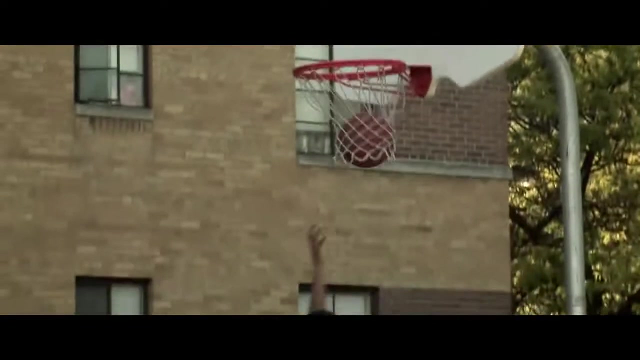 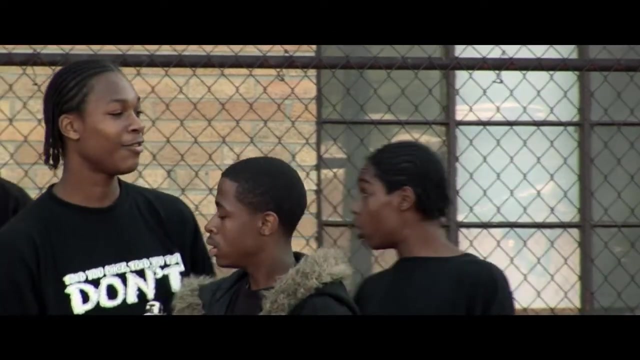 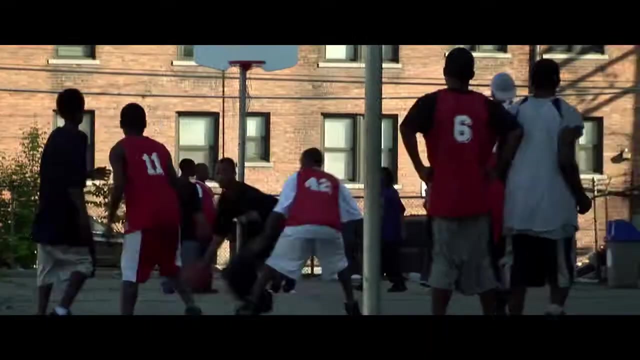 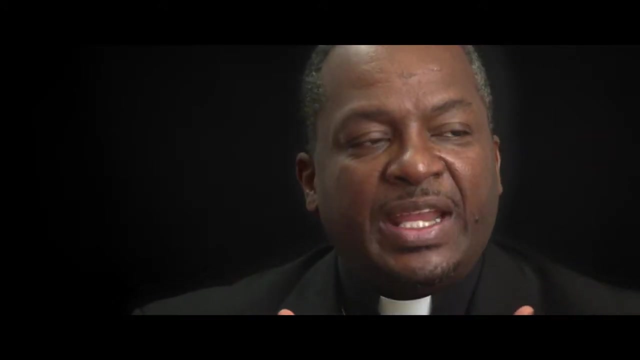 about my people. Orlando Patterson is a sociologist with Harvard University And his view is that black men are being destroyed by culture. It's a cultural thing, And he says the reason for their destruction is because it's kinda like the stereotype is created and it becomes, uh, empowering. 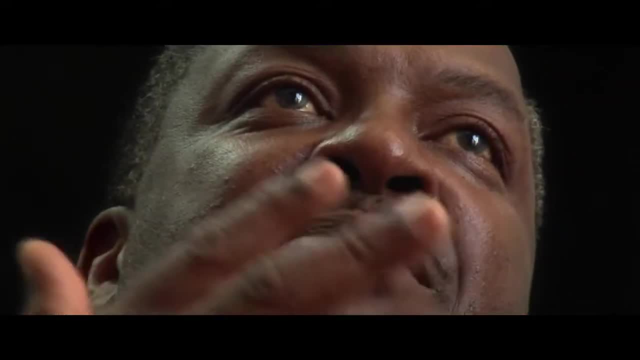 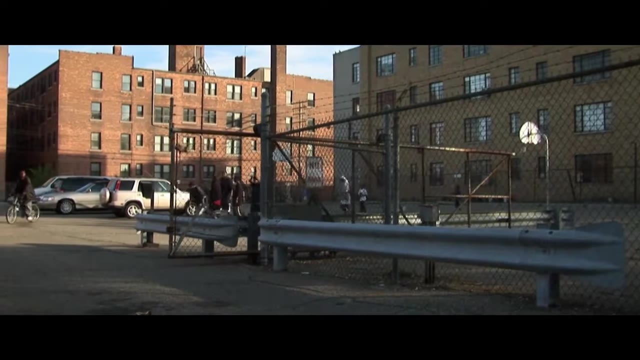 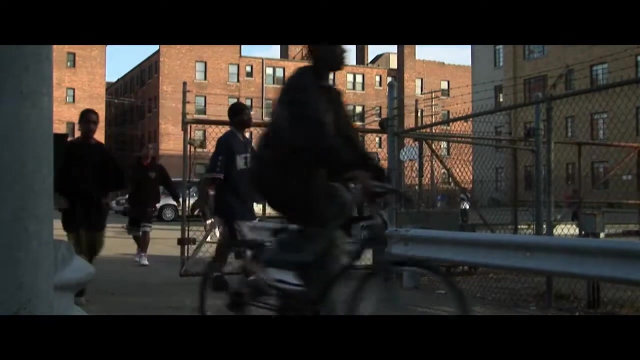 in the sense that the stereotype is respected by people everywhere: The basketball player, the rap star that They know derive value from identification with that. So he was saying he calls it the Cool Poles culture. I don't care about anything, I'm not affected by anything, I don't have to. 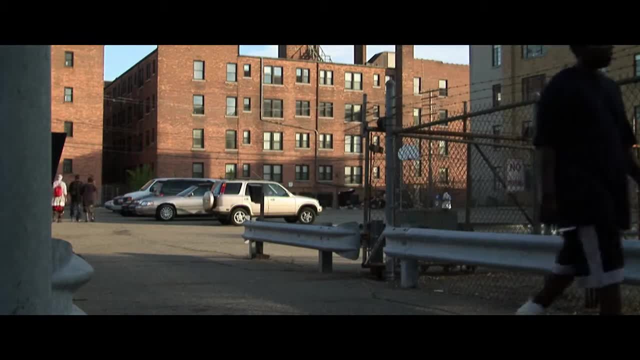 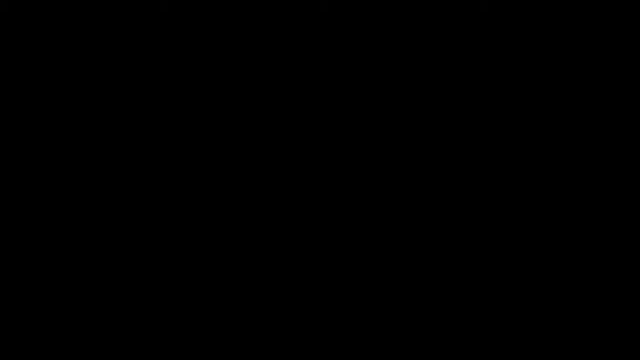 study, I don't have to do these mundane things that regular people have to do. I identify with the gangster rapper and with the athlete, But he's saying that in scientific studies that black youth self-esteem is higher than normal because of their identification with 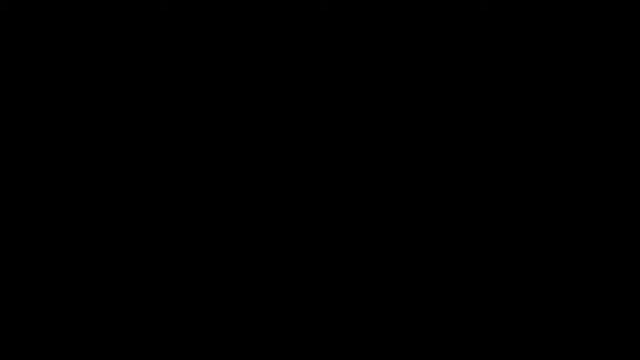 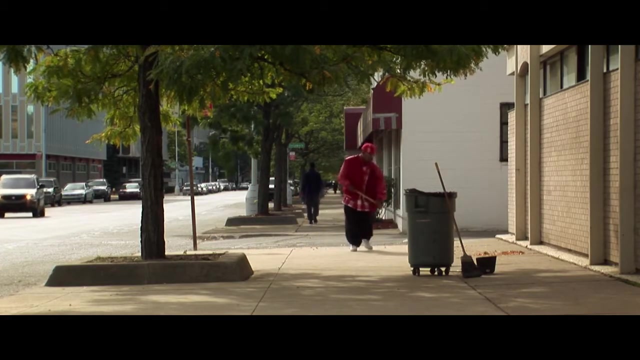 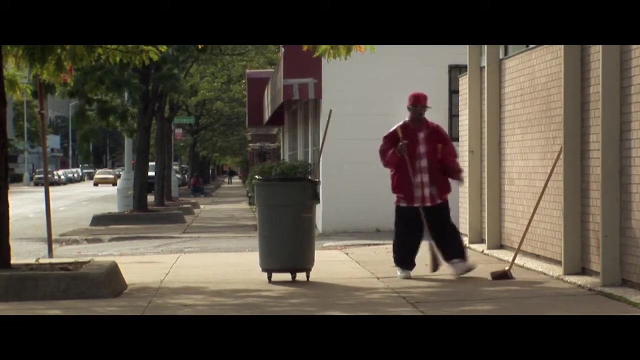 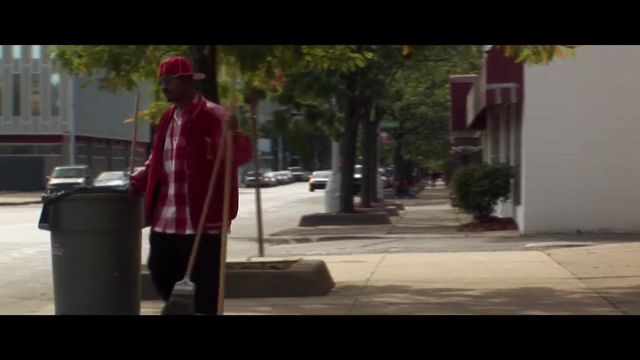 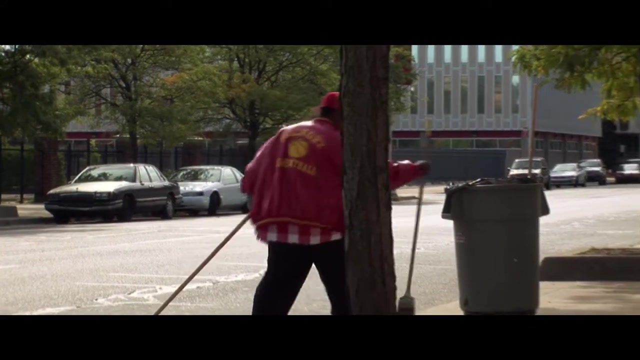 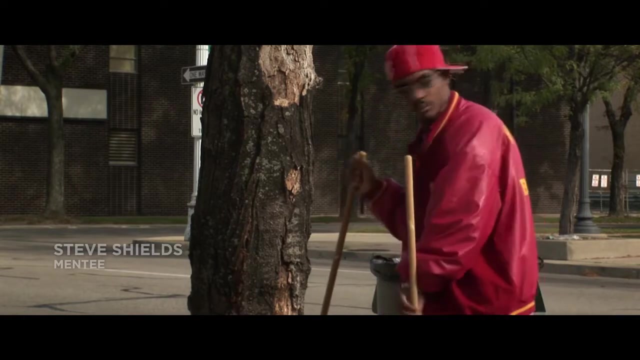 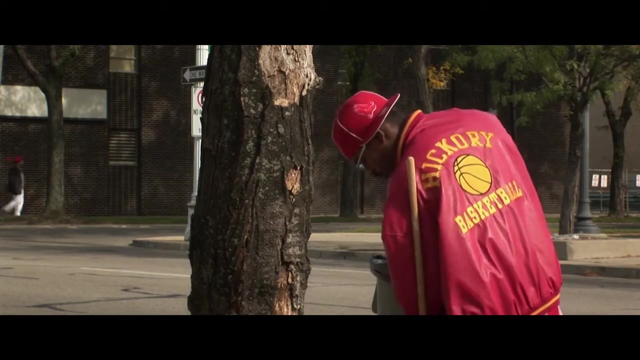 these stereotypes that are being celebrated everywhere. My name is Steve, but I'm known in the street as Vino, aka King Vino, I'm 32.. I'm from the east side of Detroit. I ended up selling drugs at 11 and joining my neighborhood gang, So 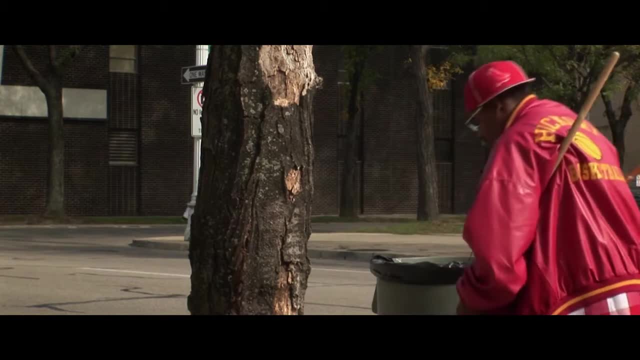 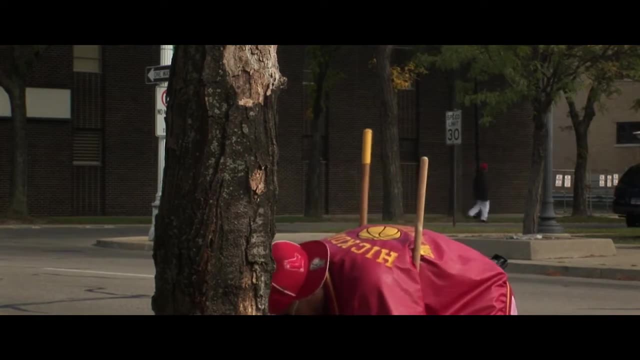 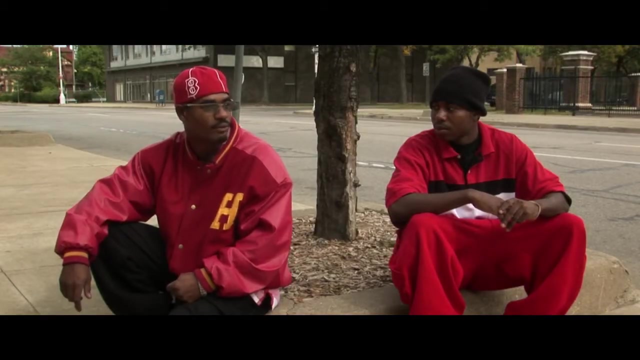 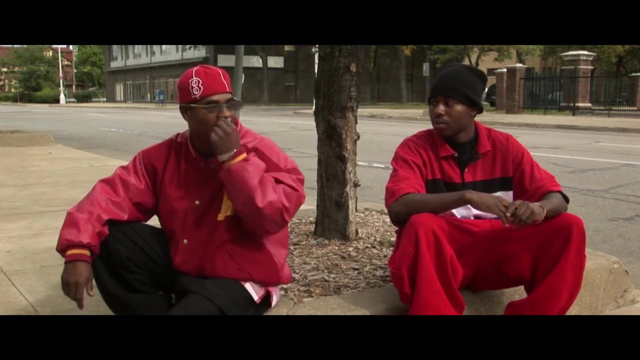 I end up using drugs. I end up going to prison. I spent 10 years in the state penitentiary. I've only been home now for like a month and a half. I see myself right now sweeping up leaves and raking leaves, basically, And I say just to catch. I didn't want to be. 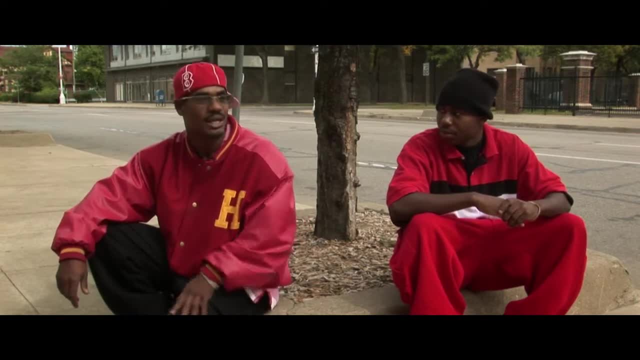 When I, before I, went to prison- I did 10 years- It was like I don't want to be a bum. You know what I'm saying. I used to always say: I'm the freshest, I'm the cleanest, I'm 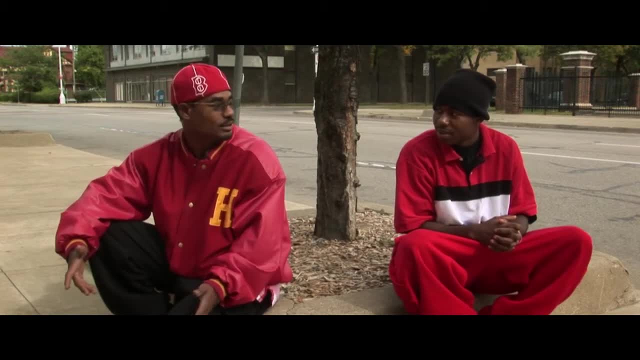 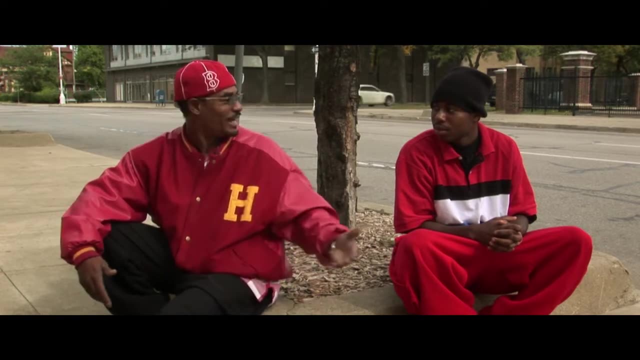 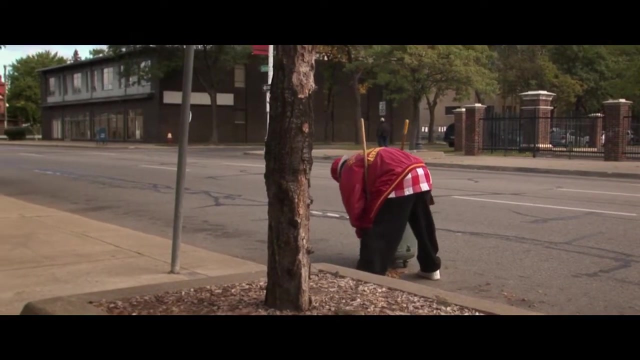 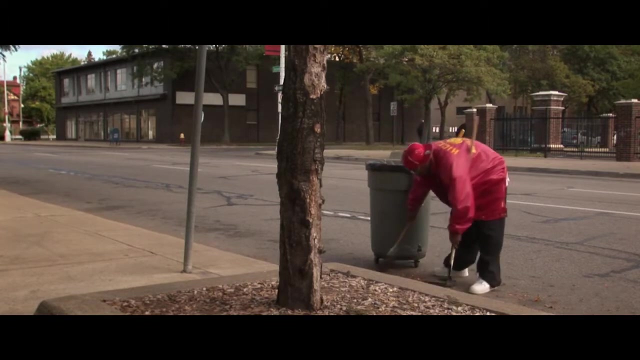 the best And everything I do. all praise due to Allah, the Beneficent, the Merciful. But at the same time I'm sitting here doing what I said I didn't want to do at 32.. Oh, I said when I was like 10,, 11, and 12, I used to look up to like drug dealers and 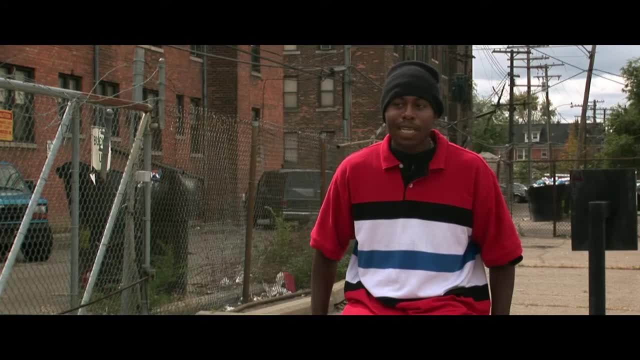 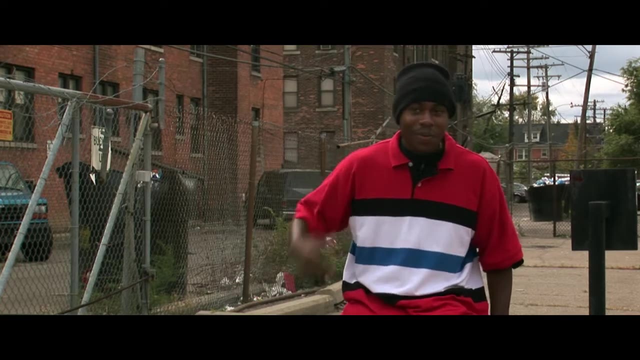 I used to always want to be a bum. I 였 like robbing them And they used to always tell me like you should go play basketball or go play video games or something. But at that age you be like just looking at the clothes they wear. 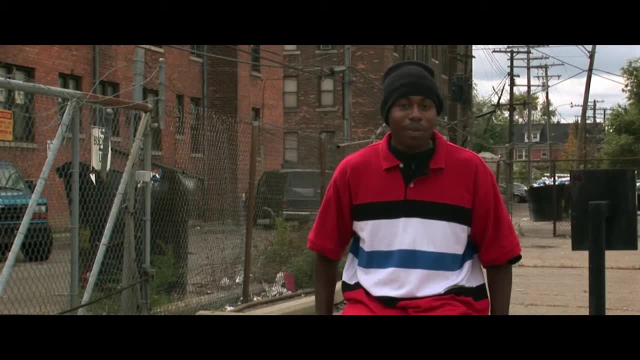 looking at the cars they got. So you really wanna be like them more than anybody, more than your parents. You wanna be like them because you know they don't, they don't work no, nine to five jobs. It's like you, you look up to them, even though they do what they do, you ain't looking. 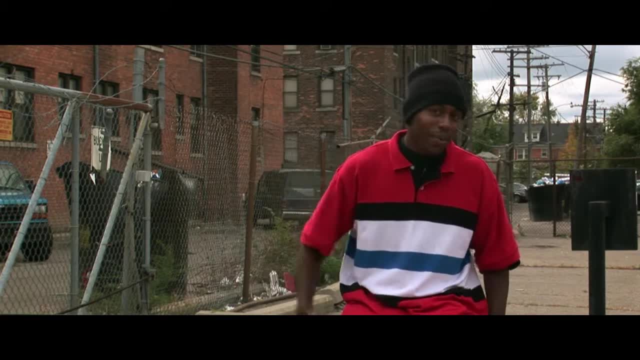 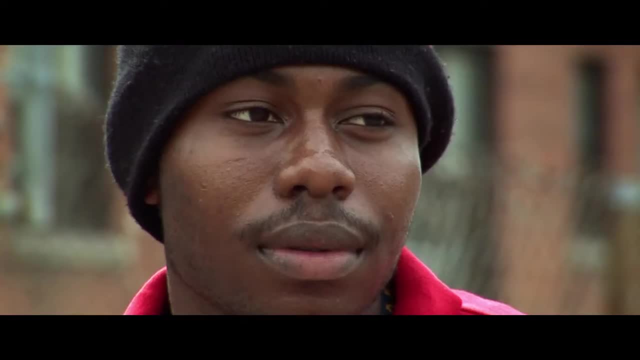 at that, You looking at the clothes, the cars. they wake up. when they want to wake up, go to sleep when they want to go to sleep. They control their destiny. so you know, I look up to anybody who control their own destiny. 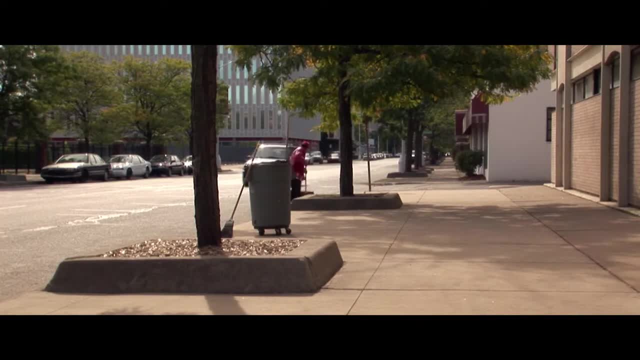 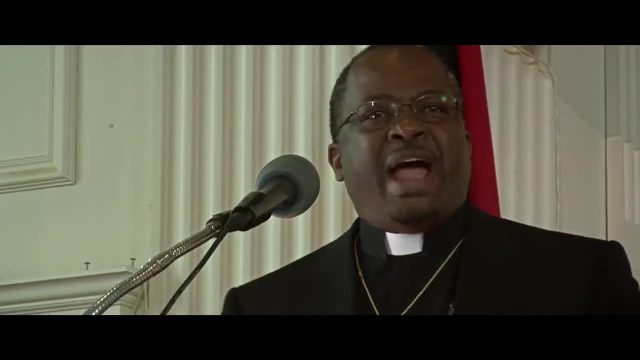 We live in a world where black manhood is a joke. it's a joke, And what most black men call being a man has nothing to do with manhood. Little knuckleheads with their pants all down their back, they ain't got nothing to do with. 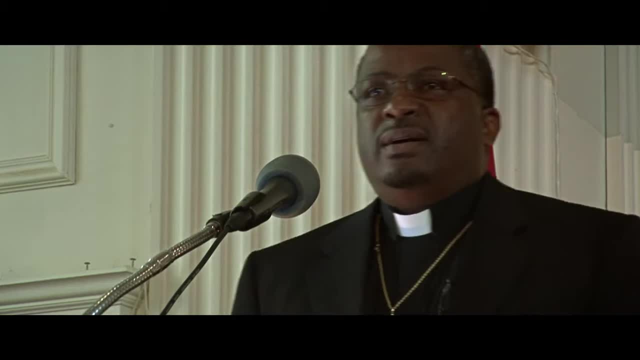 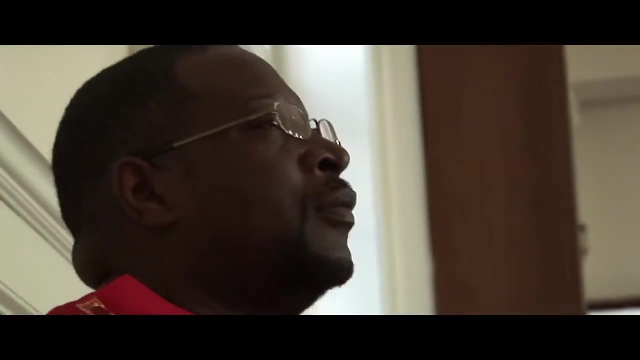 manhood. Those people ain't got nothing to do with manhood. Your grill Foul mouthed rappers ain't got nothing to do with manhood. Calling women bitches and hoes in public ain't got nothing to do with manhood. 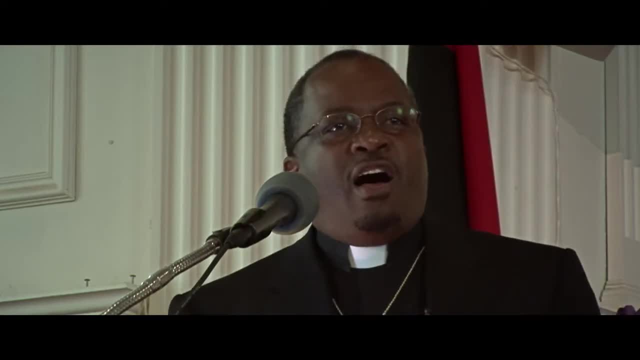 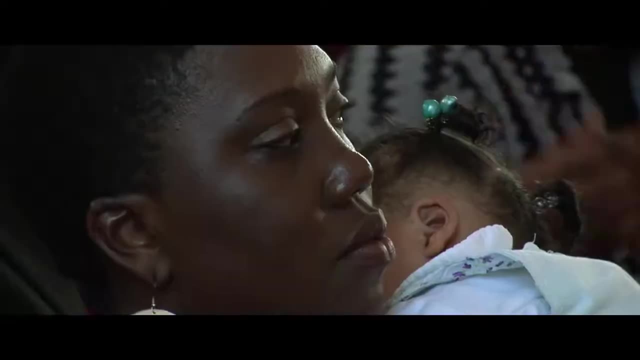 Pimps and predatory hustlers and dope men. oh, I'm getting mad, I'm getting paid, I'm going to be a man. You ain't a man. You a predatory hustler, You a man. A man is not a man for himself. 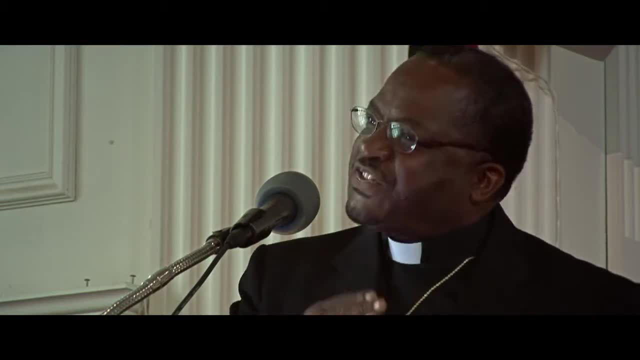 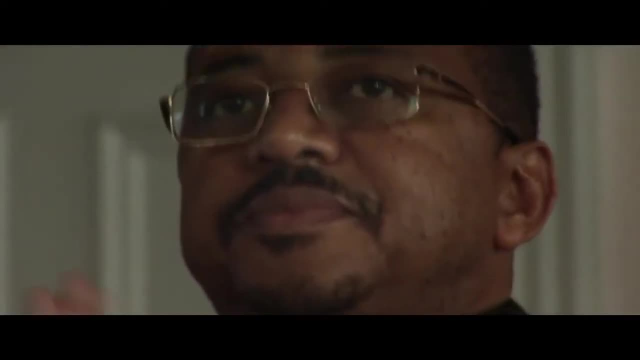 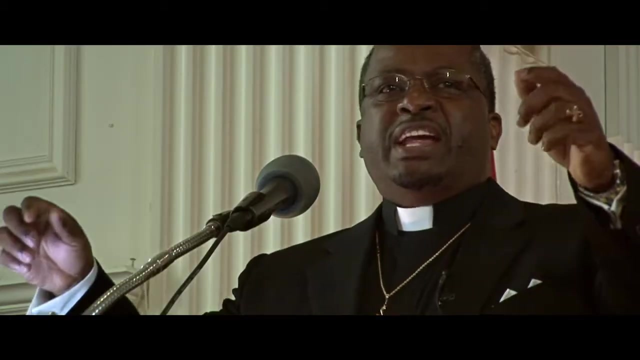 A man is a man for his people and for his family and for his community. He's not a man for himself. The best and the most distinguished men are not the ones that had the diamond rings and all the accoutrements of wealth for themselves. 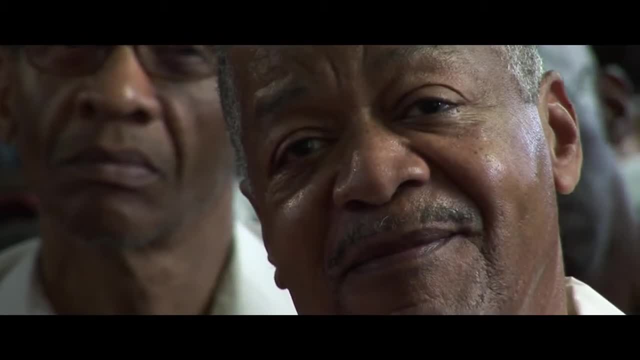 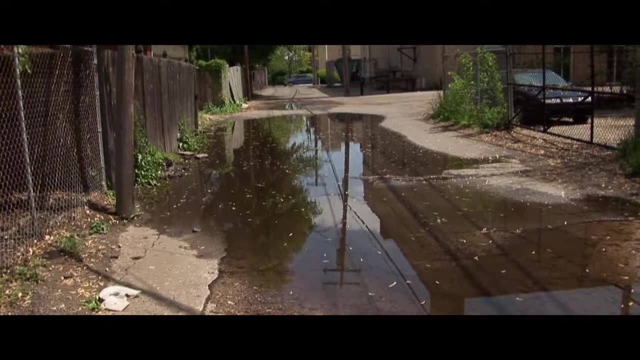 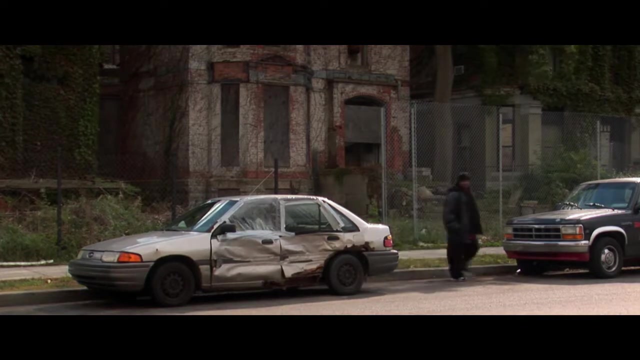 The best and greatest men were known for the wealth themselves. That's not how it is. the wealth they gave to other people to make other people better, to make other lives more rich. i got up one morning, man. i remember it was in january, uh, 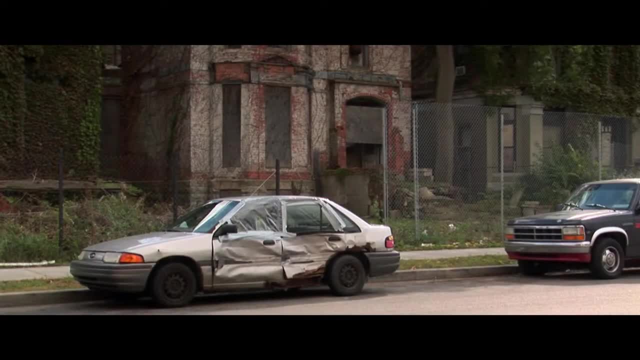 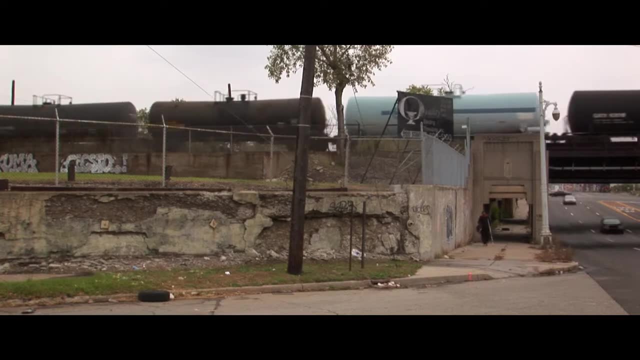 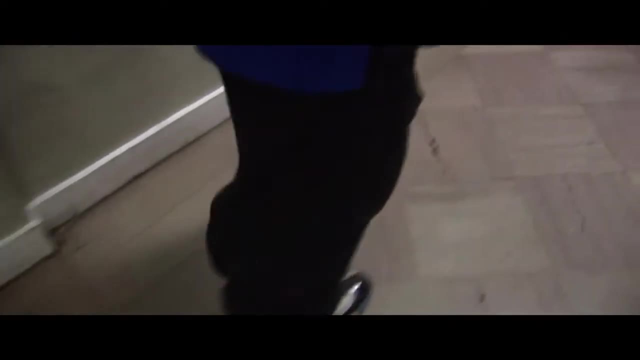 i think i had like two dollars in my pocket, but i i know where to go, okay, and i just i walked, man, i walked about five miles, just not knowing what to do, just thinking, and i ended up at the shelter downtown on peterborough. man, i got in there, found out my mother and my little brothers was there and uh, 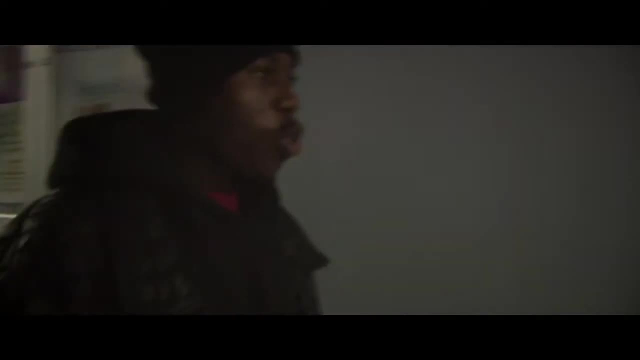 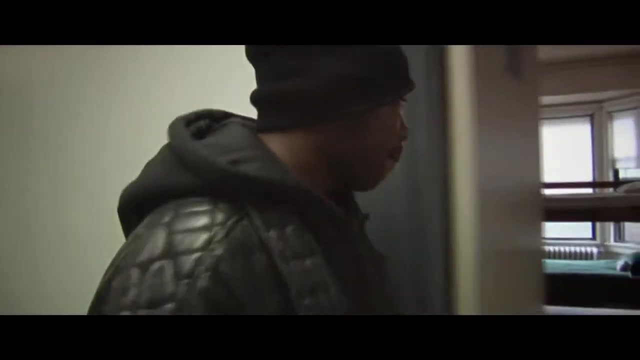 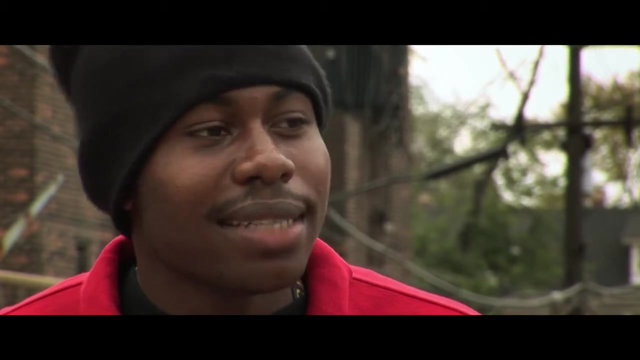 home the shelters. yo, i stayed in the football- not long, but you don't got to stay there long to realize you at the bottom. yo and i got kicked out and, uh, i went to a shelter called the nso you know that's the worstest place you could be. it's like 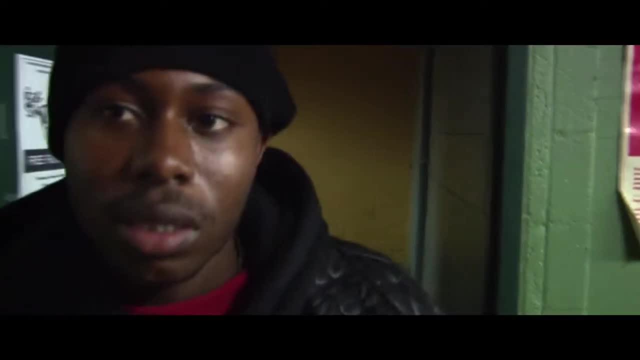 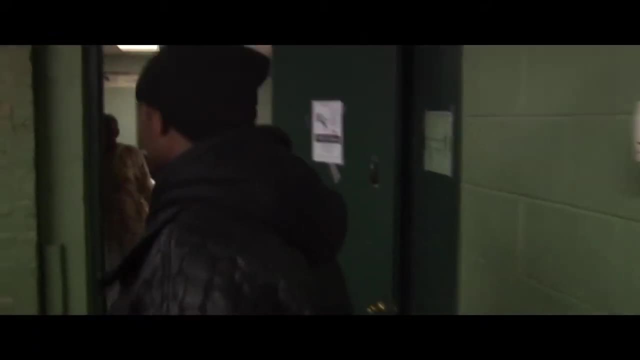 you need to get yourself together when you go there. like it was people there that was like mentally insane, but i guess the city ain't had nowhere for him to go, so they right there. you know, i'm not gonna lie to you. i'm not gonna lie to you. 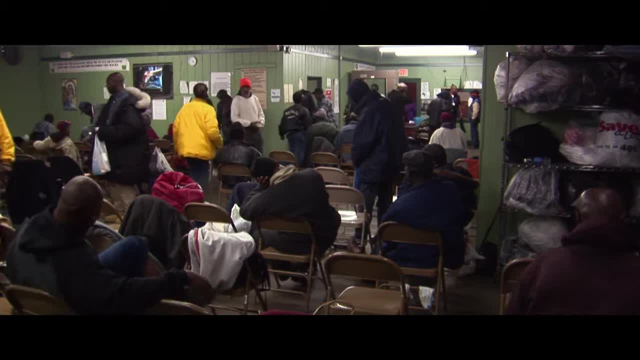 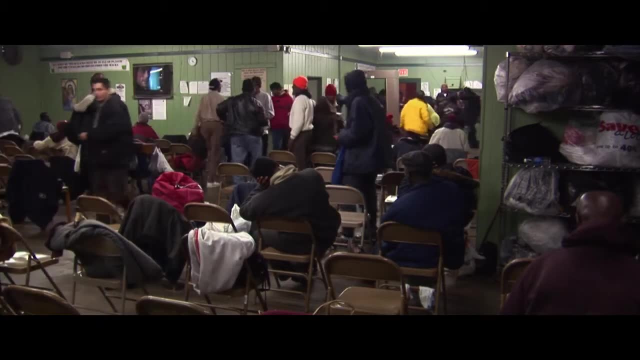 you know, it didn't seem like they was really getting help, like they wouldn't get the medication they needed. and you got seats, you got chairs that you sit in and go to sleep in at night. you know what i'm saying? you got no shower, no, nothing. so 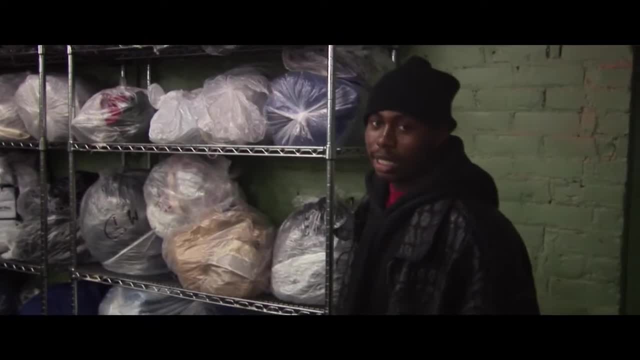 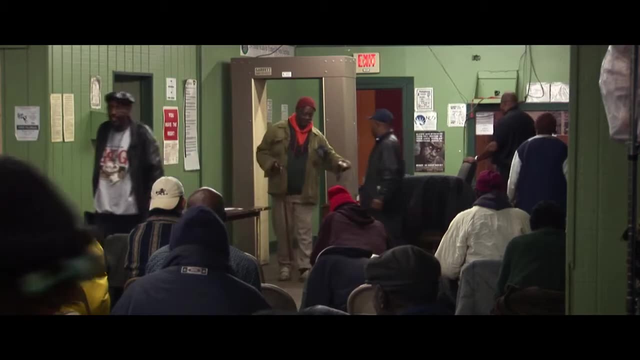 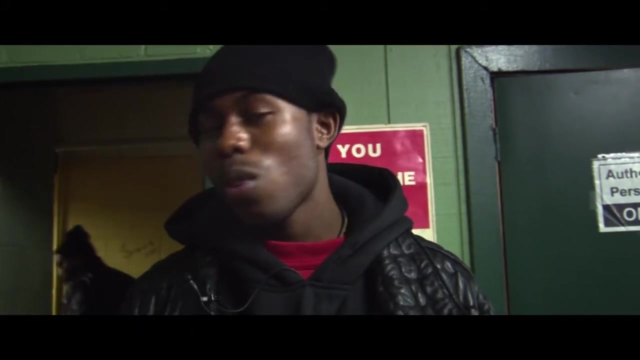 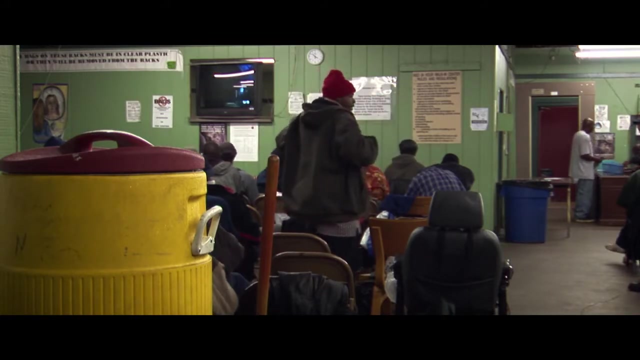 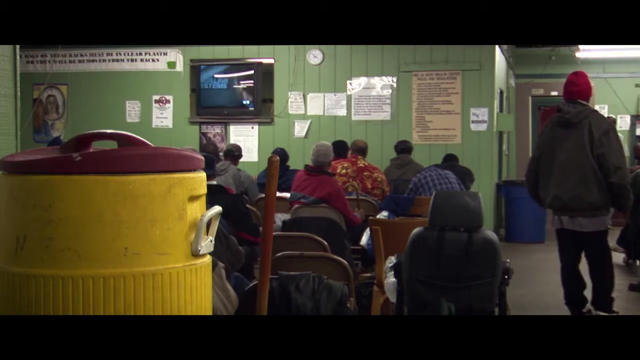 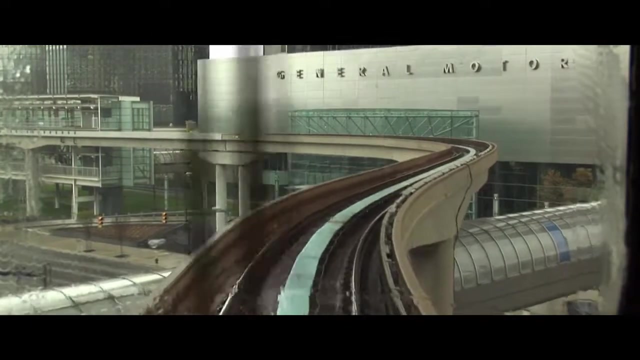 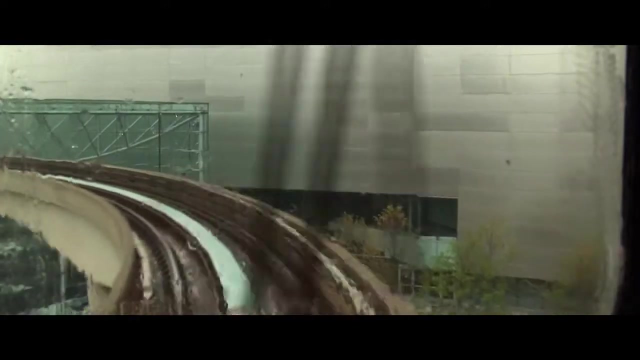 right here. you know what i'm saying, where the stuff got stored, that in anything. i'm glad man didn't make sunshine, cause he may not let it shine all right on me. i'm glad man didn't make tears drop, cause he finds joy in every tear. 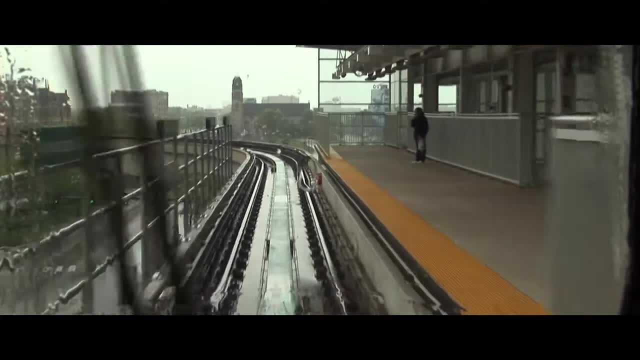 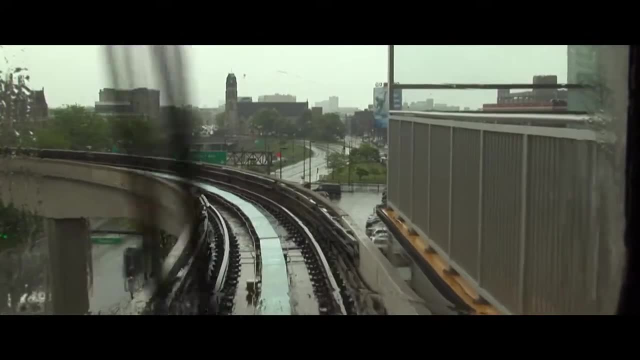 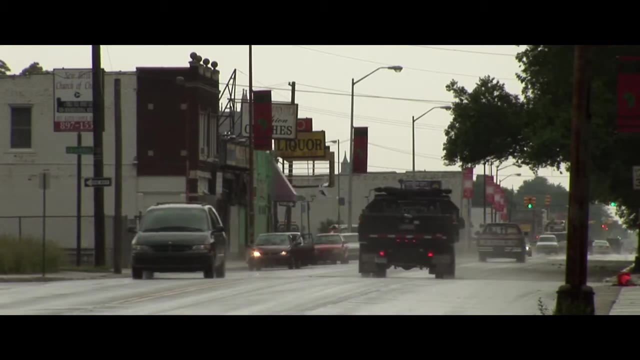 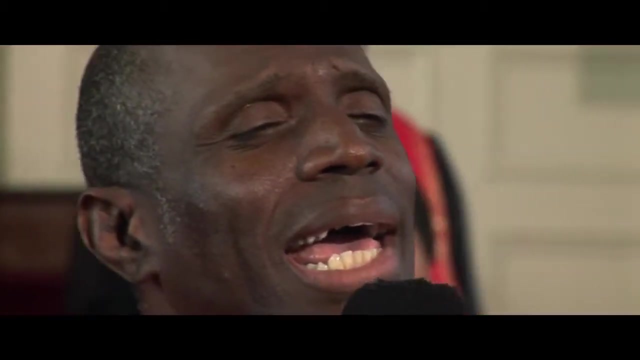 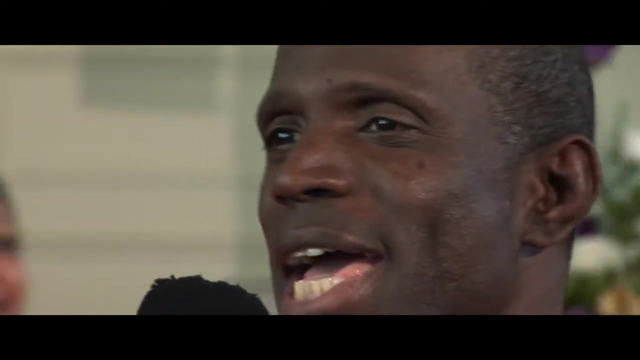 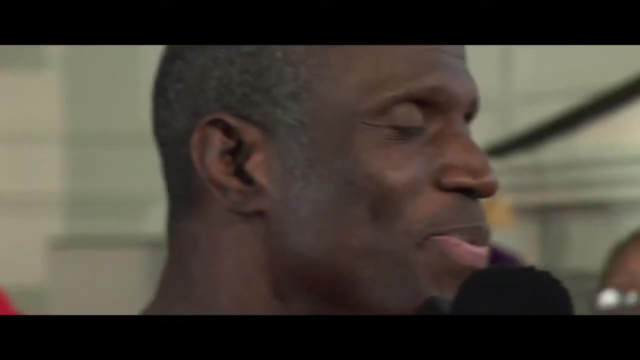 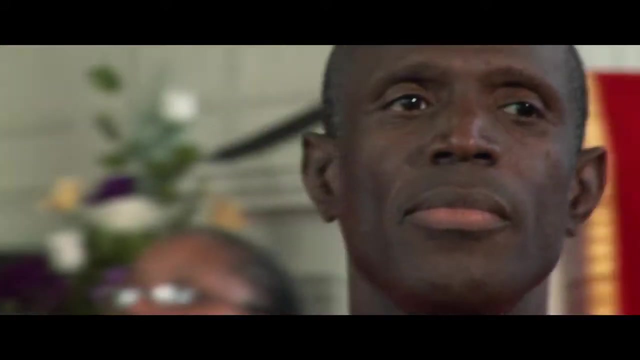 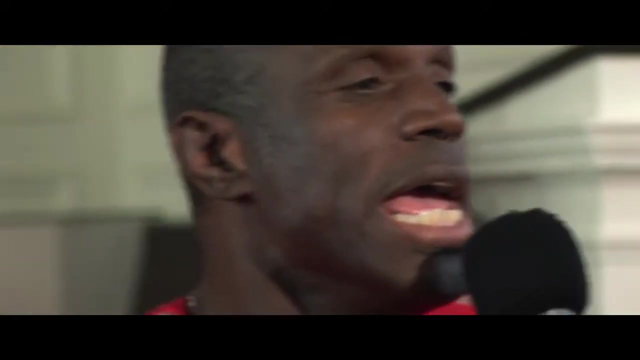 i'm glad man didn't give life just to you- you know, that's same for everything else to me- Cause he would surely, surely destroy, destroy me. I'm glad, I'm glad, I'm glad, glad, glad, glad, I'm glad. God made me. He made me in his image, made me in his image. 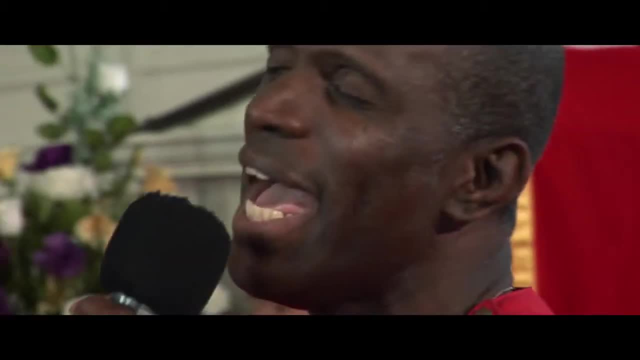 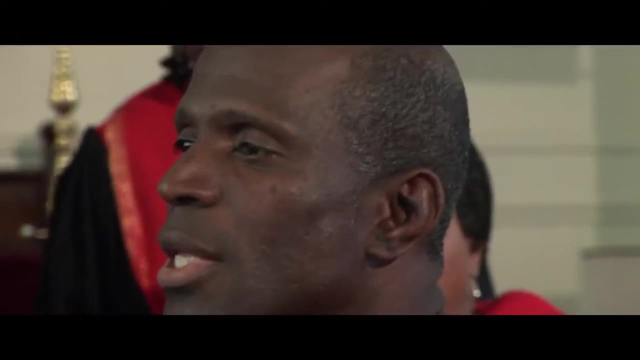 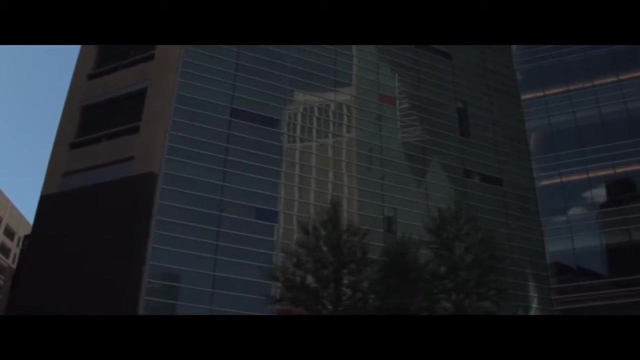 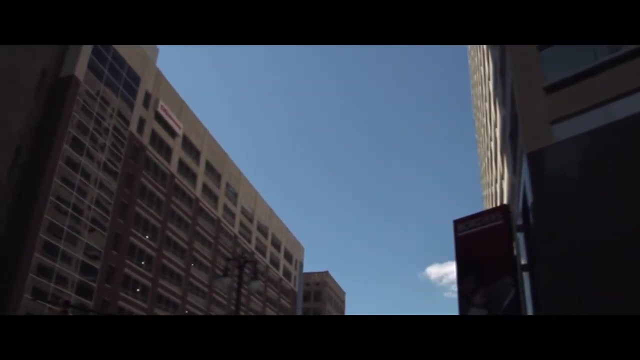 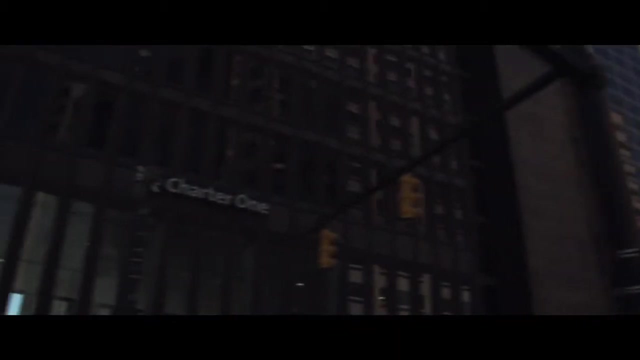 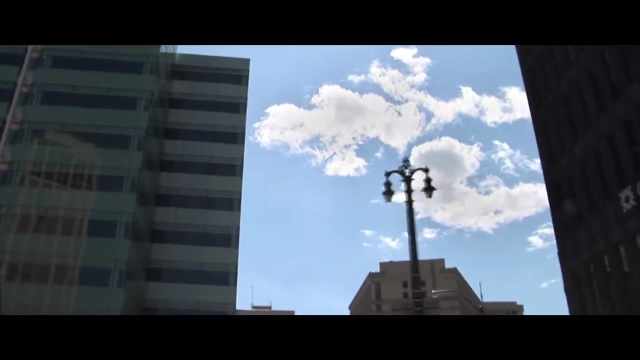 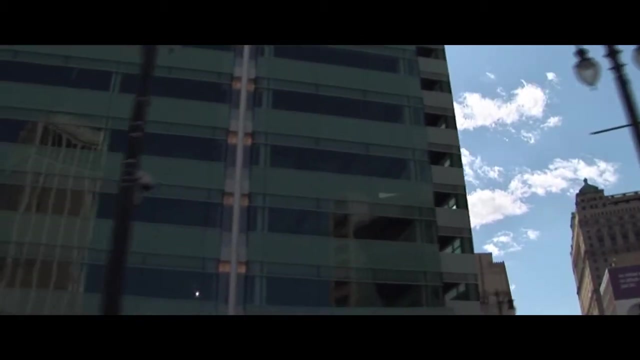 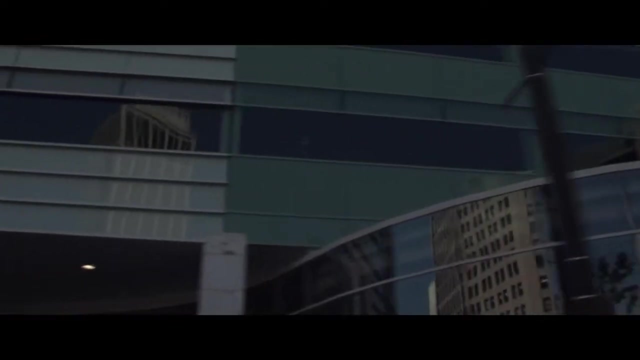 gave me life. He made me black, just like him. He trusted the world in the palm of our hand And he told us: black folks, you've got to see about yourself. He came, He gave me wisdom and knowledge. To blame somebody else for the state of our lives? to blame somebody else is to give them. 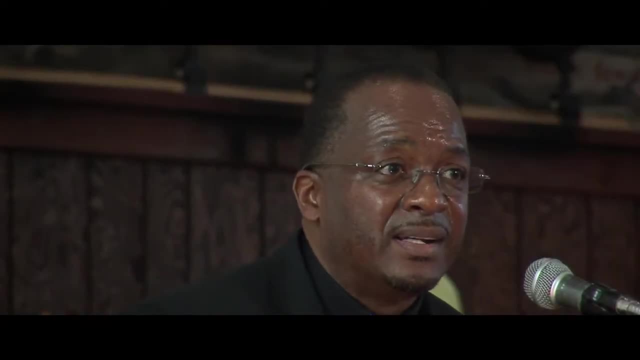 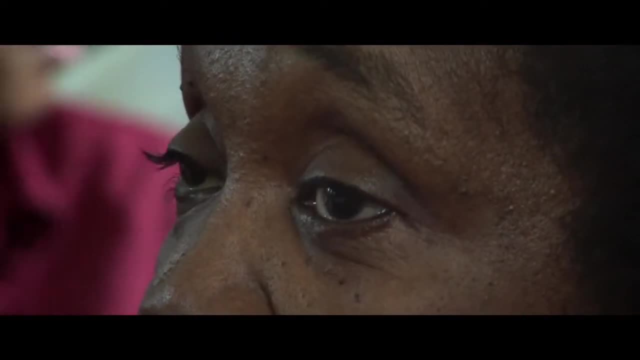 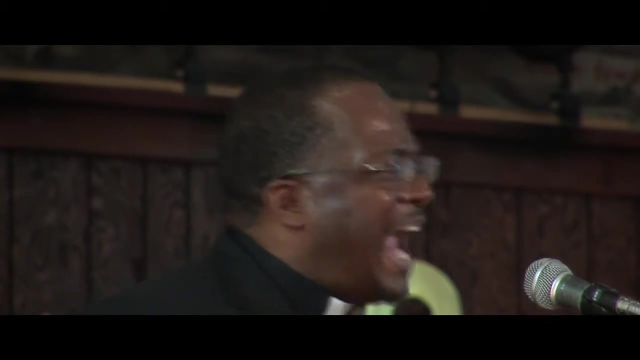 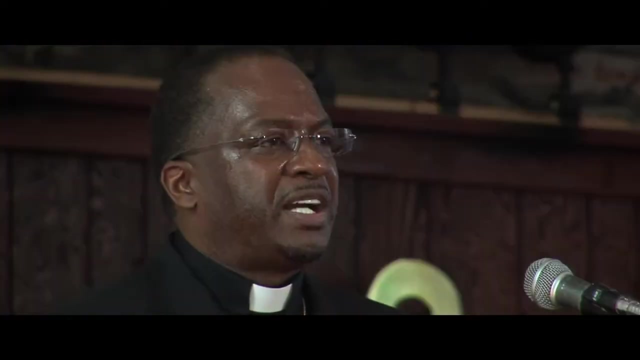 I mean, you know, I had a hard, hard childhood. I had difficultyyou're responsible. Be responsible. You'll be healthier and you'll be happier. You'll be more respected if you'll be responsible. Teaching kids to be responsible, because responsibility is at the very heart of what it means to a 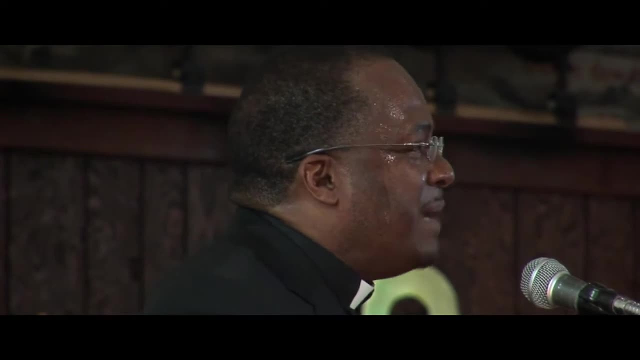 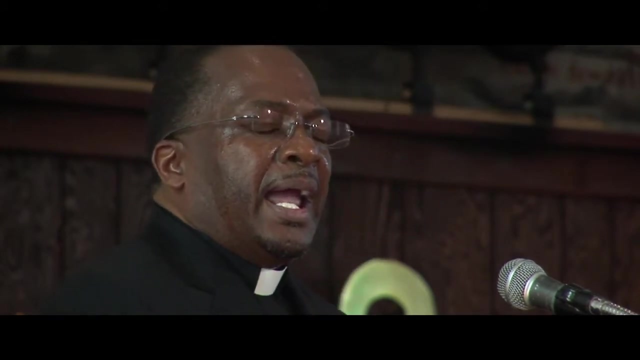 man. The song says: I'm glad God made me. He made me in his image, He made me black, like him. Yeah, Yeah, Yeah, Yes, like him. He's saying that put the whole world in your hands Be. 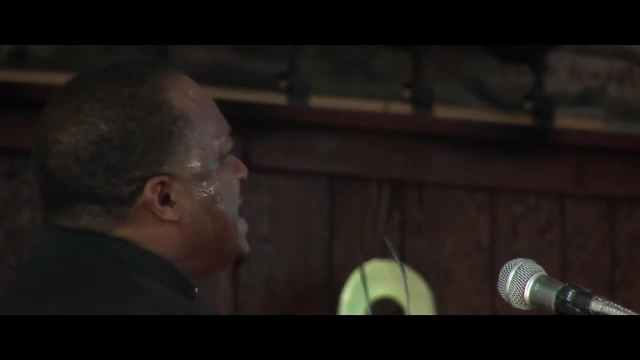 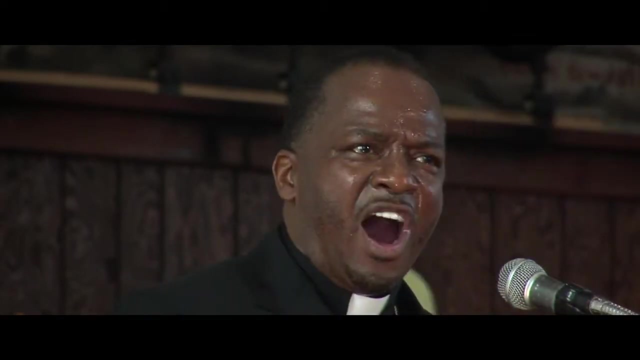 responsible. Don't sit there and tell God: well, I wasn't the president, I wasn't rich, I wasn't powerful, So they messed up the world. God is going to tell you: I didn't give them the world, I gave you the world. All of y'all got the world. I'm 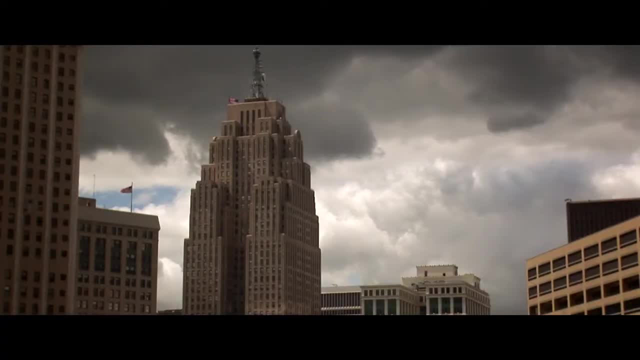 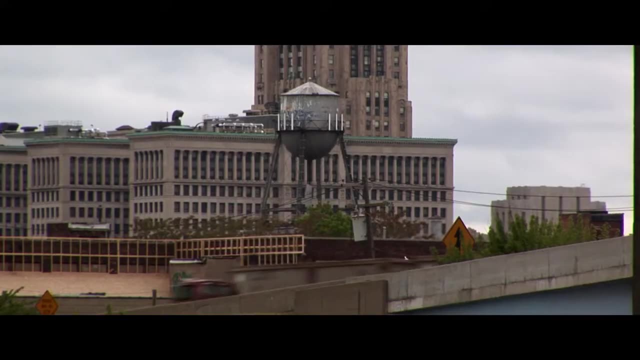 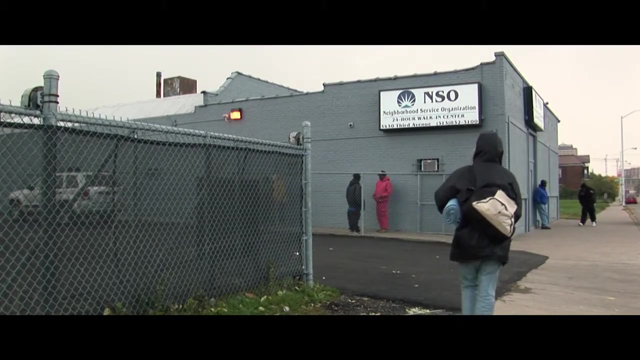 holding you accountable for the world. So when you join the church you can say: look, I want to transfer to Atlanta, Oh yeah, And get out of this lifestyle you're in. Change your life, brother. I can't change man. You can't change brother. Jesus changed, Jesus changed, I'm not going. 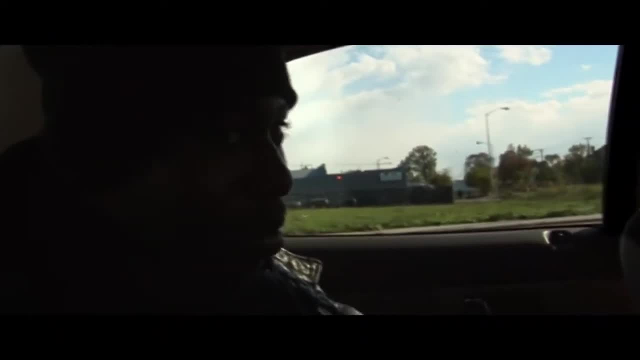 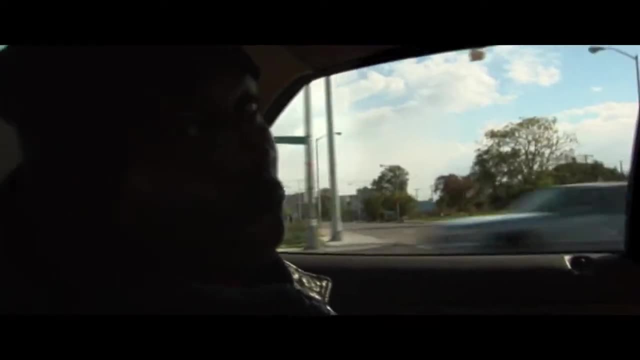 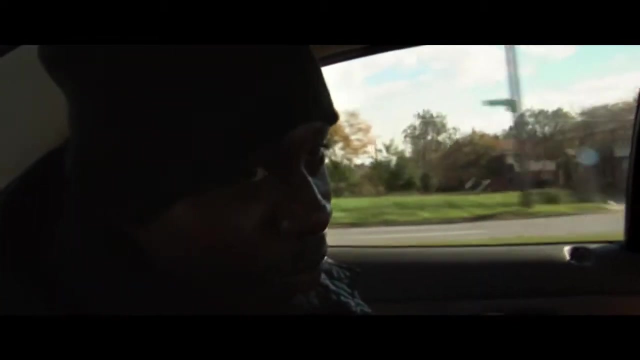 to stop hustling because I know where I can be at if I stop hustling. man. People say get a job. Alright, I'm a Detroit city Highest unemployment rate for like two years, maybe three. But everybody say: go to church, Go to school, You go to school and you get a. 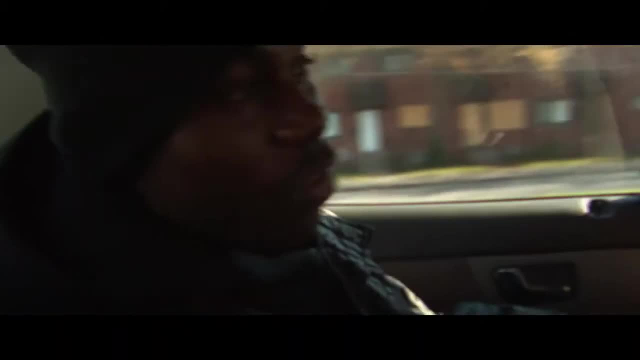 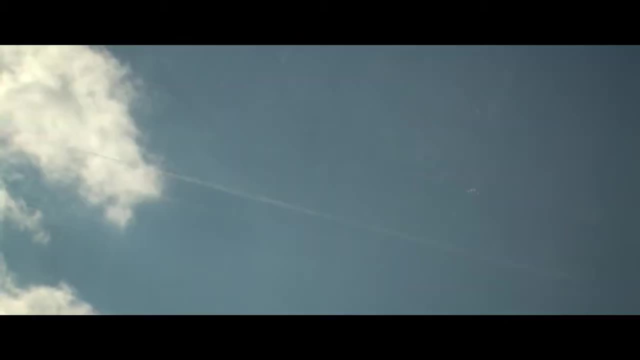 degree But the economy down, we facing millions and millions of dollar deficit. What I'm a go to school for man. You a fool if you go to school. I used to work at White Castle. I knew it like two people went to college. You know what I'm saying. I'm going to keep. 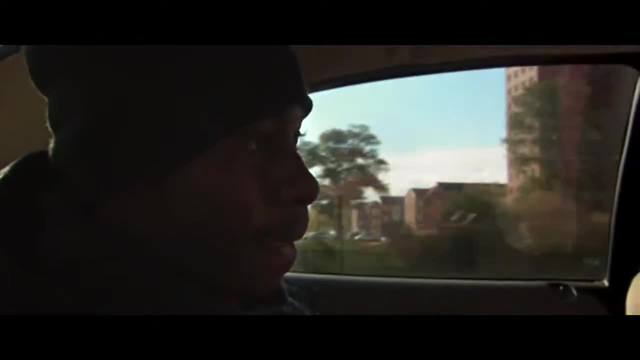 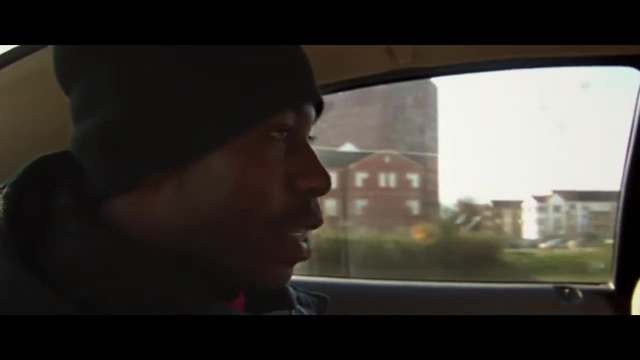 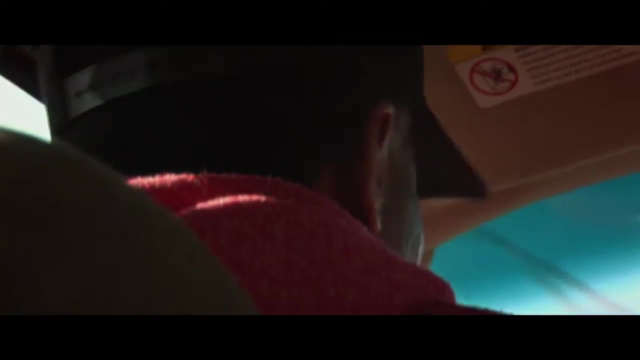 real? no, i only knew one. you know what i'm saying. he got a certificate in computers and i asked him: man like man, what's up? man, you went to school, man, why is you working here, dog? he like i can't find no job. man, all the jobs i do find, be way out. i can't get out there. 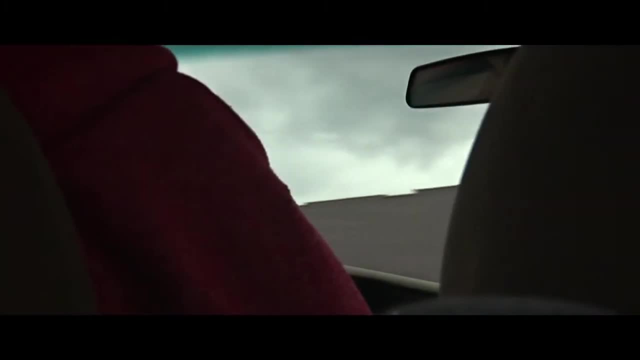 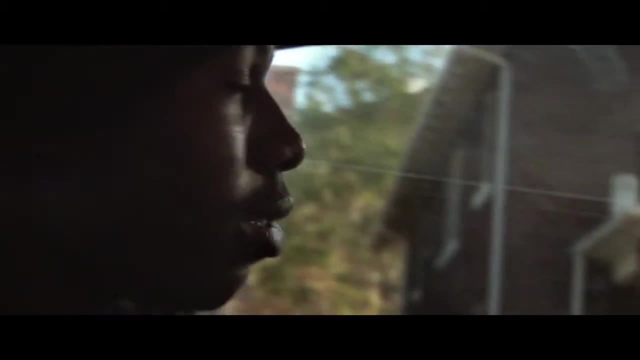 you know what i'm saying. so all that knowledge that he got, he can't use it. you know what i'm saying. y'all want people to go to college though. right, of course that's what i'm saying. that's what the minister said last sunday. y'all want people to go to 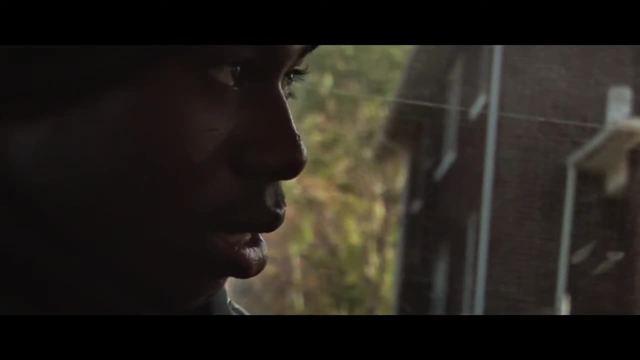 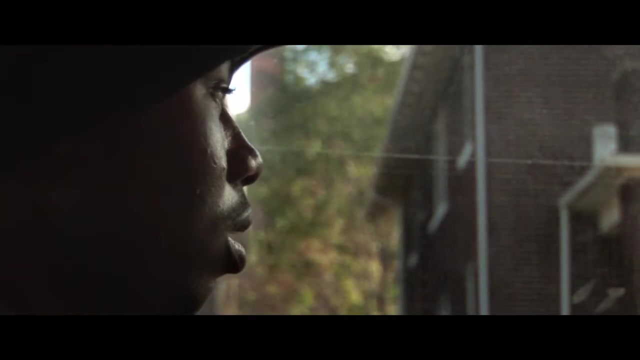 college: people to go to college and come back and bring them skills back. but bring the skills back. college is meant to work for them. man, the white people, man, no, you, i mean you. you know, we want people to go to college so you can go in business for yourself. 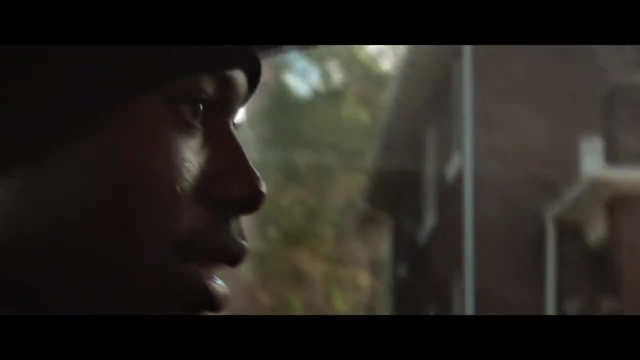 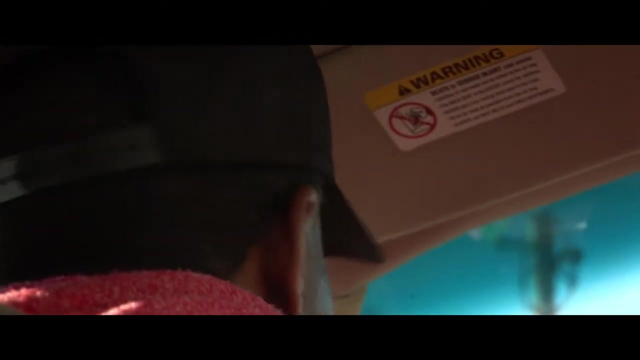 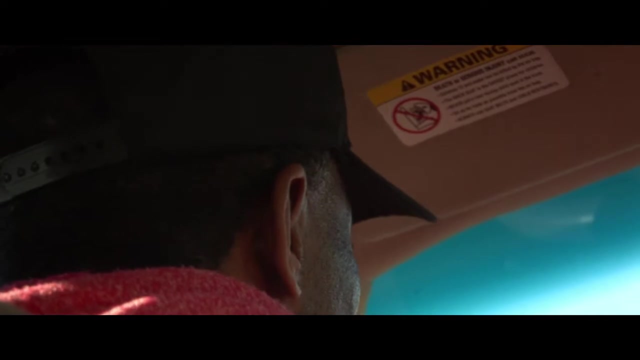 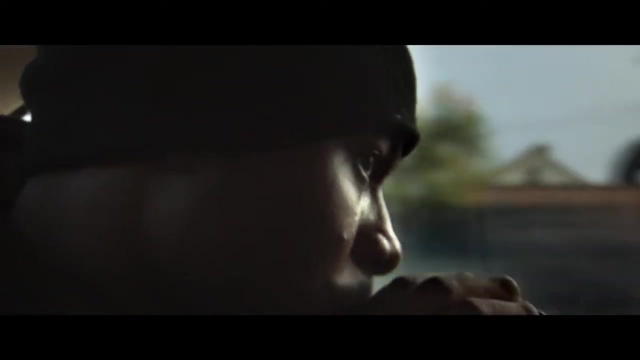 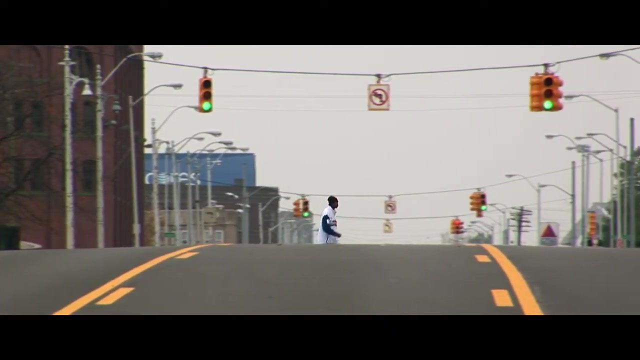 for your own people. okay, open up your own business. we're talking about being self-sufficient. yeah, so, so her money. um, you coming to church on sunday- it's youth sunday, all the youth gonna be there. i'm getting my grandson and everybody. but if i join the church, what happens if i gotta go back to the streets? 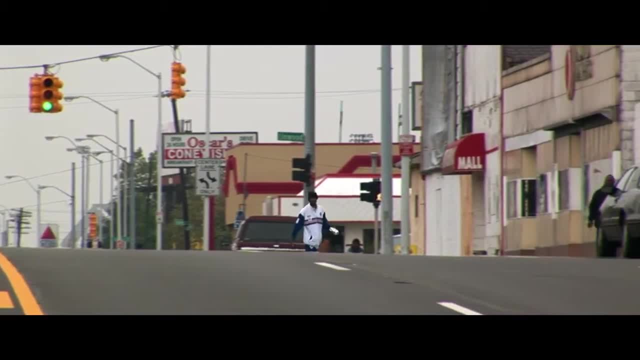 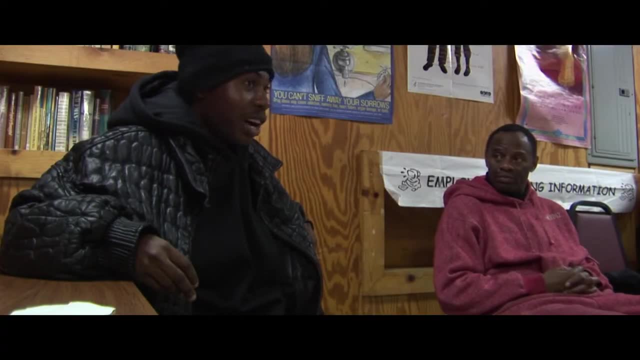 and sell something to survive. you ain't gotta do that. your mentality be a different. i'm telling you it's a difference. i don't want to join the church and then go sell a rock on monday. man, i don't want to do that. so you have to make a conscious decision that you haven't changed. 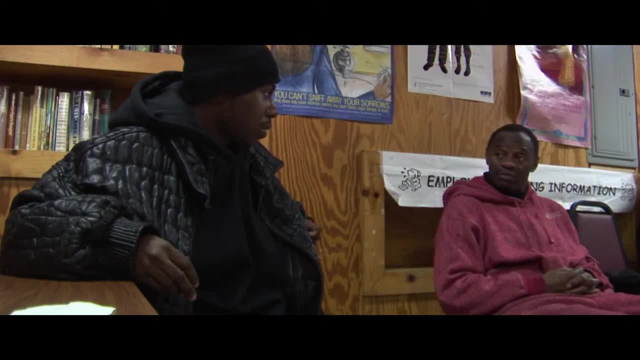 i don't want to do that. so you know what that leads to someone. let you get caught up in that. be somewhere where you ain't supposed to be. i don't want to be an outsider who has moved here and there since i've got what's going on. 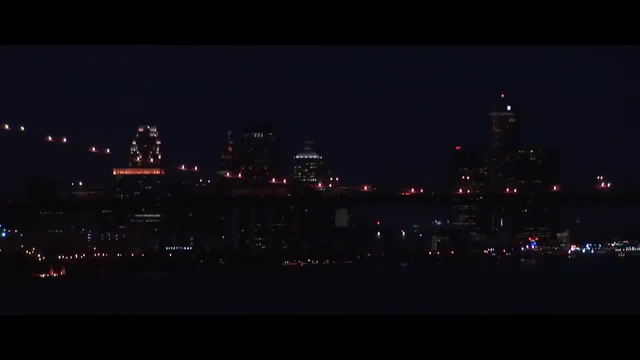 that's the issue is, i've got to do something for my people. i'll be free to do whatever that leads to. i'll be free to be educated, i'll be able to run in this place, so i'm going to do whatever i can. so i'm willing to do whatever it takes to move on and to live the life of my people. 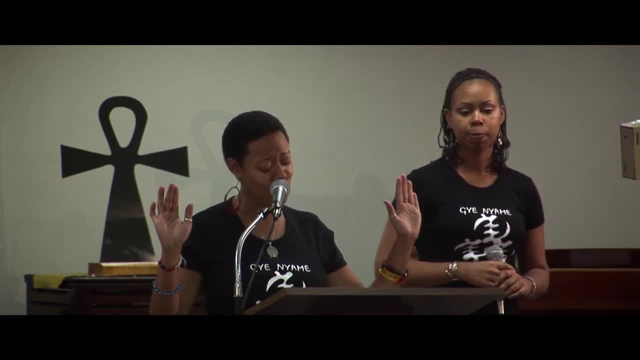 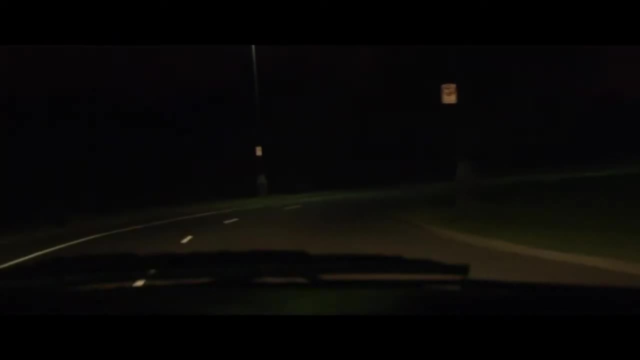 i am sure the people who made the difference in the church have a way of doing the work. i would not want to be able to live with a minority who is not fit to be in a community, and i am not trying to hide it In the ghetto streets. 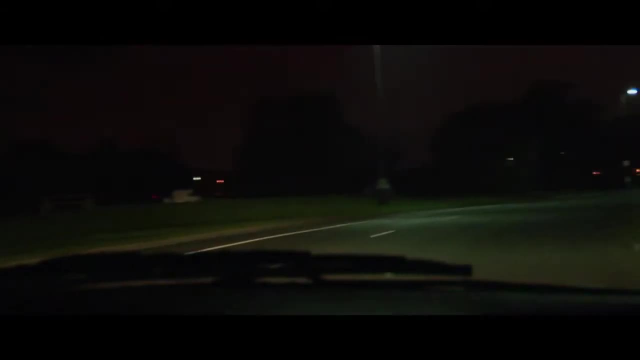 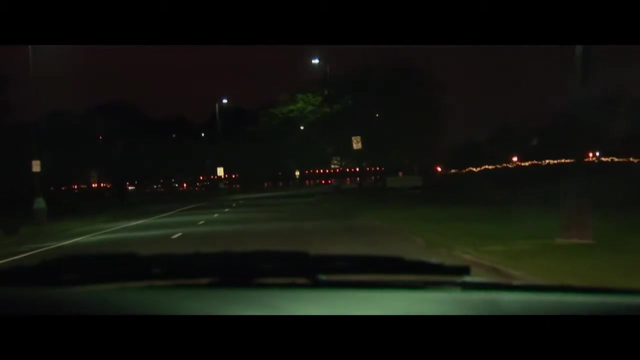 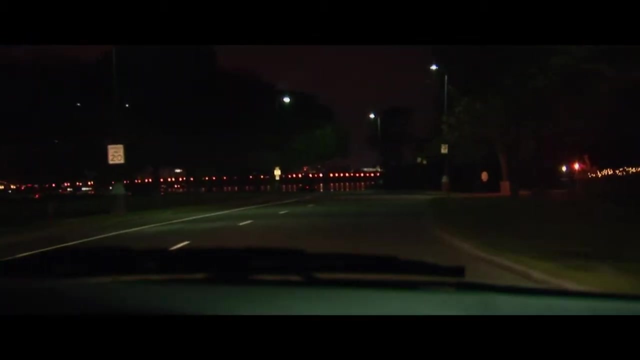 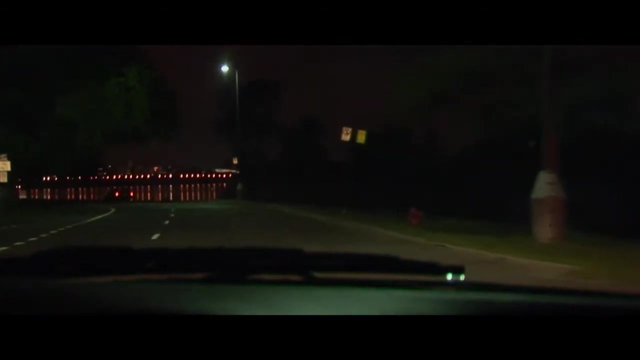 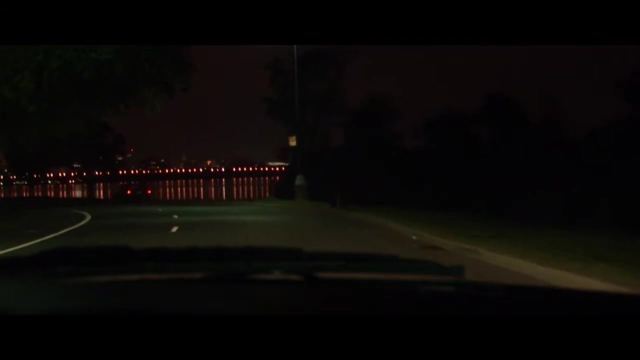 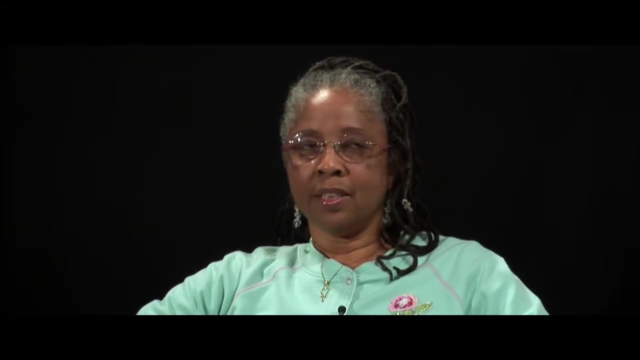 Strange fruit growing All around our feet. He left home, you know, one night, like young people do, Probably about one o'clock in the morning, on an early Wednesday morning, And he just didn't come back, Not alive. Osakwe was brutally murdered. 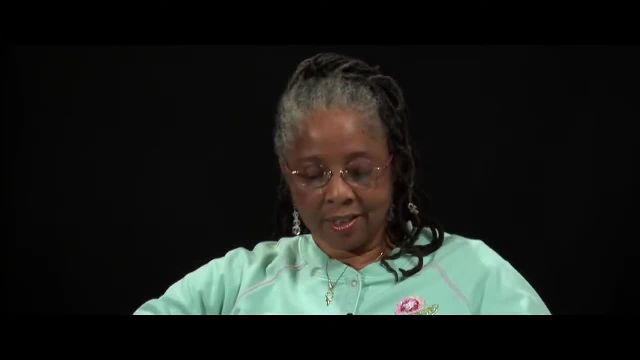 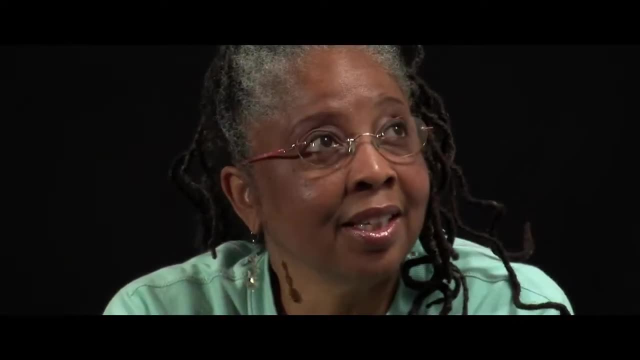 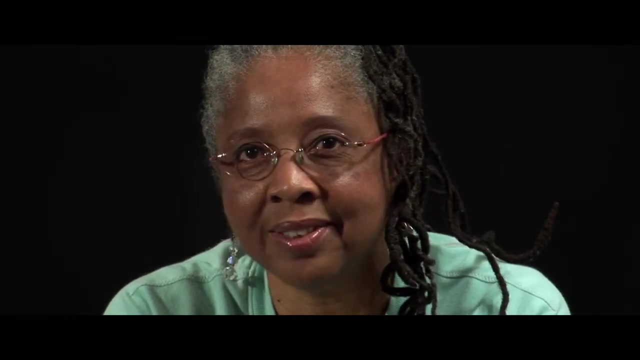 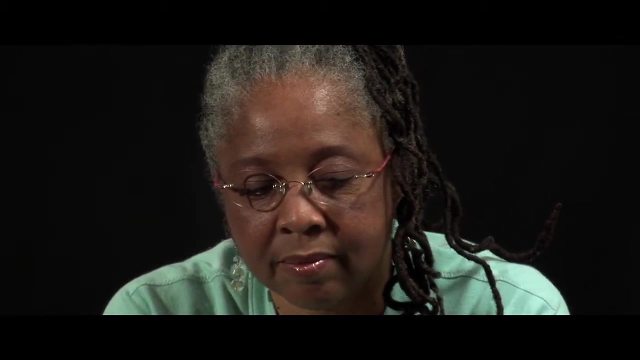 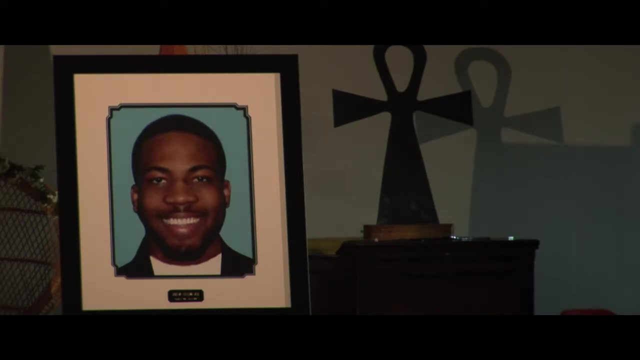 He was murdered, Taken away from us. You know, it just hits me. you know, like, hey, where's my baby? Where's my baby? You know? Yeah, Southern trees Bear a strange fruit And I don't know. 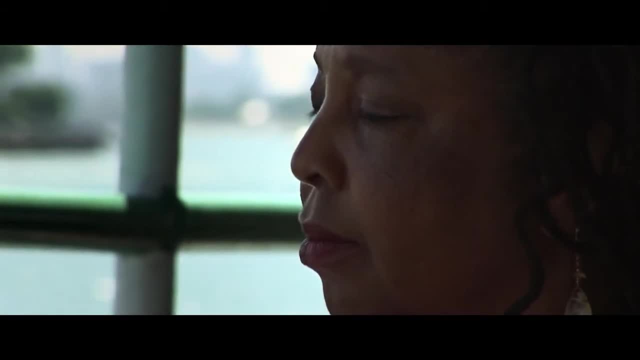 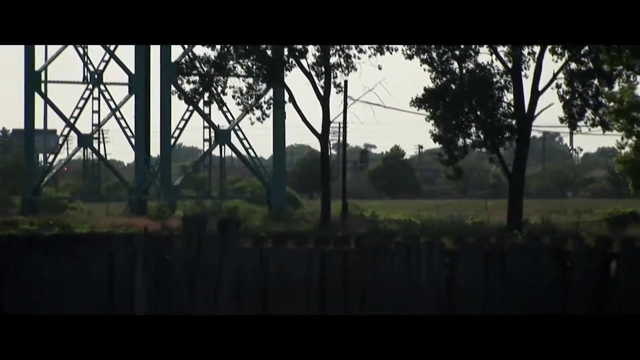 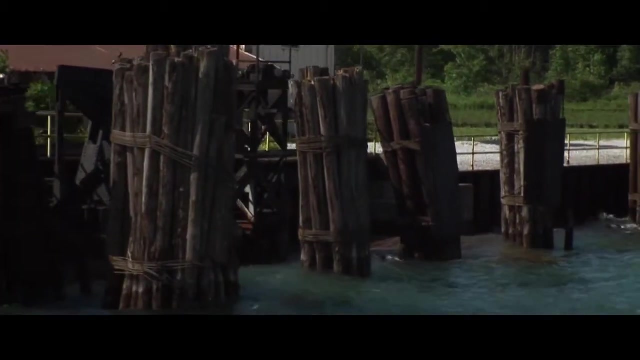 And I don't know. You know Osakwe. he had this special gift: Very charming and wise, compassionate: Blood at the root, Black bodies swinging In, the southern breeze. He was so serious about preparing to take the mantle of leadership and moving on. 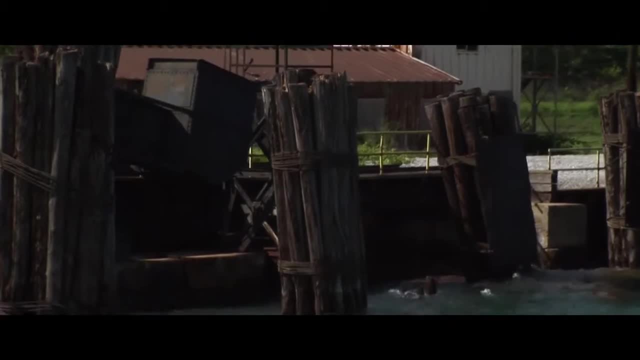 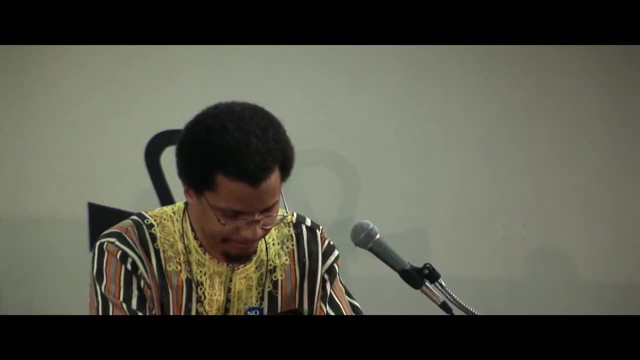 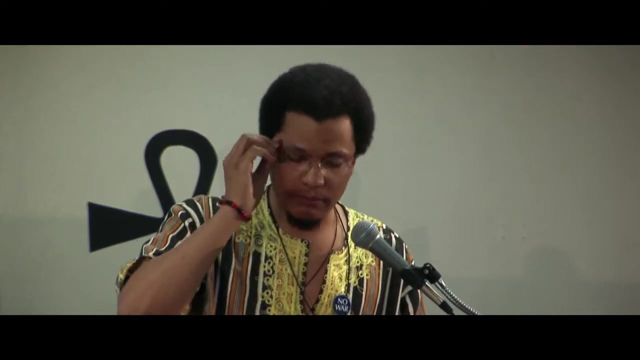 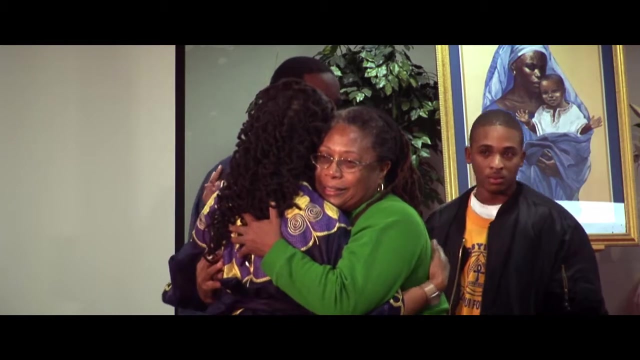 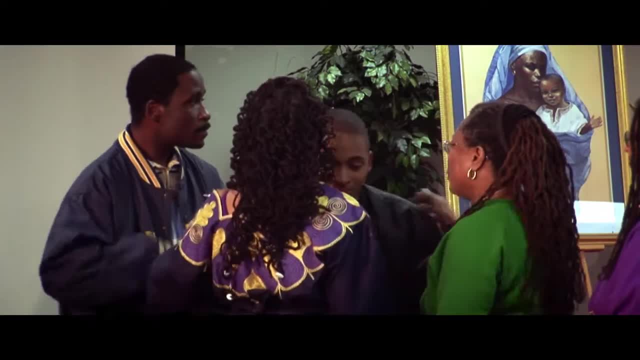 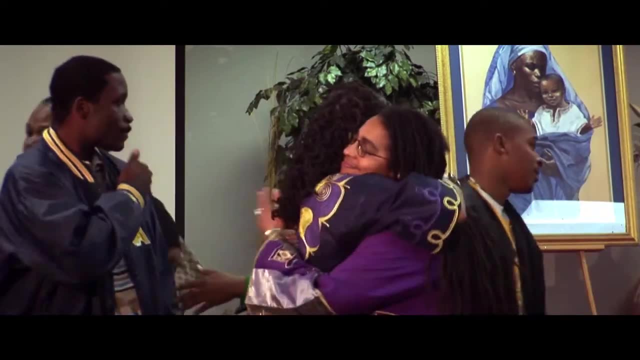 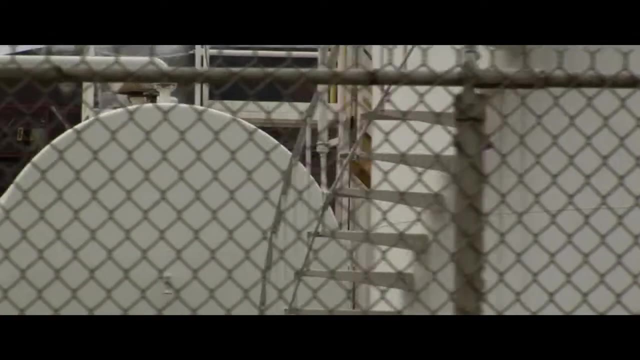 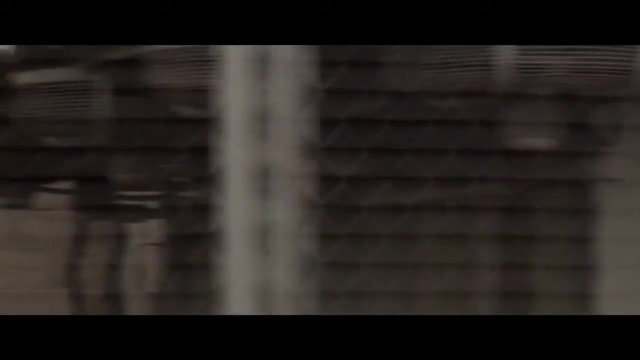 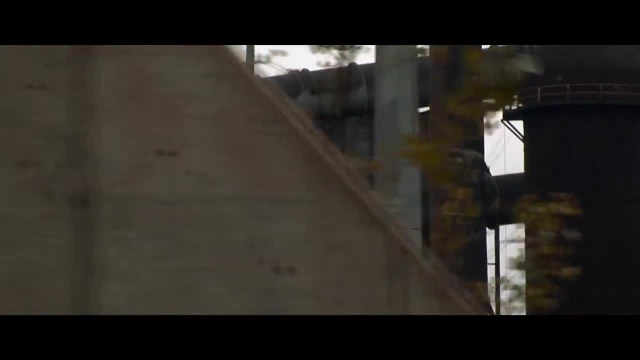 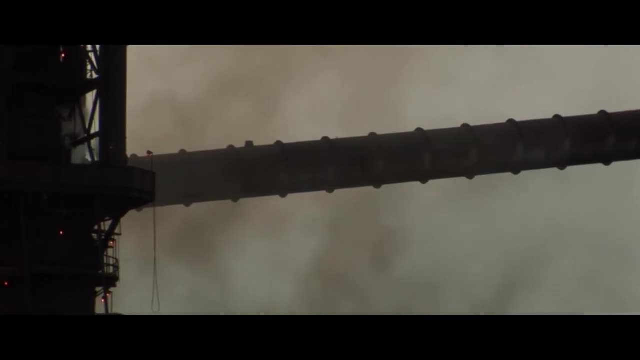 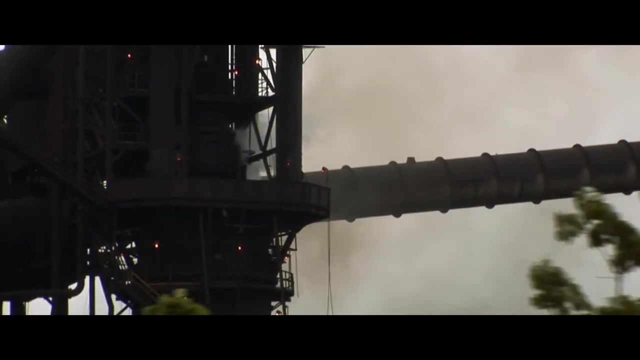 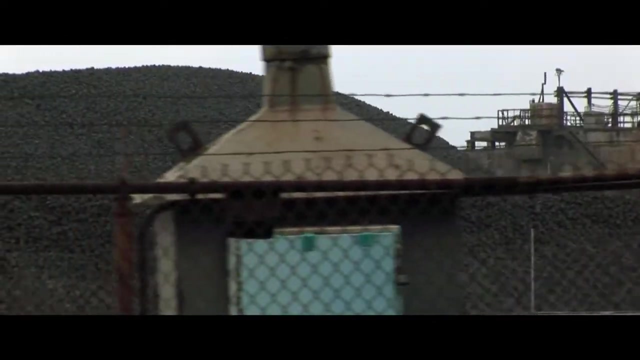 I can hardly speak it, but that is what happens. A brother kills another brother without even knowing that when you kill your brother, you kill yourself. I'm sick and tired of hearing black mothers crying because their black boys keep dying as we sit in these seats, While ain't a nigga politician lifting one damn finger. 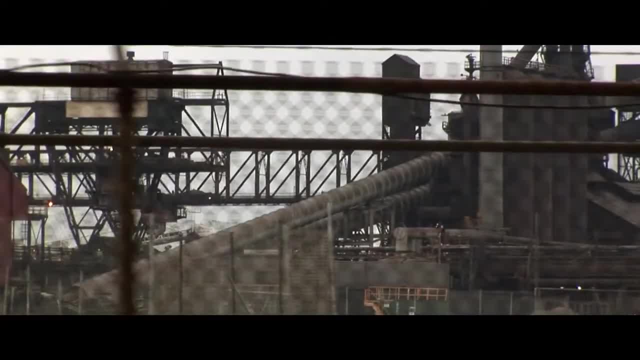 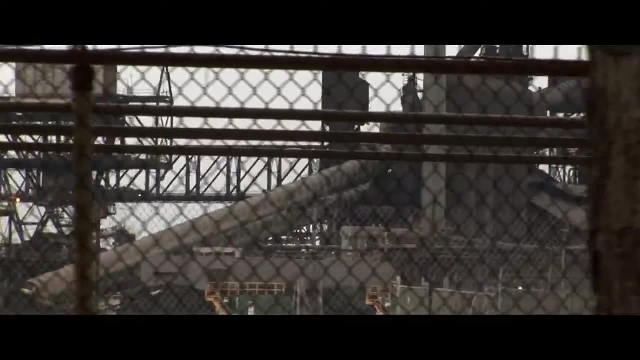 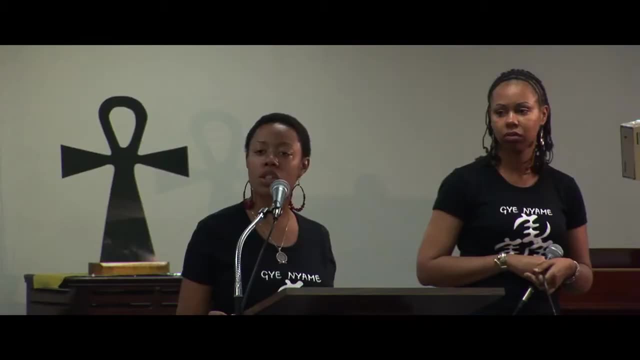 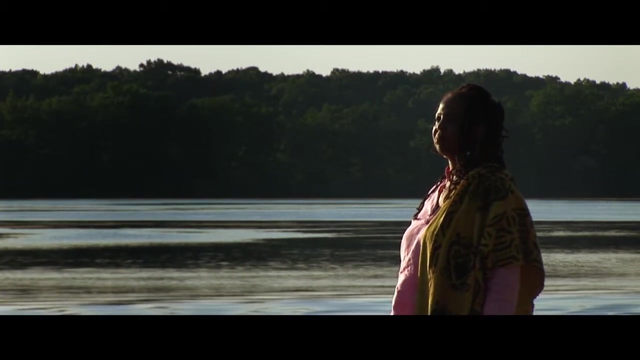 to stop the madness that's polluting our streets? When will we let this nonsense stop? When will our sons let their guns drop? Who's going to pick this strange and bitter crop? He's supposed to be here. He's 19 years old. 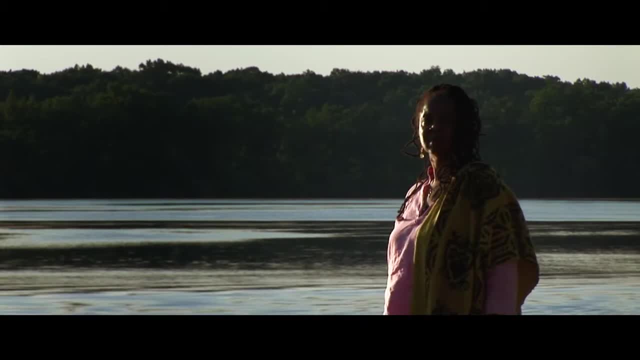 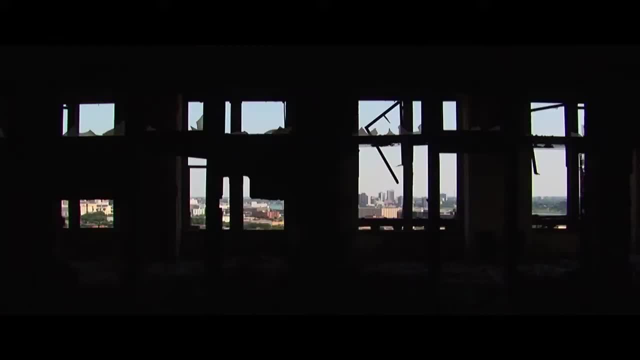 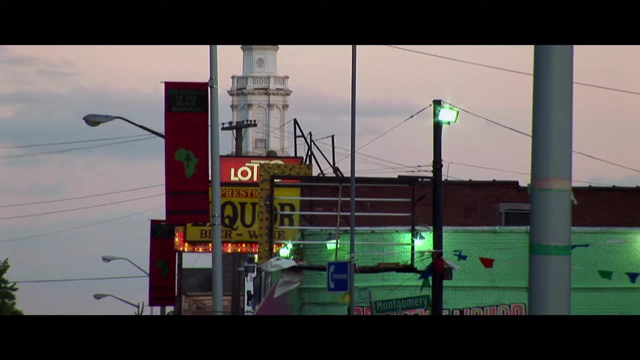 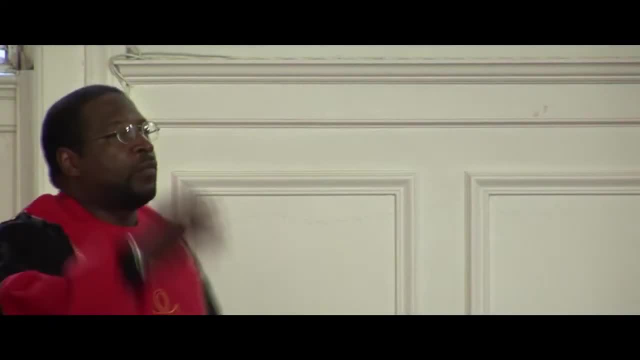 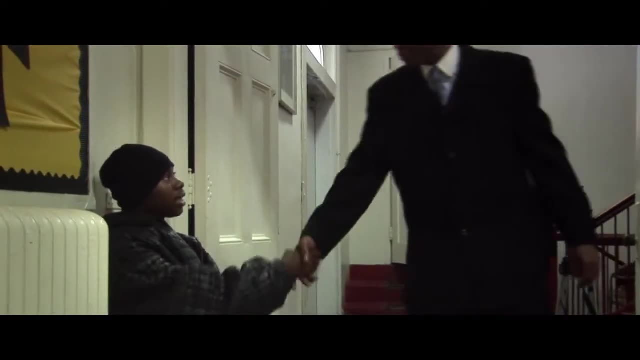 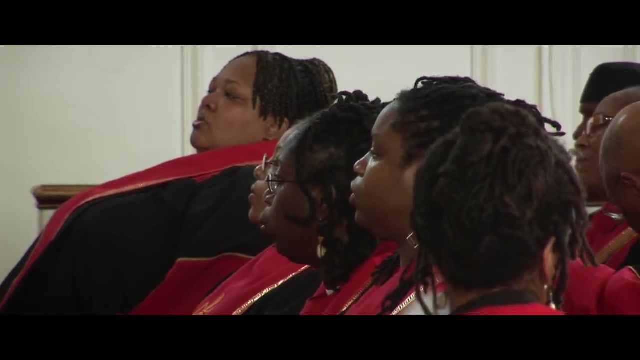 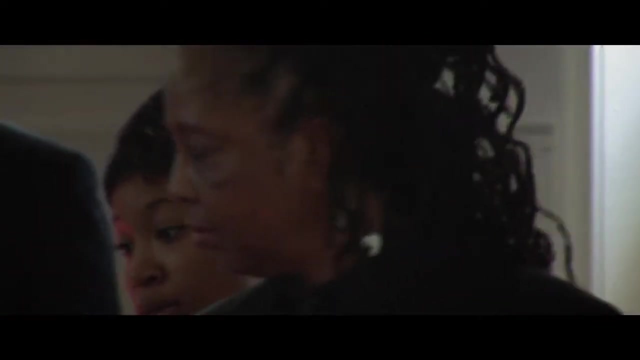 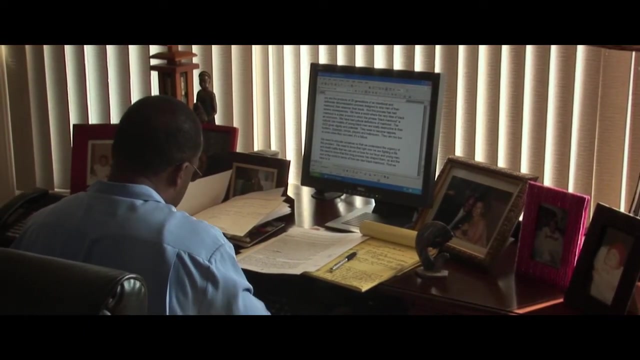 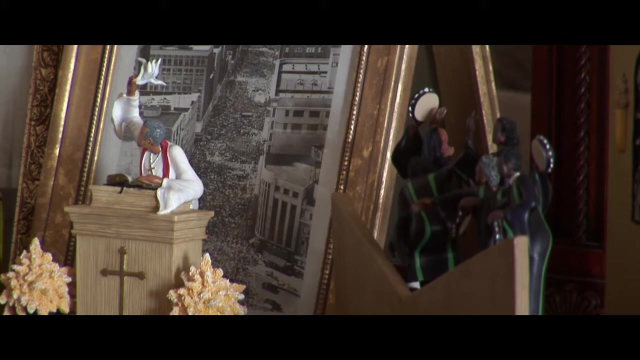 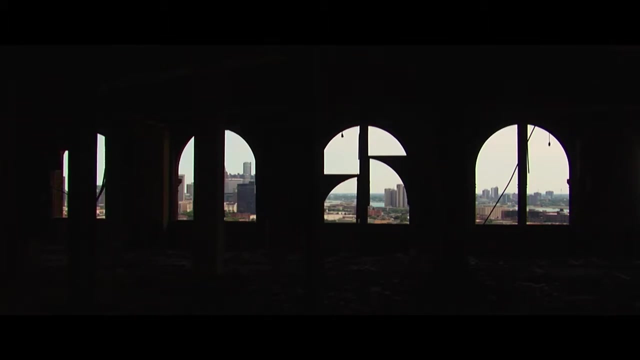 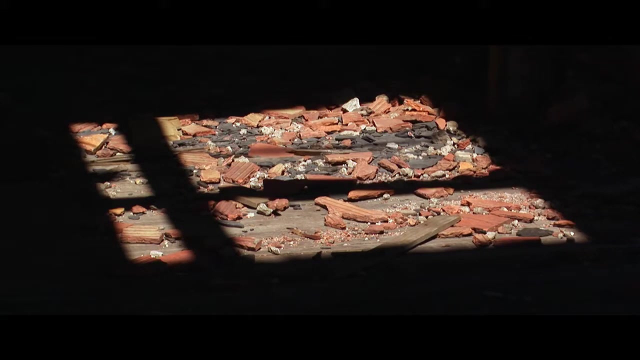 We'll be right back. You remember the story: they cried to God, praying for deliverance from their slavery, and the Bible says that God remembered the covenant and sent Moses. You remember the story: God sends plagues on Egypt and finally, after 10 plagues, Pharaoh tells them to get out. 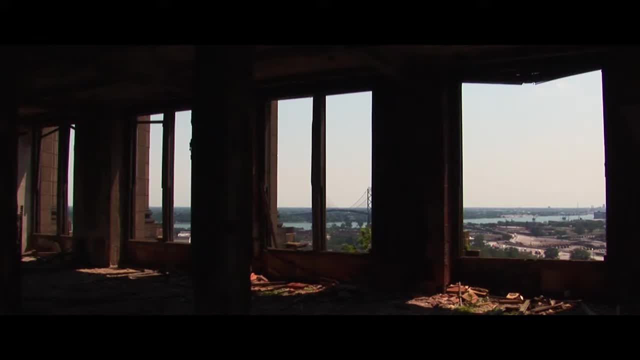 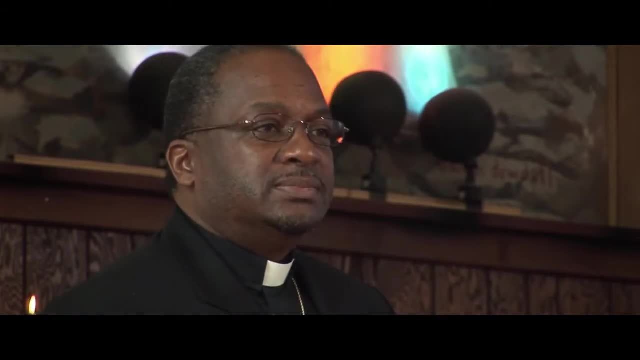 Get out, Get out And they pack up head out, walking fast and singing: Freedom, Freedom. They're walking fast and singing. It's a great day, It's wonderful. We are no longer enslaved. No more bricks without straw. 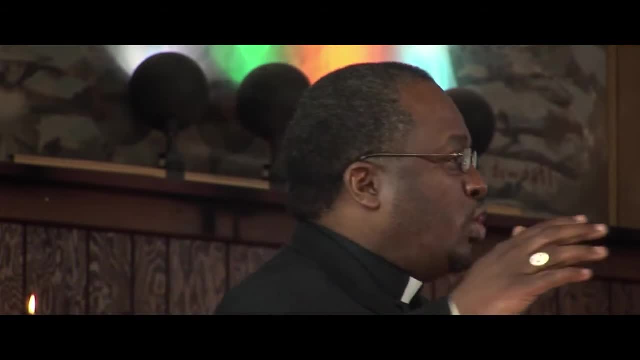 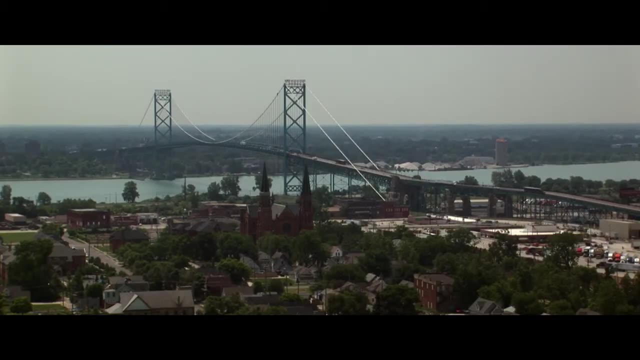 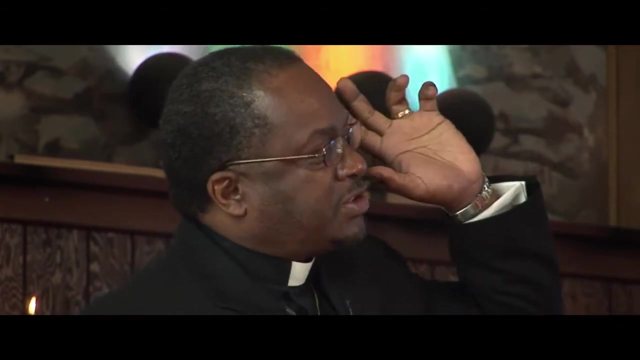 No more building pyramids, No more doing whatever we were doing. We are able to leave, to go get out. We're leaving, We're leaving. Then they realize We don't know where we're going. So God then provided a pillar of cloud by day and a pillar of fire by night to guide them across the wilderness, take them to where they're supposed to be going. 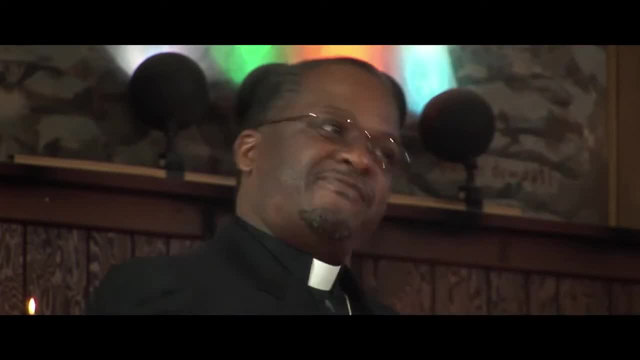 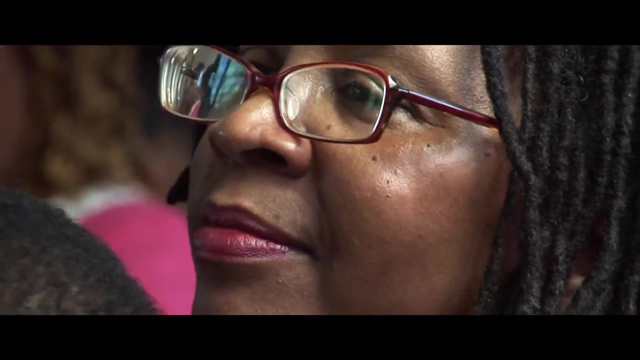 So they start following it, pillar of cloud by day, pillar of fire by night, go back to walking fast and singing freedom, freedom, having a good time. And then they think, wait a minute, Wait a minute, What are we going to eat? 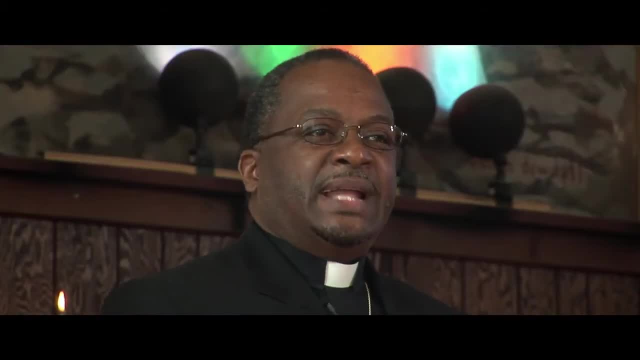 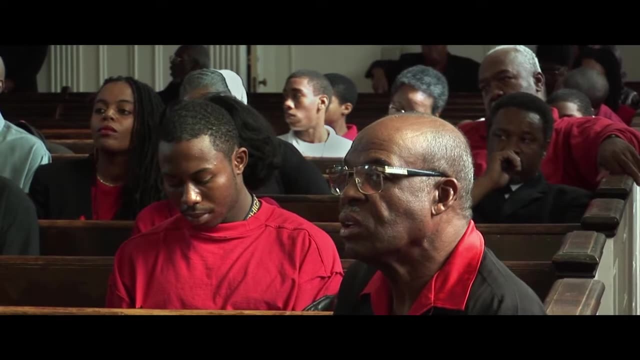 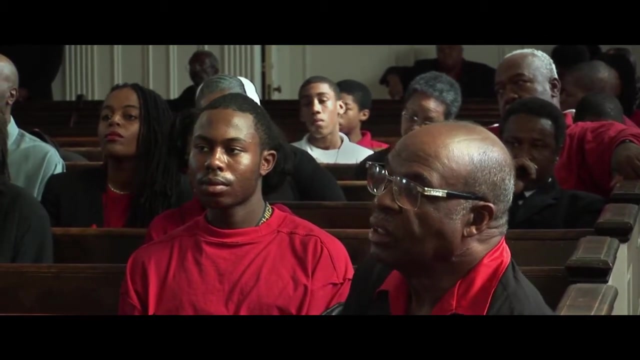 Every time they encounter a problem, they have no answer for the problem that they have encountered. As soon as the next challenge arises, they repeat their slave mantra and negative affirmation: Better to serve the Egyptians than die in the desert. We don't want all this problem. 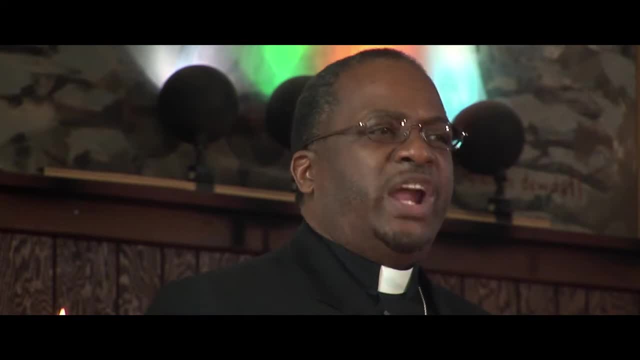 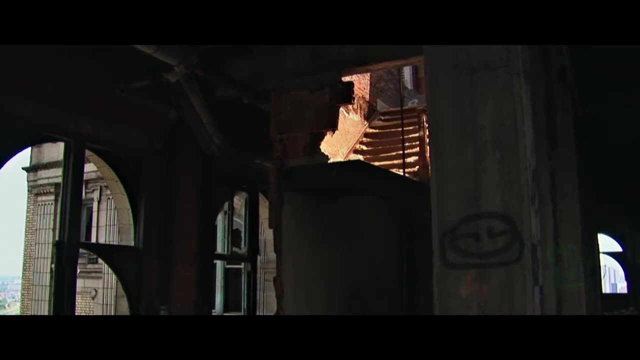 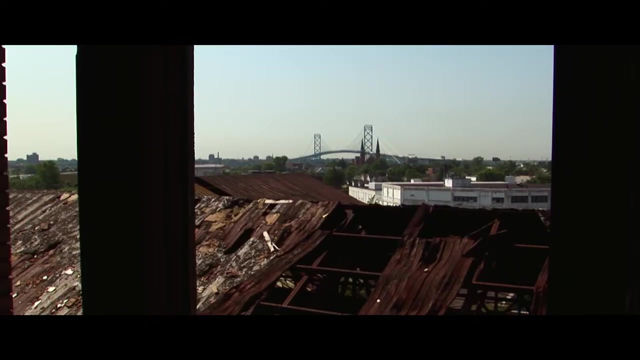 We don't want them to figure all this out. We don't want them to figure all this out. We don't like freedom. We don't like freedom. Freedom is not heaven. Freedom is nothing but an honest opportunity to struggle and build and grow. 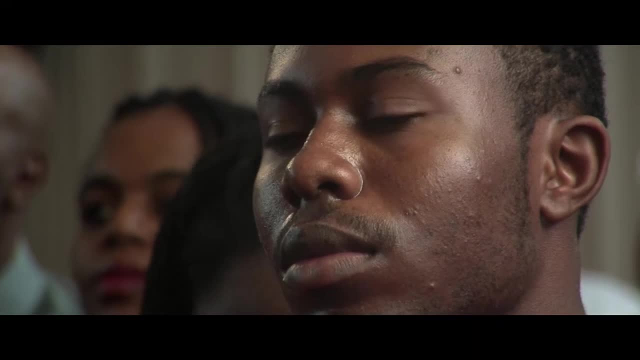 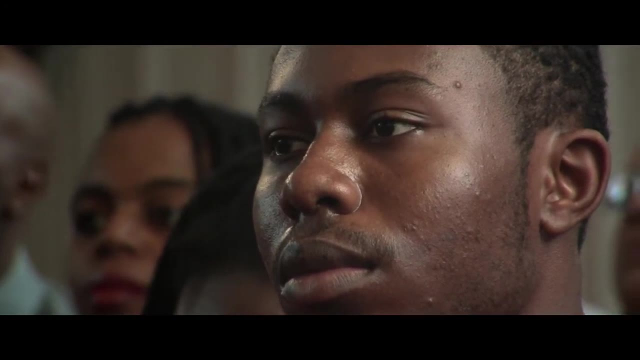 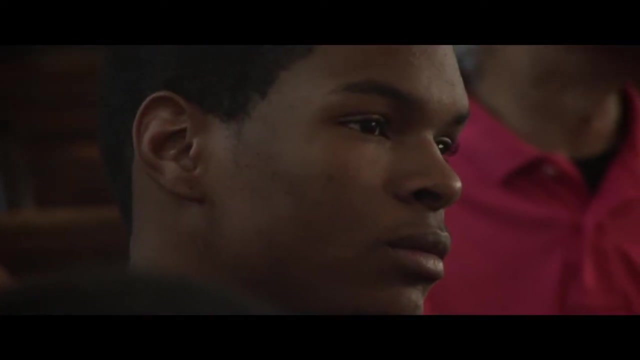 It ain't no promise. It's an opportunity. It's a chance. Freedom is a chance, Amen. It took two generations for Israel to learn to live freer than in the Promised Land. We don't know how long it'll take us to learn. 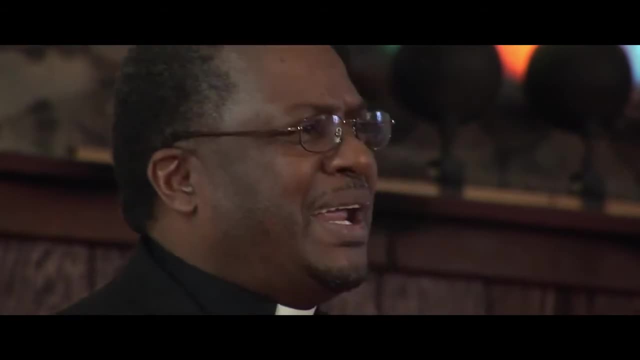 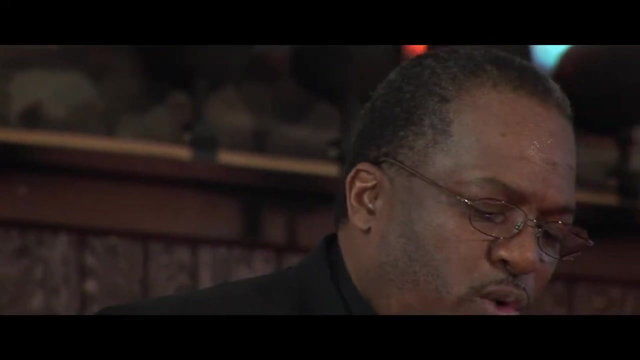 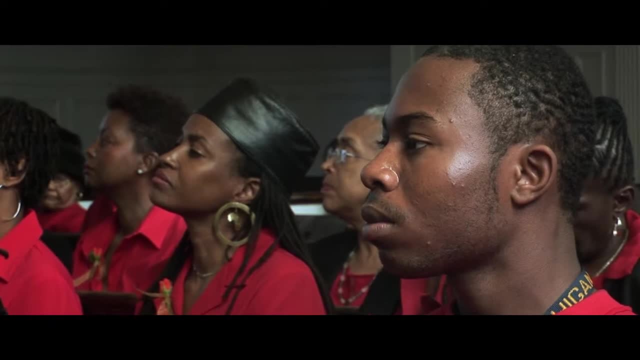 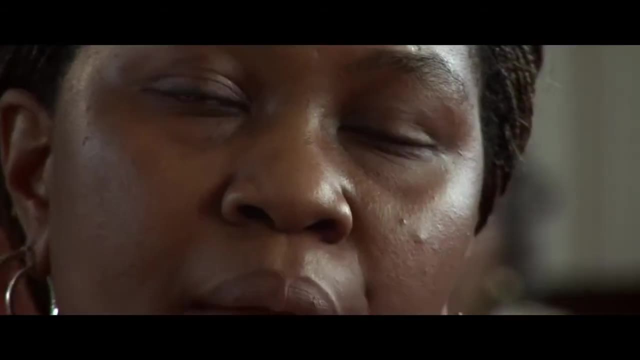 We can work hard, We can, We can, We can. In the Shrine of the Black Madonna, we are dedicated to this work. We believe that the Church has to be a counterculture—a counterculture of positive role models, positive. 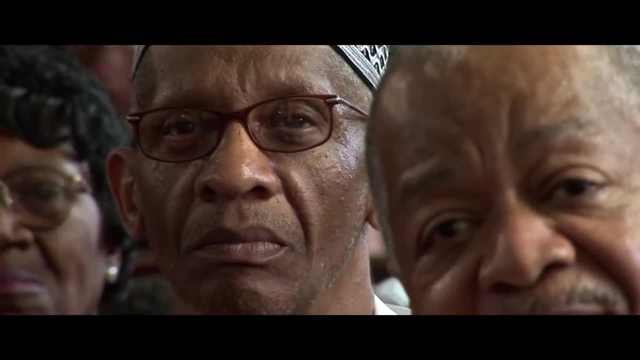 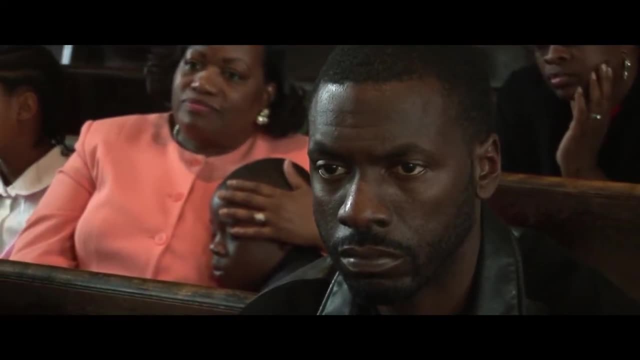 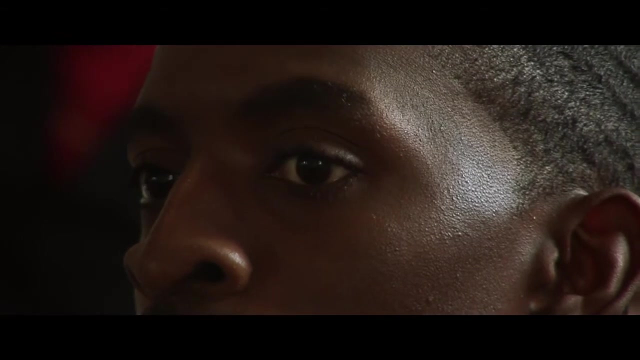 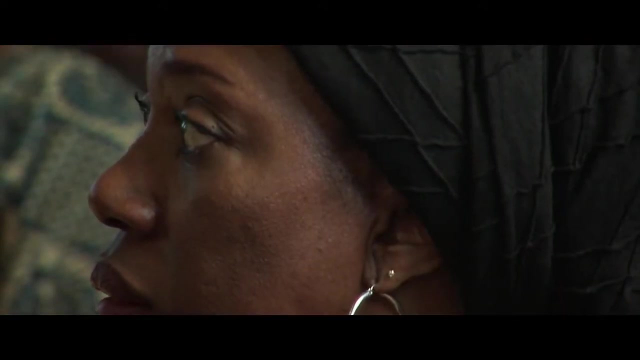 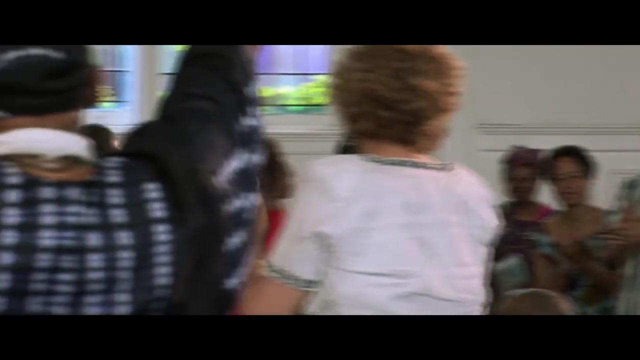 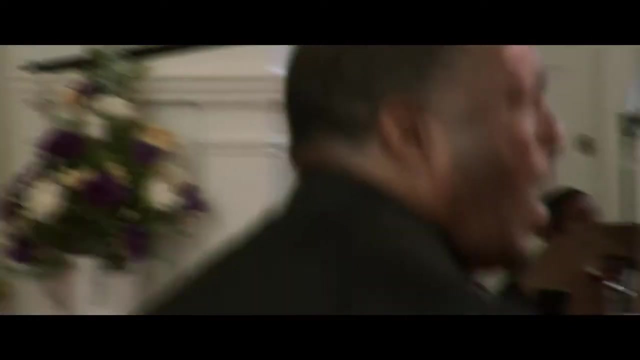 influences and positive action. So we are calling on Father's Day, real men, to be men For all those hiding in a cave on the ground. we are saying to you: almighty man of palabra, God is with you, God is in you. Almighty man of valor, if you made mistakes, say I'm sorry and move on. Almighty man of valor, do something positive with your life. Don't drink it away and cry it away. Don't give it away. 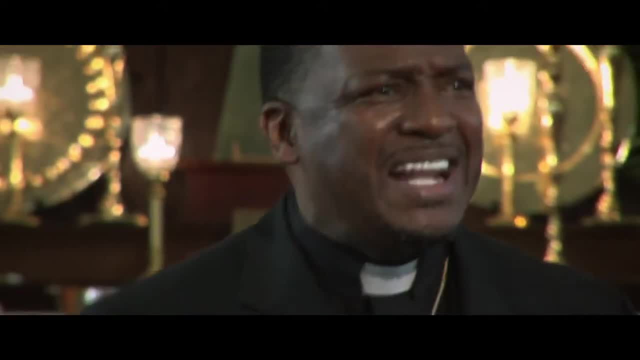 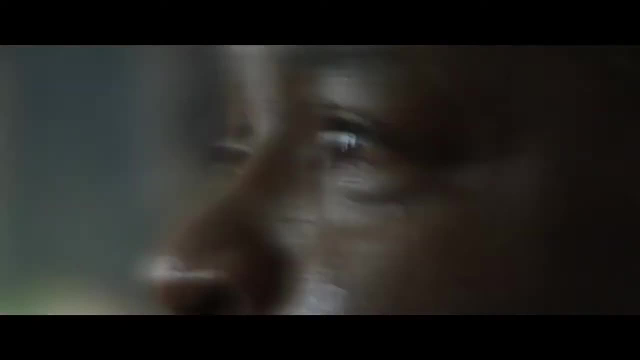 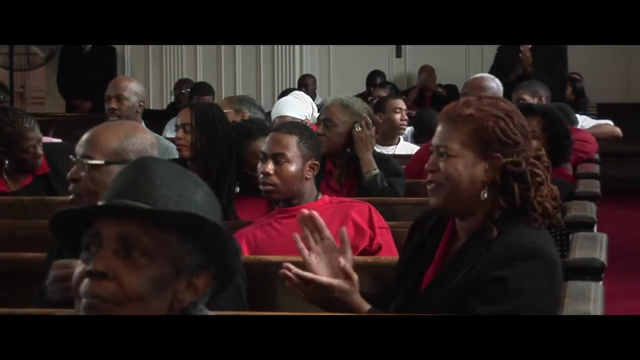 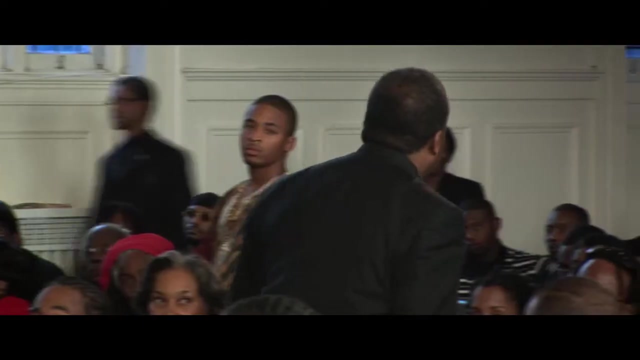 Don't let somebody steal your dignity and your humanity and have you waste your skin, your life, your DNA. Don't have them waste it, Just living, breathing, but meaning nothing, doing nothing. Almighty man of valor, We stand here as a black organization with resources, with institutions, with the ability to make a difference. 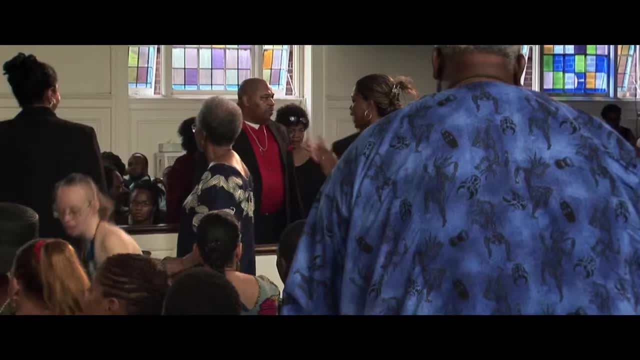 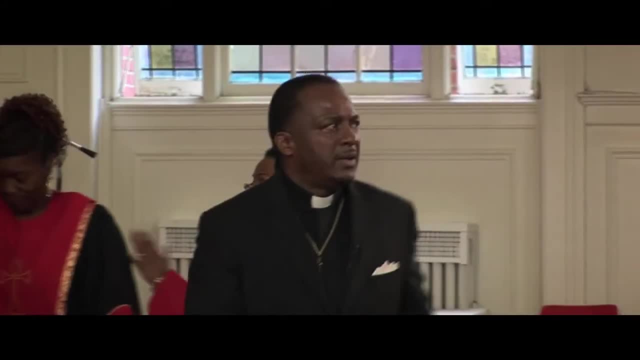 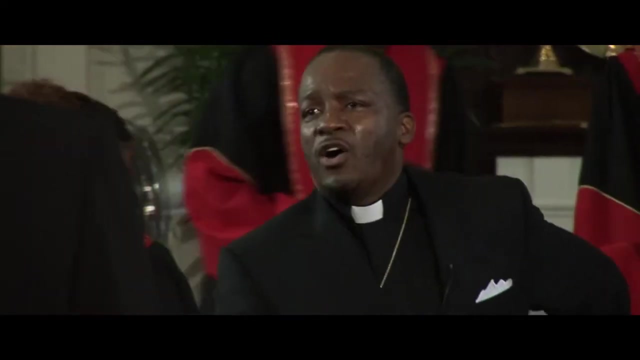 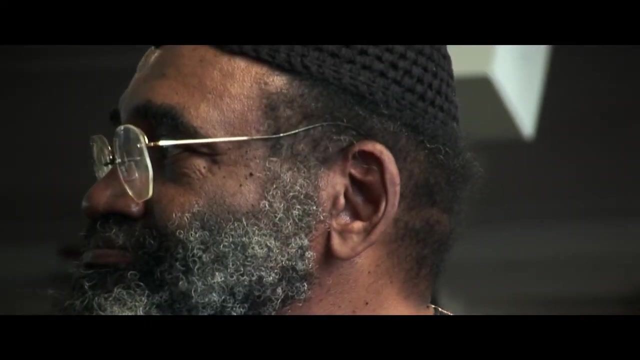 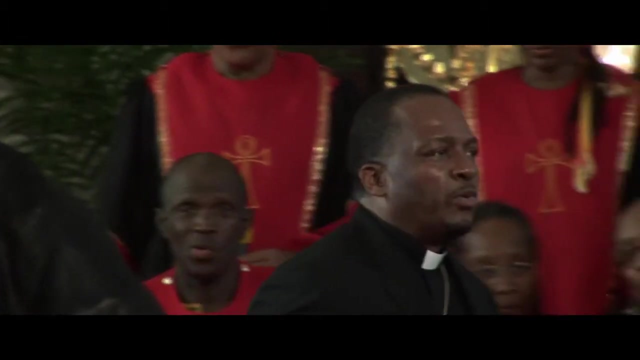 Now we need some brain power. We need some brain power to run them. We're going to open the doors to the church. We're going to open the doors to the church If you want to join us in our mission to restore our people to our original place of power and dignity in the world. 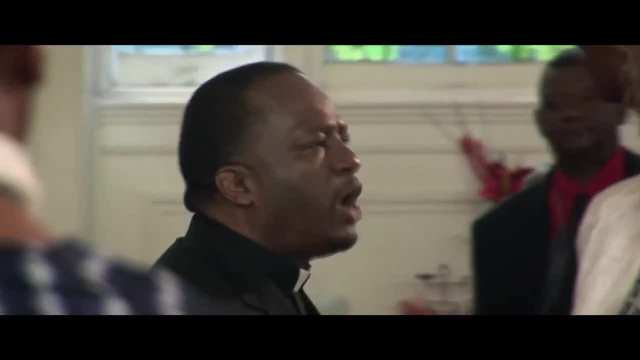 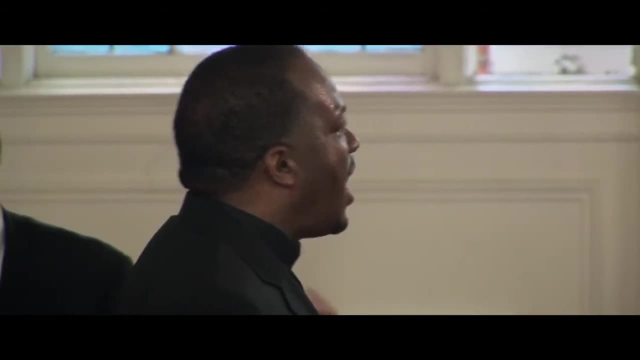 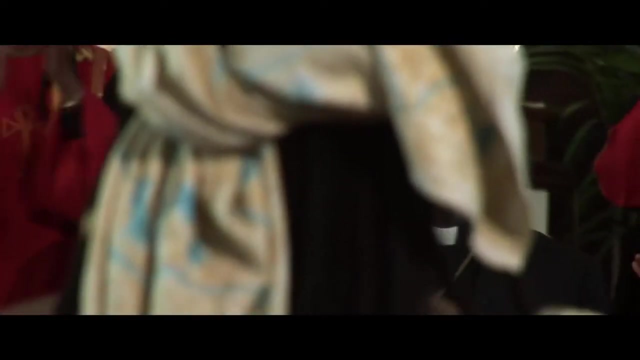 if you want to be excellent, so that you can contribute excellence to our great mission, we're going to open the doors. If you want to serve God and praise him, too, we're going to open the doors. We're going to open the doors to the church. Move on out and come on down the aisle. 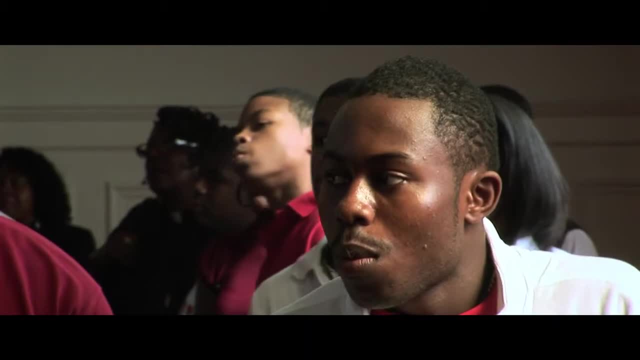 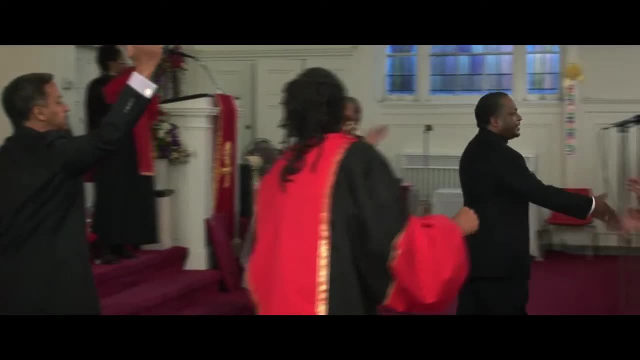 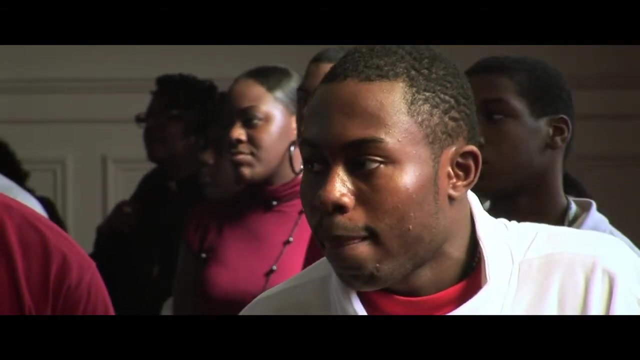 Stand up and stand up. The gospel is with you. The gospel is with you. The gospel is with you To Jesus. It is with you. Stars shine like a suitor. your strength is with us. Now you're living your life. 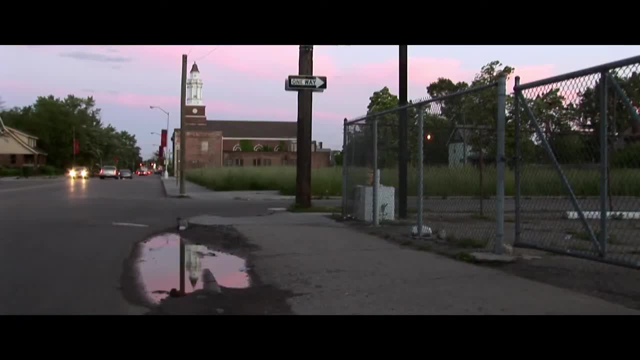 Now you're living your life Today of all days of faith. please fight class戰 and have an open heart, like a suitor that may smile Next že ztenijte zteníkan. I'm a p finde Now, great, great. 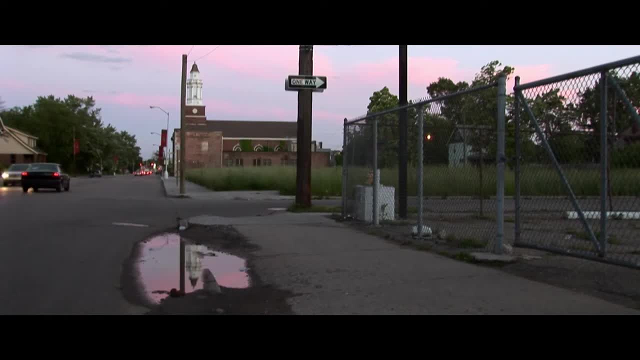 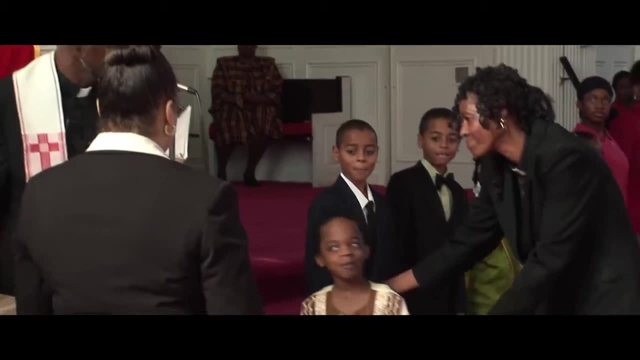 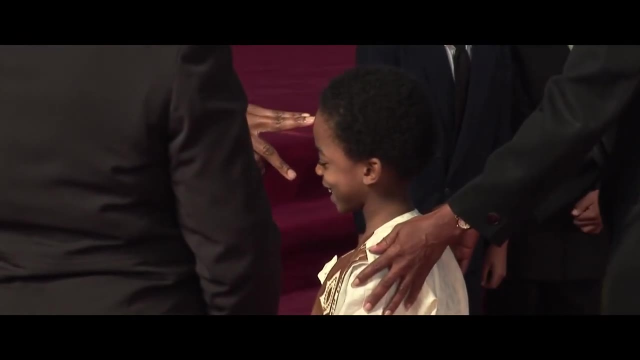 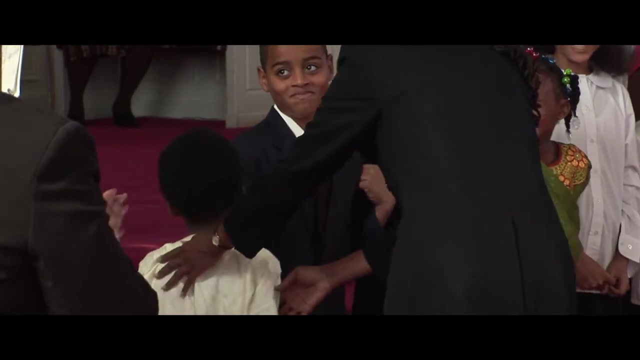 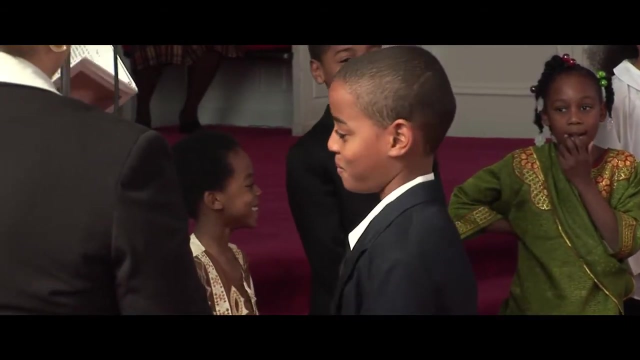 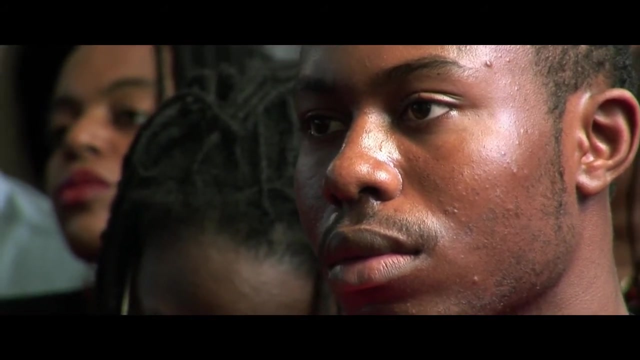 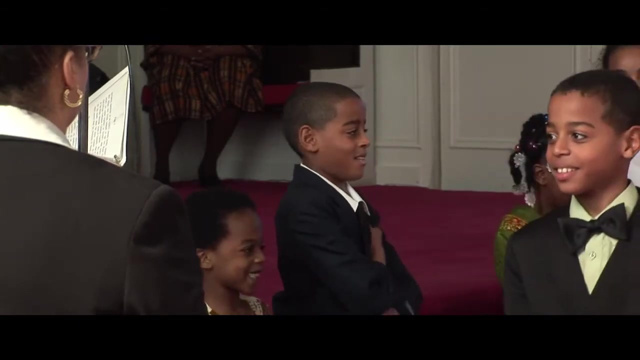 Loyal, Loyal, Loyal, My Dance and dance. Brother Jaylon Jordan. Brother Jaylon, we baptize you into the black nation. Brother Justin, Jordan. Brother Justin, we baptize you into the black nation. Brother Julian, Brother Julian, we baptize you into the black nation. 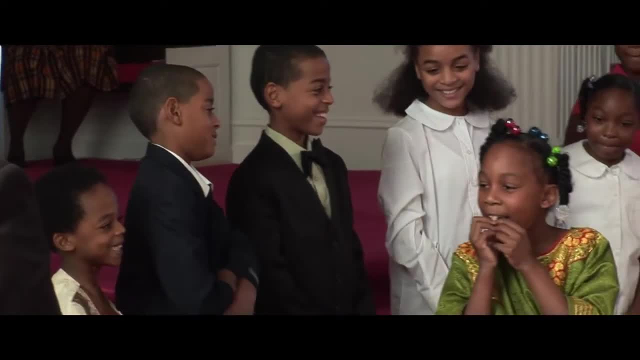 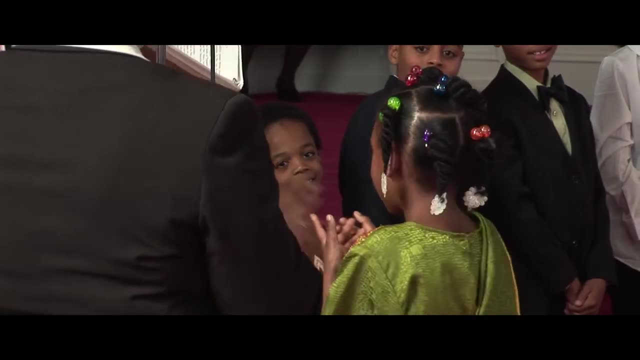 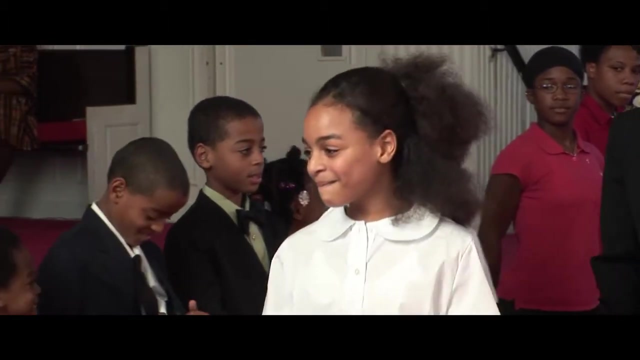 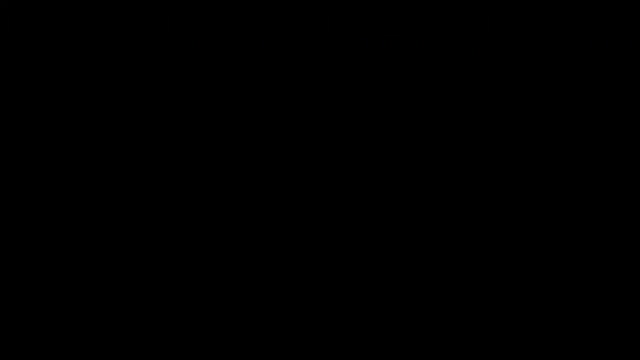 Zarianna Williams. Zarianna, we baptize you into the black nation. Arianna Jordan. Arianna, we baptize you into the black nation, Jade Oliver. I believe that human society stands under the judgment of one God, revealed to all and known by many names.